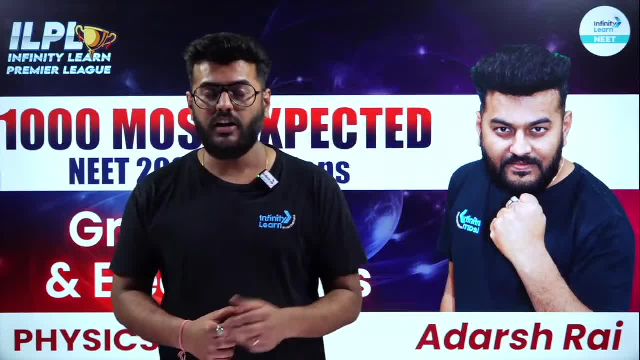 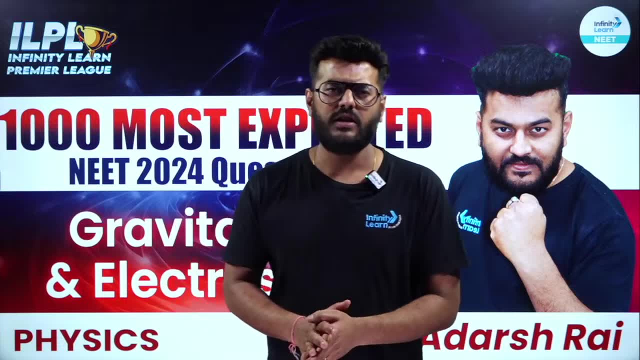 For example, if I talk about Motion Under Gravity, Satellite Motion or Kepler's Motion, These topics are not related to Electrostats. There are many topics in Electrostats as well. For example, Capacitance is not related to Gravitations. 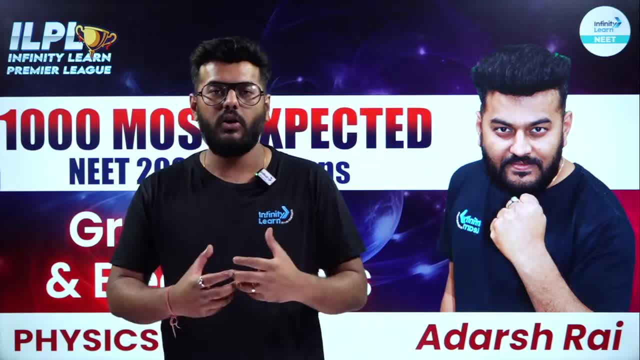 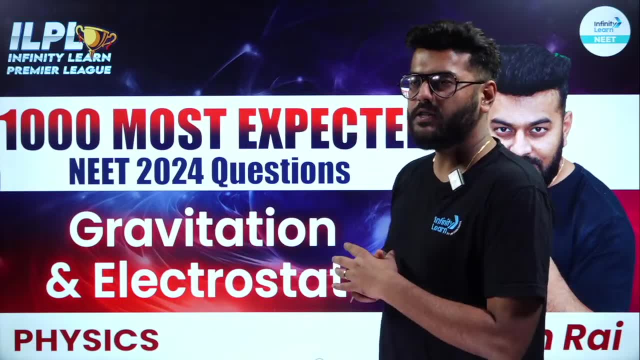 So we have to see the individual topics, the similarity and the dissimilarity, And it will be a very good session. I hope you are going to love it. Now, come on, Come quickly. How are you all doing? Abhishek? good afternoon. 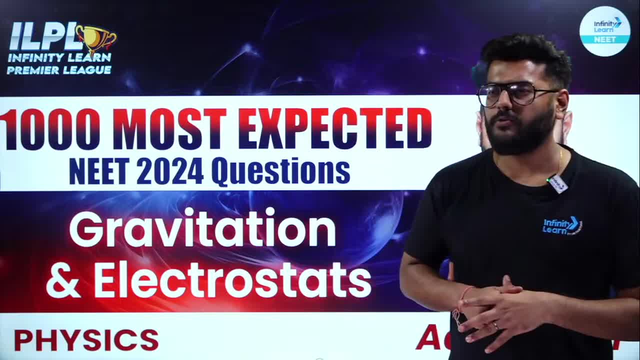 Savage Gaming. Hi, How are you Apoorv, good afternoon. Will there be a Capacitor in this or will there be a separate session? No, there will be a Capacitor in this. Don't worry, Sir, I don't know Hindi. 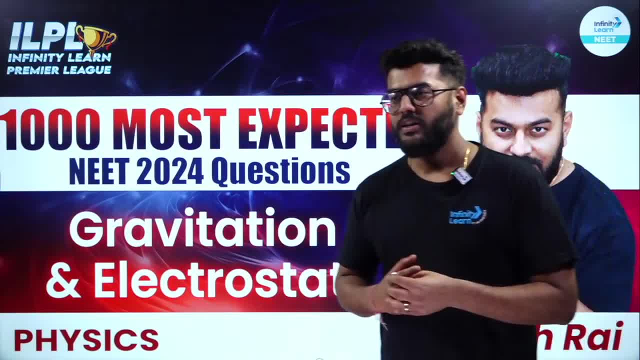 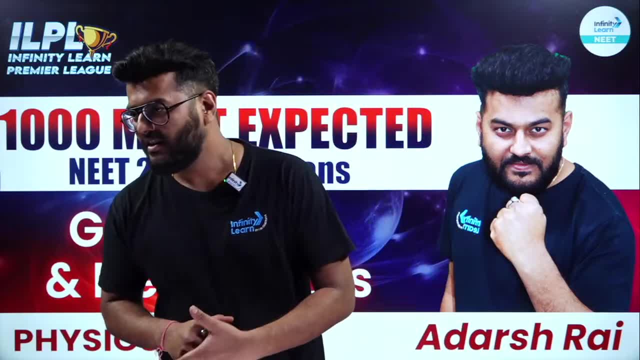 Can you explain in English? I will try my best to speak in English. The words, the letters, the things which will be there are mostly in English, But the explanation will be in Hindi. If you face any difficulty in between, please do let me know. 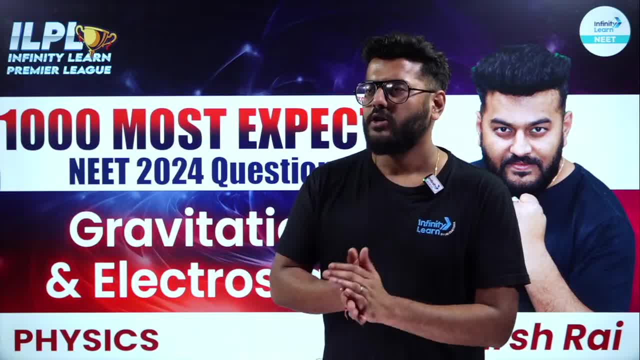 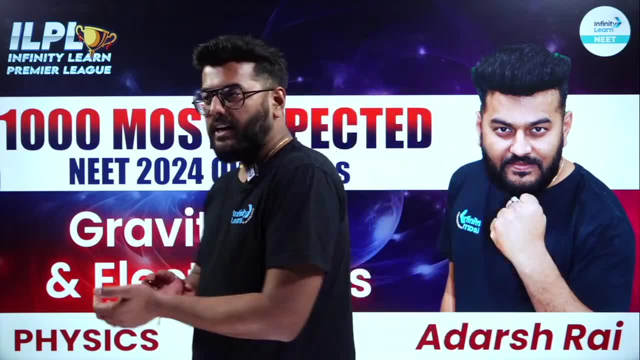 I will be very happy to explain you again. Okay, Scored 170 and 180.. That's very good, Very good. In which one My name is Sujit? Okay, Hi, Sujit: 170 and 180.. 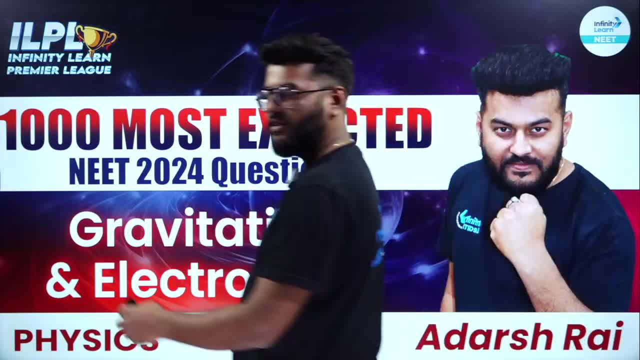 That's a good score. Very good, son, Abhishek, very nice. Take 180.. Then only two questions are left. Right And two questions are left. I think I have done it wrong. That's why it is 117.. 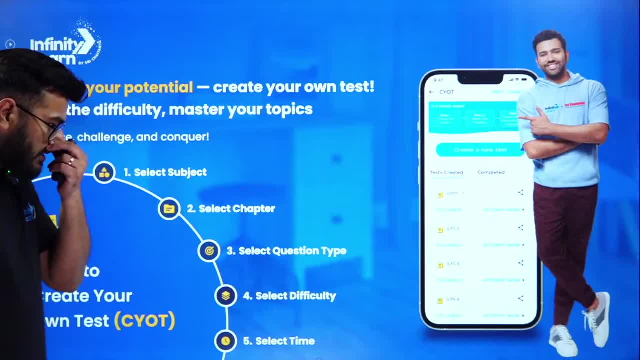 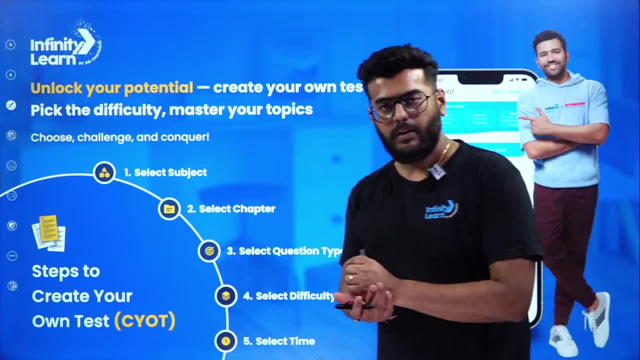 Come on. So let's start today's session Before moving forward. as I say in every session, please try CYOT as soon as you see the session. CYOT, Try it. CYOT is free of cost. Please download it on the application. 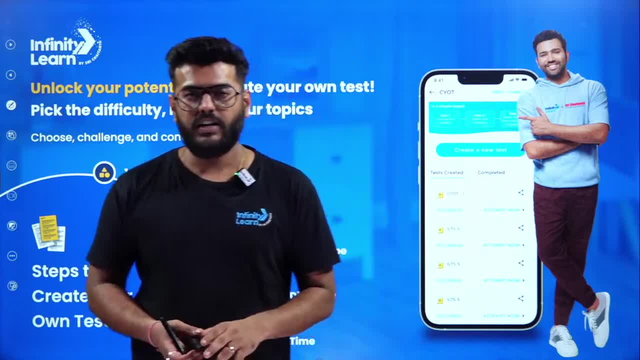 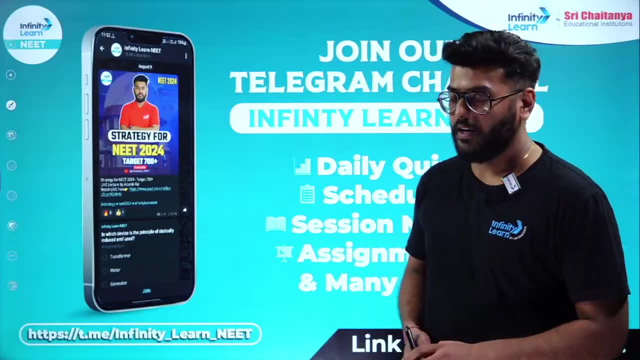 And as soon as you register on the application, you can very easily avail the CYOT feature where you can make a test and study yourself that how we are performing. You will get all the notes of today's session on the Telegram channel, So just after this session it will be uploaded there. 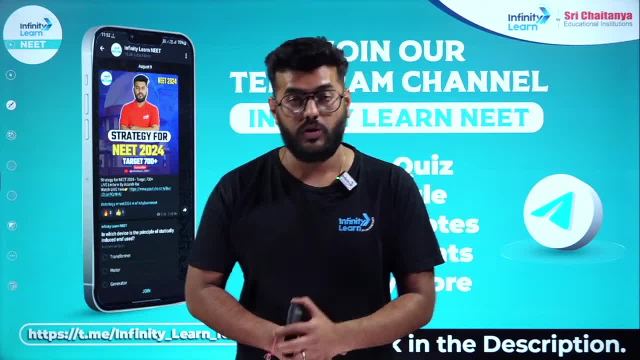 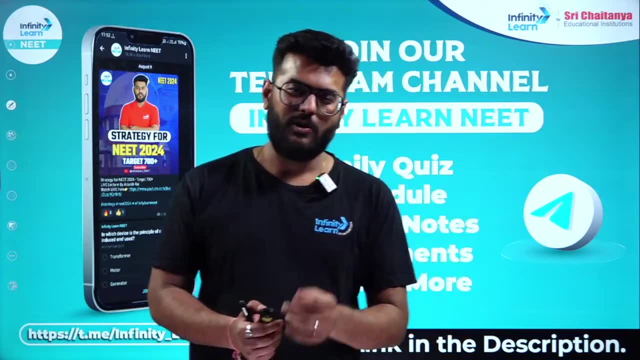 Those who have not joined the Telegram channel, please do join the session. And those who are watching the session from wherever, please like the session. There is only one request. Just like the session, Baba YouTube will be happy with it And these sessions can be promoted to the rest. 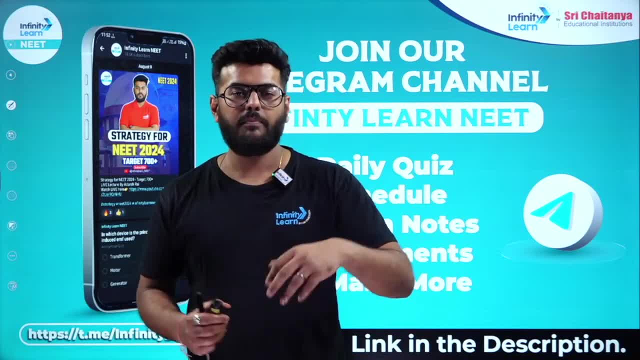 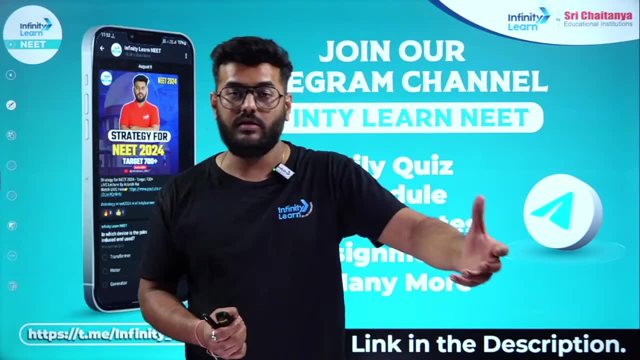 So if you do not want to help anyone, but maybe you want to help your friends or any other unknown person who may need these sessions, then please do let them know You will like it. Only then the algorithm of YouTube will promote those sessions. 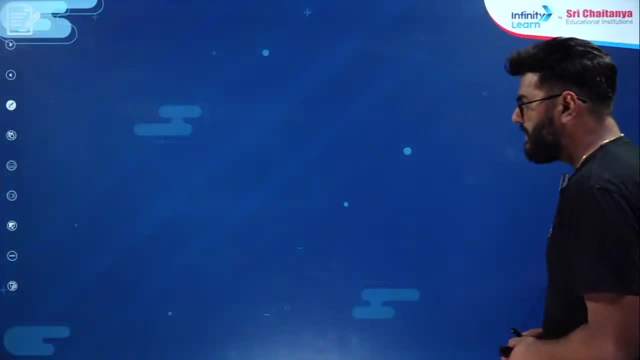 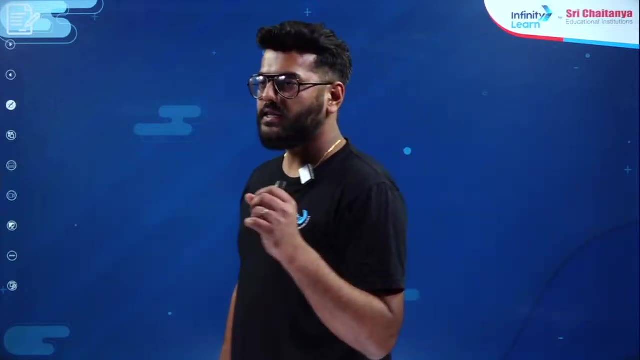 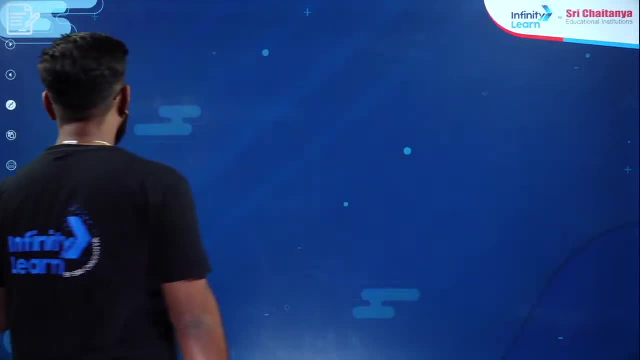 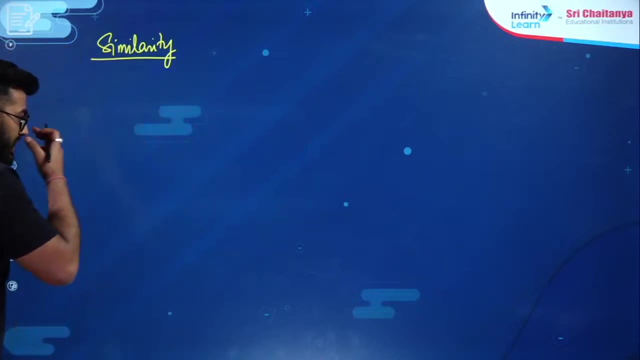 And in your electrostats. So let's talk about the similarity. First of all, let's talk about the similarity. Ok, If I talk about the similarity in gravitation and electrostats. So, first of all, The universal law of gravitation is that force is directly proportional to. 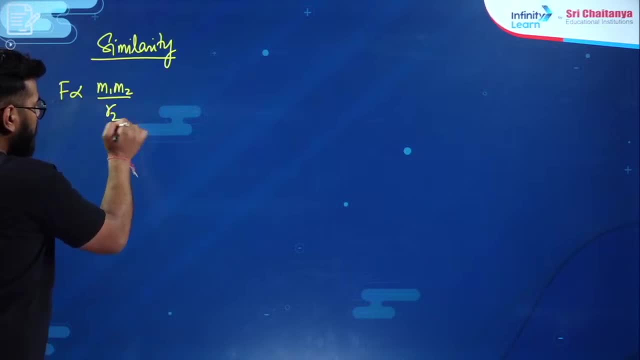 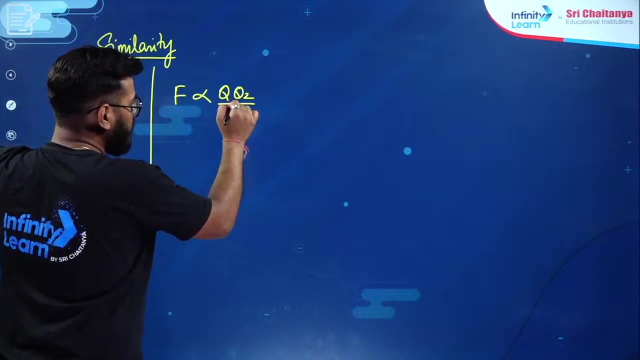 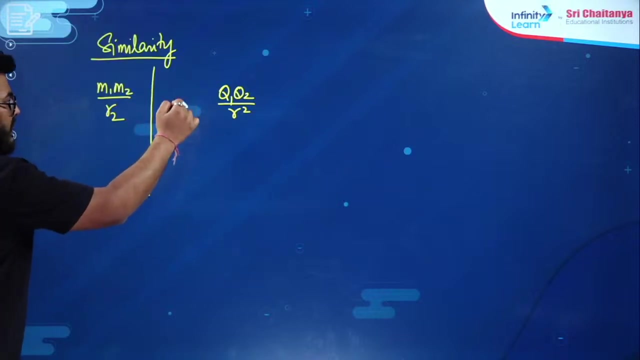 M1.. M2 upon R square, Just like in electrode, the electrostatic force, which is the chose, is directly proportional to q1 and q2 by R square. OK, Here the constant multiplied after the proportionality is G, and the constant multiplied here is K. 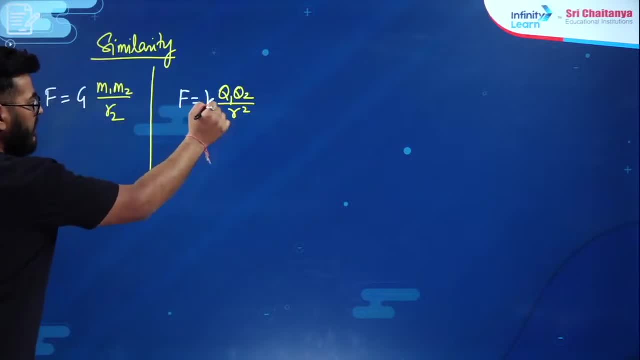 Here it is G and here it is K, Meaning the value of K is reciprocating G here, The value of K is reciprocating G here, And K is 1 upon 4 pi epsilon naught. This is the first similarity. 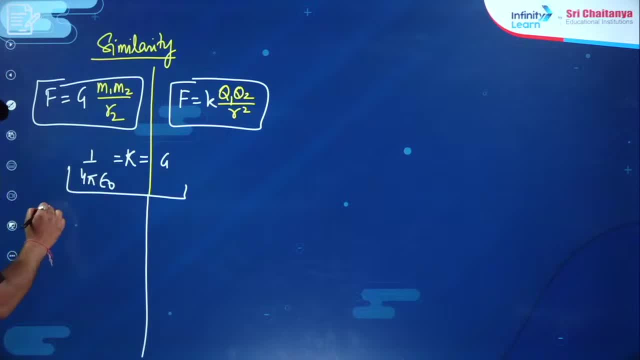 Then you will see the next similarities: in gravitational field, gravitational potential and gravitational potential energy. In all these things you will see the similarity. And here in electrostatic, when you talk about field, you will see the similarity. When you talk about potential, you will see the similarity. 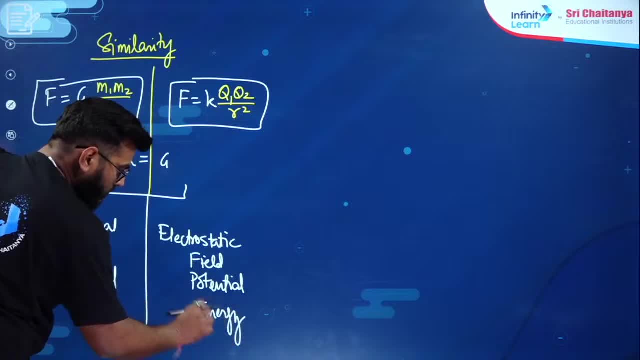 And here you will see the similarity. And if you talk about energy you will get to see the similarity there. So if we read one here, then the other can be done easily. But where 1 upon 4 pi epsilon naught is there, you can replace G. 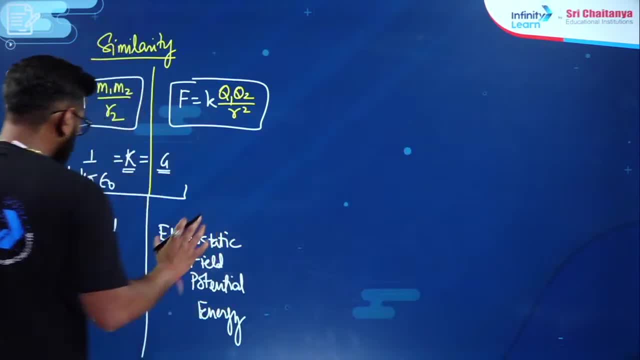 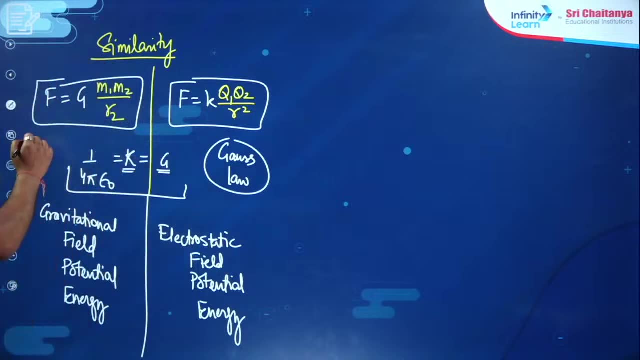 Along with that, Gauss law is also similar. For both Gauss law is also similar. Gauss law is also over here And Gauss law is also here. Here also the same Gauss law exists Here. Q enclosed upon epsilon. naught is there. 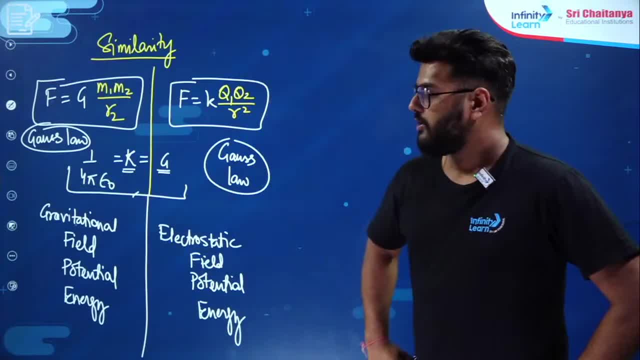 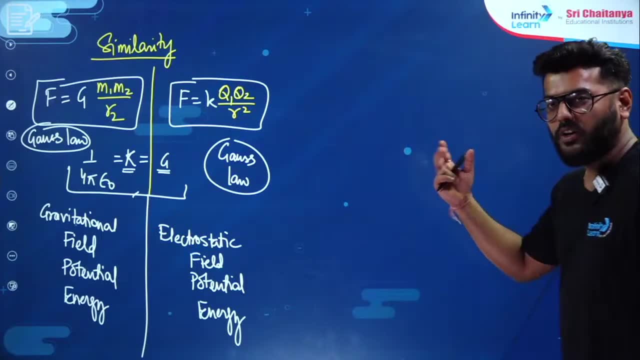 And it reciprocates the value of epsilon naught. So here, M enclosed into G into 4 pi, is there There? Q enclosed upon epsilon naught, is there, In gravitation, G into 4 pi? is there instead of 1 upon epsilon naught? 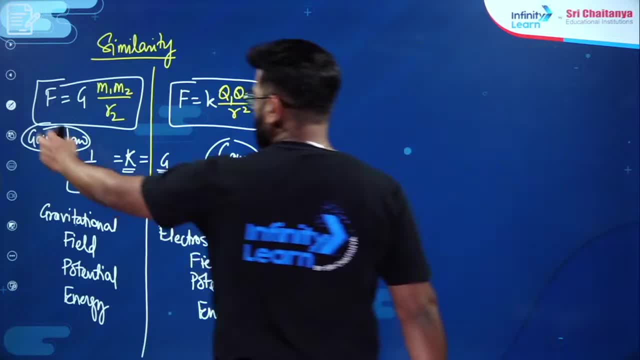 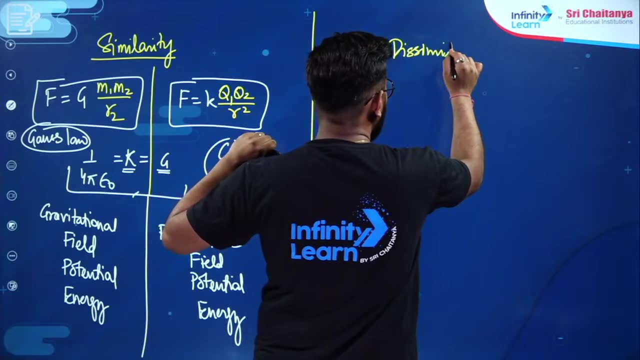 So I will tell you about Gauss law also. Now, what is dissimilarity? What is dissimilarity? See what dissimilarity is. So if I talk about dissimilarity, if I talk about gravitation, then in gravitation, sir. first of all Kepler's law is like this: 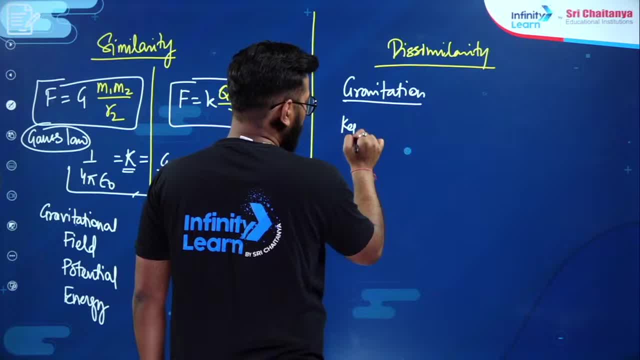 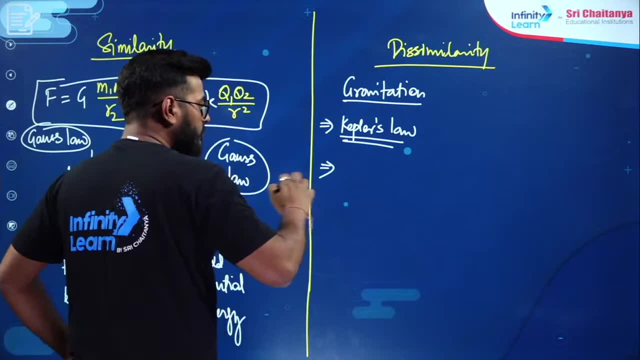 There is no law like this in your electrostats, So Kepler's law is an individual topic which we will have to study separately. The lecture will start with this only today. Then if I move ahead after Kepler's law, then motion under gravity: 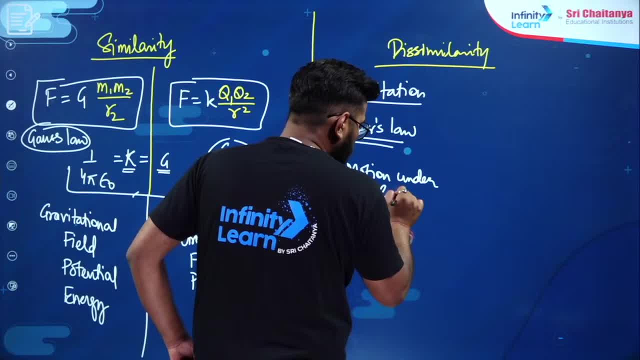 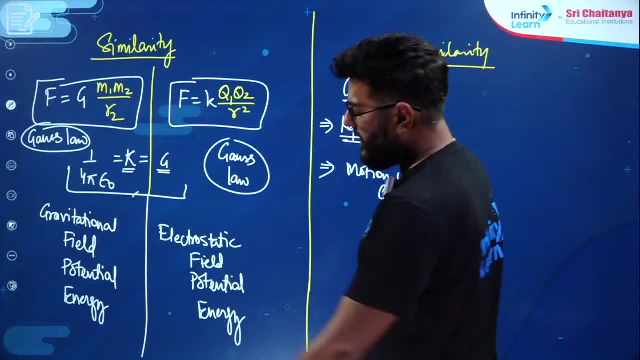 Now, if you see it in one way, then the motion under gravity, the gravity, the acceleration due to gravity, that is the magnitude of your electric field intensity. The magnitude of the electric field intensity is motion under gravity, which means acceleration due to gravity. 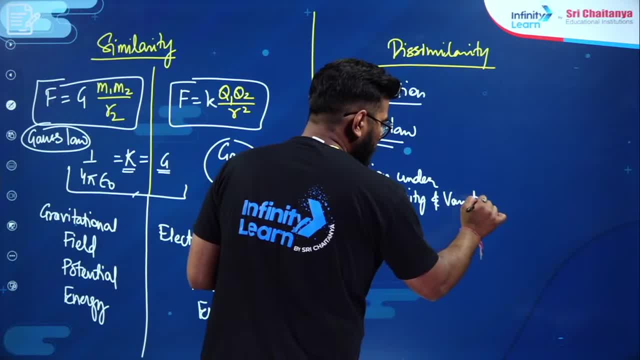 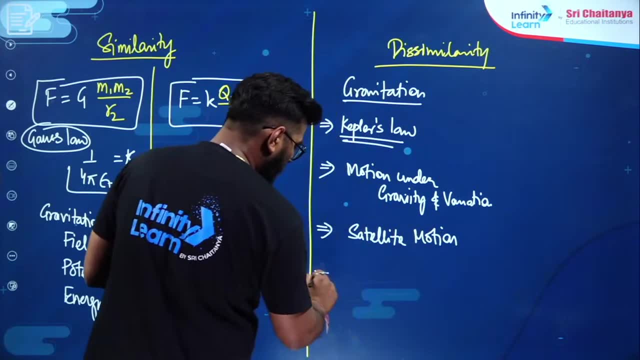 And its variation and variation. this is a completely different thing. Then after that I will talk about satellite motion- Satellite motion, not types of satellite satellite motion. And then after that I will talk about escape velocity. All these topics are individual topics of gravitation. 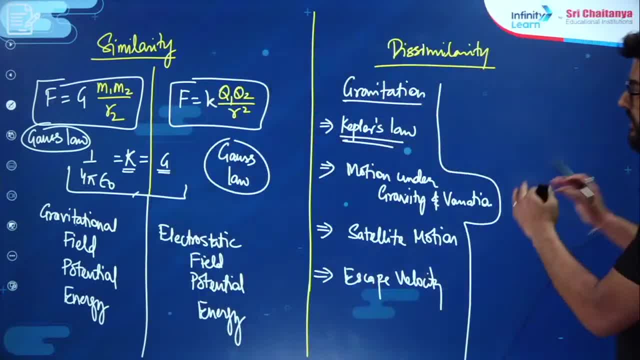 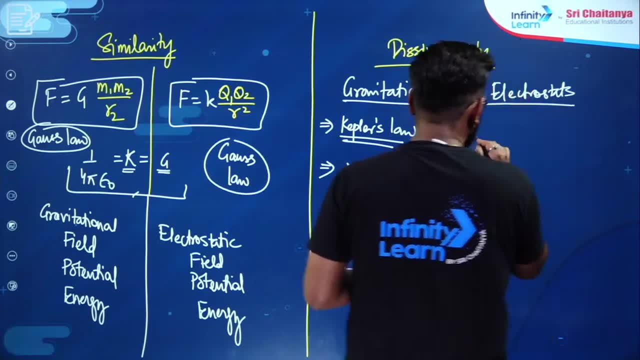 which have no equal importance with your electrostats. If we talk about individual topics in electrostats, then in electrostats you will see electric dipole first of all, which is an individual topic. After dipole, the next thing you will see. 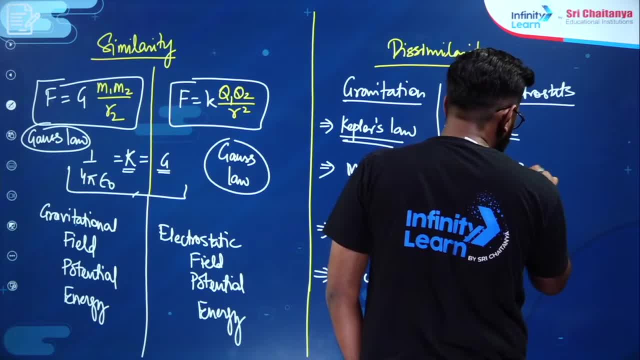 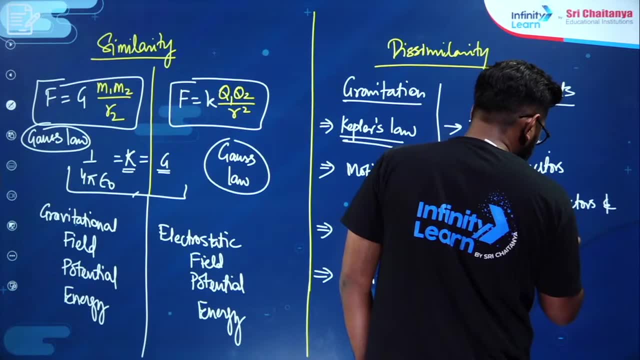 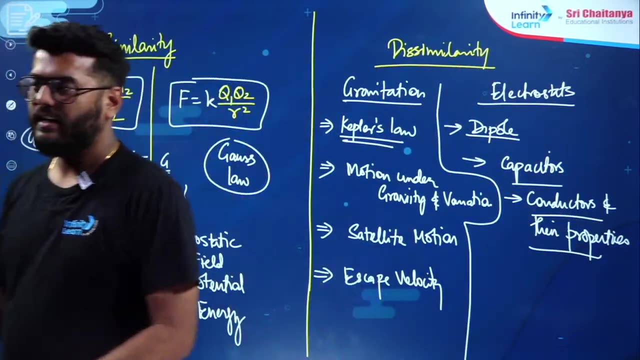 what is that going to be seen After dipole? the next thing you will see is capacitors- Okay. then after that, conductors and their properties- Okay. all these things will look different to you in capacitors, which is not linked to it. 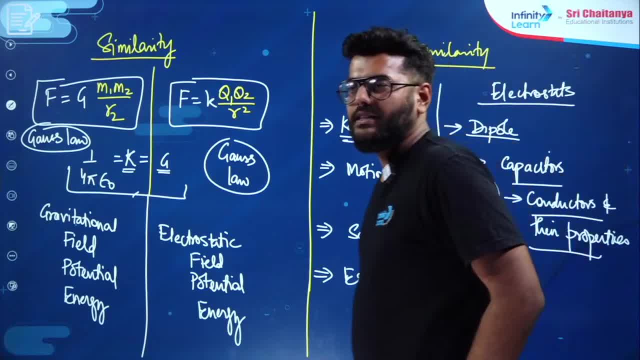 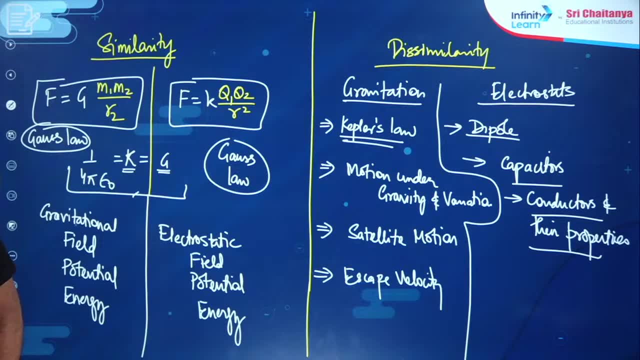 Okay, force in unit mass is kind of what field is. I am trying to understand. force in unit mass is kind of what field is. Force in unit mass is kind of what field is. No dear, I have to explain a little bit. 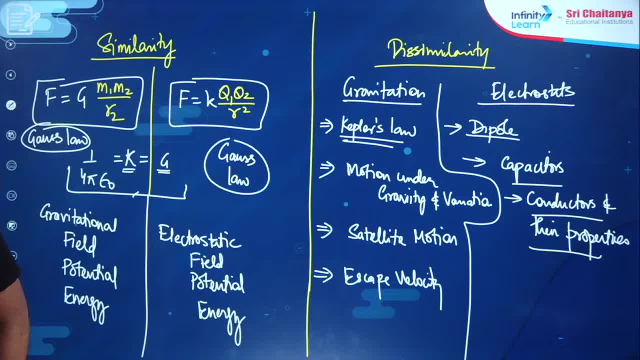 I am not able to understand what you are asking. The sign of ray optics is a mistake In the telescope. the second peak current was asked. RMS is written. Okay, these two are wrong, No problem, Okay, No problem. We have to learn from mistakes. 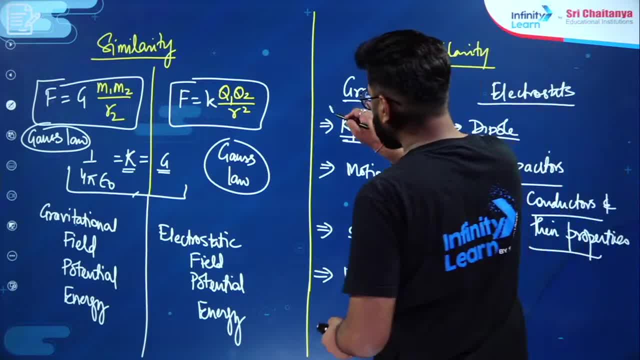 So let's start, sir. We will start this chapter with our story of Kepler law. First we will understand Kepler law of gravitation, Then we will jump to electrostats In the middle. we will keep jumping here and there. 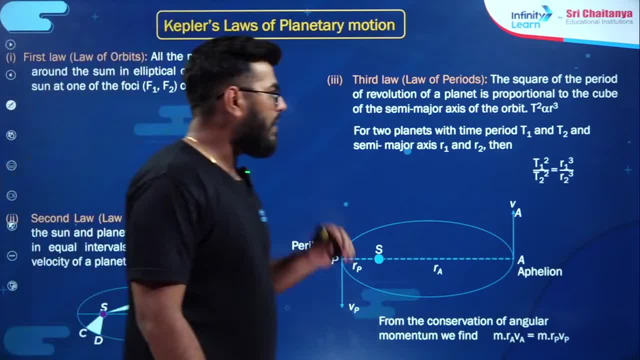 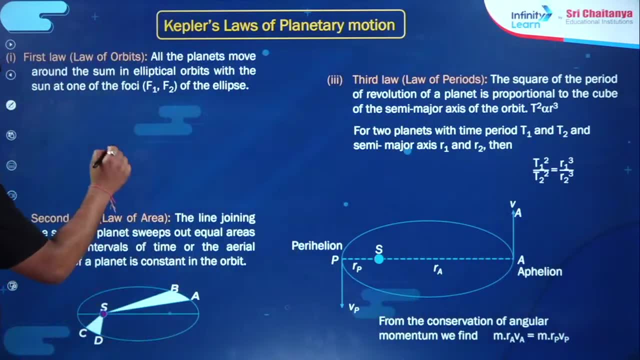 so that you will have a similarity and dissimilarity. so that you will have a similarity and dissimilarity. So here in front of you, three Kepler laws are given. The first law is the law of orbits. All the planets move in an elliptical orbit around the sun. 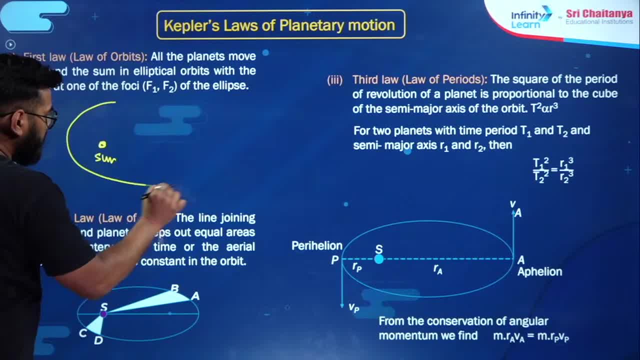 Right. This is a sun and the sun lives on any foci. The sun lives on any foci, Right. So the sun is here and the planets are moving in an elliptical orbit. Okay, The second one is the law of area. 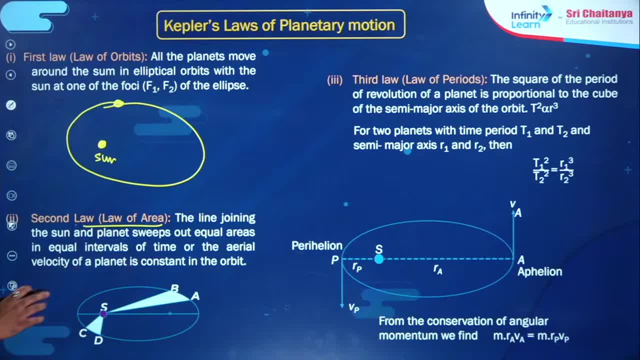 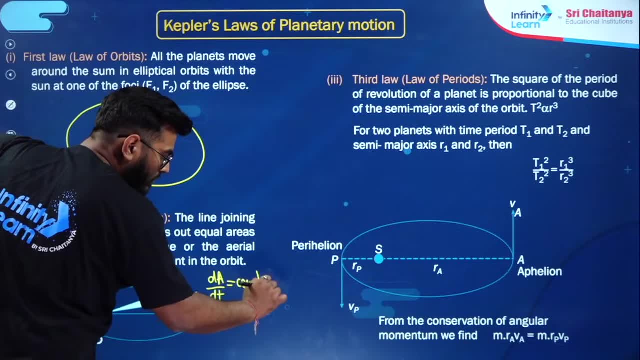 The law of area is that the equal area sweeps in the equal interval of time. That is, the aerial velocity of DA by DT is constant. This is constant. Now, one more good conclusion can be drawn from this, Which can also be drawn from this: 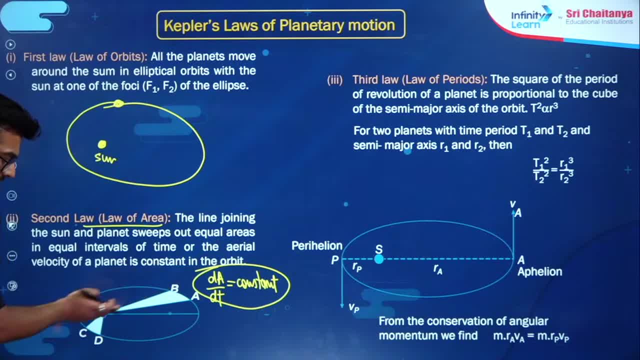 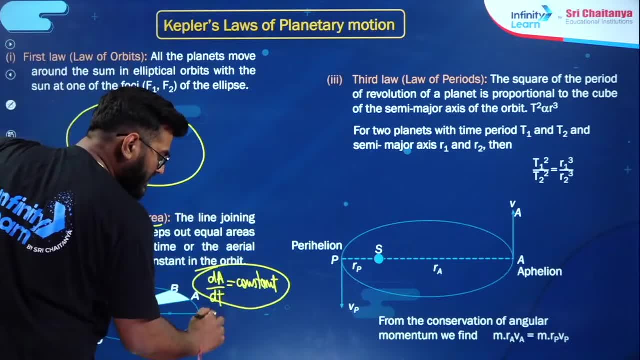 And the second one is that the only force on the planet is the gravitational force, And the axis of rotation is passing through the sun, So angular momentum should have been conserved anyway, Because the net torque is zero. But still, you can also deduce from this that the net torque is zero. 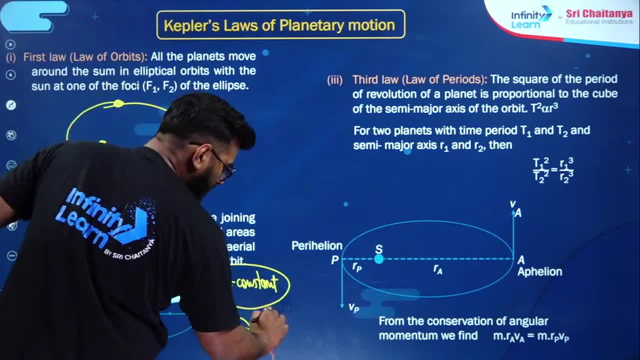 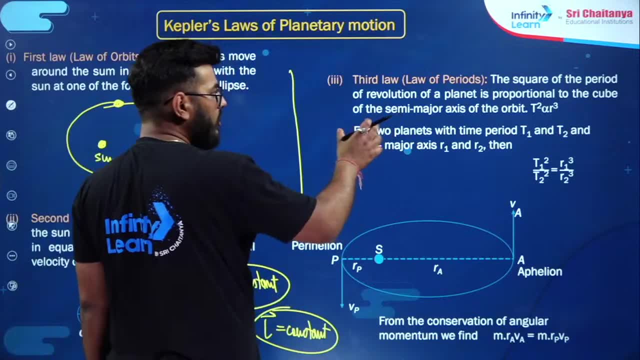 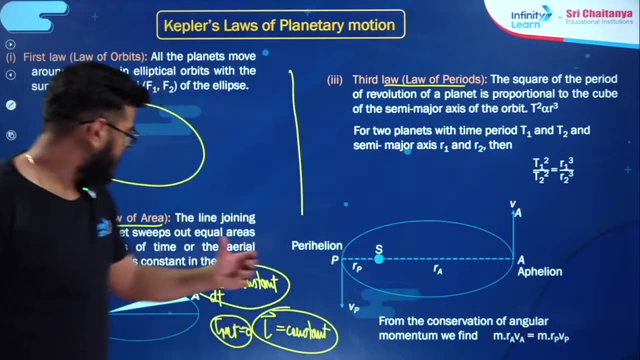 But angular momentum of the planets is always constant. The angular momentum of the planets is always constant. If I talk about the third law, The third law says a simple thing: The square of the time period. The square of the time period is the semi-major axis. 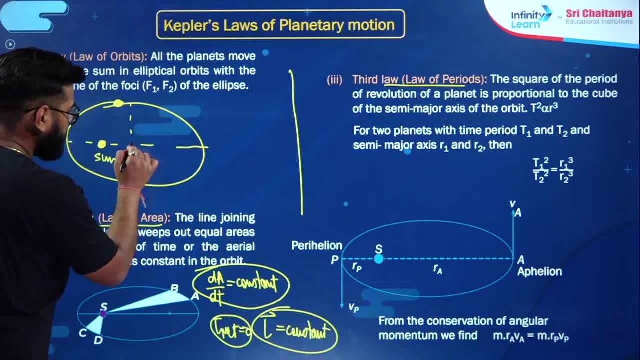 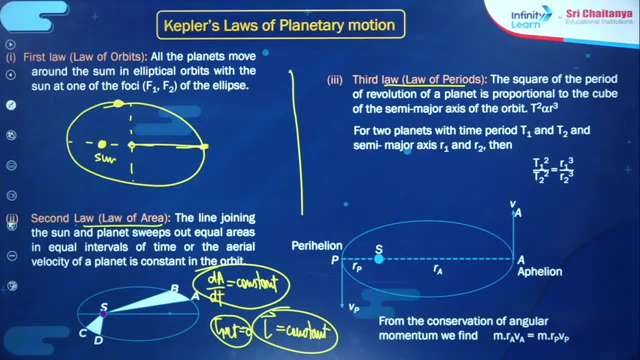 That is this distance. This Semi-major axis is called this distance. This distance is directly related to its cube. Okay, The square of the time period of two planets is directly related to their cube. Okay, Now let's ask some related questions. 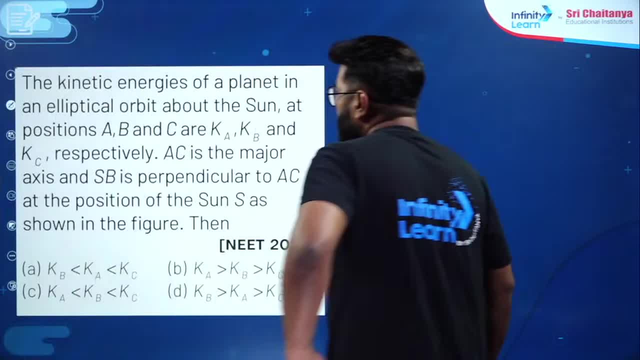 Quickly. the first question comes in front of you on the screen. The kinetic energies of a planet in an elliptical orbit around the sun are at the position a, b, c, r, k, a, k, b and k c respectively. 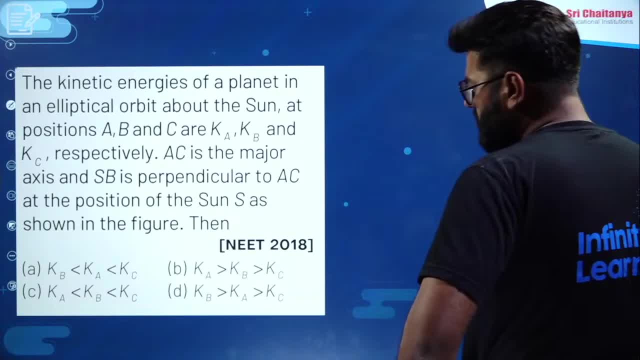 a- c is the major axis. s, b is perpendicular to a- c At the position of sun as shown in the figure. It is not a figure. I will make it a figure. Look at the figure. It is something like this: 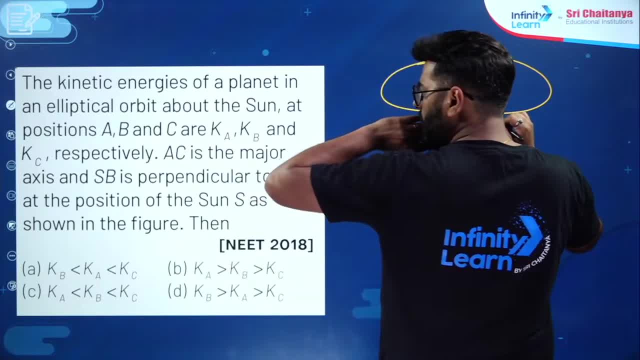 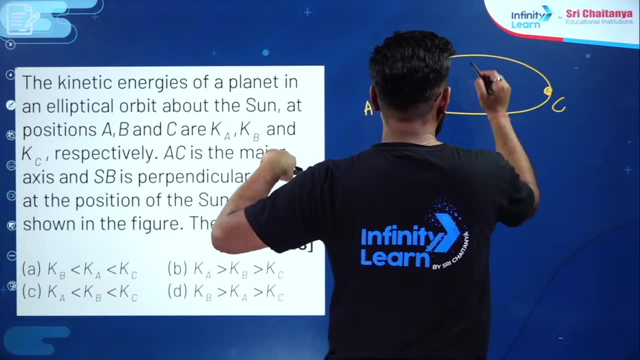 This is the sun And there are three points given here. Okay, a, c is the major axis. Okay, One is here, a, c point is here And b point is here. Okay, Now we are being asked where the most kinetic energy is. 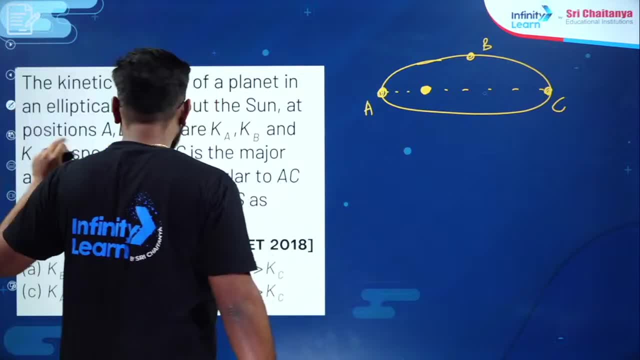 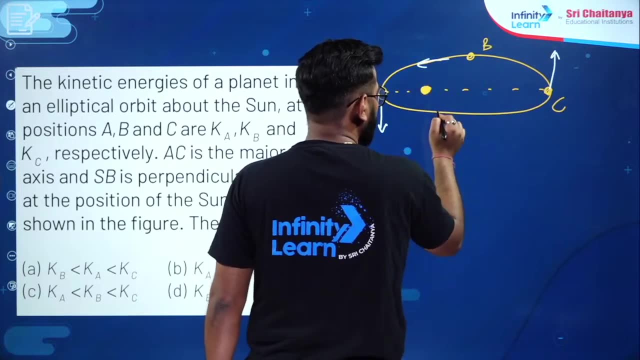 So look, It is a simple fact. The angular momentum is always conserved, Absolutely right. So the angular momentum that will be at the a point will be at the c point if the planet is moving like this. Right, Okay? 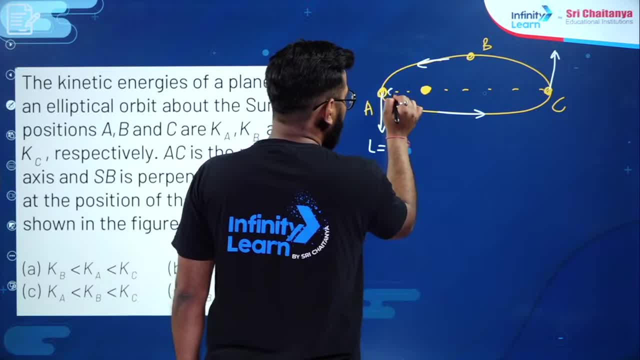 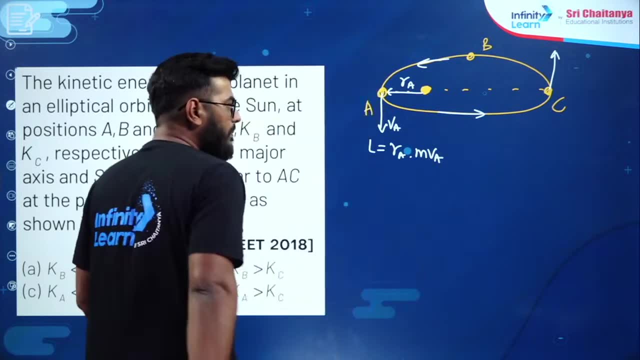 So what will be the angular momentum here, Sir? this distance is r a into m into v a. Suppose here the velocity is v a So r a into m into v a. r into p perpendicular, or r perpendicular into p. 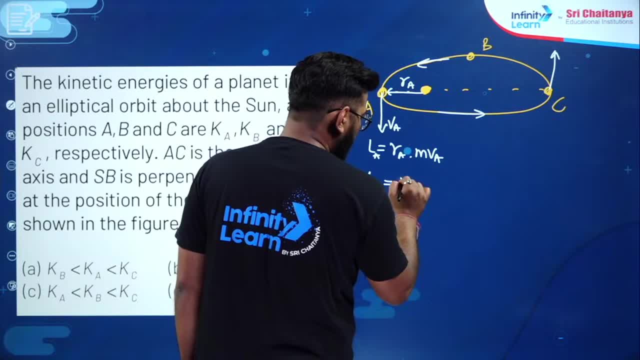 This is angular momentum at a. What will be the angular momentum at c? r c into m v c, Where r c will be this distance, Okay, And v c will be this So r c into m v c. 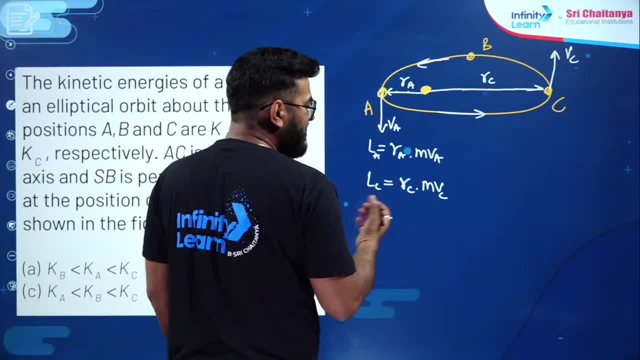 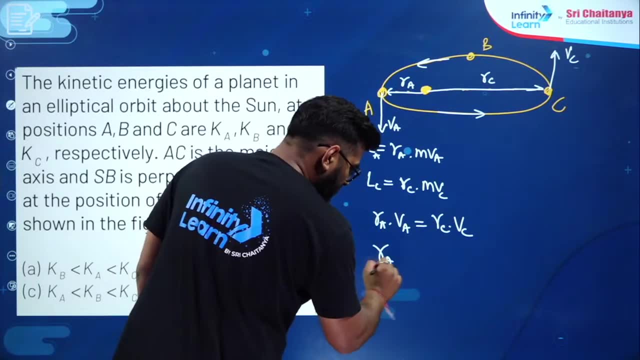 And these two are equal. These two are equal. What do you understand from this, Sir? r a into v a is equal to r c into v c. Now, r a is equal to r c, Sir. what will be the value? 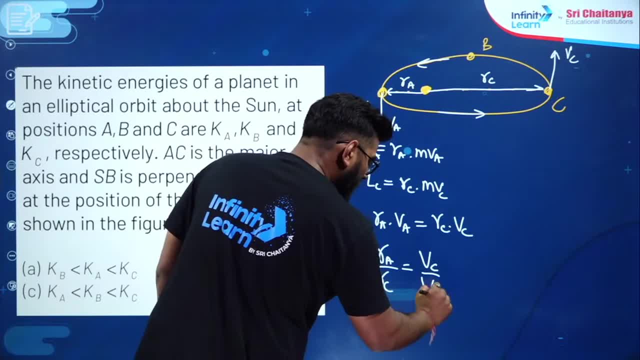 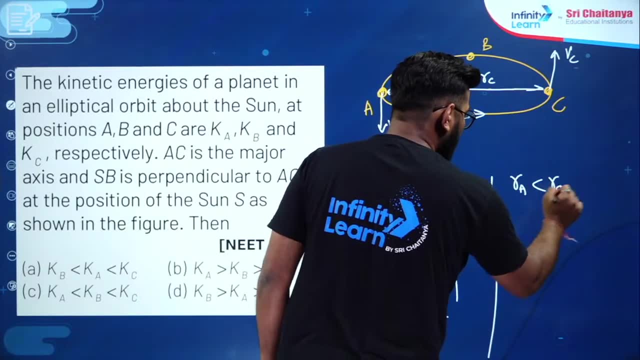 Sir, this will be equal to v. c is equal to v a And after seeing this, we understand that the value of r a is much lower than r a c. r a is lesser than r c, So the value of r a upon r c will be lower. 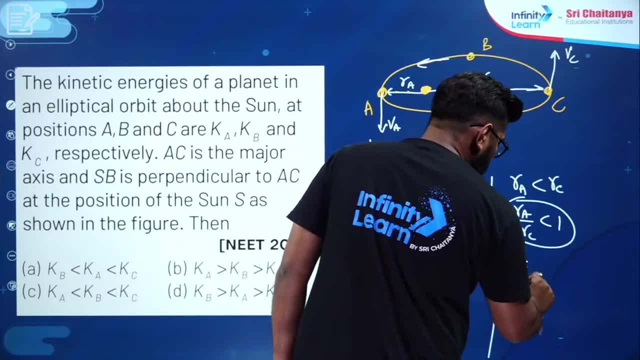 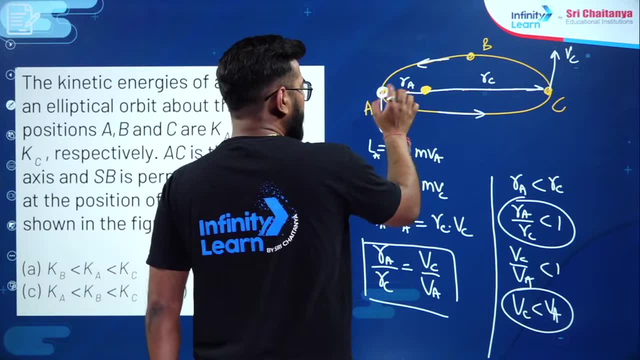 It is lower, Vc upon Va will be smaller than 1, that is, the value of Vc will be smaller than Va. Moreover, because R is less here, the velocity will have to be more, because the magnitude of this has to be equal to this. 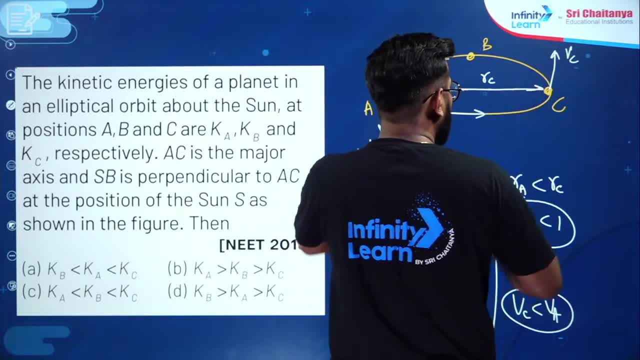 So here this is smaller, so we have to increase it. So here this is bigger, so we have to make it smaller. And let me tell you one more interesting thing which you always have to remember Here. this point is called perihelion point. 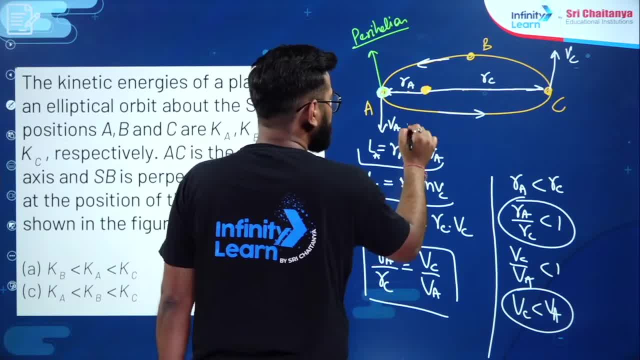 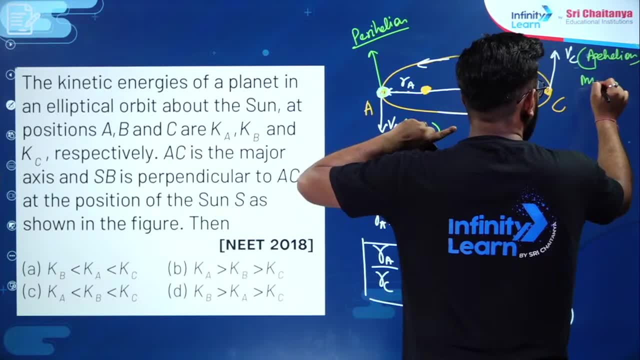 What is it called Perihelion point? At perihelion point, the velocity is maximum, And this is called epihelion point, And at epihelion point the velocity is minimum. Now, the maximum velocity is here, the minimum velocity is here. 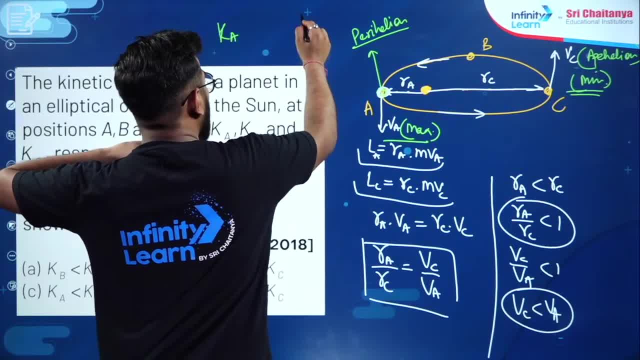 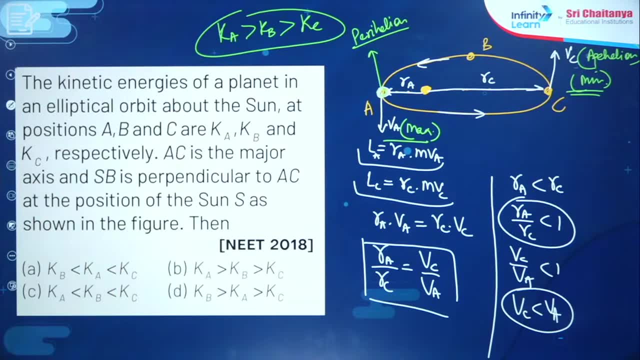 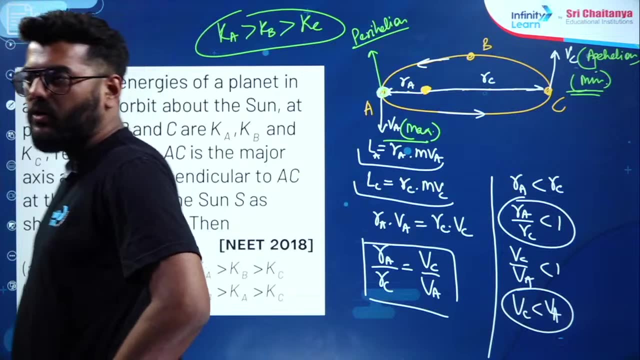 So obviously the kinetic energy will be the maximum at K and the minimum at Kc, And somewhere in between them K will also come. So option number B is the correct answer. Is it clear? Did you understand? The angular momentum is also constant in electron revolution. 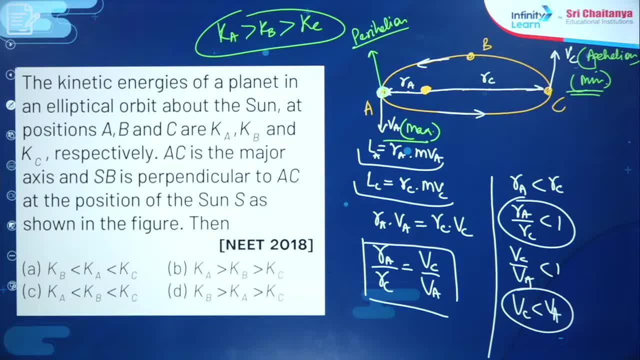 Yes, absolutely, So, obviously Exactly. And the integral multiple is of h cross. Siddharth Chandra is absolutely correct. Very nice, 1 plus e is to 1 minus e. He also told the ratio: Very good, That's very good. 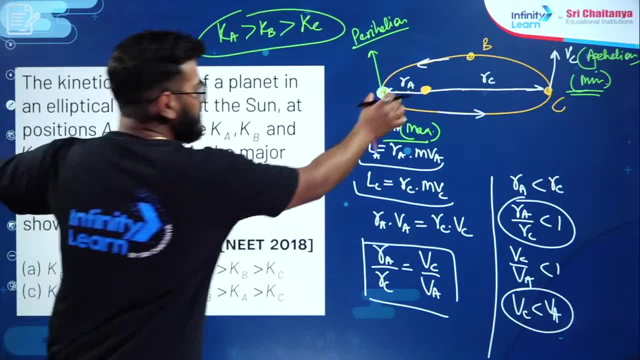 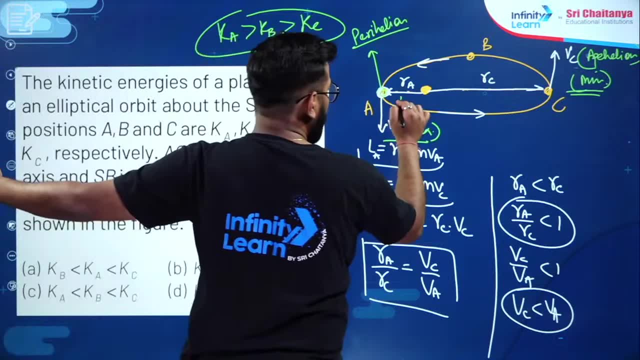 Very good, Very good. Apurv has also told the ratio, sir, That what is the ratio of these distances? And if the ratio is of distances, then the ratio of velocities will also be known. Absolutely, This distance is your, a minus ae. 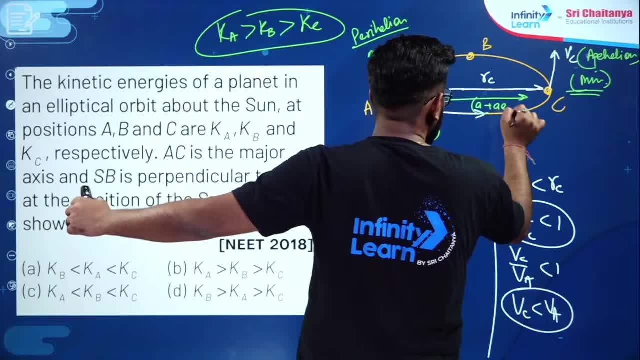 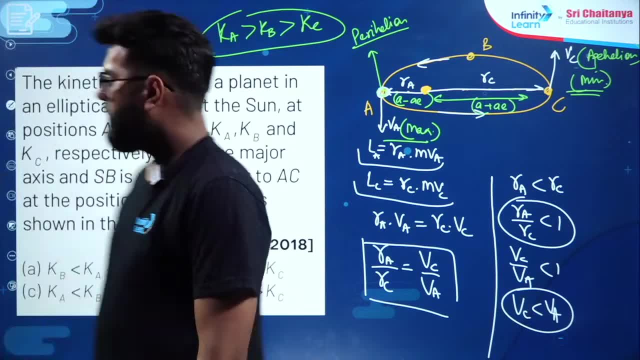 And this distance is your a plus ae. So according to that, the ratio of rc is to ra is also given. So the correct answer is option number B. I hope you all understood. Let's move on to the next question. The figure shows the elliptical orbit of planet M around the sun. 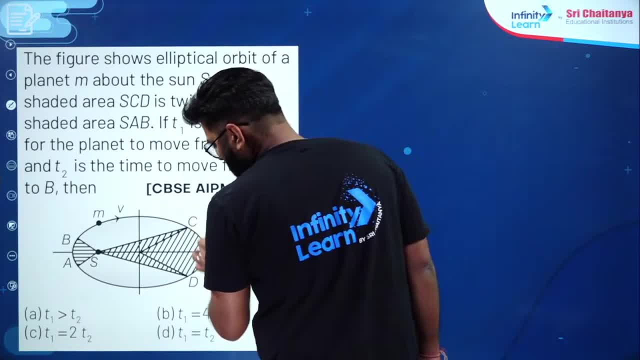 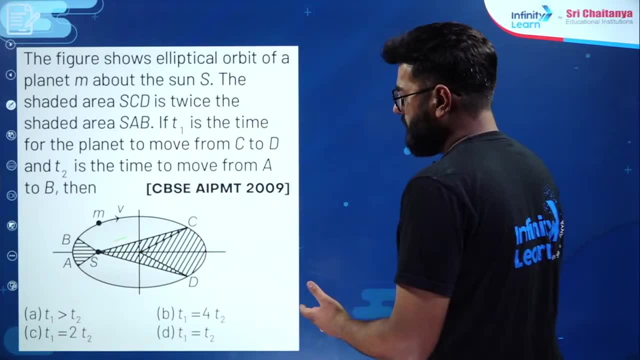 The shaded area scd is twice the shaded area sab. The area scd is 2 times the area scd. If t1 is the time for the planet to move from c to d, t1 is the time to move from c to d. 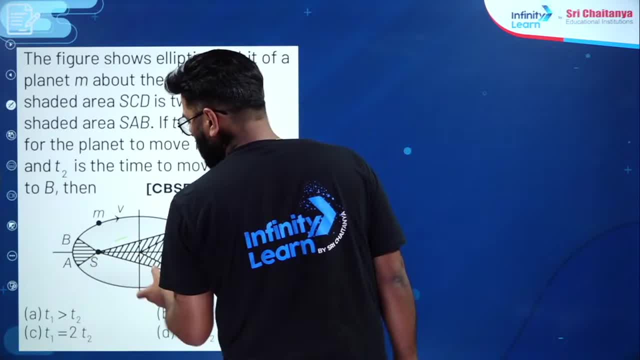 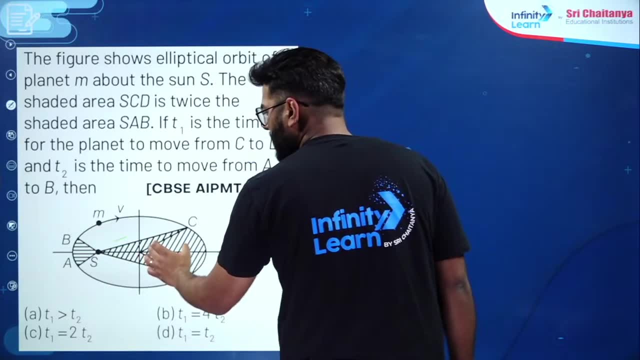 then t2 is the time to move from a to b. Obviously, sir, the area is 2 times, so the time will be double. So here the time taken in sab will be half of this. If t1 is applied here, then t2 will be t1 by 2.. 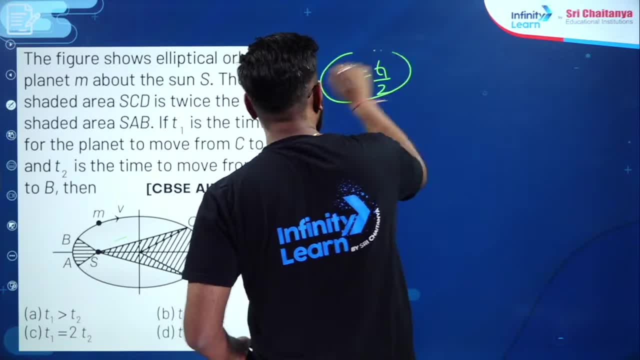 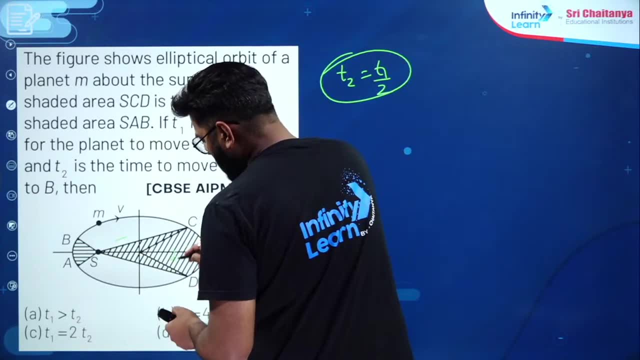 The value of t2 will be t1 by 2.. How do you know? Oh man, the aerial velocity is constant. The aerial velocity is constant. To do this double area, consider this 2x. This is 2x. 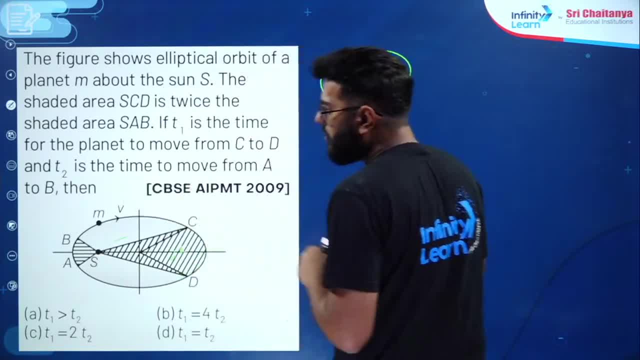 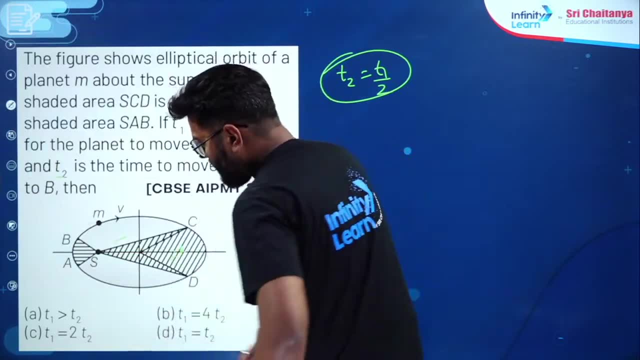 So t1 is taking time to do 2x. So t1 by 2 will take time to do x. Simple thing. So the point is simple. The value of t2 will be t1 by 2. And according to that, two options are set here. 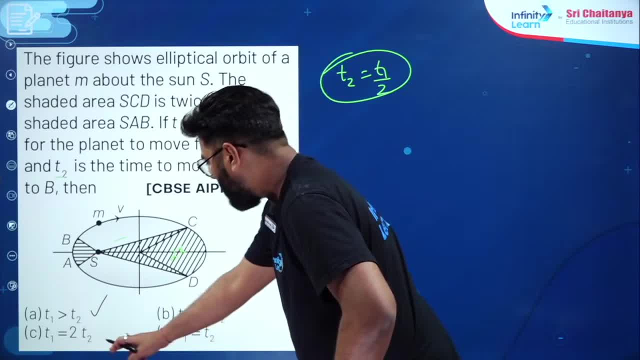 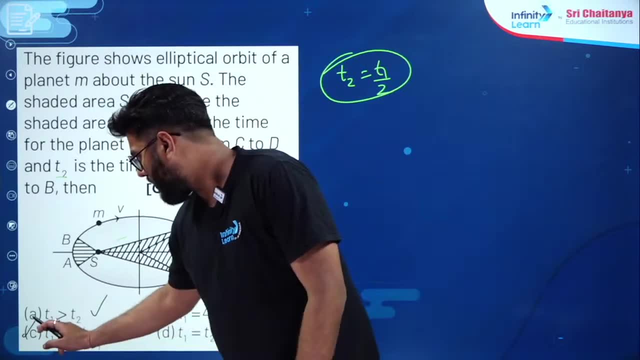 One is also set And the second one is also set. t1 equals to 2 times t2.. Option number a and c are set. Both are set. Both are set. This too and this too. Okay, So with these two questions, I just want to tell you that. 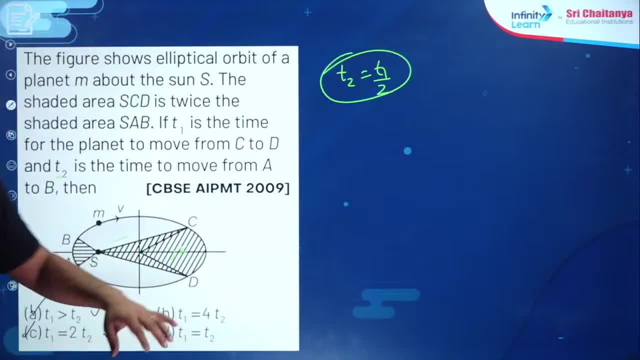 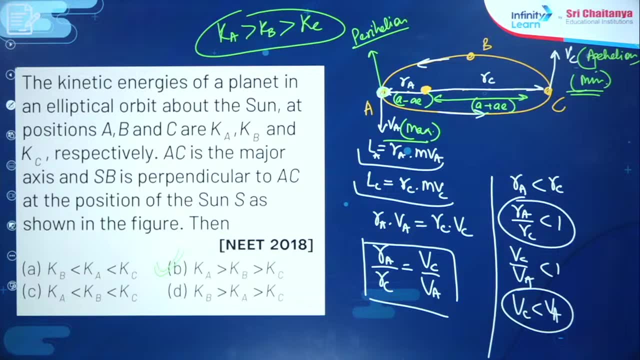 there can be a question on Kepler Law And if there will be, then mostly the chances will be related to the area And here it will be related to the conservation of angular momentum. Clear, Both are correct. Both are correct. c is also correct. 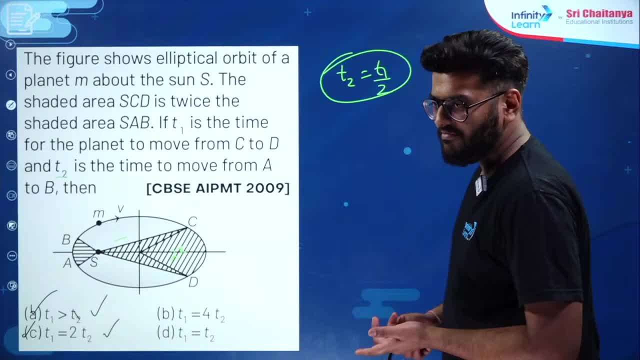 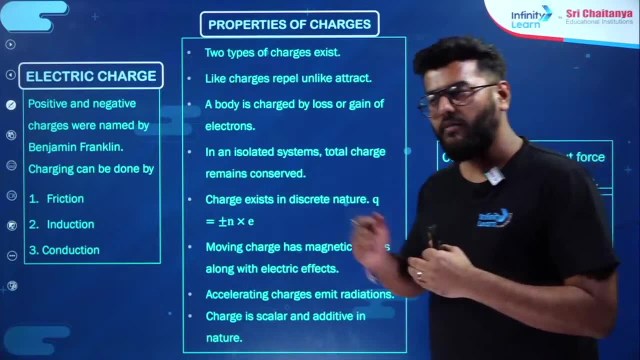 a is also correct, a is also correct, c is more than 2.. Okay, Come on, Let's move forward. and you know, Now let's switch to electric electrostats. Now let's switch from gravitation to electrostats. 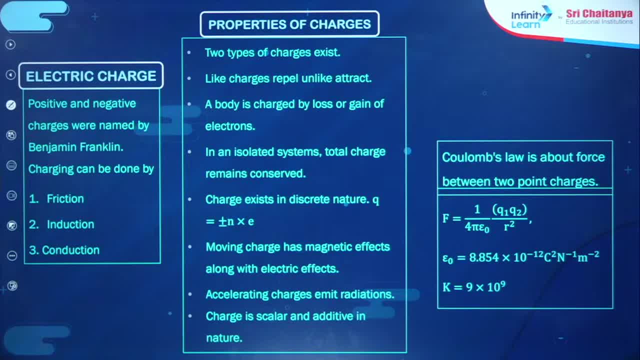 Okay, Now if we switch to electrostats, then look, first of all we need to know the property of charges And then, soon, we'll know your Coulomb law, which in a way reciprocates your universal law of gravitation. Clear, The one with the R in which the derivation is there. 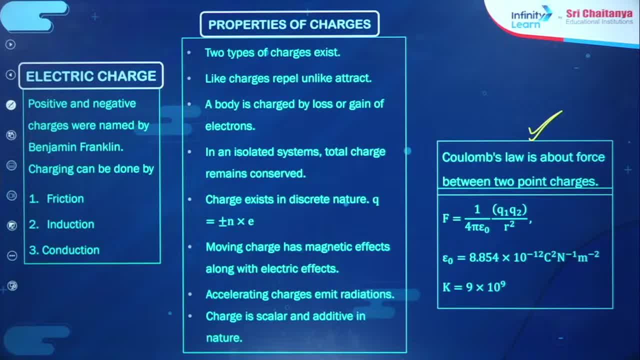 Yes, Which one are you talking about? Which R one? Which R one? do you understand? Electric charge is of two types: positive and negative. Obviously, if you talk about the masses in gravitation, then the mass is of the same type. 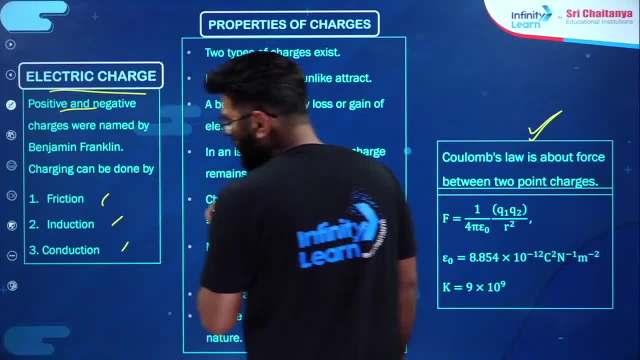 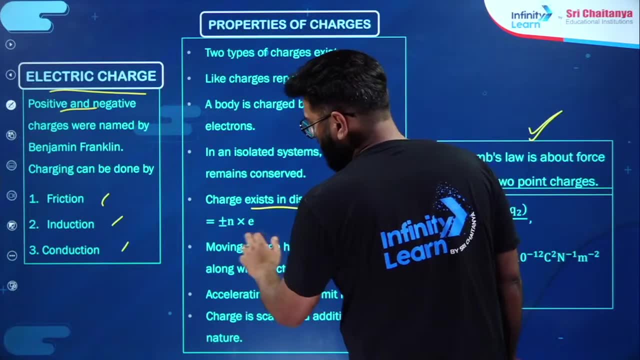 There will not exist two or four masses. Friction, induction and conduction are three methods through which you can develop charges. After that, there are some properties of charge. Charge is always quantized. Charge is always plus or minus. any Moving charge makes magnetic field. 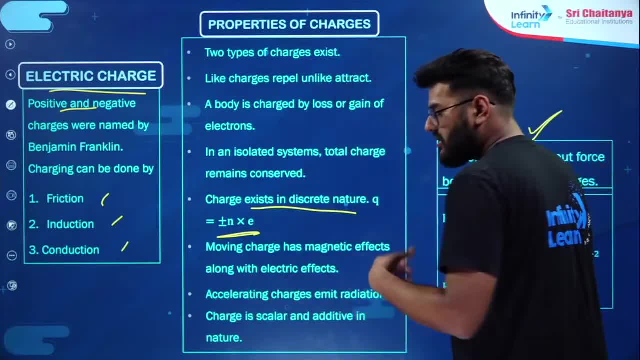 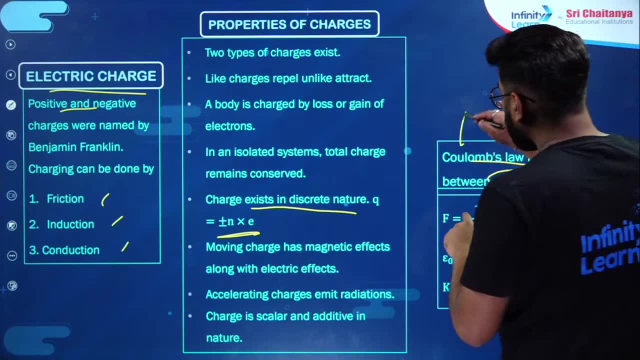 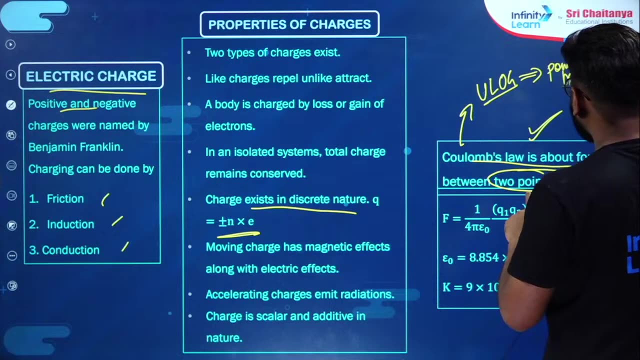 Static charge makes electric field, Accelerating charge makes EM waves. The Coulomb law is valid for two points charges. The universal law of gravitation is also valid for point masses. It is simple to say that the force applied can be both repulsive and attractive. 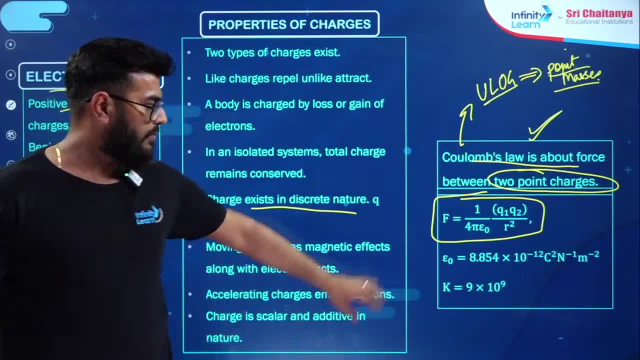 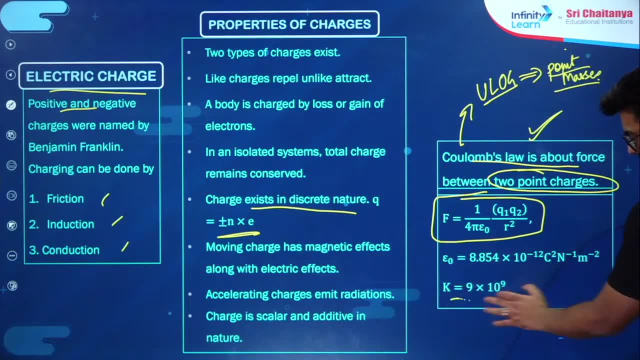 Same forces, same charges will apply. repulsive Opposite charges will apply. attractive, Clear, And this is it. Your calculation will come. The value of K is 9 to 10 to the power of 9.. And the value of epsilon naught is 8.85 to the power of 10 to the power of 12.. 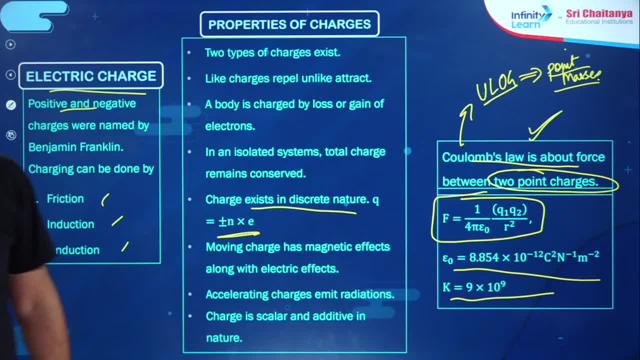 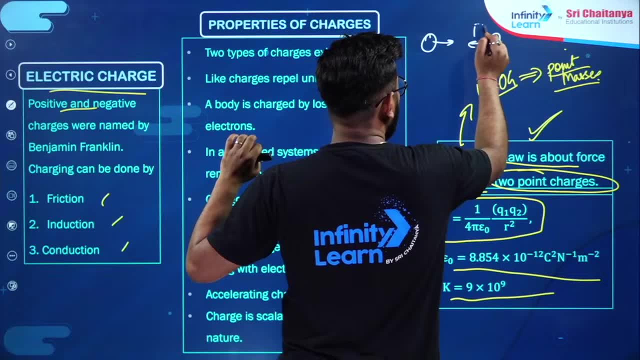 Sir, tell me the direction in the Coulombic force. What are you asking? Direction in the Coulombic force. There are two positive charges. It will apply here and here. It is attractive, It is opposite. It is opposite. 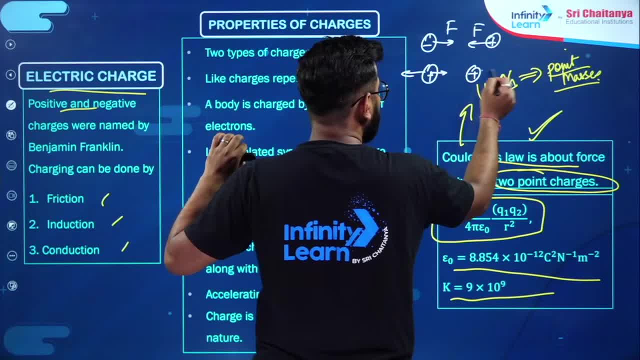 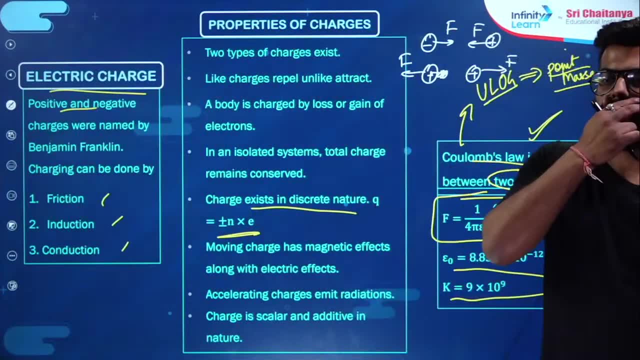 Sorry, It is opposite. And if they are the same, then repulsive force will apply Here F, here F. This is what he is asking. If you have taken the center of the solid sphere, but if you had taken it from the center. 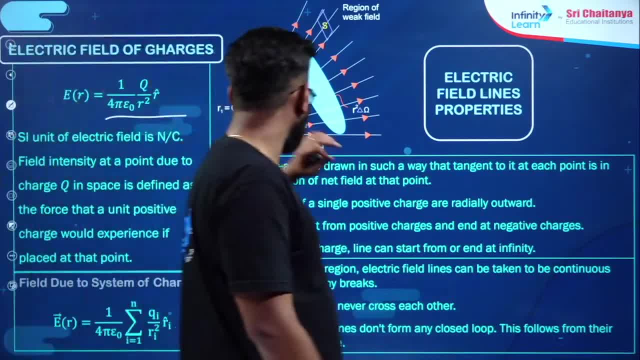 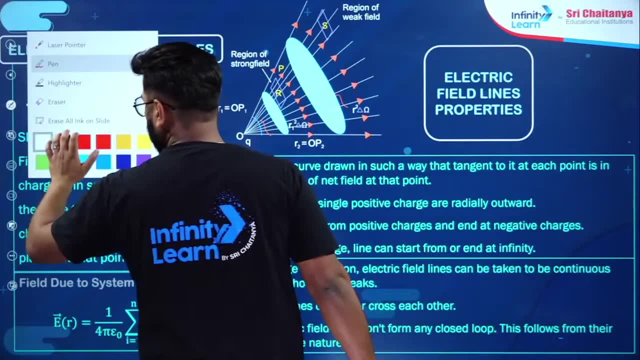 Okay, you are telling from the aspect of the center of the charge. Come on, I will tell you about it too. Okay Now, if I talk about the electric line of forces? Okay, So, electric line of forces Here, basically, I am giving you the final formulation quickly. 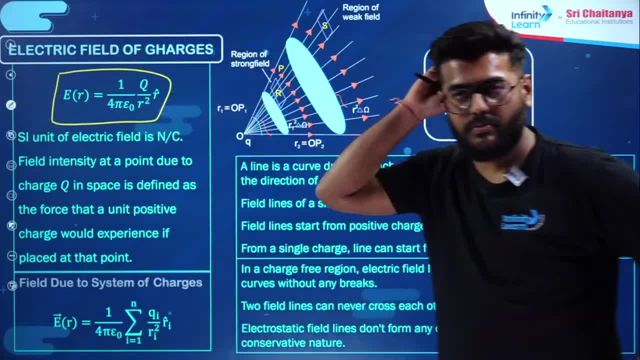 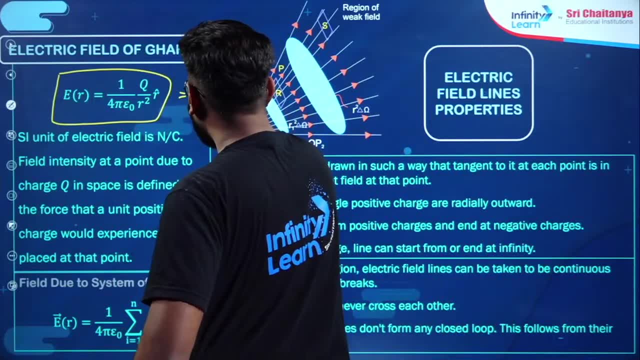 It is my bigger agenda to ask questions, Right? So electric line of forces means the electric field lines that will be in the nearby region due to a charge. You simply know that Whichever force is divided by Whichever charge is, by its method. 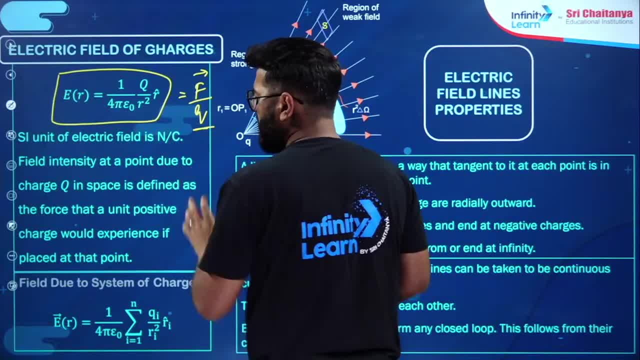 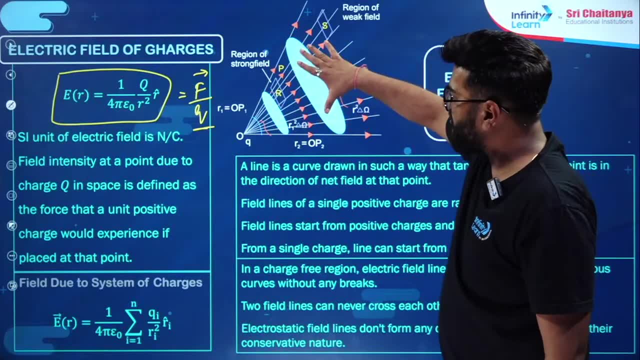 Okay, So force upon charge will give you electric field line in the nearby region due to any charge And it happens by going away from it. Okay, As you go away, you will see that the intensity of electric field lines is also decreasing. 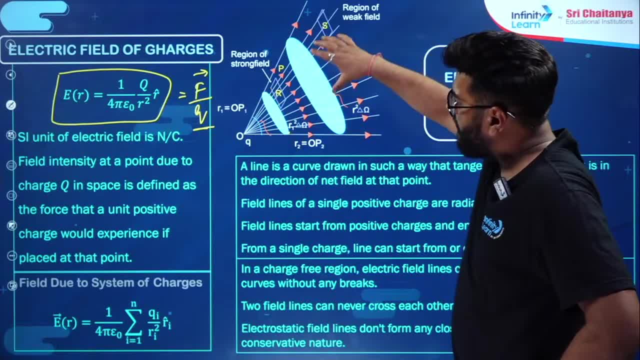 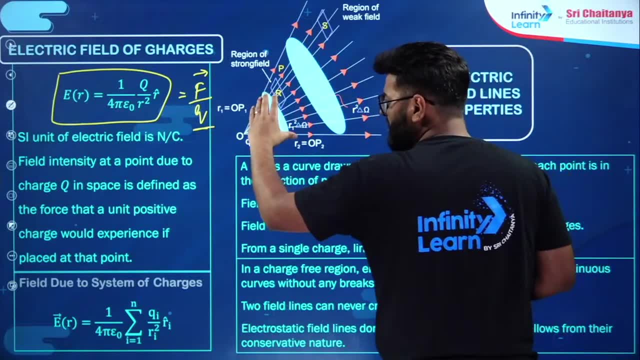 From that area you can see that the number of field lines and the area has to be increased. So how do we know the intensity of the number of field lines, The number of electric field lines passing through a cross-sectional area, As it decreases because the area is increasing? 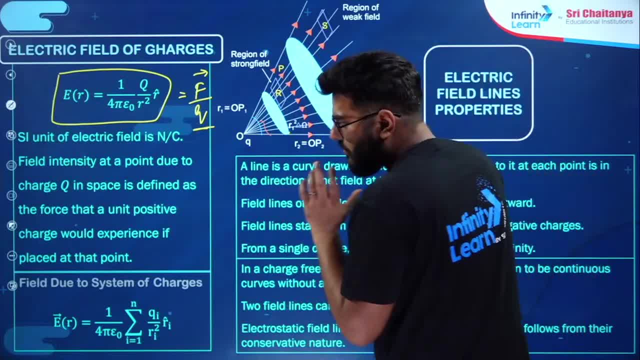 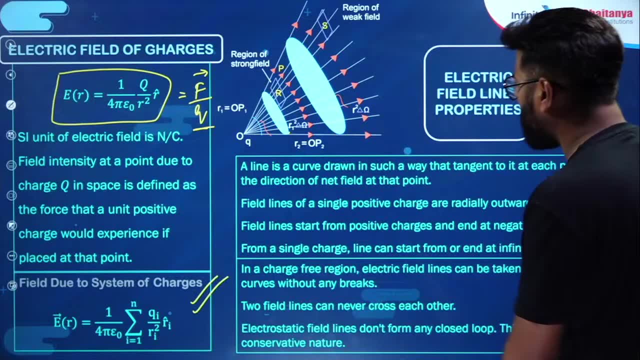 So we can also say that the magnitude of electric field lines is decreasing gradually. Okay, If there are a lot of electric charges, So due to everyone, the electric field line will be the net vector of everyone. Okay, Now there are some properties. 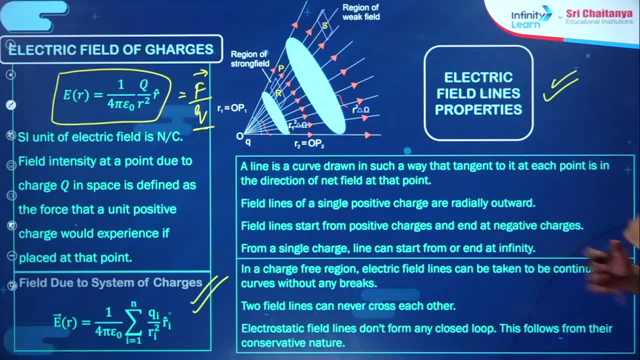 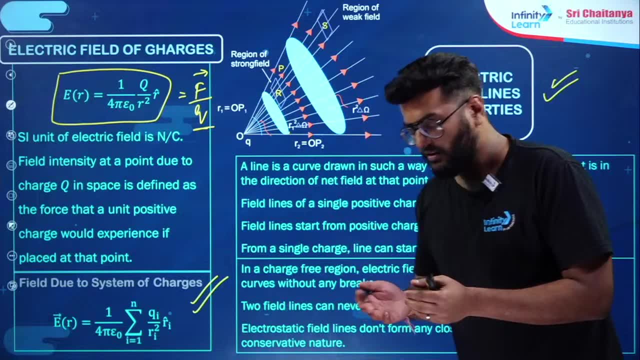 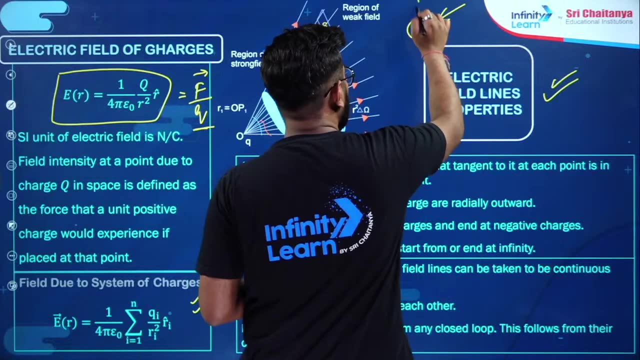 You can see, here You have given properties for everyone. These same properties will exist in your gravitational field lines, Except for one property, Because the masses cannot be positive or negative. Due to the masses, the gravitational field lines will remain, They just keep coming towards them. 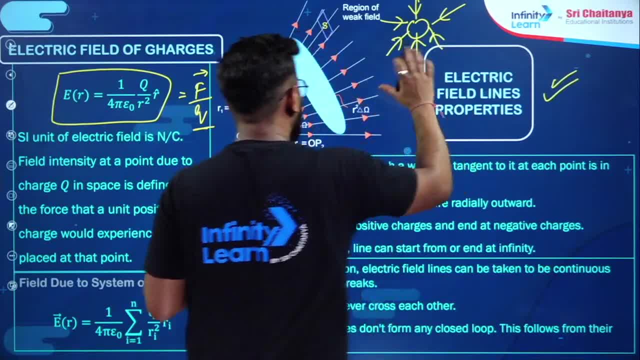 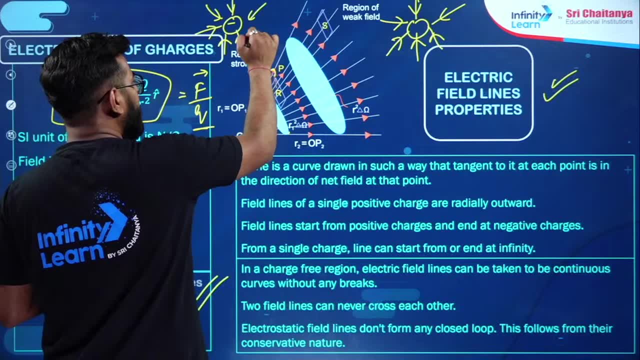 Here the point is: Sir, look, Because of the positive It will go away. Because of the positive it is going away And because of the negative it will come towards it. Okay, In this, the electric field lines are in this way: 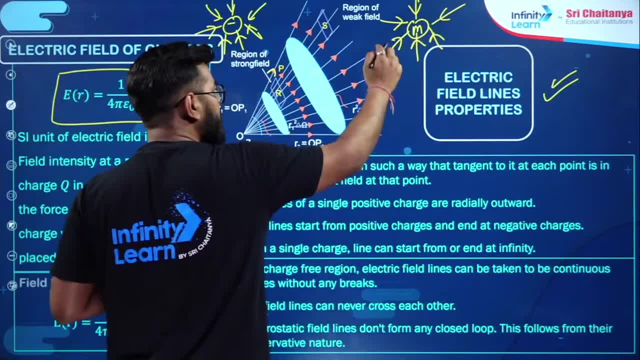 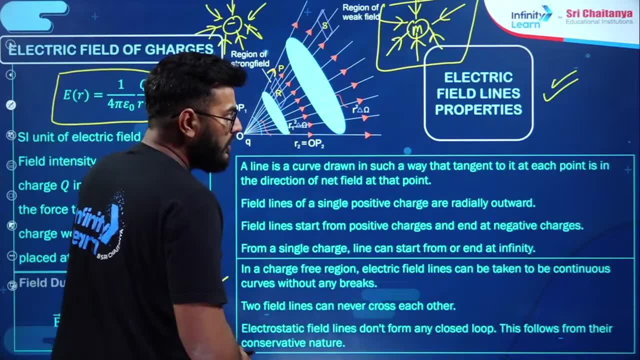 But if I talk about the mass In the mass, the existence of gravitational field lines is in the same way, Because the positive and negative mass does not exist, Plus m, and because of them the gravitational field line will come inside it. Rest properties are as it is. 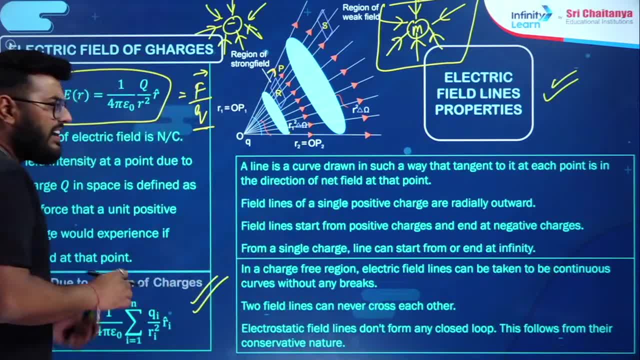 Properties are as it is: Field lines are always straight lines. The direction that will be there will be known by its tangent. Okay, So let's move on. Then let's move ahead. Polar molecules Now. as I said, 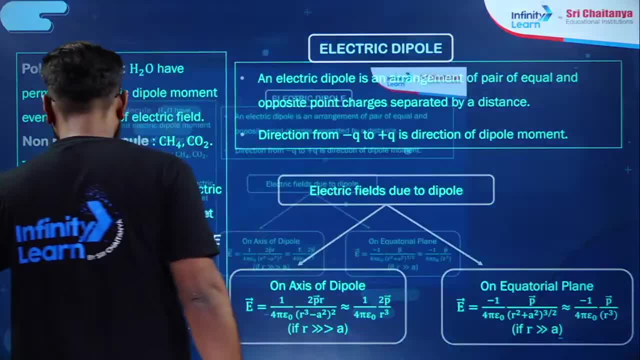 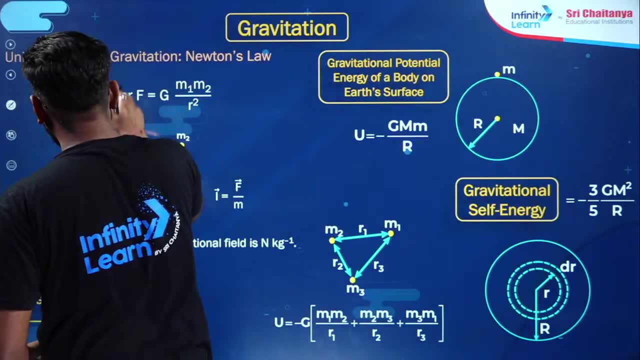 Electric dipole. Okay, Before that, I will tell you about the gravitation. Before that, I will tell you about the gravitation too. So look at the gravitation. The force that will remain in gravitation is M1 M2 upon Gm1, M2 upon R2.. 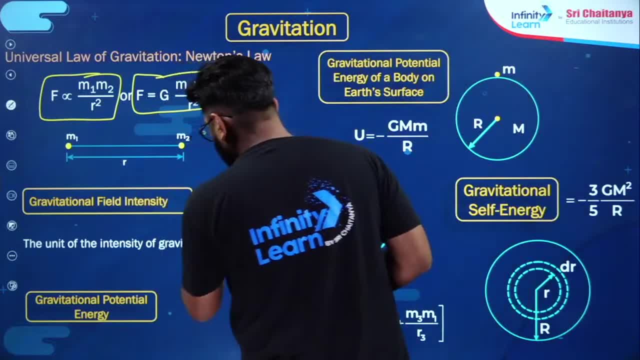 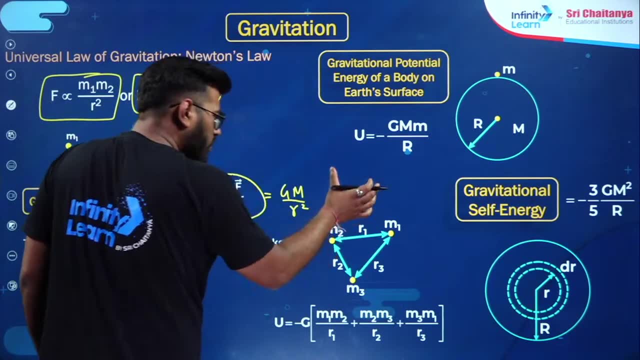 Same validity. Similarly, After that, the gravitational field intensity will remain F upon M. That is, due to the mass, the gravitational field intensity becomes Gm upon R2.. Simple, It will keep coming towards it. Wherever the gravitational field lines will be, it will keep coming towards it. 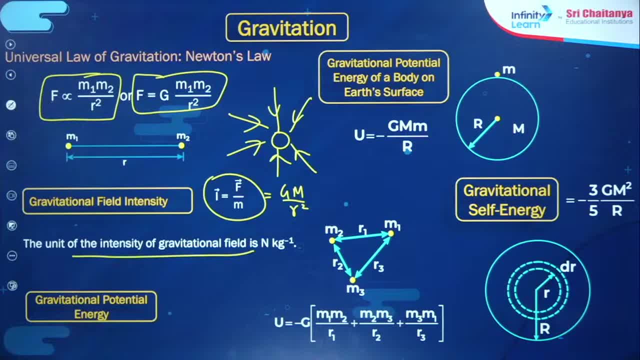 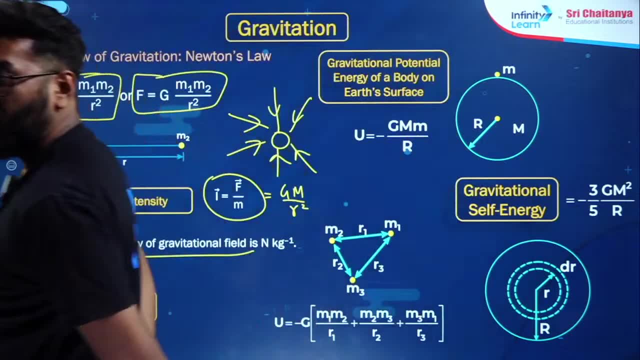 Okay, So it is the same phenomenon. Unit of intensity of gravitational field line remains Kg upon Newton. And this concept of potential, energy and potential. we will read it now, As we will talk about electrostatic potential and capacitance. Okay. 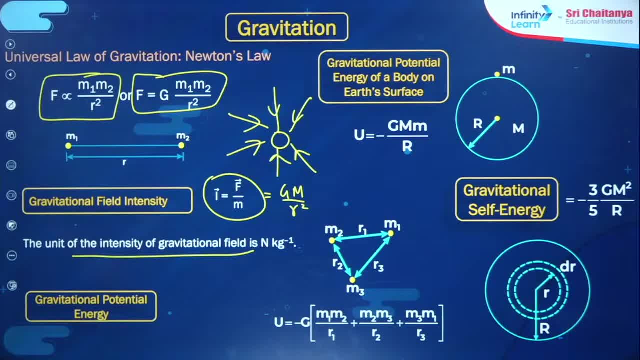 So, while defining potential, no change in kinetic energy for external forces and opposite in electric and gravitational energy. No, No, It is not like that. This is not it. While defining potential, no change in kinetic energy for external forces and opposite in. 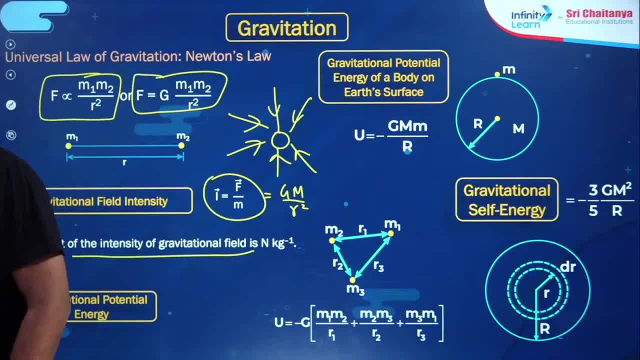 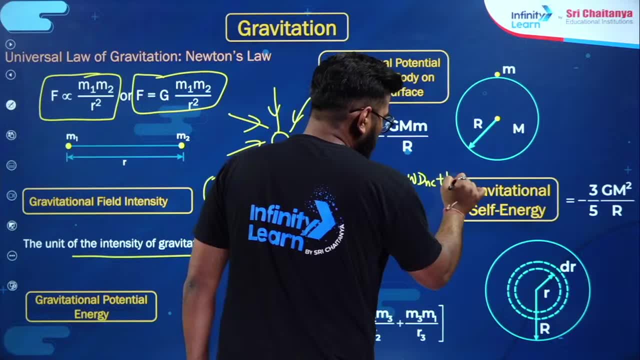 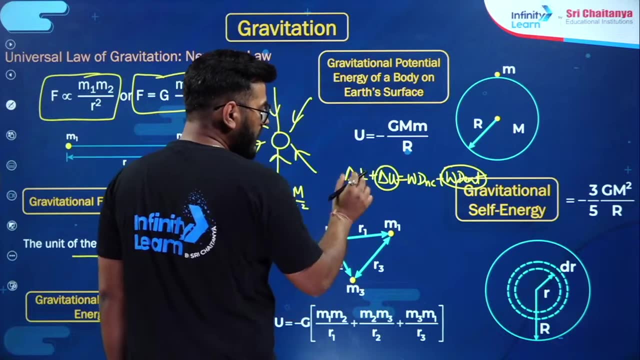 electric and gravitational energy. No change in kinetic energy for external forces and opposite in electric and gravitational energy. It is because delta K plus delta U is equal to work done by non-conservative plus external forces. This is the calculation. Okay, Now what do you want? 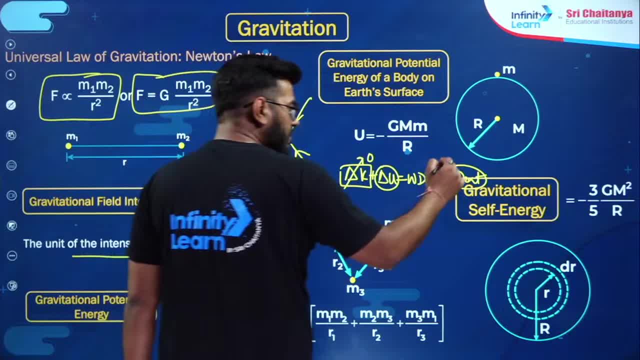 That whatever external forces you are applying, you should convert it completely to delta U. That's why you take it very slowly, so that delta K becomes nearly zero. This way, we will come to know that whatever work we are doing, it is going completely. 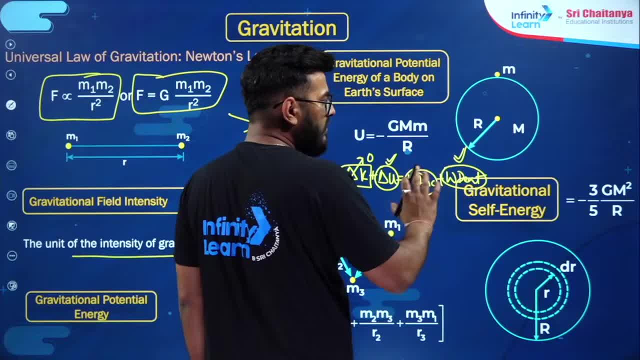 to delta U And we also ensure that there is no non-conservative, no friction force. This is the reason why we take it very slowly, Because there is no change in kinetic energy. So if there is no change in kinetic energy, then delta K and delta U are equal. 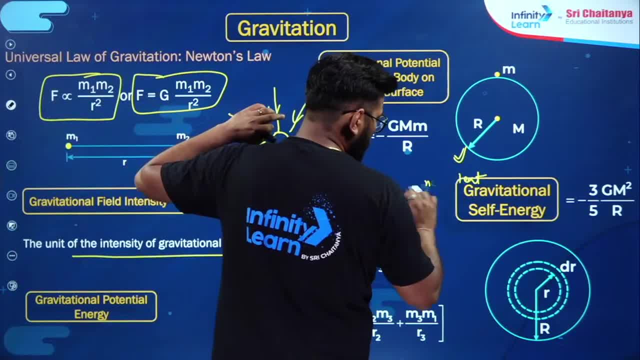 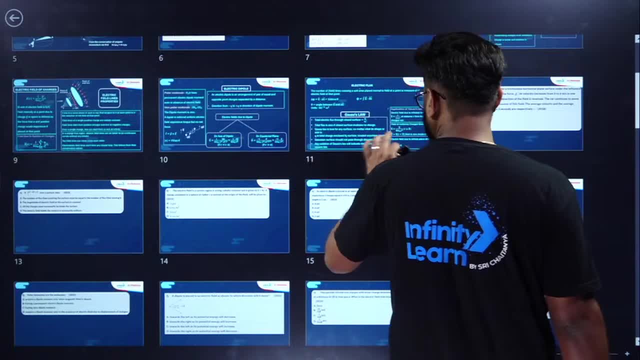 This is the reason why we take it slowly. This is the reason why we take it slowly. Work energy theorem is valid. to make it exist Clear. Now let's see the question related to Incher Quickly, As you remember the first question. 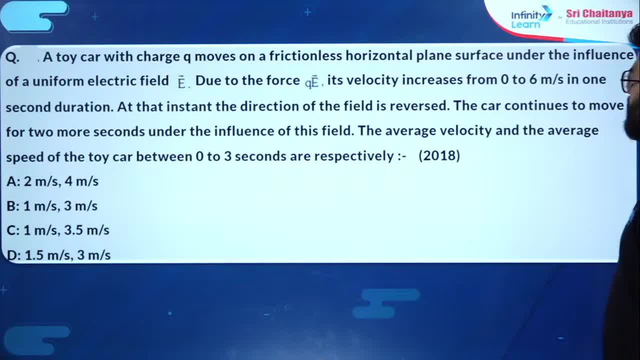 It was asked in JEE 2018.. A toy car with a charge q moves on a frictionless horizontal plane surface under the influence of uniform electric field. E Okay, Due to the force qe, its velocity increases from 0 to 6 meter per second in one second duration. 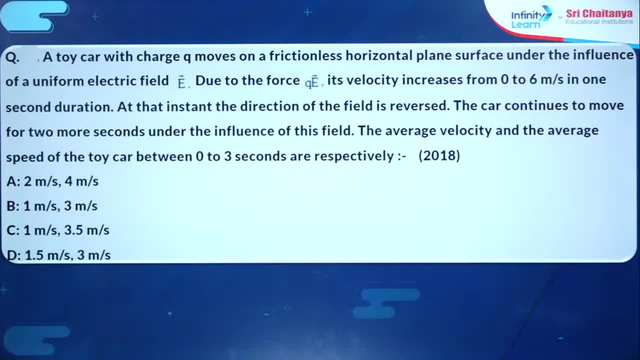 At that instant the direction of field is reversed. The car continues to move for 2 more seconds under the influence of this field. The average velocity and average speed of the toy car is between 0 to 3 seconds. This is a very good question. 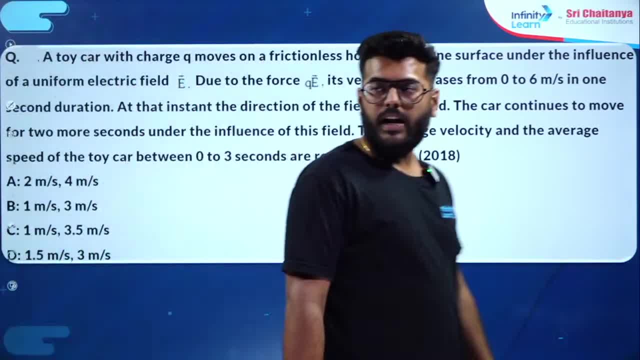 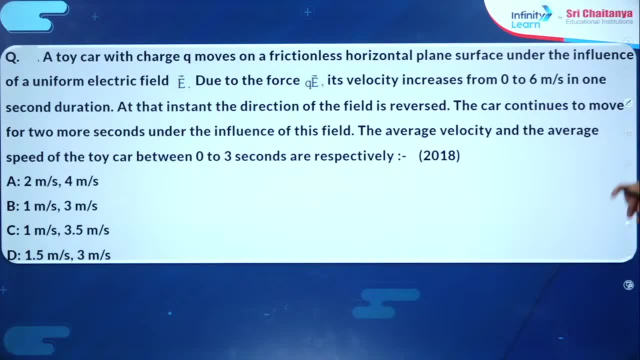 Let's quickly try this. Let's quickly try this. I am giving you one minute. Quickly try this and tell us the answer. Come on, everyone, Try this and tell us the answer. Toy car. This is a toy car with a charge q. 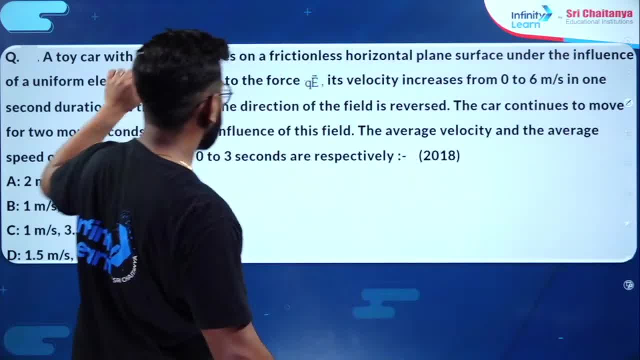 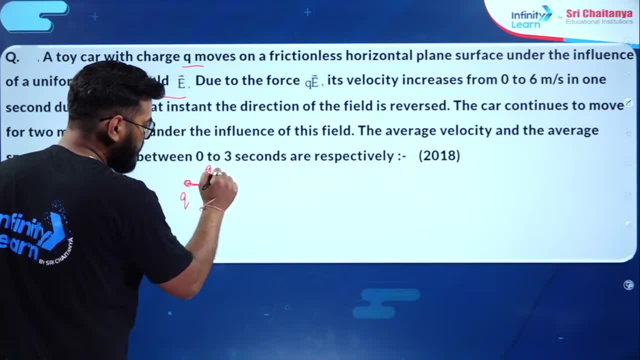 It is moving on a frictionless horizontal surface. Let's try it together: Influence of electric field. E Look, there is q. There must be a force applied on it. How much qe, Due to this qe force, there will be an acceleration qe by m? 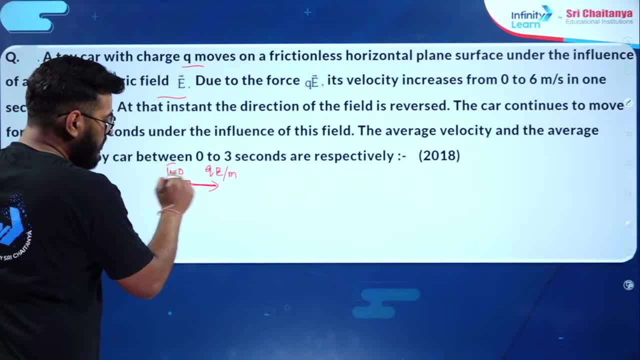 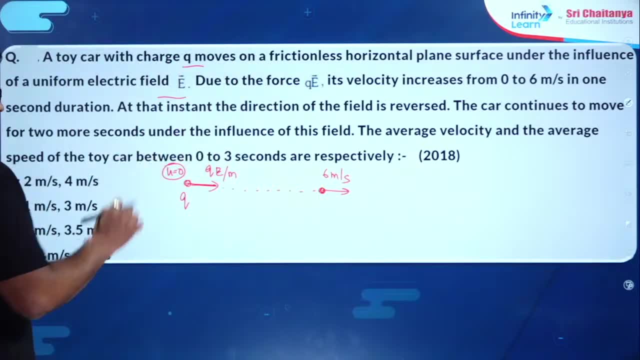 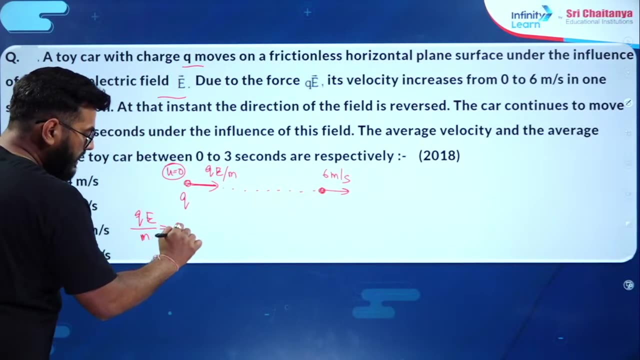 Due to this, its velocity will change. From where u is equal to 0.. The velocity will change. How far will it go? 6 meter per second. Okay, In one second. In one second. So we understood the value of acceleration. 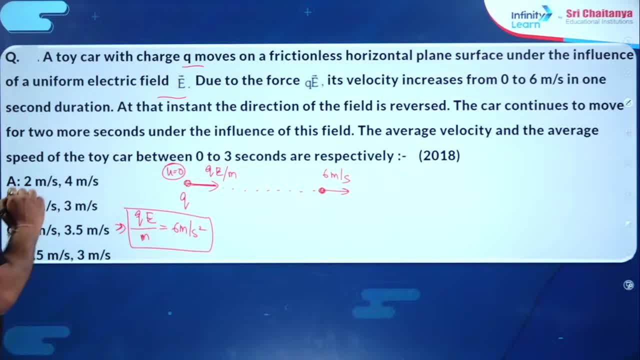 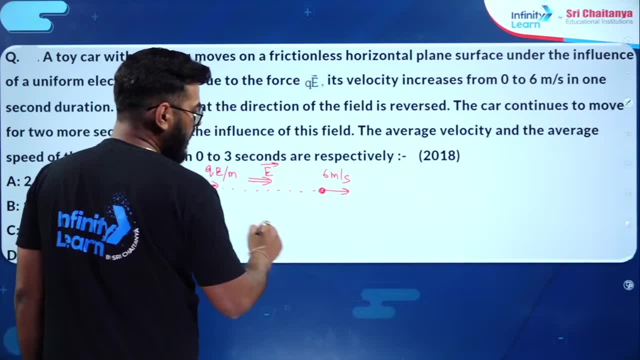 The acceleration qe by m will be 6 meter per second square. Okay, After that. at that instant, the direction of the field is reversed. Earlier, the electric field was here. After that, the electric field was here. Okay, Okay. 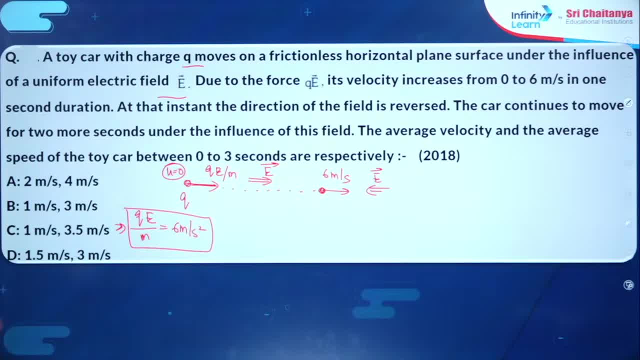 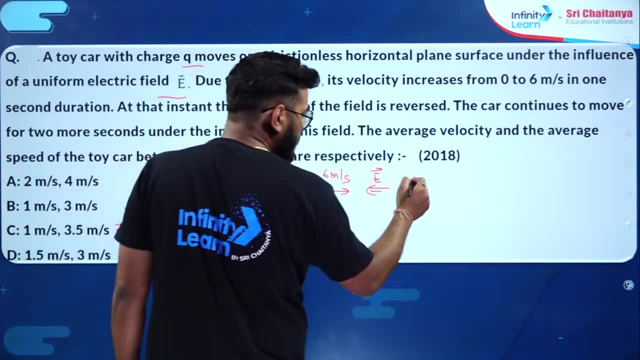 Now the car continues to move for 2 more seconds under influence of this field. The average velocity and average speed is Now in this field. what will happen? It is going backwards. Now, where will the force be applied? How much will the acceleration be? qe by m. 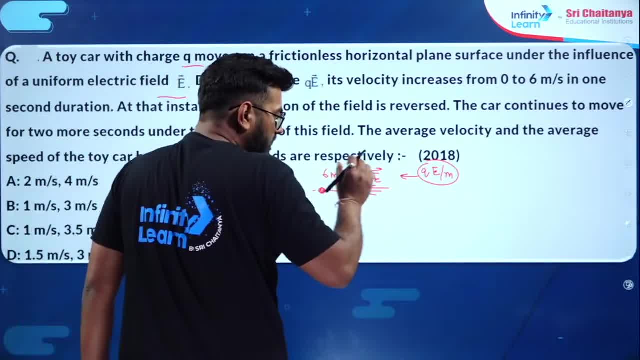 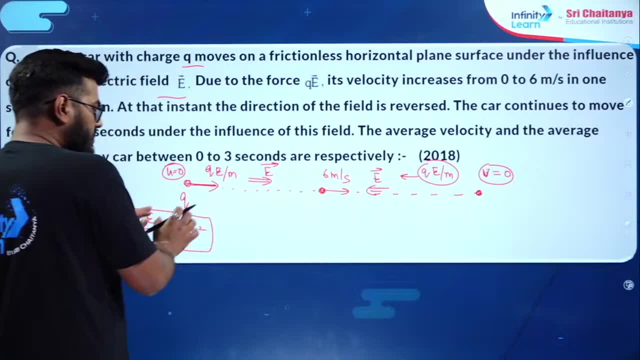 And how much is the acceleration of qe by m? 6 meter per second square. In the next 1 second it will be 0 again. The final velocity will be 0.. In each second the change is 6 meter per second. 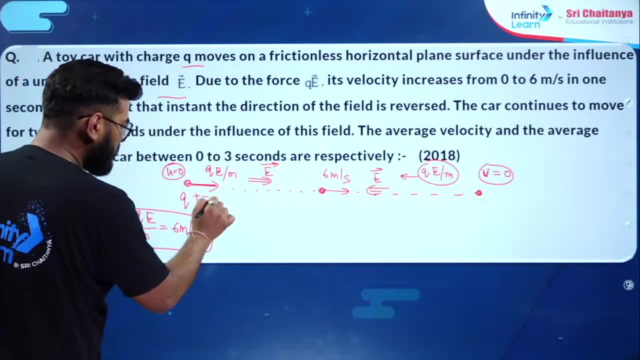 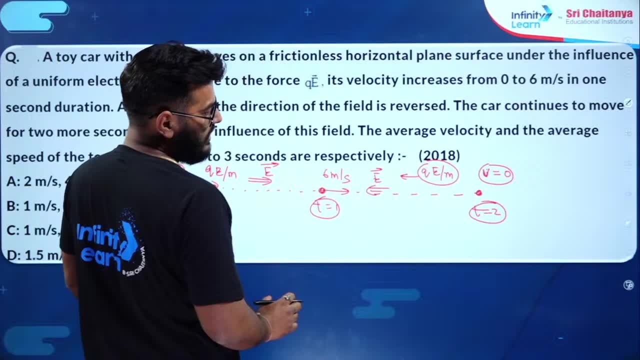 In each second. the change is 6 meter per second. So here t is equal to 0.. t is equal to 1. And t is equal to 2.. Okay, Here the final velocity is 0.. Now what will happen after this? It will be reversed. 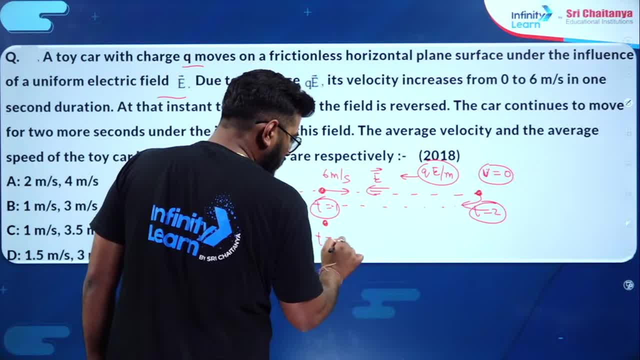 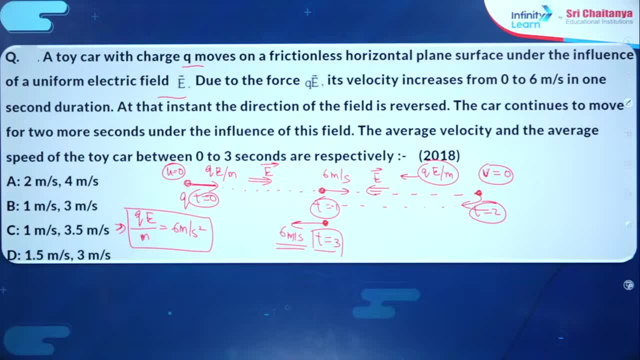 Because the acceleration is applied here. So where will it come back? It will come back here. This will be t equal to 3. And the final velocity will be 6 meter per second. Clear cut. Now we have to tell the average velocity and the average speed. 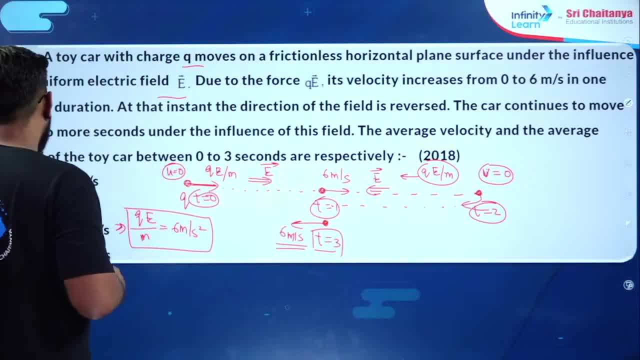 So for the average velocity you should know this distance And for the average speed you should know the total distance. In that way your average velocity and the average distance will be known. I have got the answer. Option no B and C. 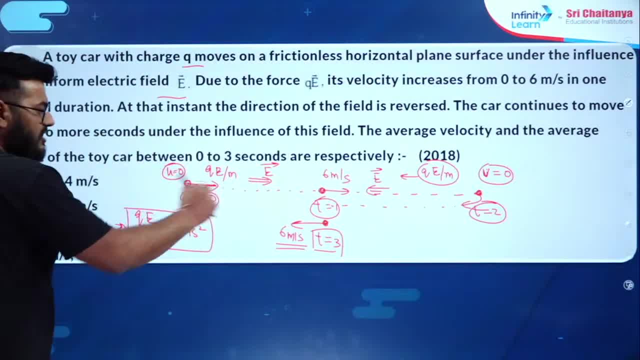 Now let's see Now what will be the average velocity, Sir. we have to know the distance. Sir s is equal to ut plus half at square. Initially it was rest. We have to do half at square, So it is 6 into t square. 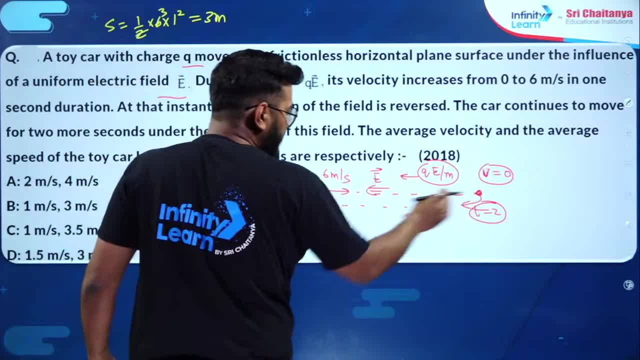 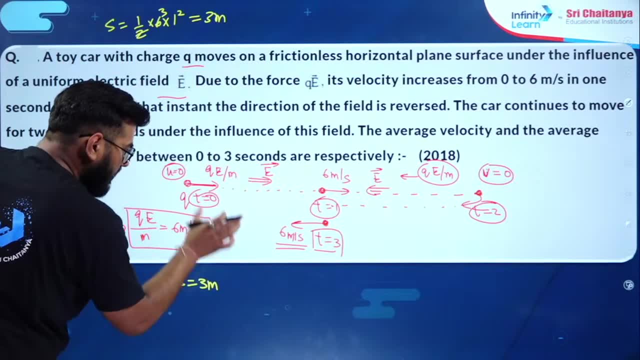 This is 3 meter. This is 3 meter. In this also s is equal to vt minus half. at square It will be 3 meter, So the displacement will be 3 meter. This distance from here to here is 3 meter. 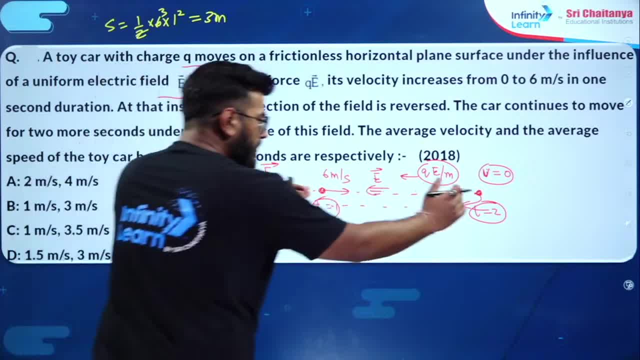 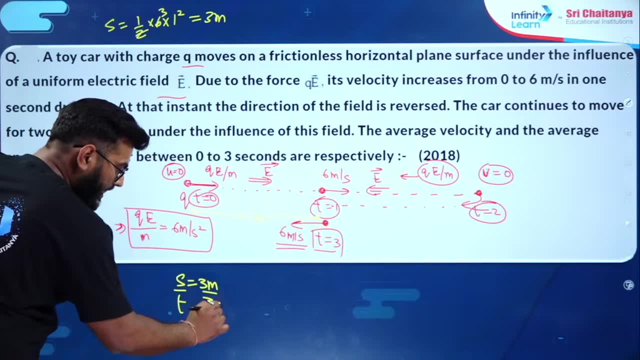 From here to here is 3 meter. This is also 3.. This is also 3.. So 3 meter is 3. by What is the total time? Total time is 3 second. What is the value? 1 meter per second. 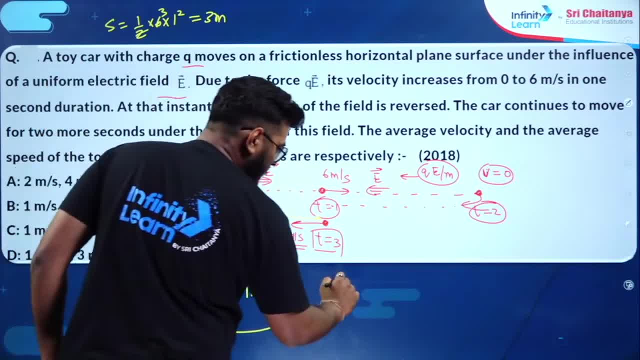 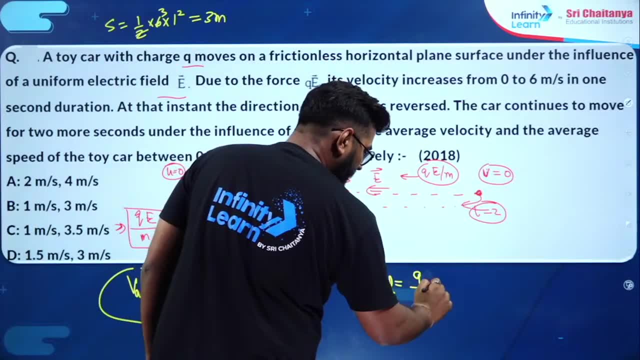 What is this Average velocity? I will talk about the average speed. I will talk about the average speed. Total distance is 3 plus 3 plus 3.. That is 9 by 3. That is 3 meter per second. 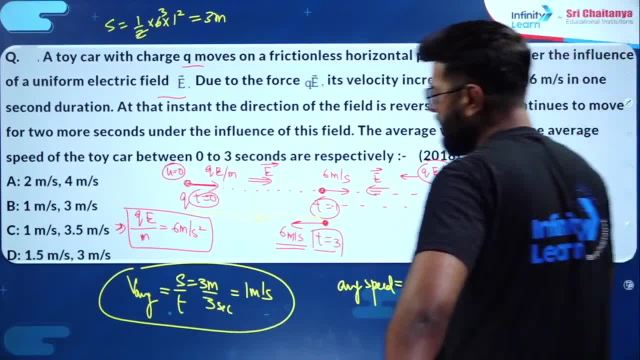 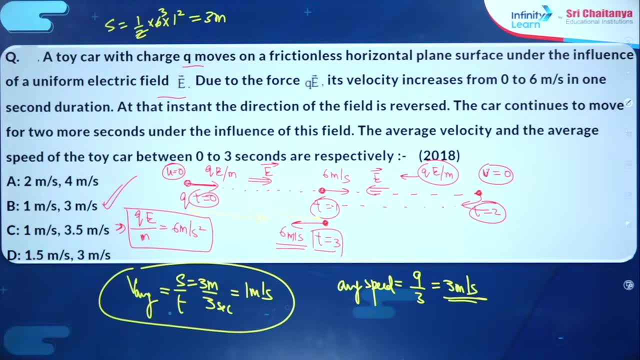 Which option is being set. Which option is being set? Option no B. Are you getting my point Clear? Siddharth Chandraji, Option no B is correct. It is not 1 and 3.5.. How did 3.5 come? 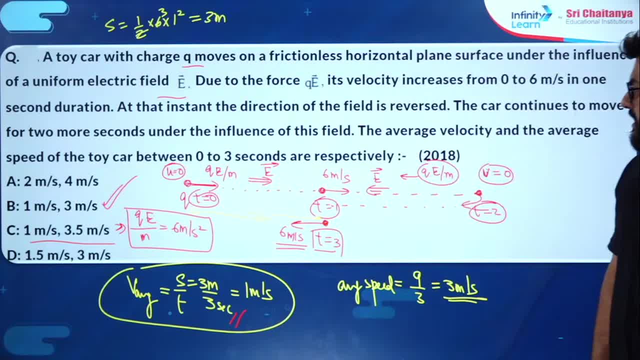 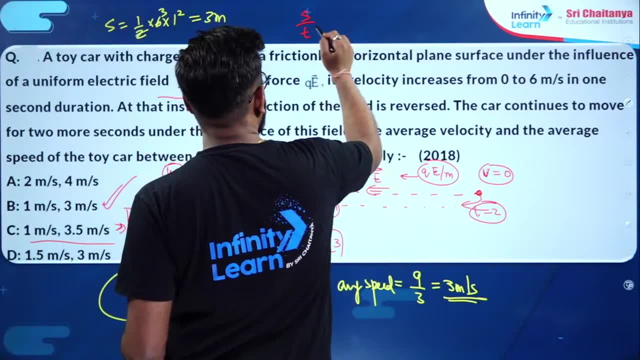 3.5 cannot come. If you divide it by 3 seconds, 3.5 cannot come. Do you know the value for that? S by 3 is equal to 3.5.. S by 3 is equal to 3.5.. 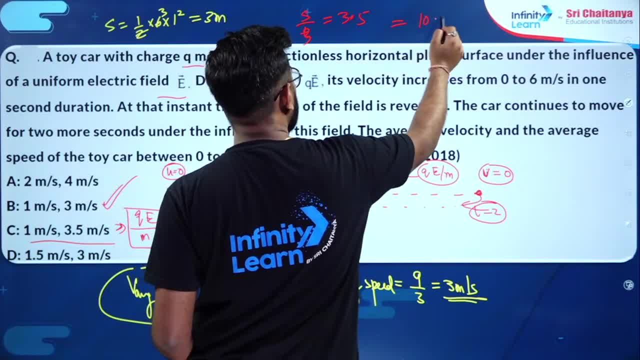 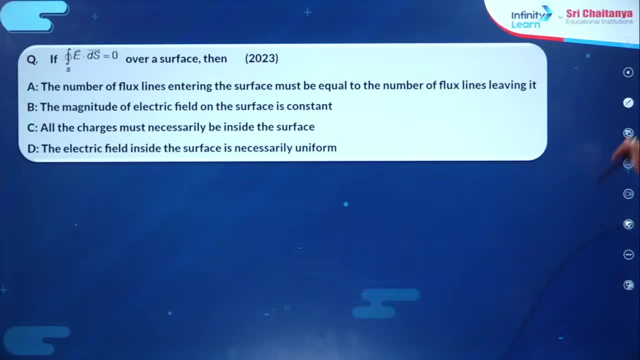 S by 3 is equal to 3.5.. Your displacement is 9.. 10.5.. Your distance is 10.5.. Only then 3.5 can come. I hope everyone understood. Electric field line in a certain region is radially acting outward. 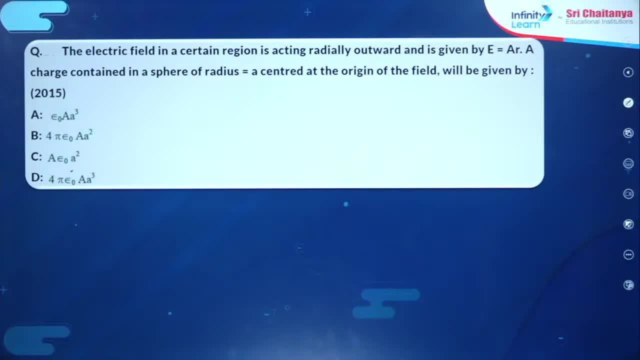 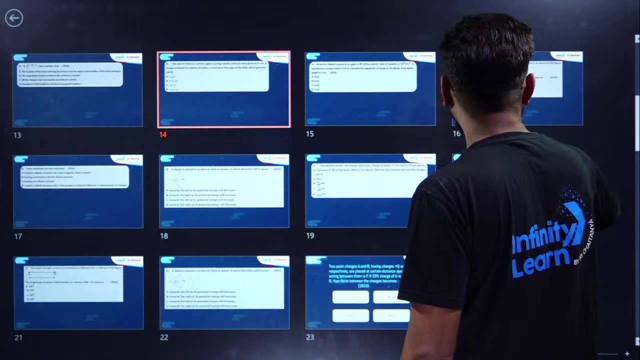 Electric field line in a certain region is radially acting outward. Electric field line in a certain region is radially acting outward. This is related to Gauss law. This is related to Gauss law. This is related to Gauss law. This is a very famous question. 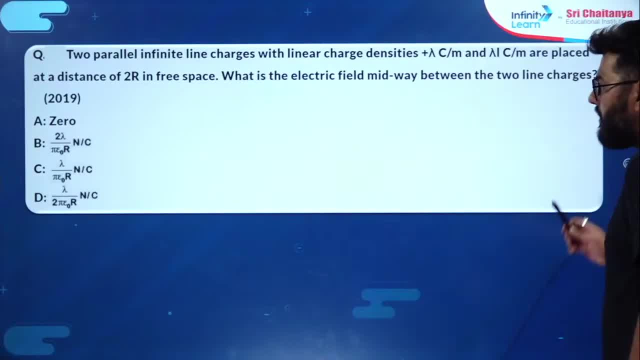 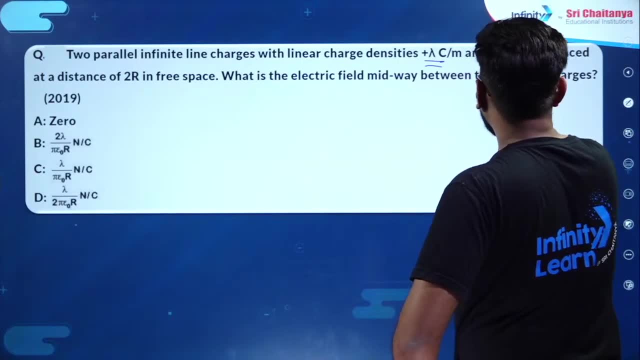 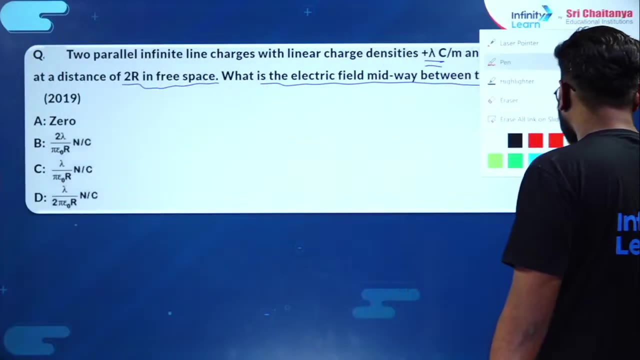 This is a very famous question. This is a very famous question. 2 parallel infinite line charges with linear charge density plus lambda and minus lambda are placed at a distance 2R in free space. What is the electric field midway between the 2 line charges? 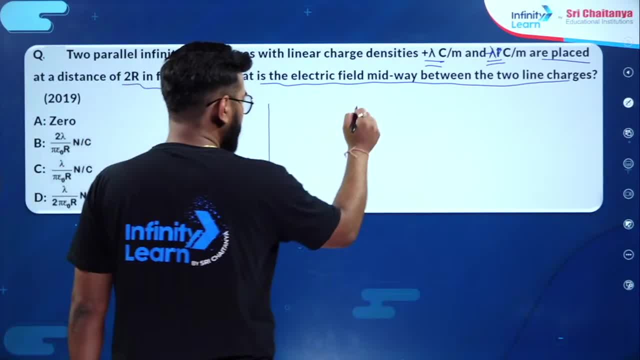 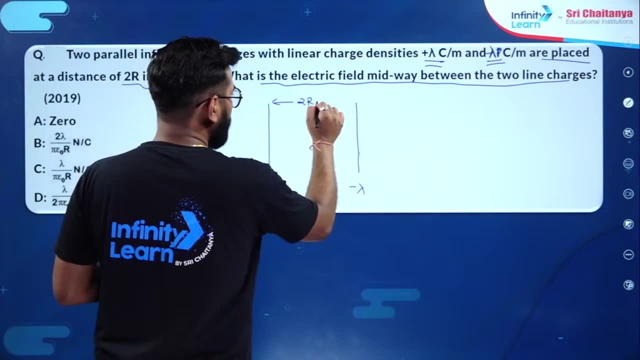 one here is plus lambda, one here is minus lambda. in between these are infinitely line charges. the distance between them is 2R. distance is 2R. now what is the electric field midway between the two line charges? here? electric field line will be how much? 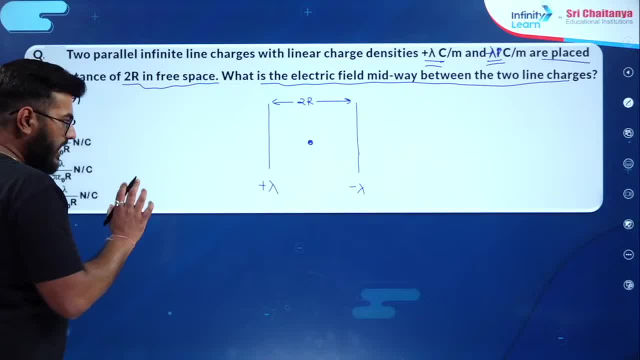 so you should know, electric field line due to a line charge and due to line charge, electric field line due to line mass. electric field line will be equal means. here I am relating and telling you. suppose there is a line charge on which positive charge is given. so in its near about region electric field line will be how much? 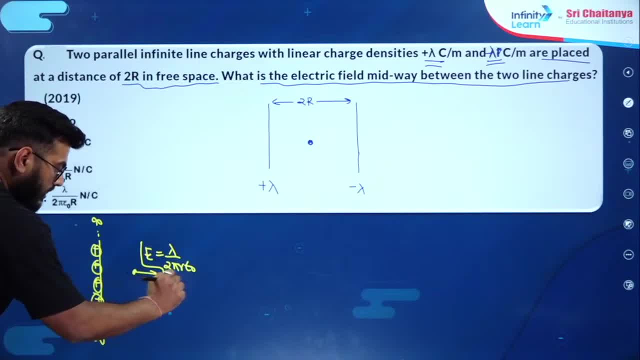 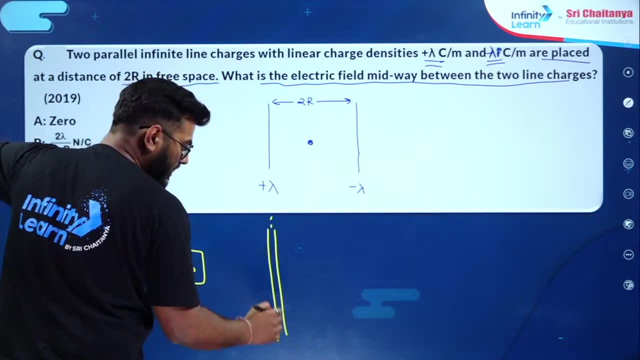 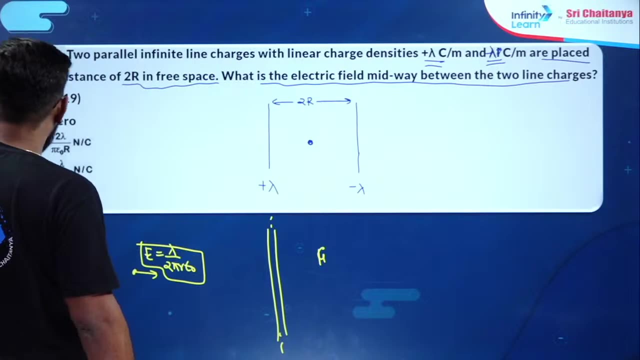 lambda upon 2 pi R epsilon naught. now suppose line is given as mass, there is a mass on it. total of M, mass is going up. so here, how much will be the gravitational field line? here, how much will be the gravitational field line? tell me, sir. let us relate. 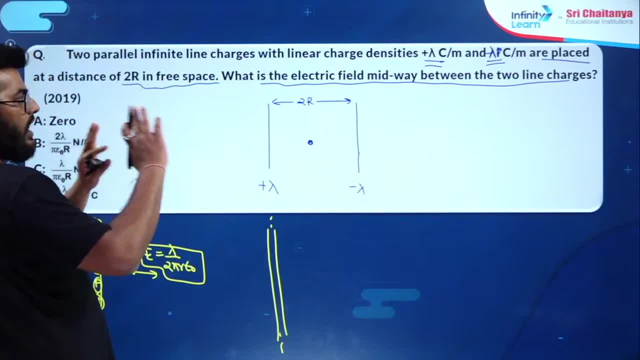 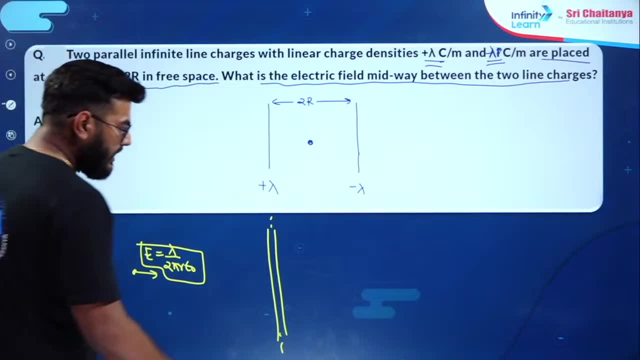 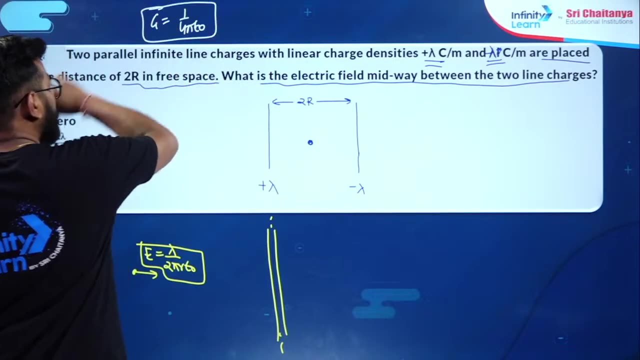 how will we relate? suppose the same question came on your gravitational field line, that here two infinitely line masses are given. how will you do then? simple point: you have to remember that the G is your 1 upon 4 pi epsilon naught. the G is your 1 upon 4 pi epsilon naught. 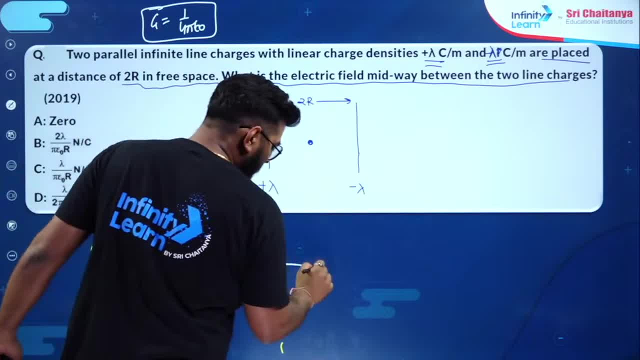 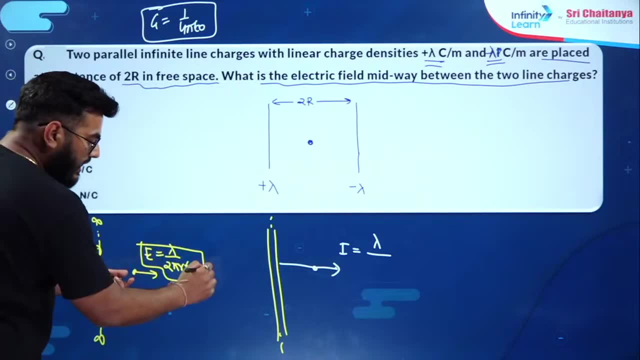 here, 1 upon 4 pi epsilon naught has to be generated and its value has to be applied. so here the gravitational field intensity will be I, how much will be lambda upon 2 pi epsilon naught? do one thing: 2 and 2 will be multiplied up and down. 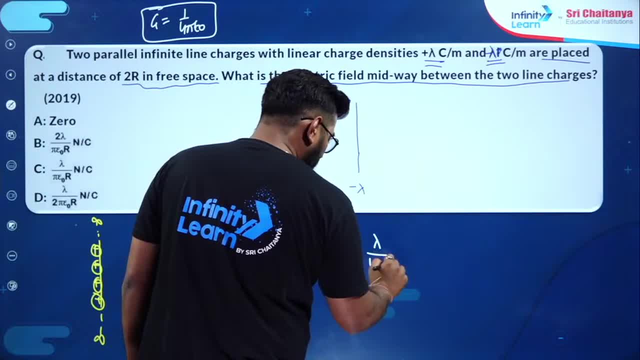 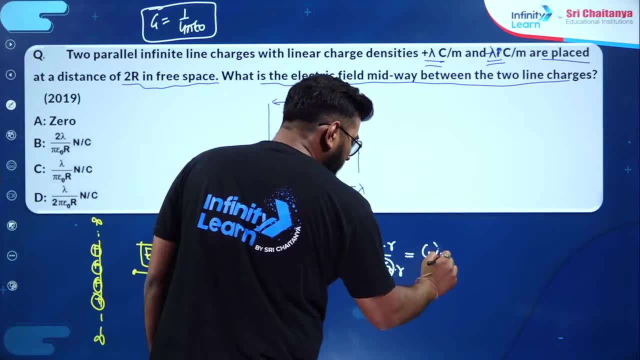 so how much will it be? lambda upon 4 pi epsilon naught into R and one more R. now, how much is 1 upon 4 pi epsilon naught equal to G, so the value will be G lambda. G lambda 2 is here 2G lambda upon R. 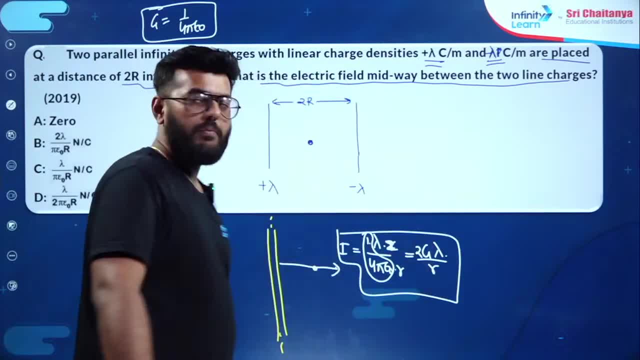 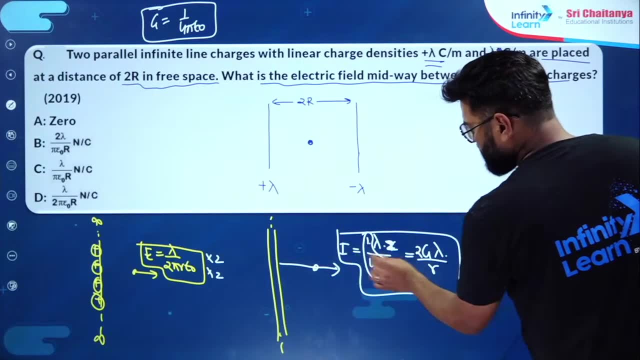 this will be the gravitational field intensity. how much will it be? 2G lambda upon R? are you understanding the thing? if I talk about an infinite line of mass, then in its near about region, which is gravitational field intensity, how much will it be 2G lambda upon R? 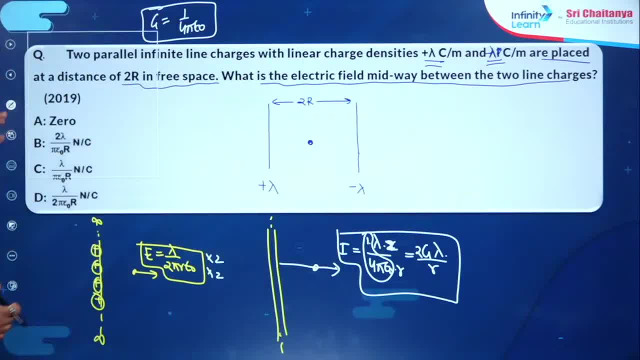 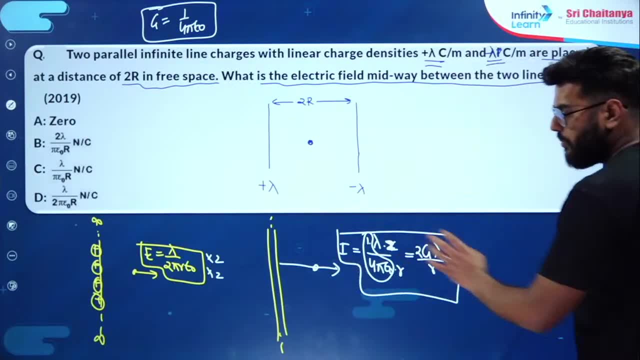 this. I am just teaching you to relate. my agenda is to take gravitation and electrostats together. that is all that you learn to relate. you know this, but you should also know this question can come tomorrow. question can come tomorrow. this is easy to do. there is no problem in this. 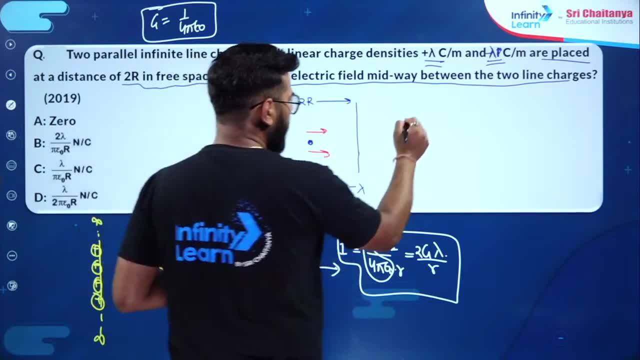 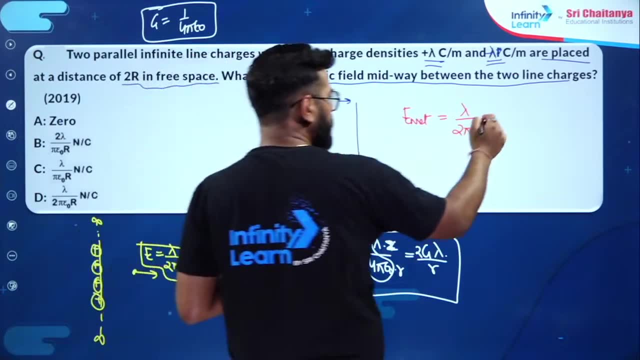 because of one it will come here, and because of the other it will also come here. so how much will be the total net? lambda upon 2 pi R epsilon naught, and because of both the words are coming towards it, so 2 will come. so 2 by 2 cancel. 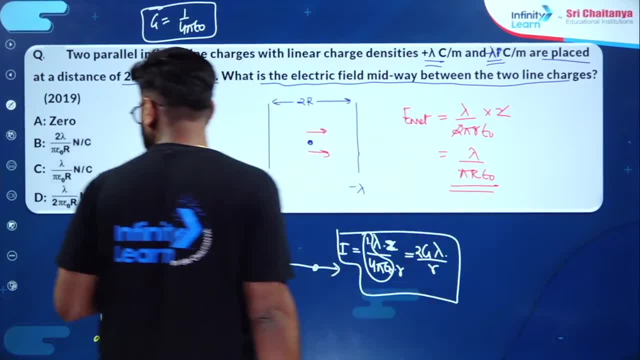 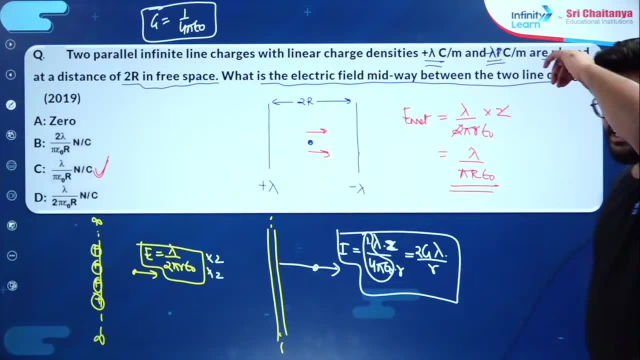 means lambda. upon pi R, epsilon naught option number. option number is C, so option number is C. are you understanding? is it clear or not? B, D, neither B nor D. what is the correct answer? option number is C. option number is C. are you understanding or not? 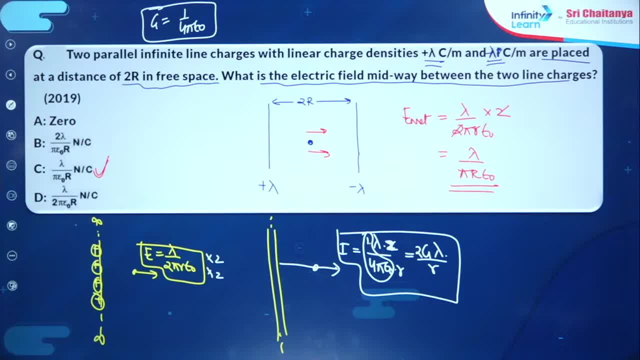 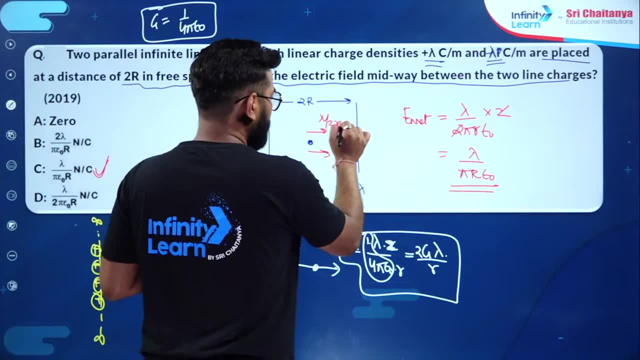 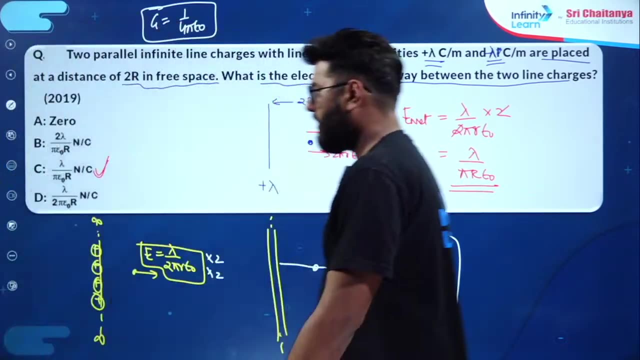 one plus lambda is given and one minus lambda is given. one plus lambda is given and one minus lambda is given. okay, so lambda upon 2 pi R epsilon naught, and because of this also lambda upon 2 pi r epsilon naught. Learn to relate. this is more important. 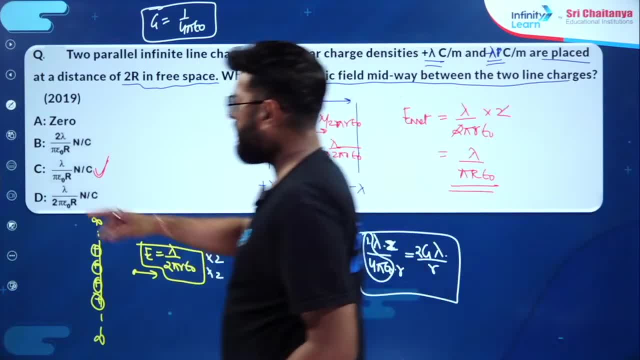 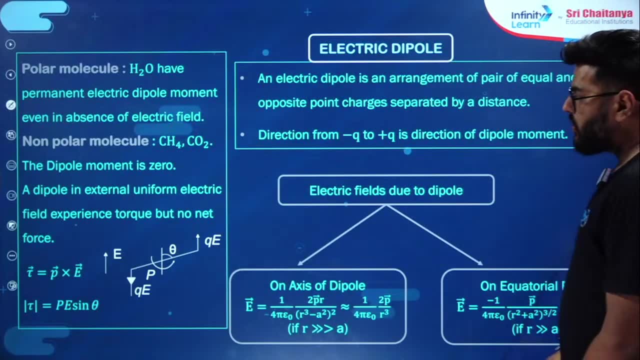 So this is related to this. Now let's switch and read a little about the concepts related to electric dipole and Gauss law. So if I talk about electric dipole, which is an individual topic of electrostats, So electrostats is a concept that is very much asked. 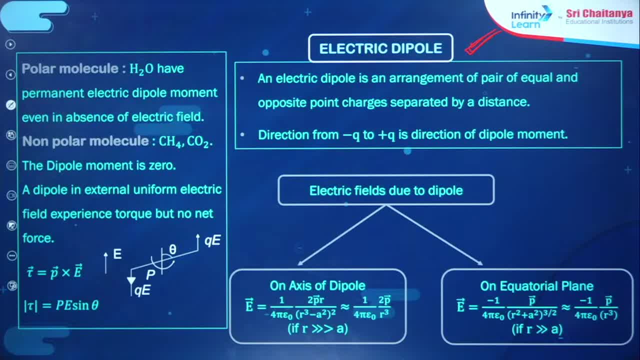 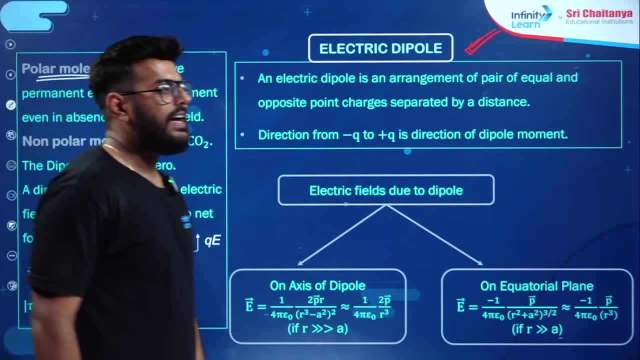 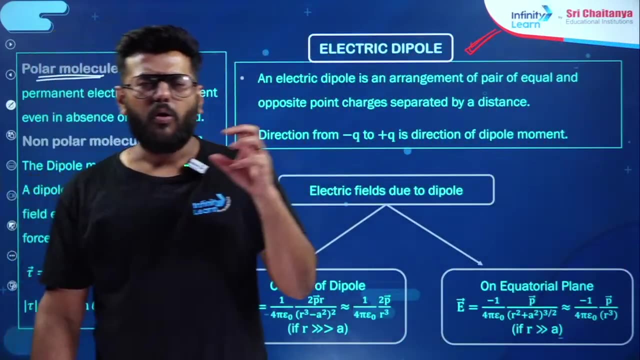 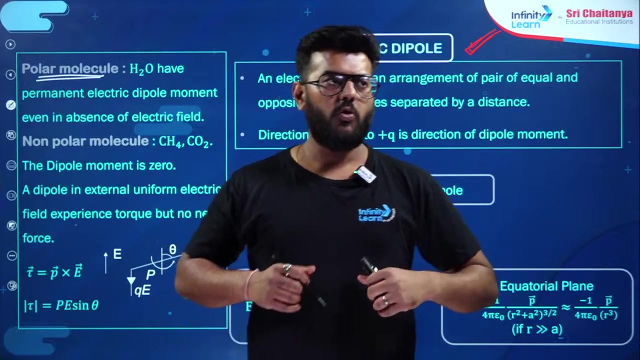 There is a possibility to get this question because it is one of the favourite topics Now. firstly, what are polar molecules? The existence of dipole itself is what happens. Its existence is simple if you have maintained positive and negative, equal and opposite charges on a particular distance. in some materials they exist naturally, like H2O. 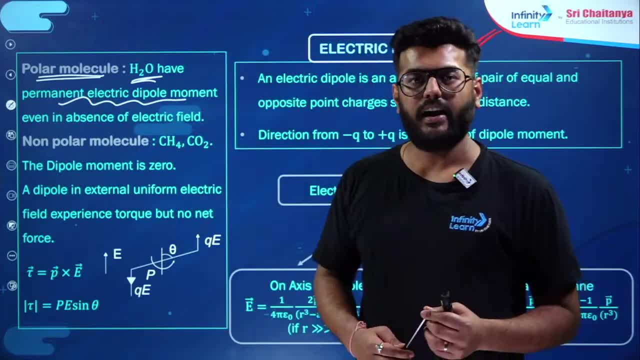 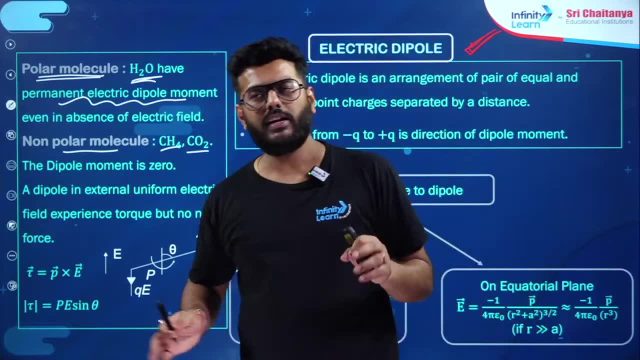 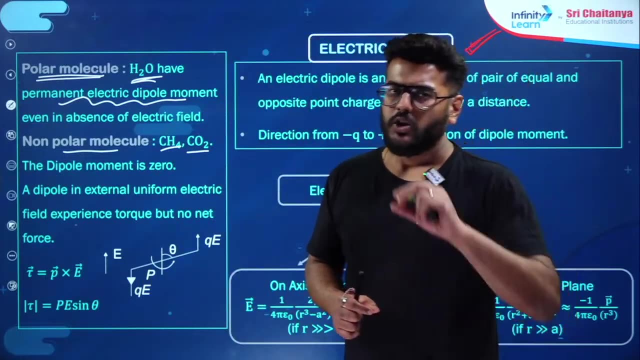 h2O. X2O is a molecule in which a permanent electric dipole is created, and in non-polar molecules like CH4 and CO2, dipole moment does not remain individually. overall, if you see, positive and negative are arranged in such a way that they do net dipole moment is zero. so if positive, 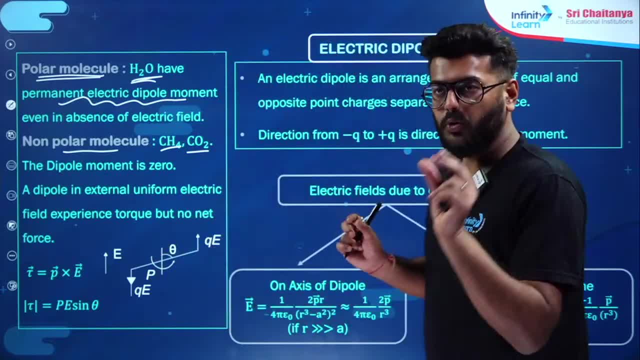 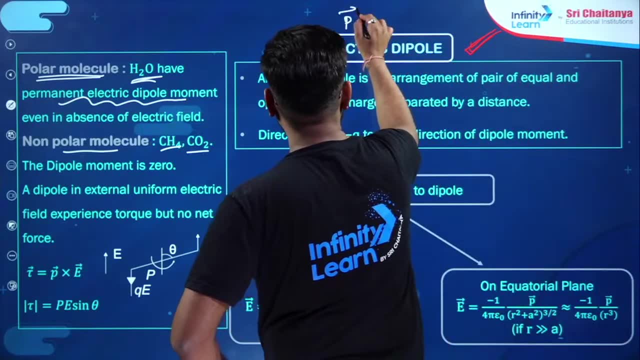 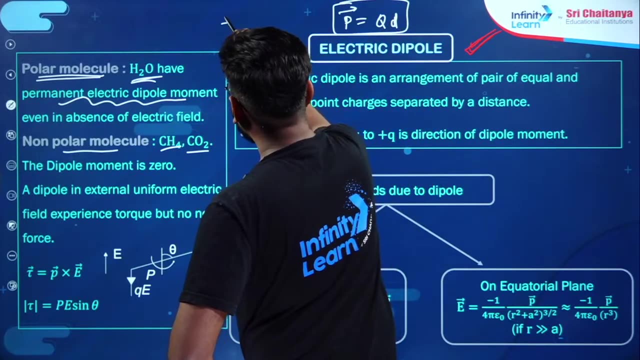 and negative charge is created in space, then it is called dipole. dipole means two poles, so electric dipole is defined by electric dipole moment, which is P, is equal to the charge, which is divided by the distance between them, is D, and the direction will always remain. 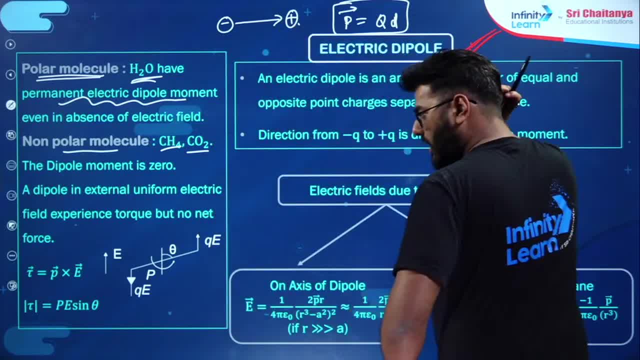 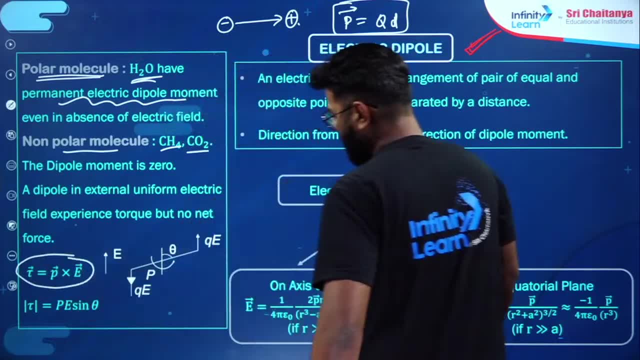 from negative to positive charge. now if you keep electric dipole in external electric field that is uniform, then the net force will remain zero but the torque will remain P cross because of electric field dipole. it is very important to take out two points. 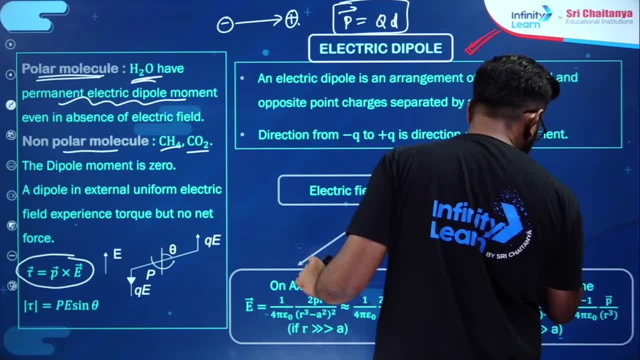 which gives a question. the first point is the axial position, which means the one which lies at the axis of the electric dipole. the other point is the equatorial position, where the point is to be drawn. This is the point where the electric dipole is placed. there is a point on which a point. 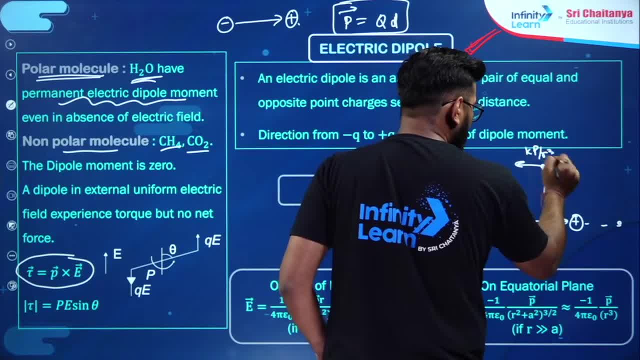 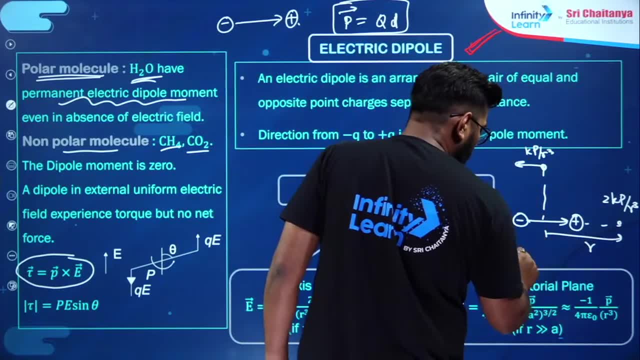 is drawn. Hence the electric dipole is a point on which a point is drawn, hence the point is to be drawn. This value is Kp upon R cube and this value is 2 Kp upon R cube. Remember one thing: to measure these distances you have to take an approximation, that the value of R becomes very big if the length of 2A is A. 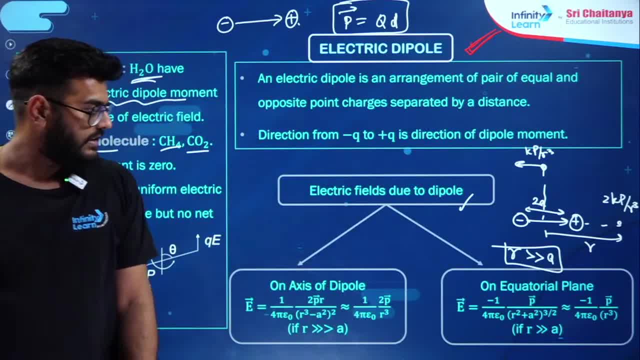 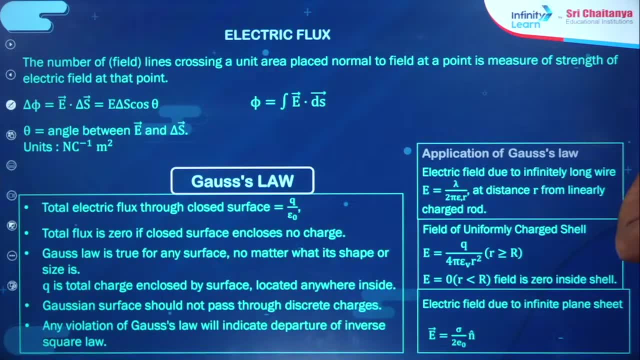 The length of the dipole remains very big. Then only the values come on the equatorial plane, minus Kp upon R cube and Kp upon R cube on the axis. The second individual topic here is Gauss law. Now I will show you how you can relate Gauss law to your gravitation. 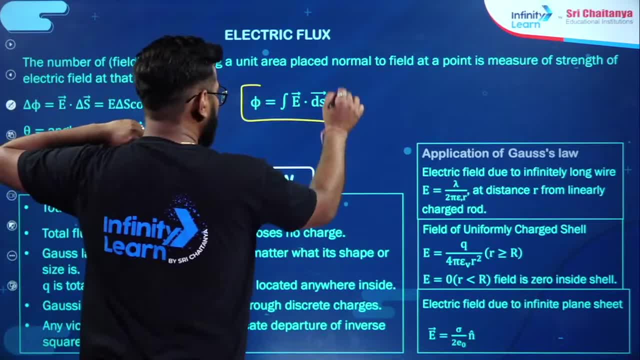 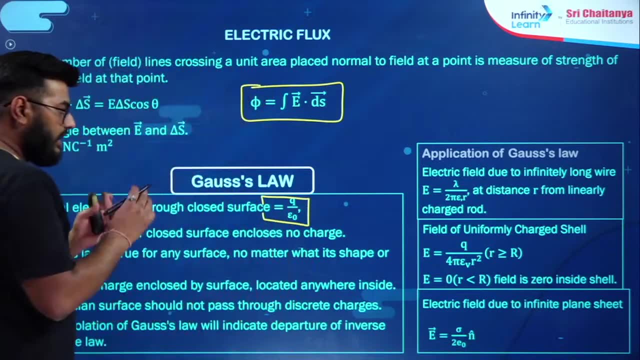 If I talk about Gauss law, then Gauss law is simple: E dot, DA. this is how you get flux. Gauss law says that the flux you are getting is equal to Q enclosed upon epsilon naught If it is a closed surface and you can relate it to the charge inside it. 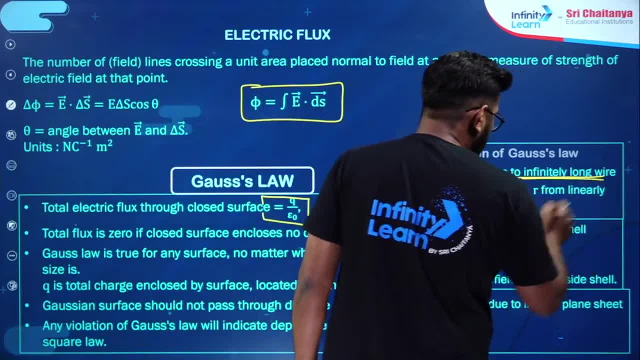 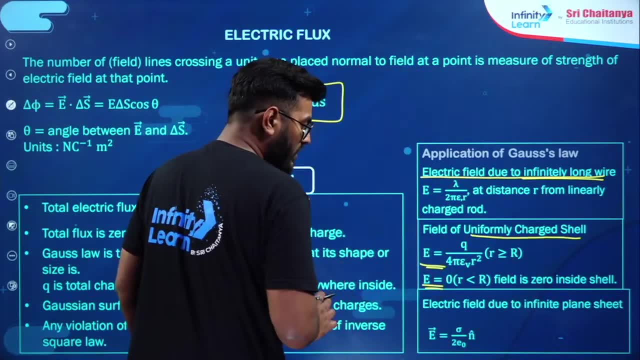 With the application of Gauss law you can get electric field infinitely for line charge. You can tell in a uniformly charged shell that electric field inside will be zero and Kq upon R cube will be outside. You can get electric field due to an infinite plane sheet which is equal to sigma by 2 epsilon naught. 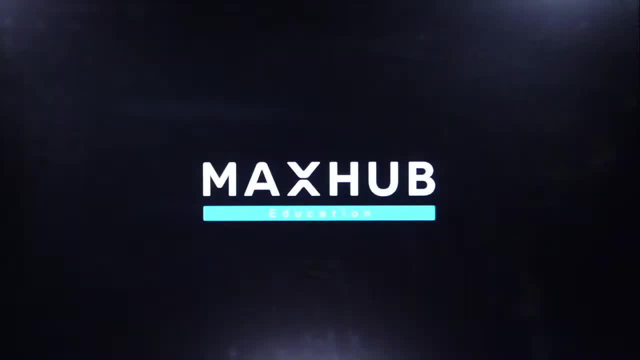 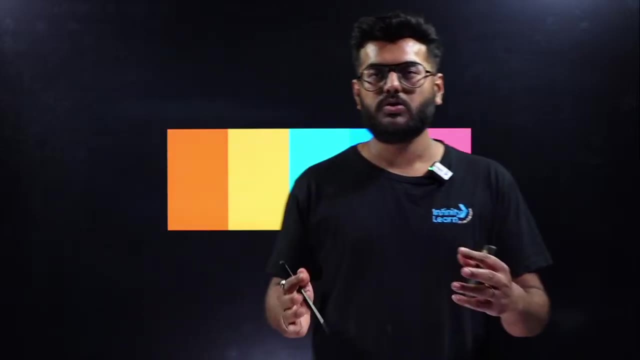 Wait for a minute. the TV is off. Take a pause of 2 minutes. the TV is restarting. So the Gauss law exists in electrostats: Whatever flux is related to a particular closed surface, that becomes your integration of the flux. 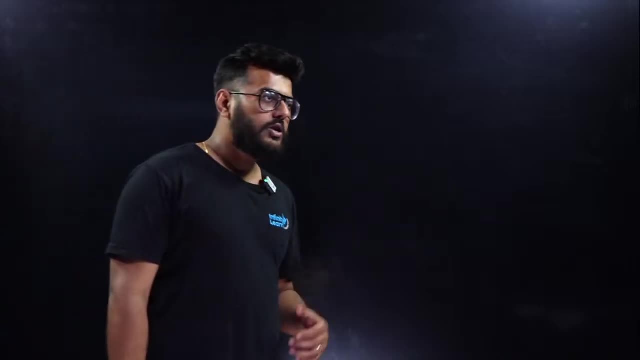 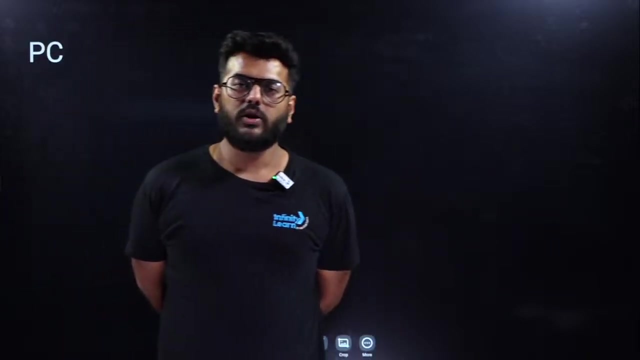 That becomes your integration of the flux. That becomes your integration of the flux. We have come up with the method of calculus, And the other method is that the charges inside that closed surface are Q enclosed upon epsilon naught. Now the same principle is also used in gravitation. 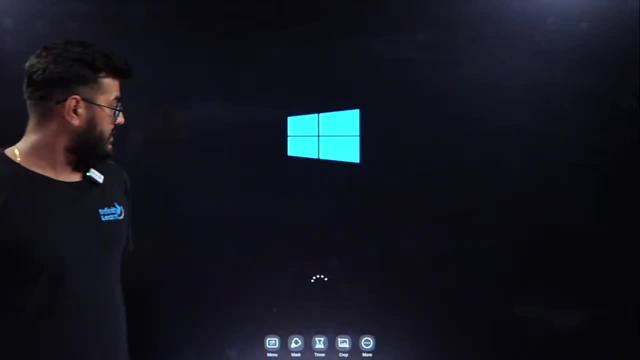 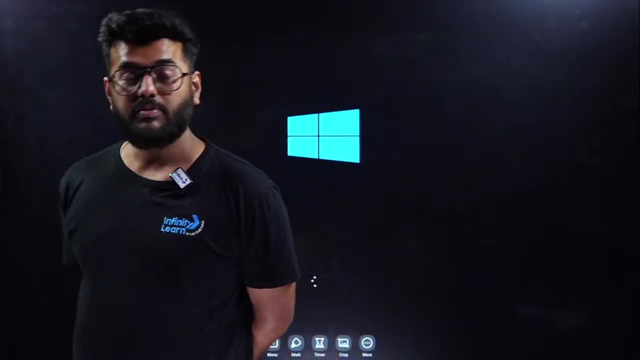 The integration of I dot DA. the way you can get flux, electrostatic flux that is equal to M, enclosed upon epsilon naught. Instead of E you have to put 4 pi into G, So M enclosed into 4 pi into G. 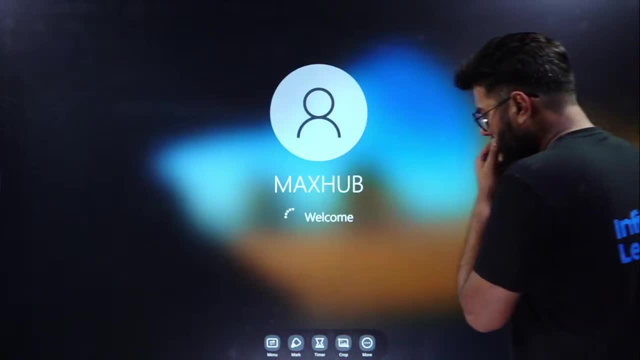 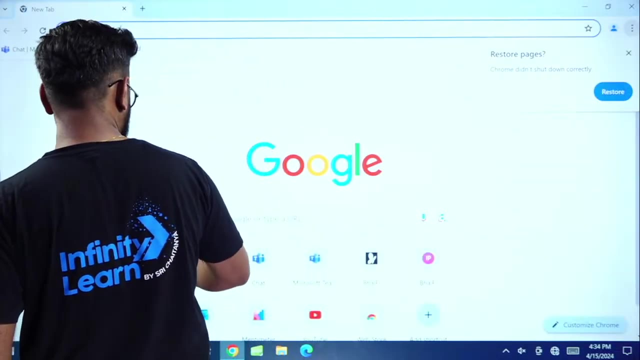 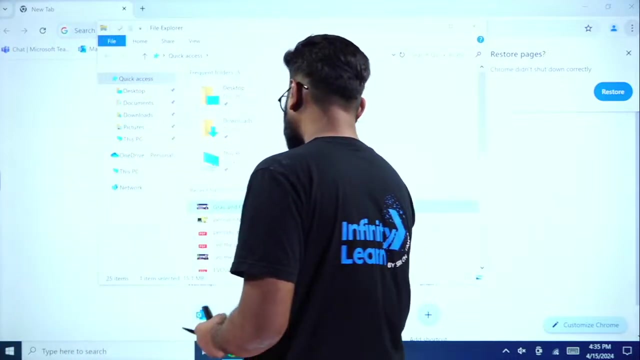 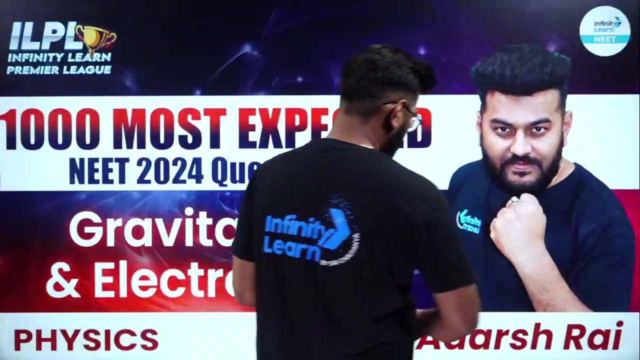 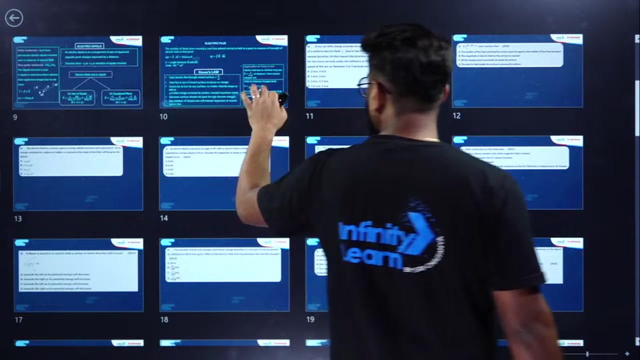 Okay, I will write the formula also. wait a minute, let it start clear till the time you tell me what are the doubts. if there is anything else, then doubt. Wait, where were we? we were here. we were in Gauss law, okay. 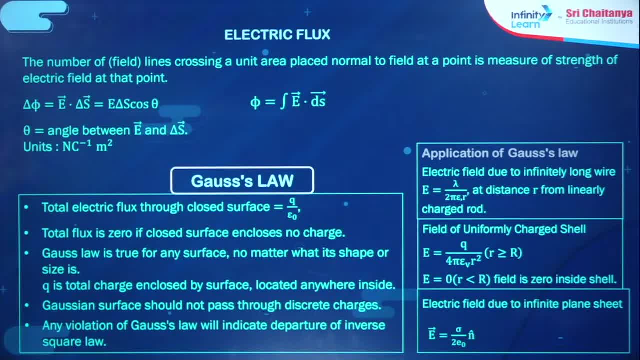 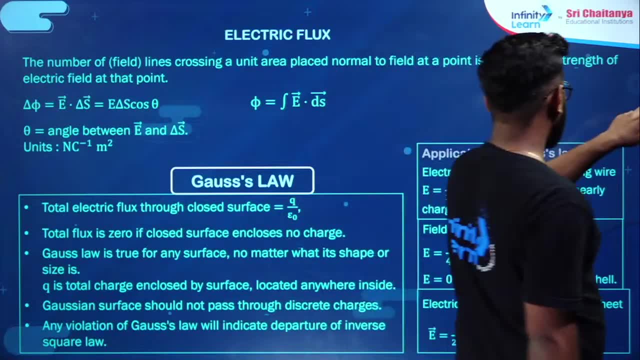 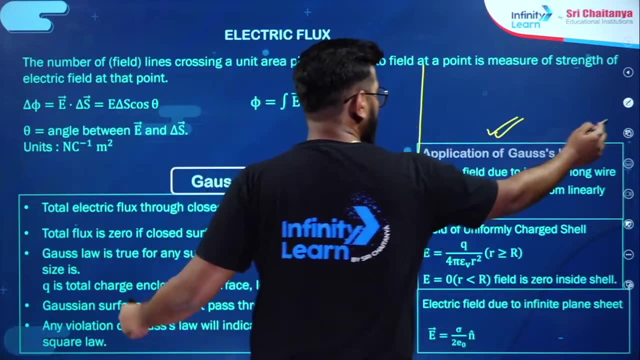 So I am non-standard. So when can I do for it? What do I have to do? I have to prepare for JEE Neat. Start it now. Okay, So this is application of Gauss law. Now, if I put Gauss law in gravitation, Then how will it look? 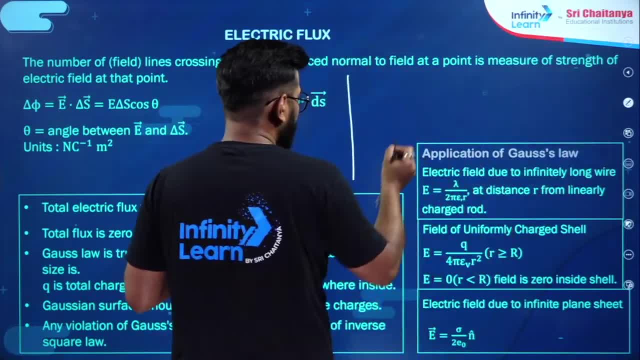 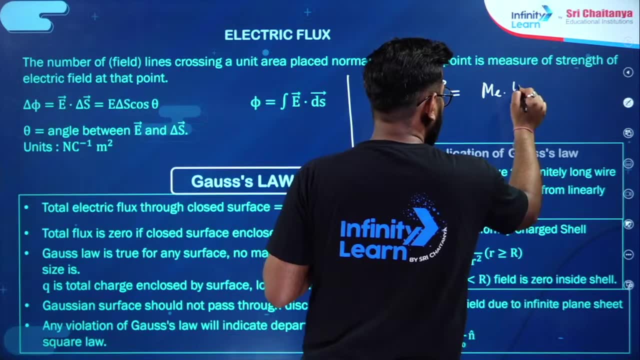 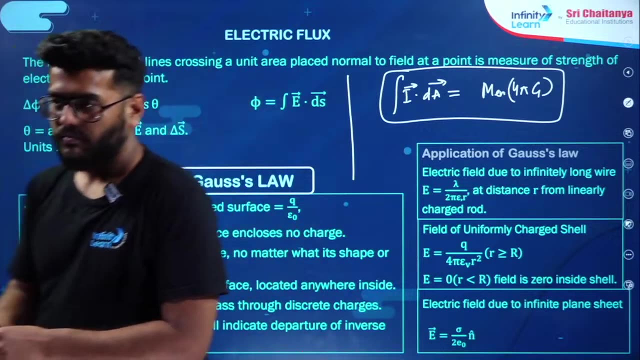 If I put Gauss law in gravitation, Then how will it look? It will become simple. Integration of ID Will be equal to M enclosed into 4 pi G, 4 pi G. This becomes your Gauss law application In gravitation. Okay, Now we will do something related to this. 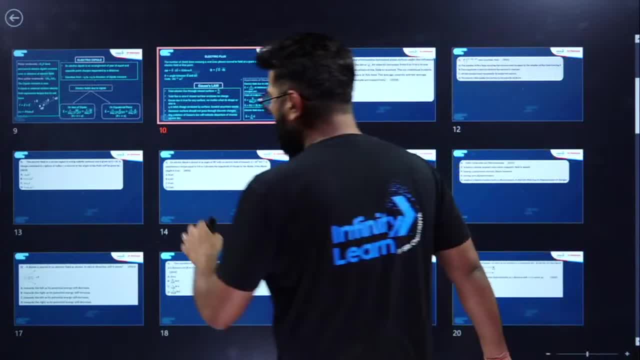 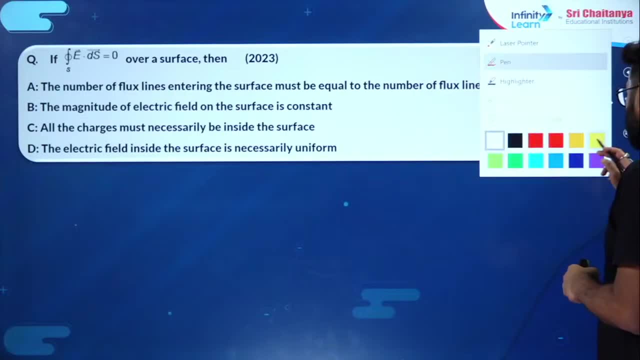 Do something related to this Question. We will do your question. What is the name With this? From electrostats? But you have to understand that thing In a way that you are able to understand gravitation. Okay, For discrete mass systems, Force Can be removed. Then yes, Yes, For discrete. 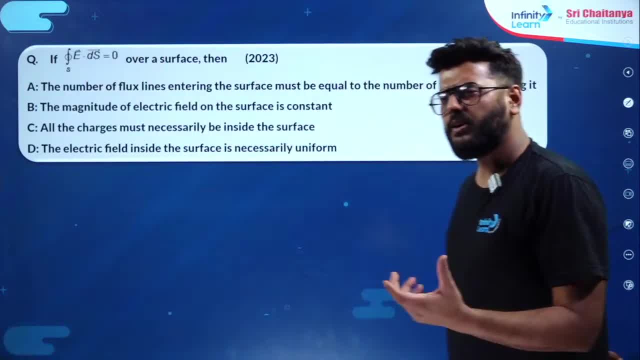 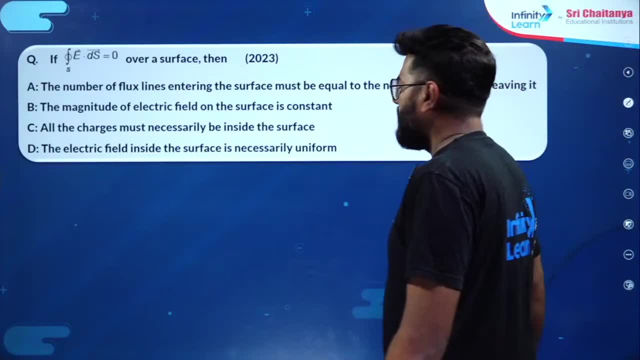 Can be removed, Then yes. And for continuous mass bodies, if symmetry is maintained, then we can get it out. For example, integration of EDA over a surface. if it is equal to zero, then what does it mean? EDA. if it is equal to zero for any surface, then what does it mean? 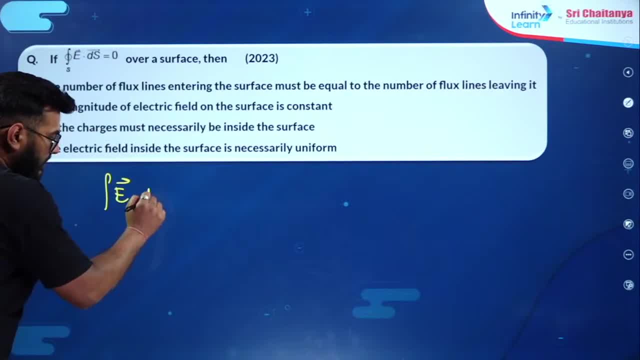 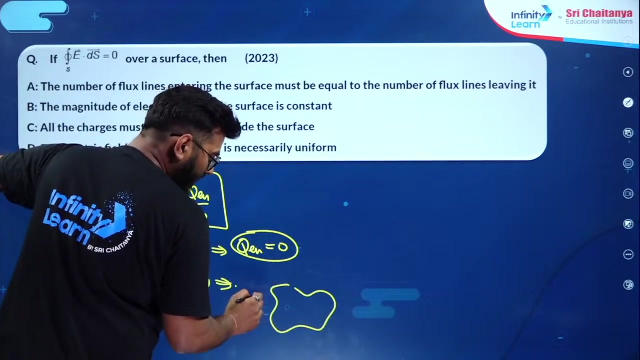 It has two meanings. First meaning is that enclosed charge of that closed surface is zero. First meaning, conclusion number one: Conclusion number one is that the enclosed charge will be equal to zero. And the second conclusion is that the number of field lines taking entry, the same number of field lines are taking exit. 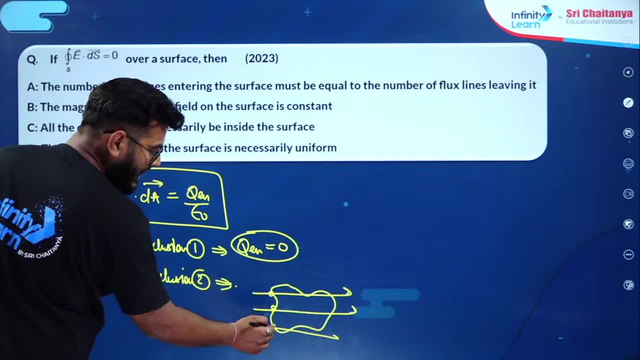 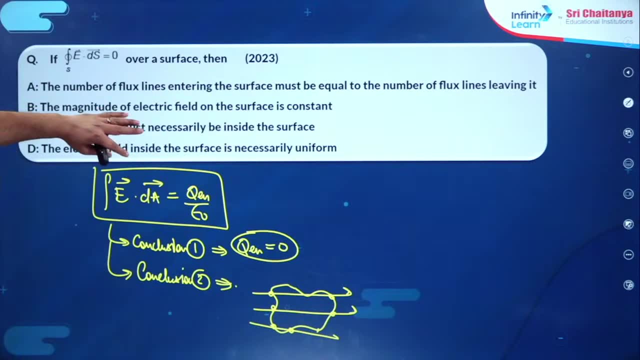 The number of field lines taking entry, the same number of field lines are taking exit. Both of these meanings are there Here. you can see that three took entry and three took exit. The number of flux lines entering the surface must be equal to the number of flux lines leaving it. 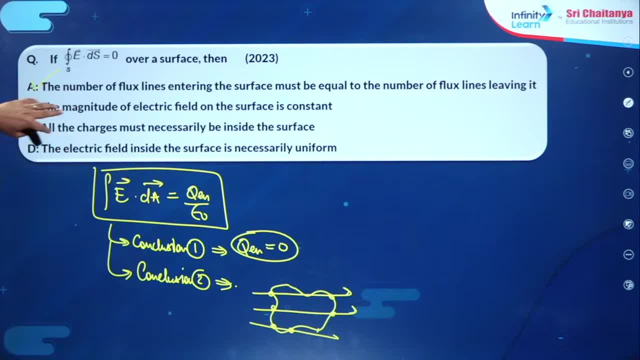 Yes option. Option number A is absolutely correct. Now, looking at this situation, it is correct. Magnitude of electric field line on the surface is constant. No, All the charges must be inside, No, Inside. I don't want to stay. 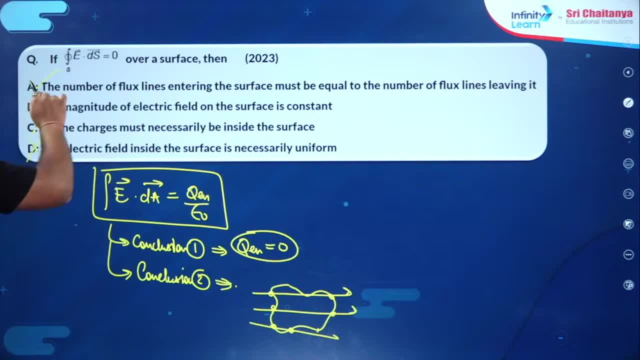 I want to do Q and close zero Electric field lines in the surface is no. Option number A is absolutely correct. Option number A is absolutely correct. What is the matter, Muskaan? very good Abhishek, absolutely correct. 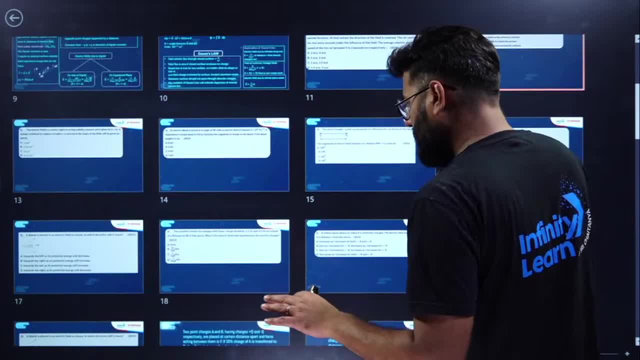 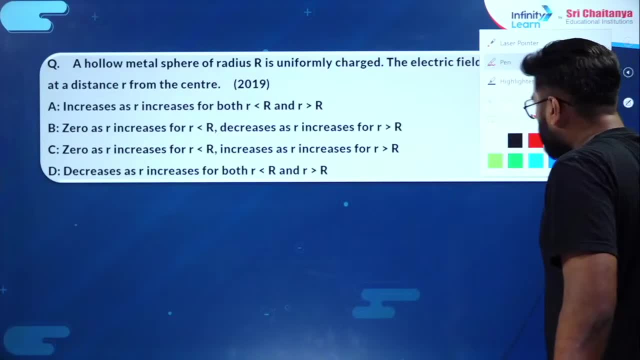 Absolutely correct. Next, if I talk about this, look at this. There is a hollow metal sphere of radius R. There is a hollow metal sphere of radius R. It is uniformly square. The electric field due to the sphere at a distance R from the center is 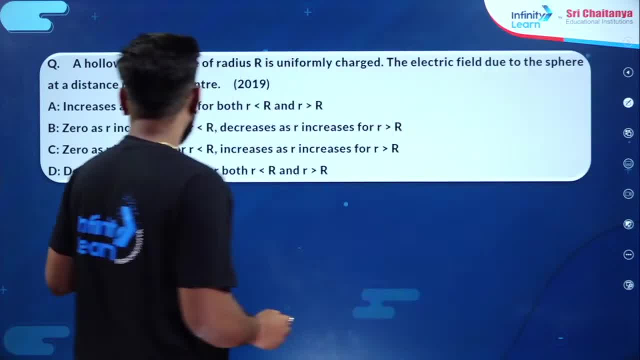 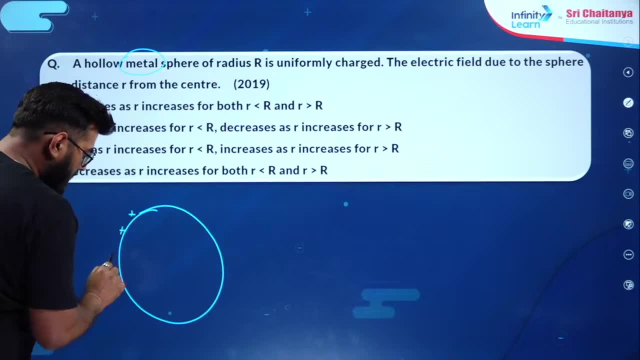 It is a simple logic. Look if I talk about a hollow sphere and it is also metal, ie conducting. So whenever you give charge in conducting surfaces, it exists only when it comes to its surface. Where does it exist? 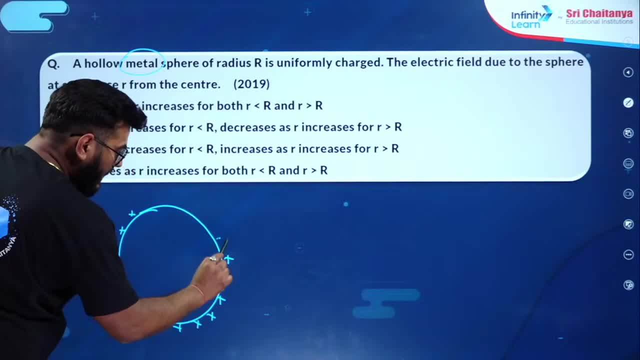 It exists only when it comes to its surface. Okay, It exists only when it comes to its surface. And if it exists only when it comes to its surface, then if I talk inside, then the electric field inside always becomes zero, Because there is no Q and closed. 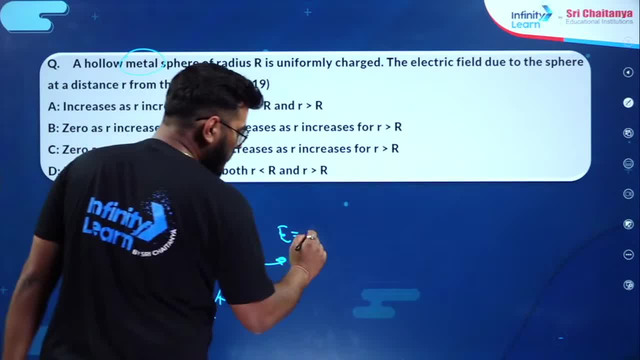 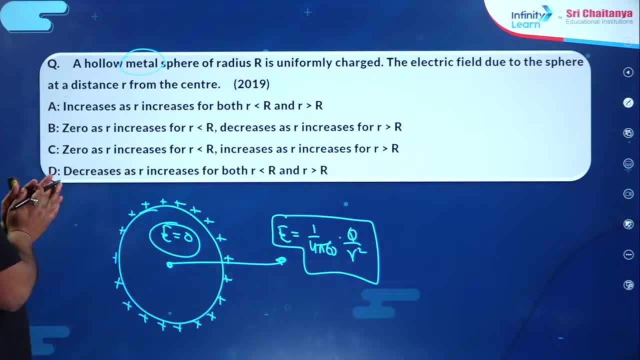 And if I go outside, then the electric field outside becomes 1 upon 4 pi. epsilon naught capital Q by R square, wherever there is a charge on it. So if I make its graph, then how will it be? How will I make the graph? 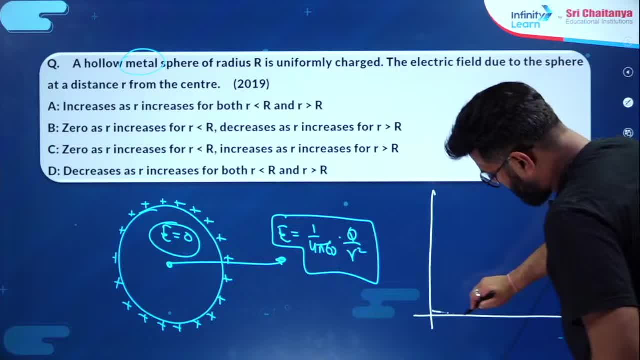 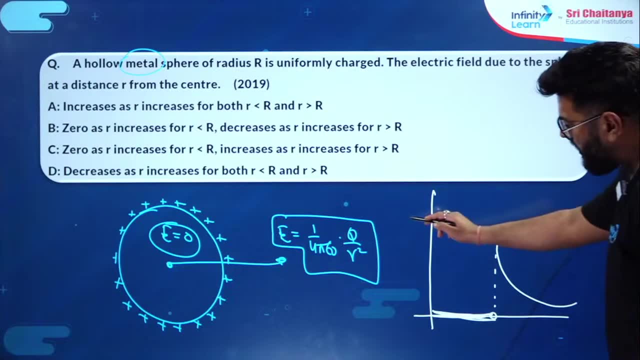 Look at the graph. it will be like this: Very standard things. Initially it remains zero And later the graph will go up and then it will vary inversely, like this: So this is the graph of electric field and R. 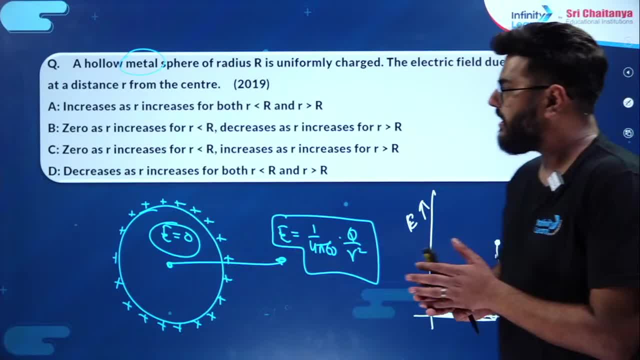 This is the graph of electric field and R, So here you can see which side it is sitting on: Zero, as R increases, for R is less than R, and decreases, as R increases, for R is greater than R. Option number B is absolutely correct. 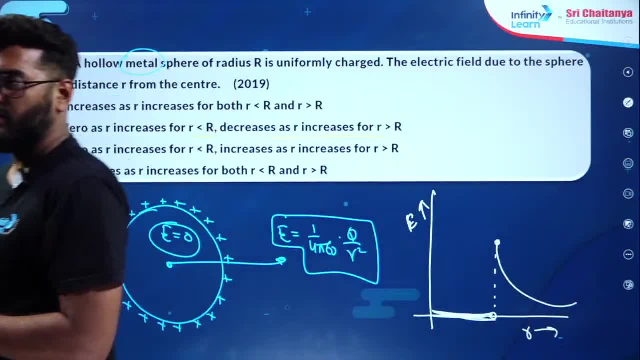 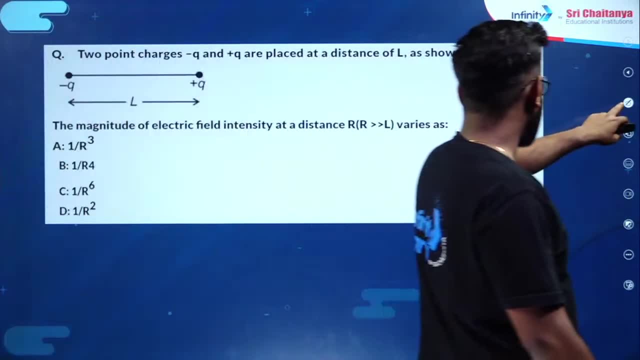 Option number B is absolutely correct. Right, Option number B is absolutely correct. Understood, Okay, Done. Look at the other question. Two point charges. Now let's talk about some questions related to dipole. Now dipole question. 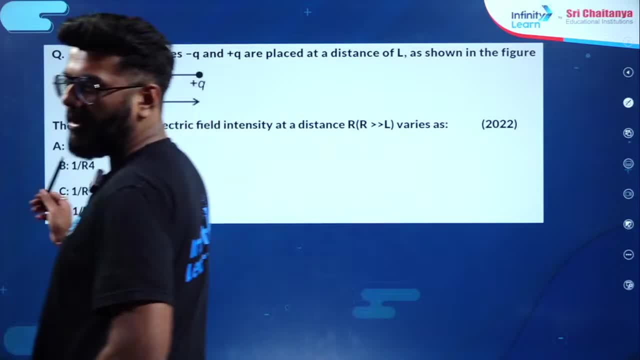 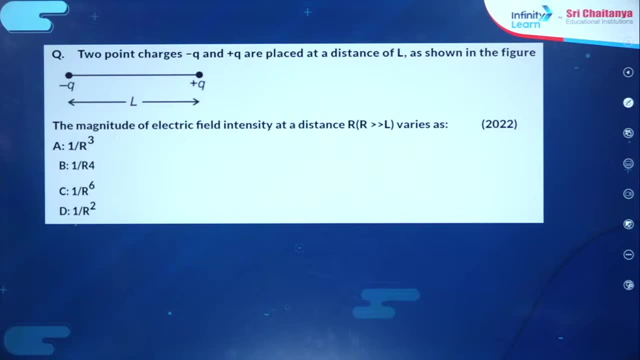 Are you looking at this question today? This question came in JEEK's January attempt. This question came in JEEK's January attempt. Two point charges, minus Q and plus Q, are placed at a distance of capital L as shown in the figure. 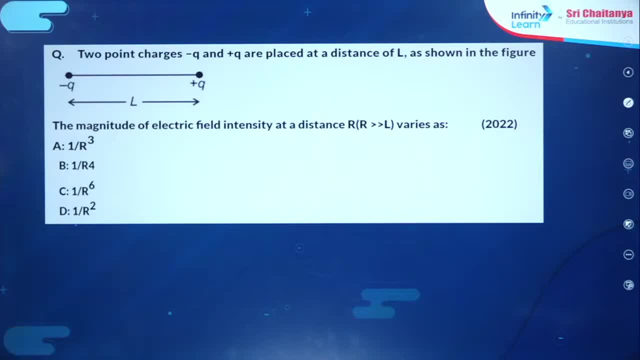 The magnitude of electric field intensity at a distance, R, varies as Now. how will electric field line vary at R distance? So do you see a dipole in front of you? Absolutely. And while looking at dipole, do you see one more thing? 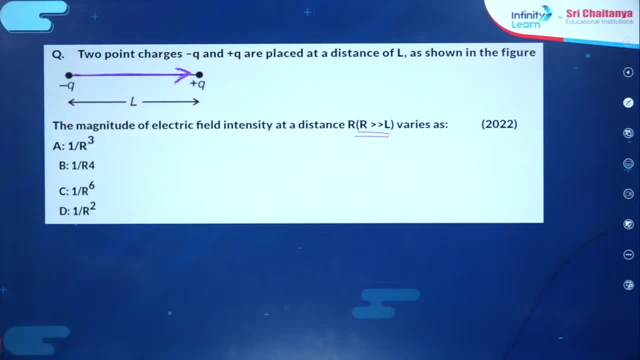 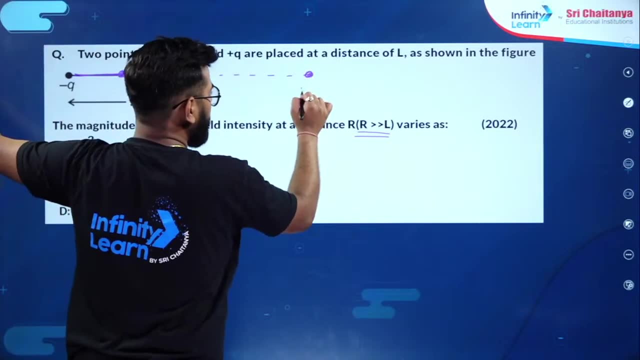 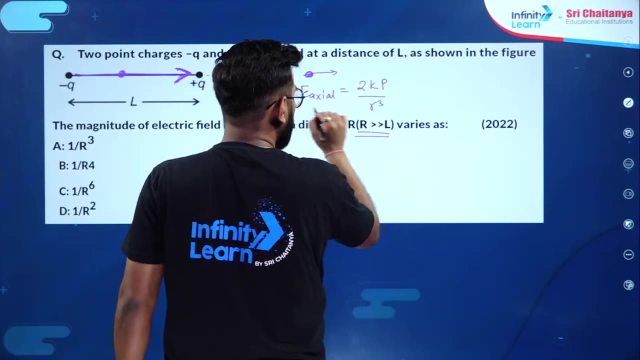 That is, R is very much greater than L, And this is the condition of an electric dipole, when I can say that on its axis, the electric field line will be at an axial point of 2Kp upon R-cubes. 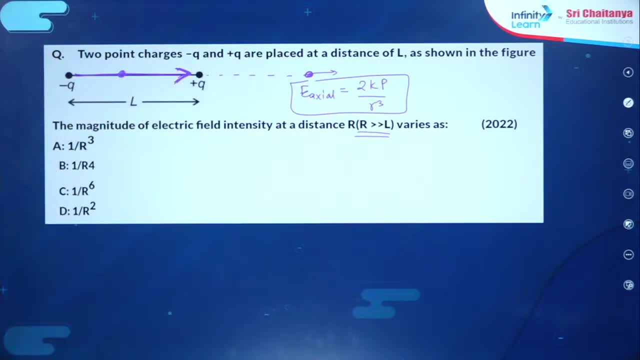 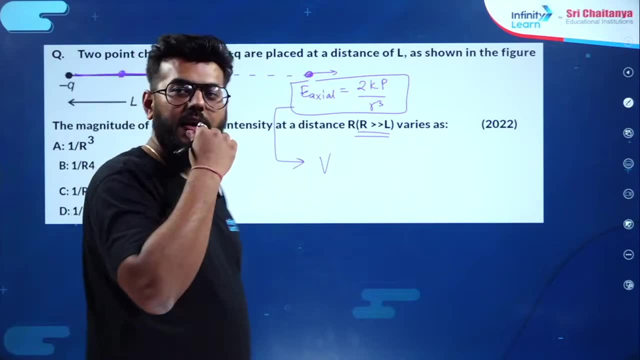 So you can see that the electric field line is equal to R-cubes. Now the question in JEEK's question did not come from the electric field line but from the potential. How much does the potential vary? What is varying? 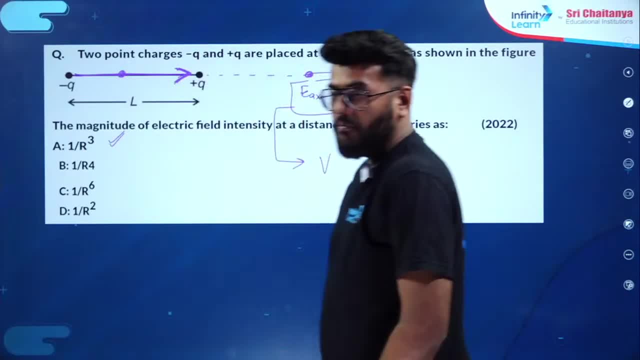 How much does the potential vary? This is the correct answer: 1 upon R-cubes. But the question in JEEK's question is exactly the same. But the electric field line is equal to 2Kp upon R-cubes. It does not come from the electric field line, but it comes from the potential. 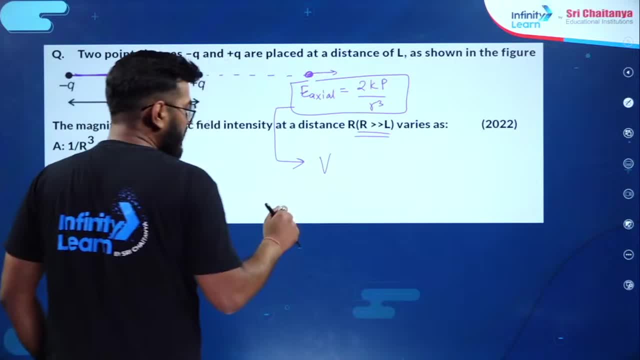 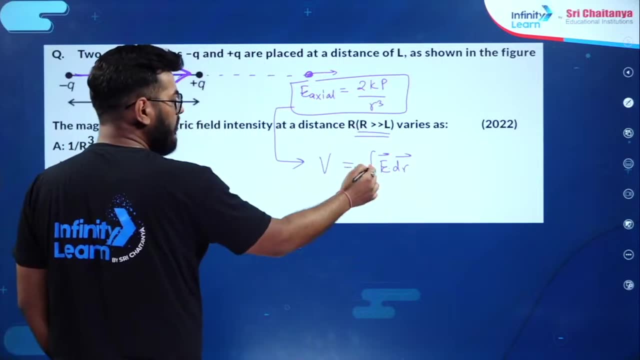 So how does the potential vary? The potential is the integration of E dot dR, minus of E dot dR. Now, if you integrate the potential of E dot dR with respect to R, Well, the problem is the R-cube does integrate. 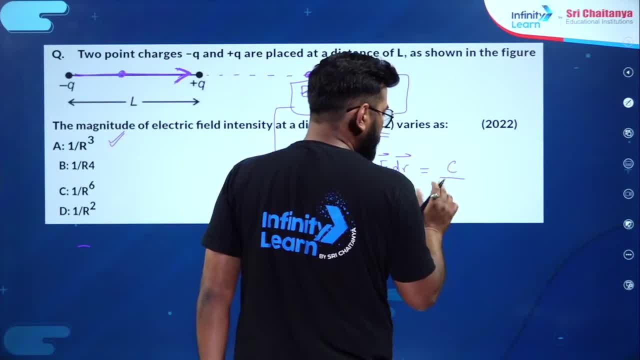 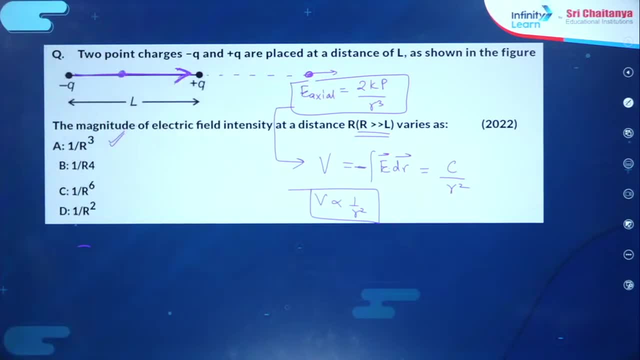 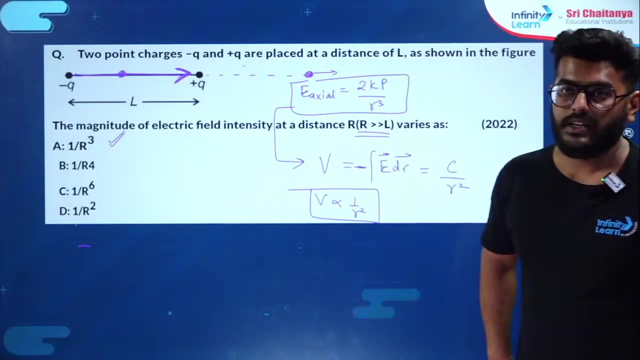 But the final answer will be some C constant divided by R-squared. So V is inverse to R-squared for a dipole And in that case the answer would be your option number D, Do you understand? So the question that came in JEE was of potential, not of electric field. 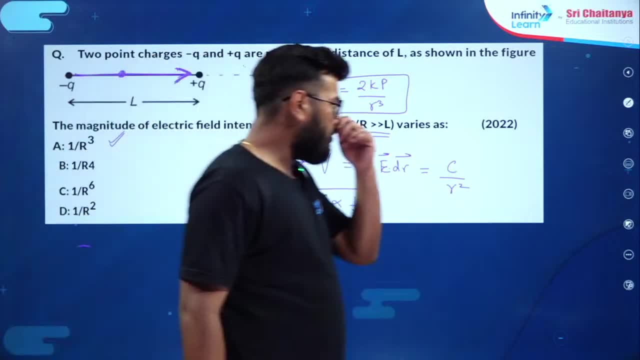 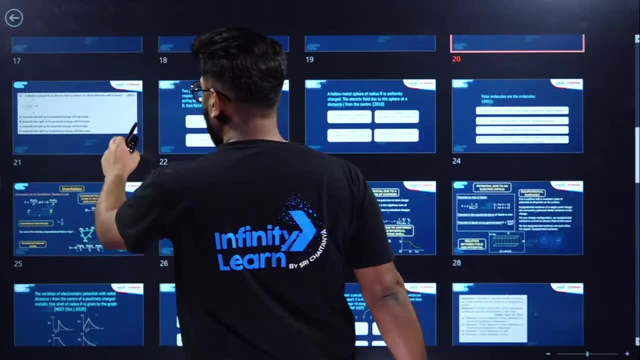 So with one question, you need to understand many more concepts. You don't have to stay focused on that question Like: look at this question, This is a very nice question which I think came in 2021.. That electric dipole is kept in electric field. 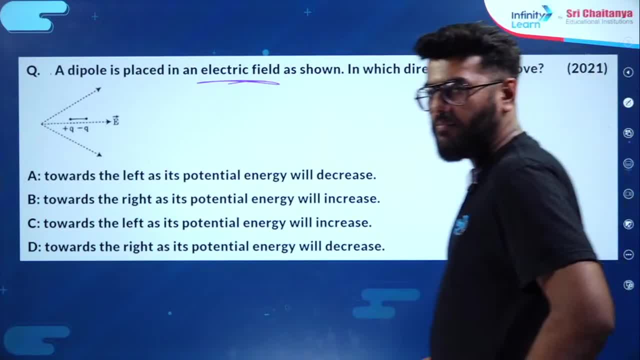 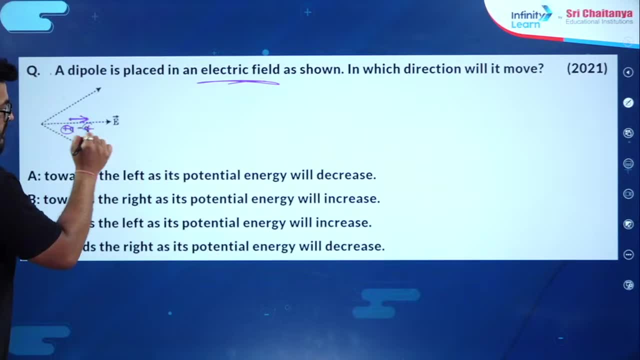 In which direction will it move? In which direction will it move? Look at the dipole in which direction it is kept. Here is your dipole. This is negative charge and this is positive charge. This is negative and this is positive. 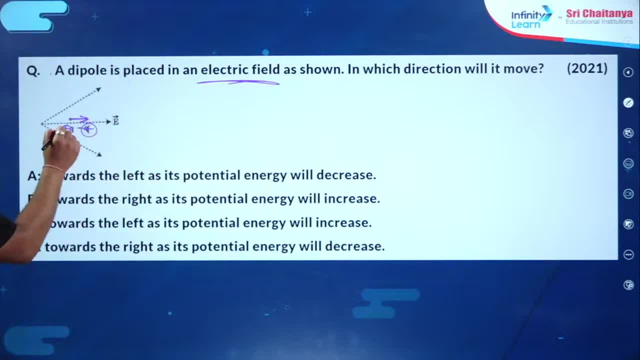 Now, where will the dipole go? Where will the dipole go? This is negative and this is positive. Where will the dipole go? Look at this, sir. If this was a uniform electric field, if this was a uniform electric field, 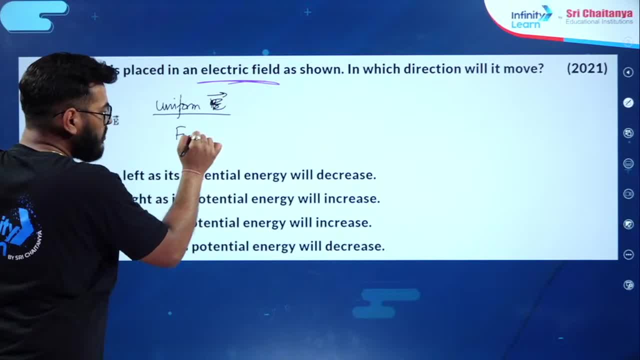 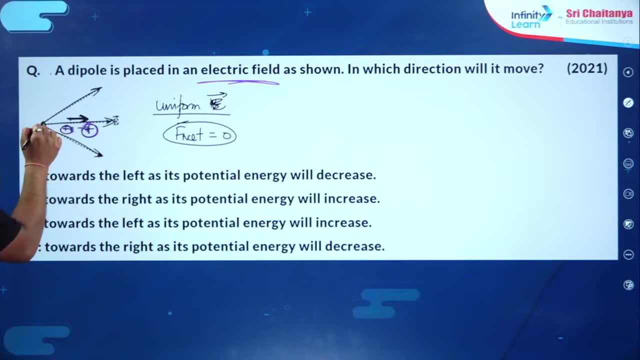 then the net force on the dipole would be. it would have been equal to zero. But because this is a non-uniform electric field, you can see that the electric field line is going like this In this way. And because the electric field line is going like this, 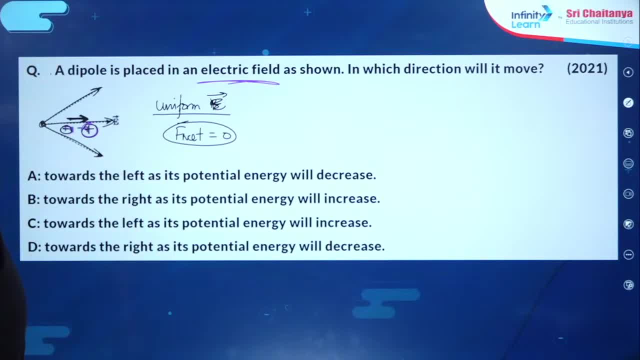 it means that the intensity of the electric field line is gradually decreasing. So the intensity here will not be equal to the intensity here. The intensity here will be less and the intensity here will be more. That means the force applied on this positive charge. 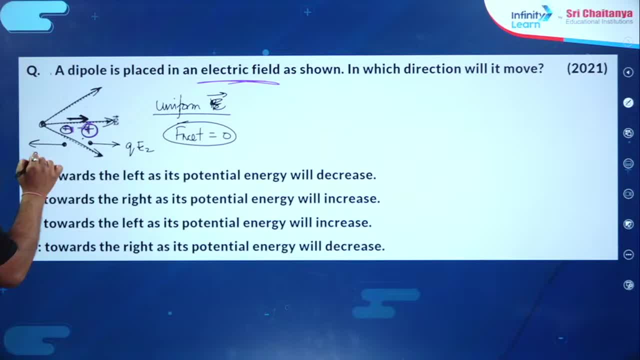 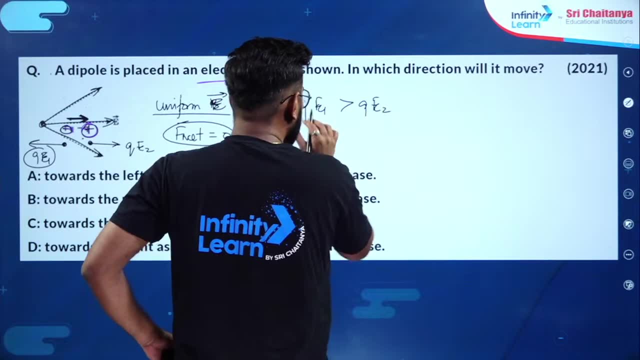 Q into E2, will be small And the force applied on this Q into E1, will be big. What is the value of QE1?? The value of QE1 will be bigger as compared to QE2.. And because the value of E1 is bigger than E2,. 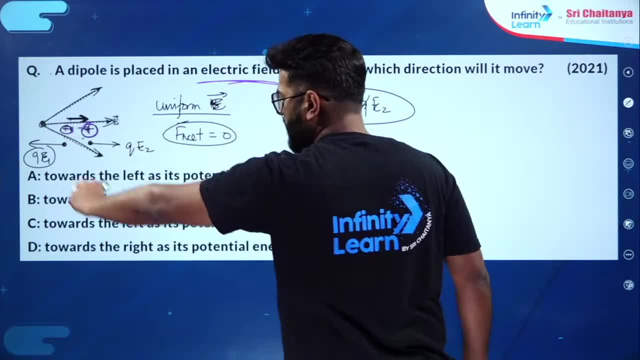 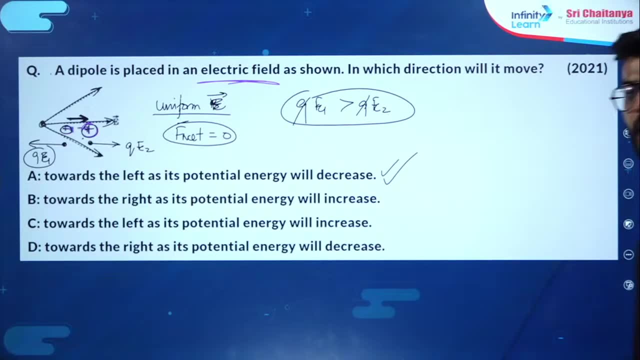 and because of this the dipole will go towards the left- Towards the left, as its potential energy will decrease. Option number A is the right answer. Option number A is the right answer, Sir. the logic above, once Limit L to R, goes to the right. 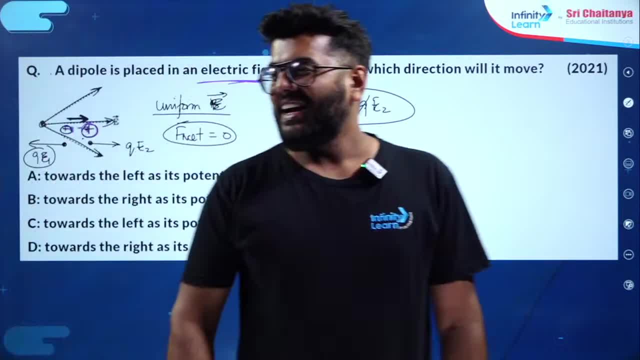 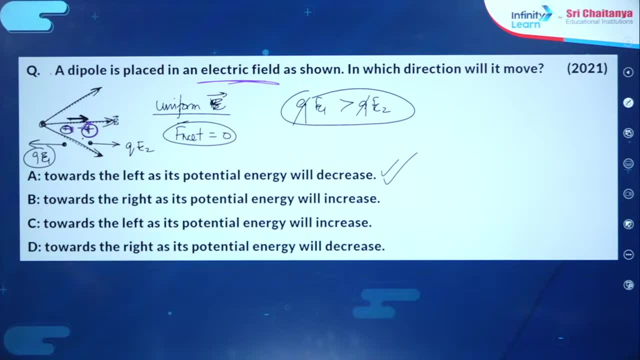 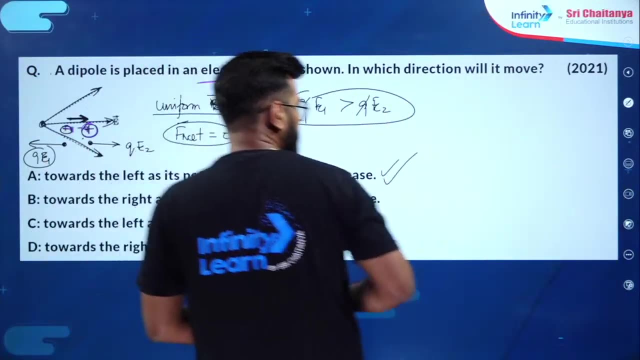 Which one are you saying? Solid angle: The surface charge density of both areas is x2.. So is that the reason of E being 0 at the center? For what case are you saying? Are you saying for this? Which case was this? 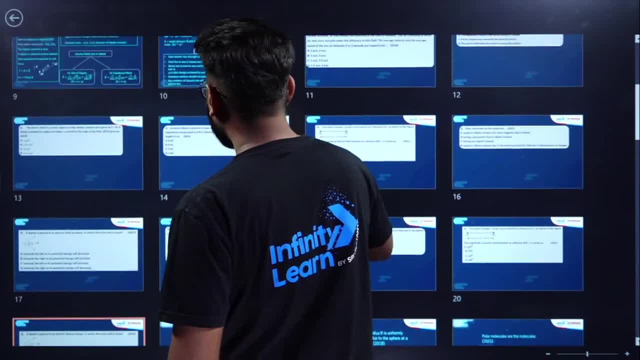 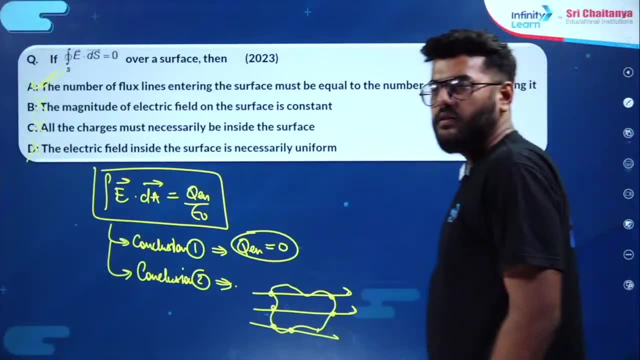 Which question did you say? Did you say for this question? Did you say for this question? E dot d A? are you saying for this? Are you saying for this, For this, for solid conducting sphere: ok, for solid conducting sphere: inside is zero. 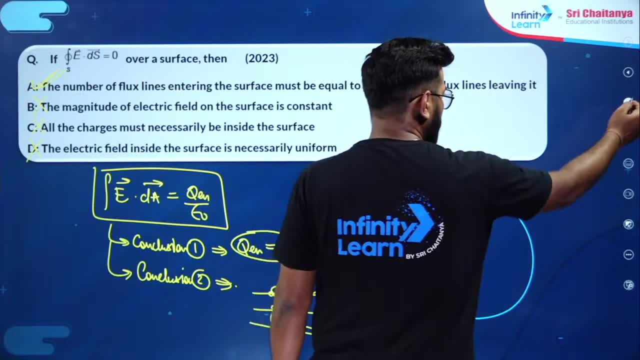 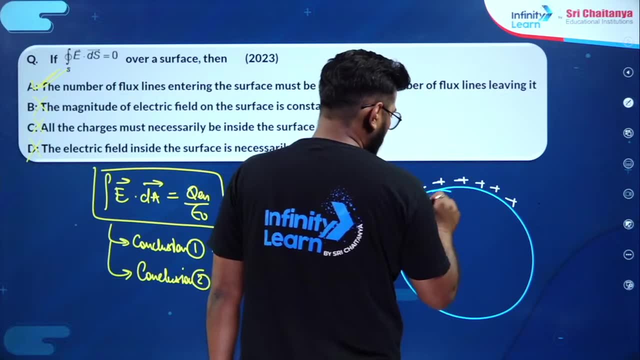 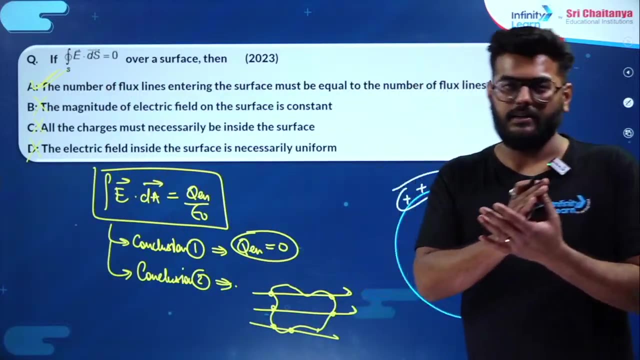 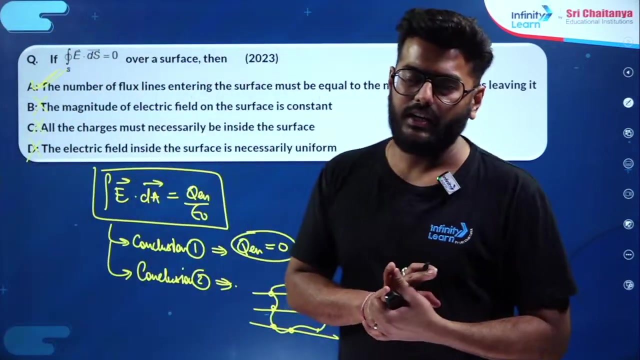 ok, yes, yes, yes, absolutely, absolutely. how is the charge distribution? by the way, look what is the point, Abhishek: that to zero electric field is a mandatory condition. electric field to zero is a mandatory condition. why? because if any of the electric field will have any one element, 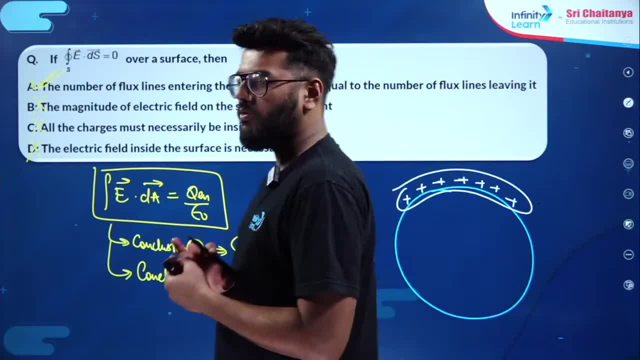 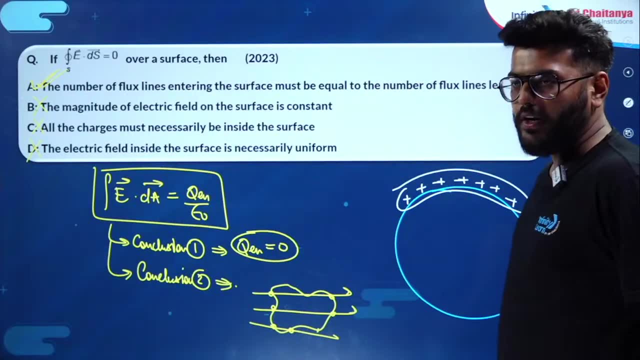 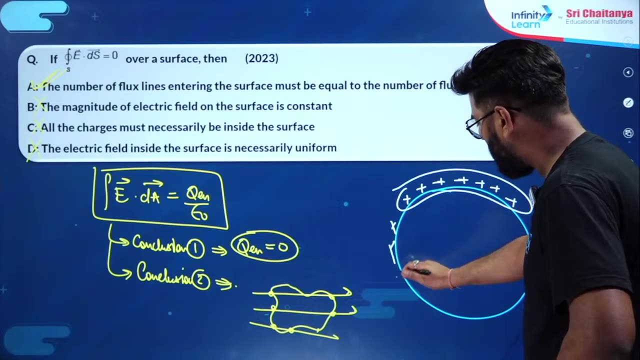 will have a small magnitude, then it will distribute so many charges. do you understand the concept of solid angle? the concept of solid angle, its logic is very good. for non conducting spheres may be. you are saying that, sir. there are so many of them and the rest of them? 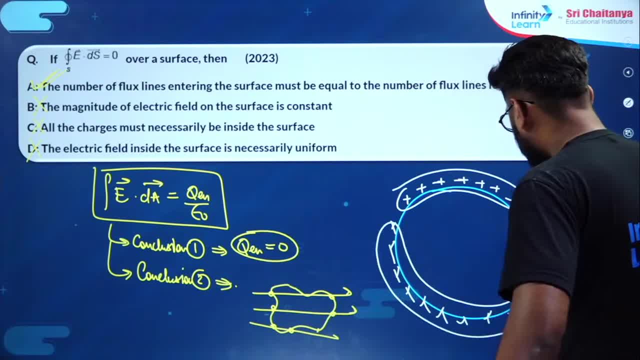 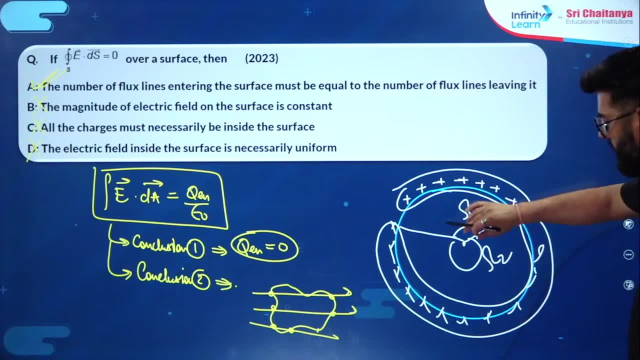 the rest of the solid angle here at the center. because of all these, the solid angle, sigma 2, and this will be because of sigma 1. so because of this, the charge will balance. that is why it will remain zero at the center. this logic is given. 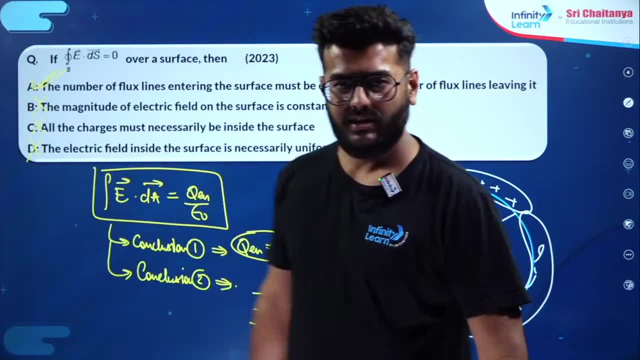 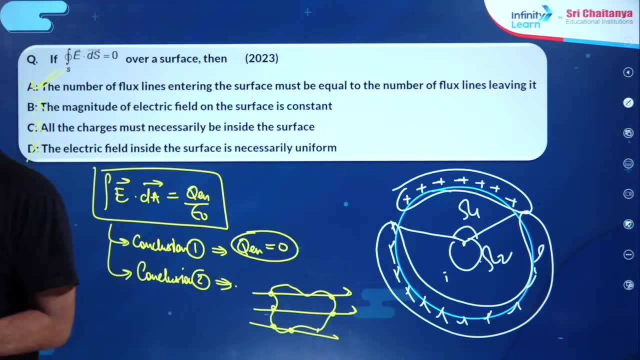 but this logic is very good in non conducting. the thing with conducting is, in conducting you have a compulsion to zero the electric field, because if you don't do it, if you don't do it, then don't do it. if you don't do it, then don't do it. 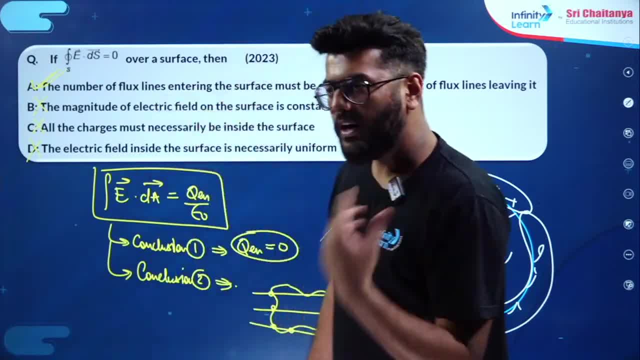 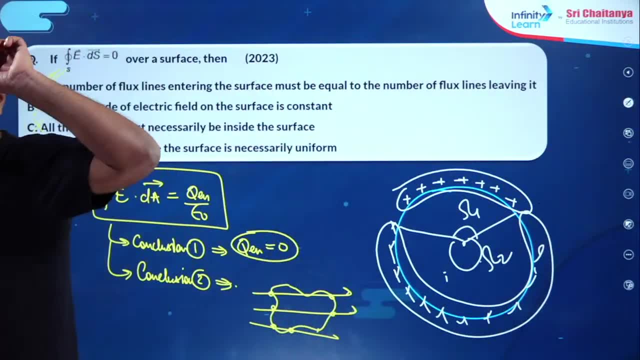 but at the same time the charge will say: ok, electric field is there, let's orient ourselves. and it will keep orienting itself like this until the net electric field is zeroed out. so when you see the word conducting, then the utmost requirement will be to zero the electric field. 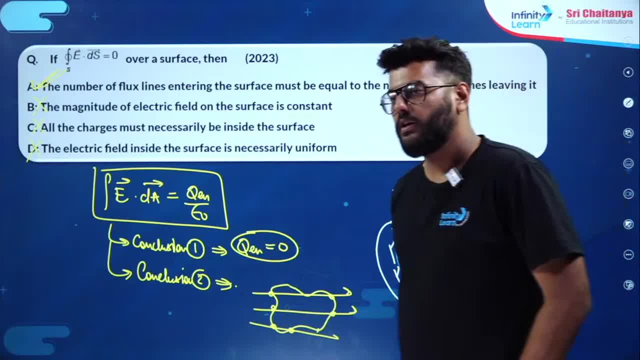 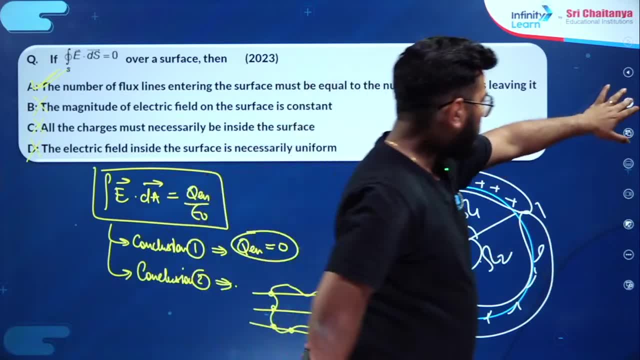 that will be your pre-assumptive fact that the electric field will be zeroed out. if I talk about non conducting, then in non conducting, if there is equatable or symmetric distribution, then with the concept of solid angle you can tell that the net electric field will be zeroed out. 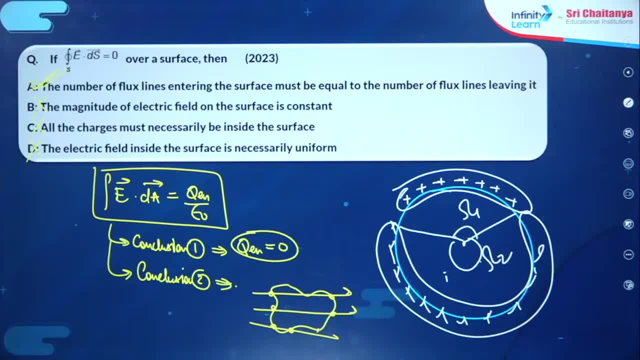 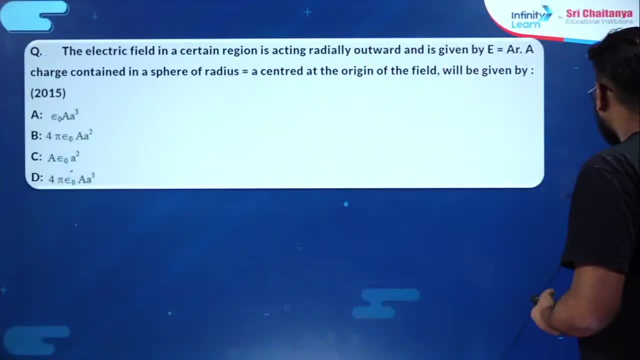 inside any point that will vary on solid angle, on non conducting. I hope you understood this. let's look at this question: electric field. electric field in a certain region is acting radially outward and is given by. E is equal to AR, a charge contained in sphere of radius small a. 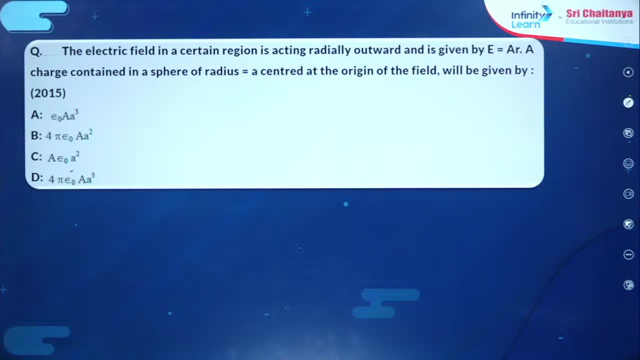 centered at the origin of field will be given by. here charge contained in a sphere of radius small a centered at the origin of the field will be given by. simple logic is: integration of E dot DA is equal to Q enclosed upon epsilon naught. we have to use this. 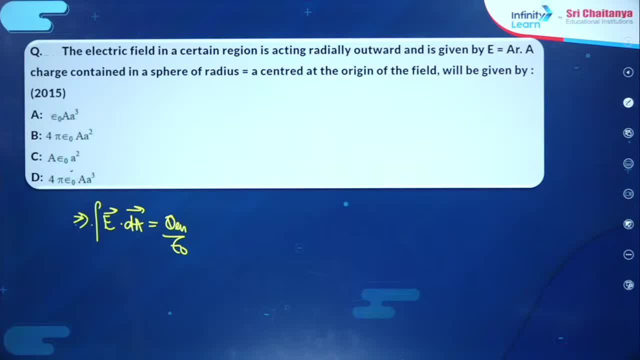 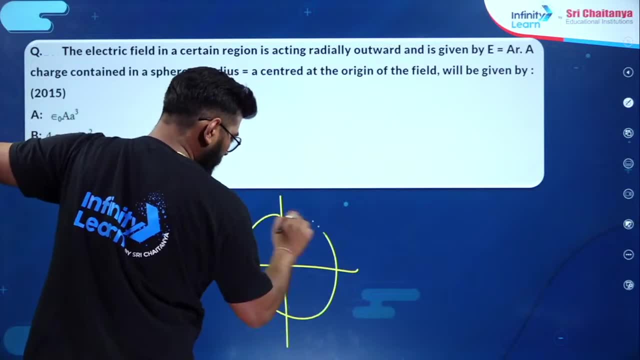 electric field is given as A into R and charge contained in a sphere of radius small a and charge contained in a sphere of radius small a and charge contained in a sphere of radius small a centered at the origin. so origin is this and in origin a sphere is existing. 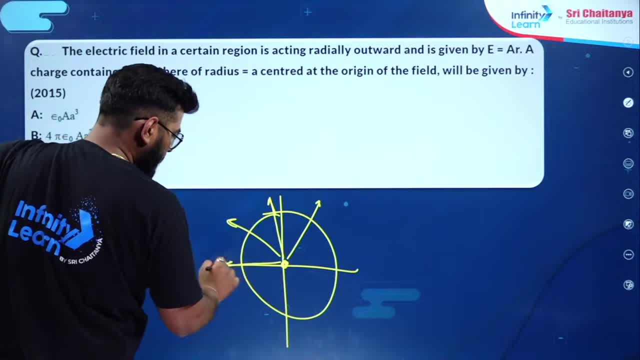 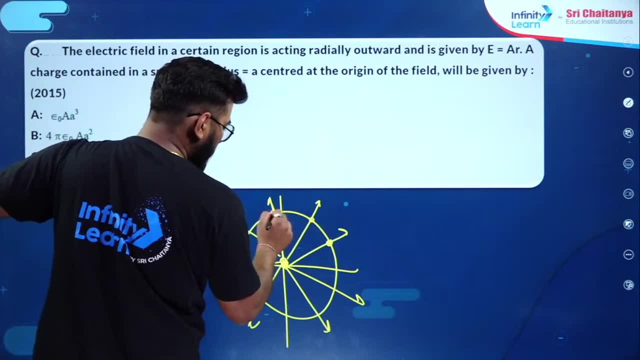 and the electric field line is going in this way: AR, which is R here, distance from the center. so every point which is coming on the surface, the magnitude of electric field which will come at every point, how much will it come? the magnitude will come equal to capital A into small a. 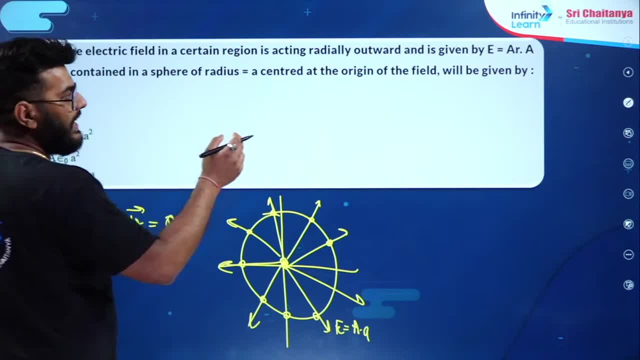 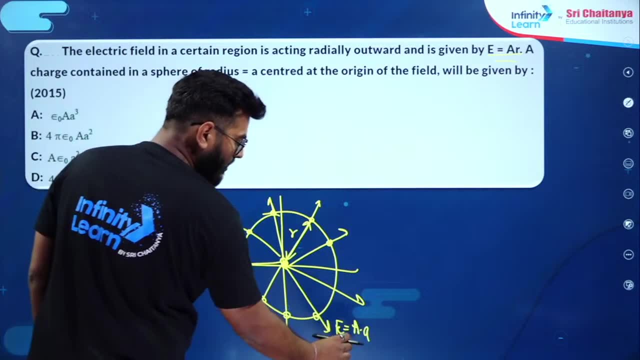 capital A into small a. is it clear? because A into R is given here. R is the distance. this is your R, this is your R, this is your R, this is the distance, R. so the value of R will be equal to A. this is my electric field line. 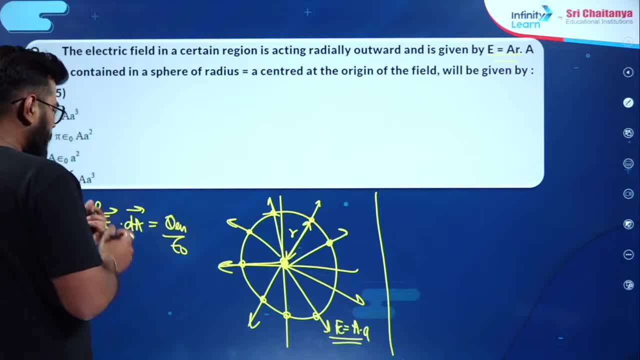 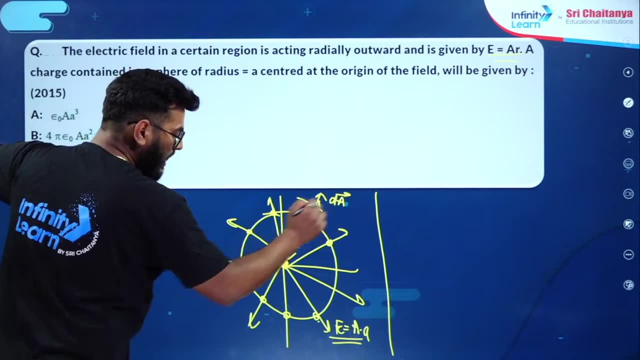 now, if this electric field line is done, then integration, its magnitude is fixed, its magnitude is fixed and everywhere you can see the DA vector which is happening, its perpendicular is coming parallel. this DA vector is also parallel here. the DA vector of the sphere will come here. so here also the electric field line. 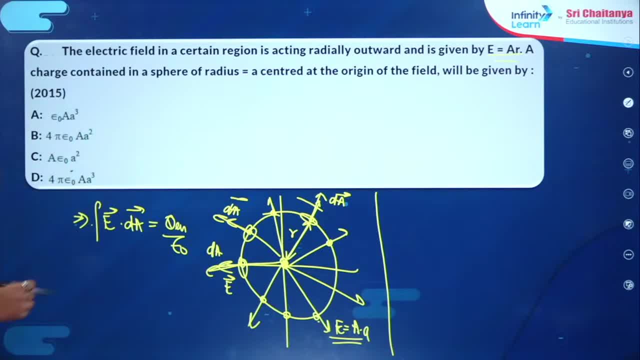 is coming parallel because E is coming parallel. so here dot product can be done and the electric field will come out because the magnitude is constant. A into small a is equal to, and the integration of DA will be. total surface area, that is 4 pi A square. 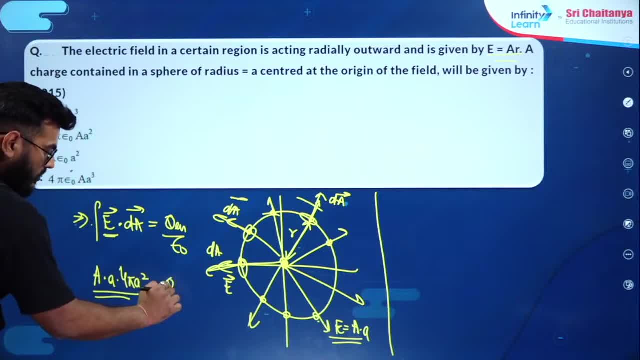 here. your integration is E dot DA and this will be Q enclosed upon epsilon knot. take the epsilon knot here and the value of Q enclosed will come. how much is coming? Q enclosed will come 4 pi, 4 pi. epsilon knot, capital A into small a square. 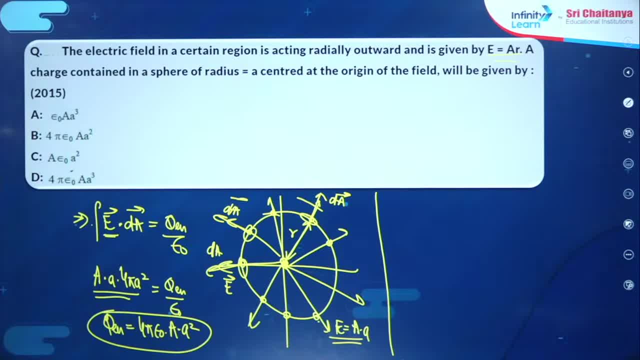 correct answer is your option number B. option number sorry, sorry, D, D. why D? it is cube, cube, A square and A cube. option number D is absolutely correct. option number D is absolutely correct. Apoor is absolutely correct. you said it right, very right, Siddharth Chandraji. 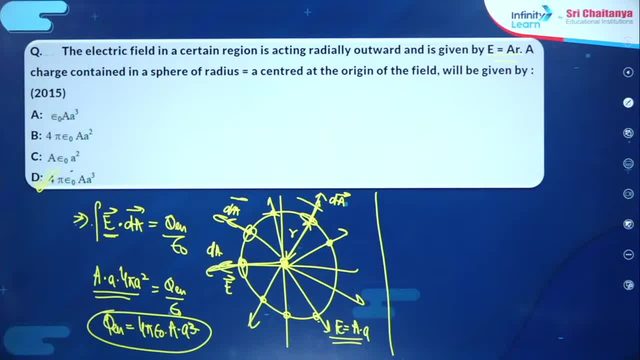 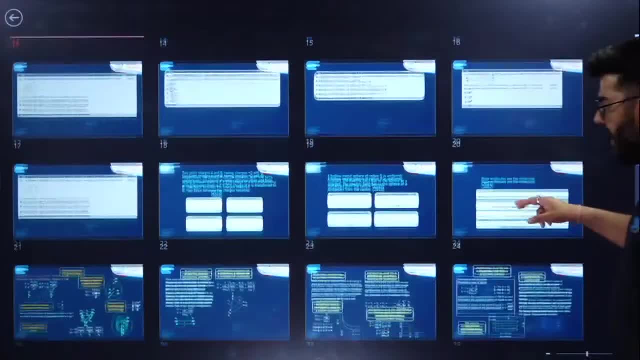 very good, Abhishek, nice. option number D is absolutely correct answer. ok, so there is some question and answer related to electric flux and dipole in front of you. now let's move forward and let's go to the next concept, which is electric flux and dipole. 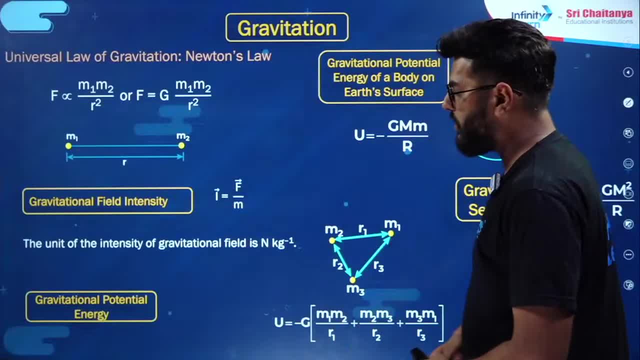 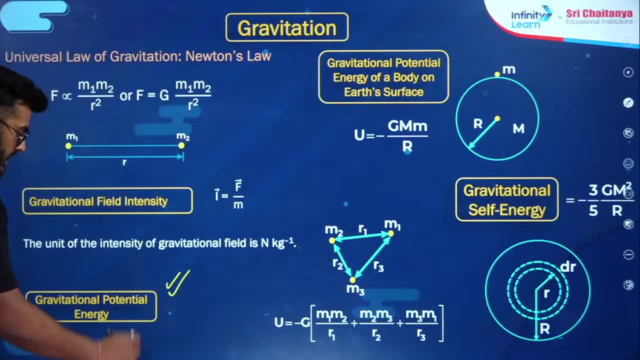 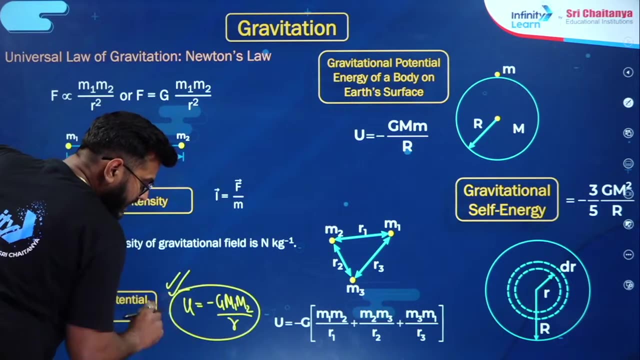 electrostatic potential energy and first of all, let's see the concept of gravitational potential energy and potential. so if I talk about potential energy between two masses, you always have to remember this is the difference. when I talk about gravitational potential energy, there comes one negative sign. this negative sign is the key differentiator. 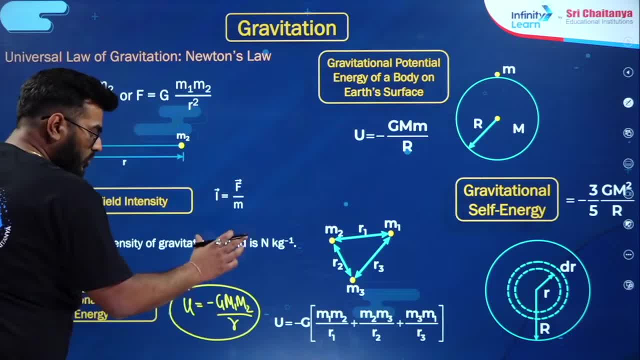 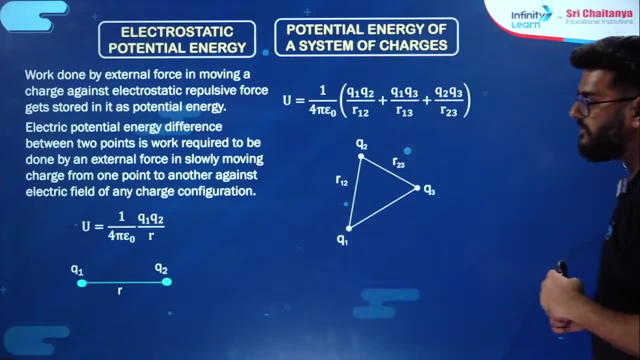 in gravitational potential energy, 0 is considered and two masses are at distance, so negative comes in them. on the contrary, if I talk about electrostatic potential energy, then there is no negative sign. It is simply KQ1, Q2 by R, And assumption is same When there are charges at infinite distance. 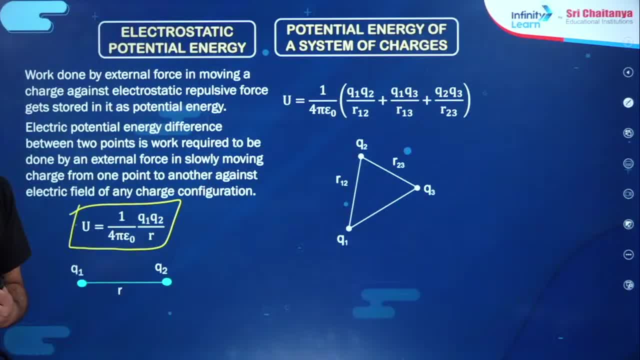 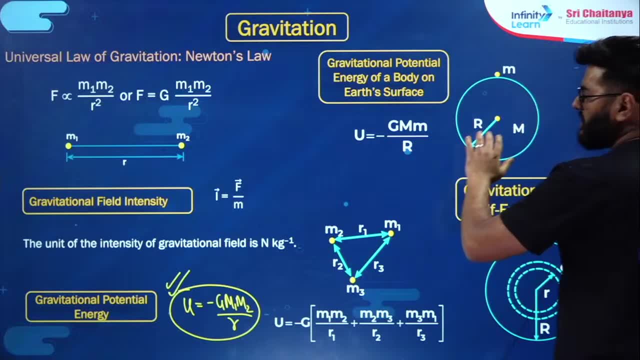 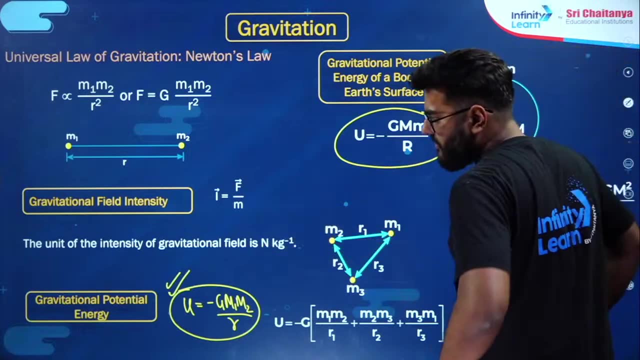 Then electric field value will be equal to zero. Clear, Ok, Then next thing I will talk about Gravitational potential energy If a body is placed on surface of earth. So see, All these concepts are valid for your point masses And if point mass is not there. 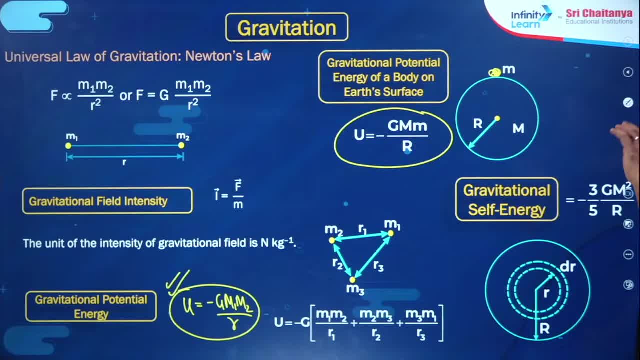 If point mass is not there, Then you have to take concept of center of mass Or center of charge, Like in this case. Here you can assume the entire sphere That it is about center of mass. This center is about assumed Means. here one mass is M And here capital M is mass. 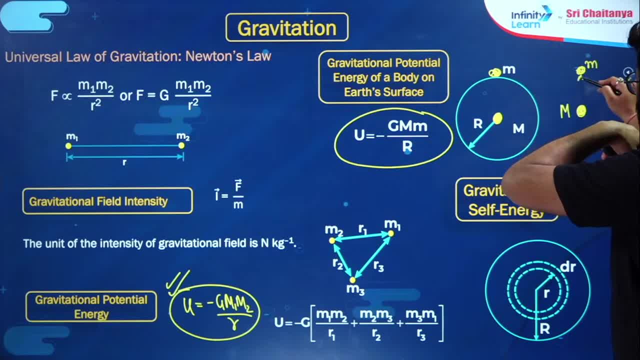 Here, one mass is capital M, Ok, And the gap between these two is R. So now the gravitational potential energy between these two Will be G, capital M, small m upon R. This will be very useful. What is it called? To find out the concept of escape velocity, The gravitational potential energy. 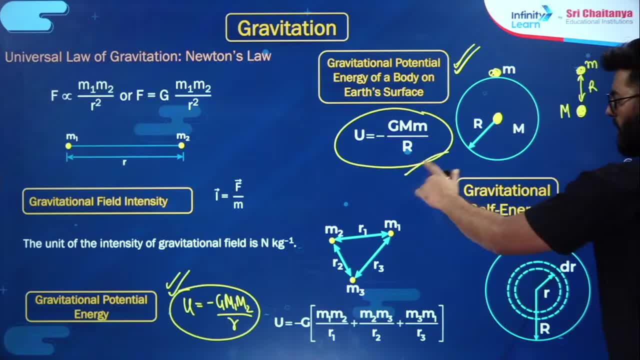 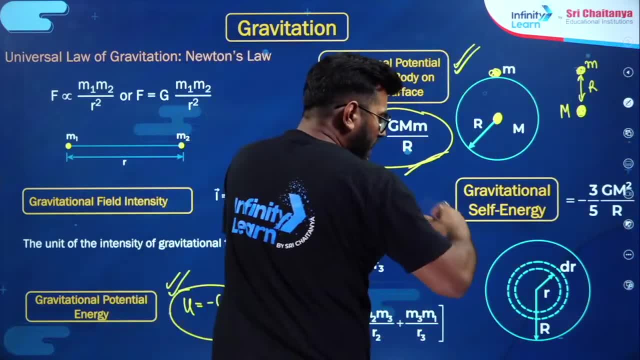 When any object is placed on the surface of any planet, Then it remains equal to this. Ok, What is the concept of gravitational self energy? Such an electrostatic self energy is also there That there is a body of mass M. There is a body of mass M, So it will have its own energy. 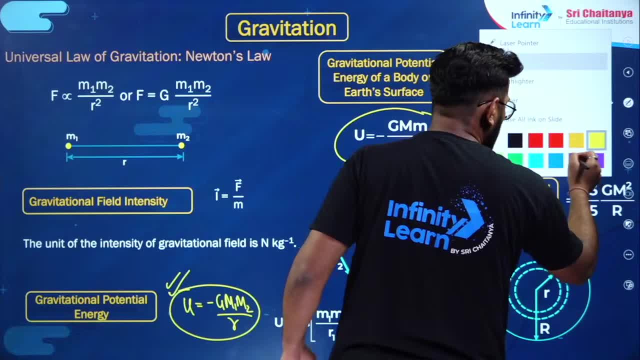 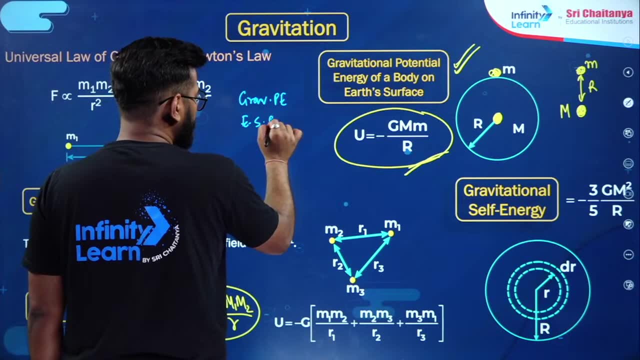 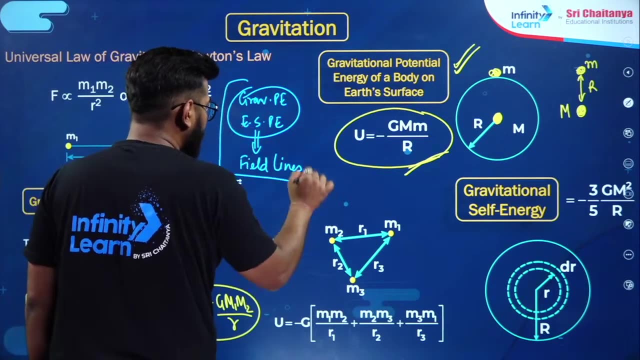 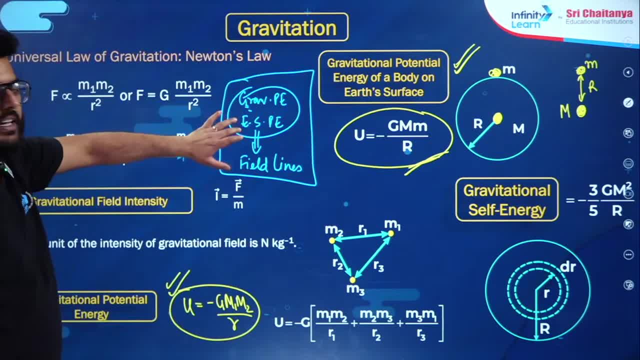 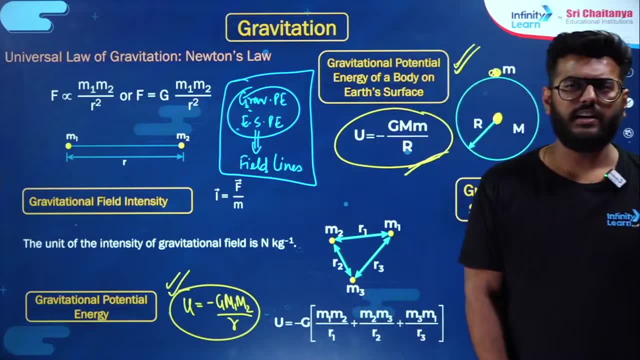 So surely you can say that there will be some gravitational potential energy Or electrostatic potential energy. If there are field lines, Gravitational field lines and electrostatic field lines, Then there will be gravitational and electrostatic potential energy. There is a house, Field lines are houses. 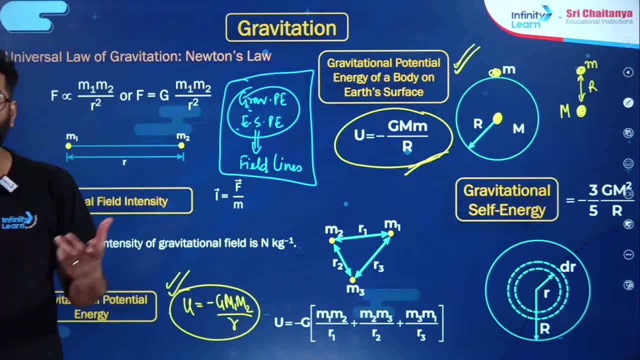 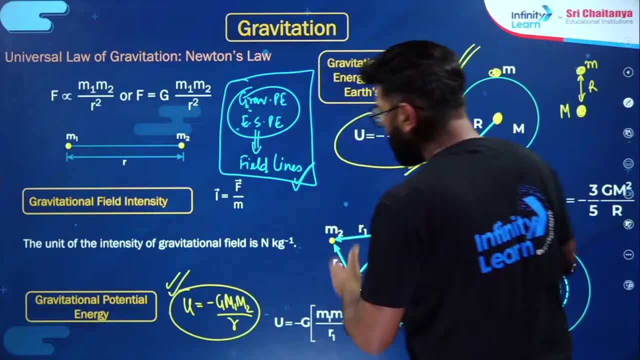 Whose house is it? Field lines are houses of gravitational potential energy and electrostatic potential energy. Who is the house of potential energy, Sir, field lines? So that's why you should know that these are their houses. So if they will be there, then they will be there. 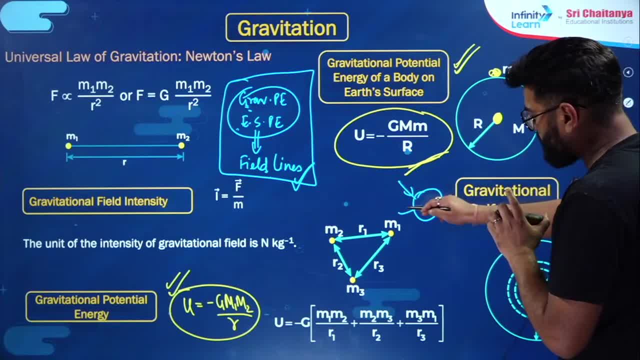 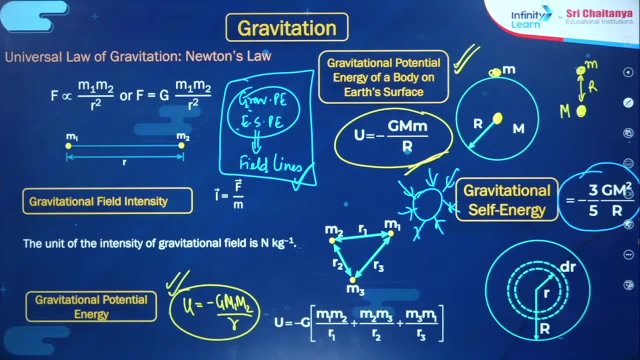 So let's assume that a single mass is made. This is a single mass, So how much self-energy will it have? It will have self-energy. Remember the direct figure Minus 3 by 5, gm square upon r. 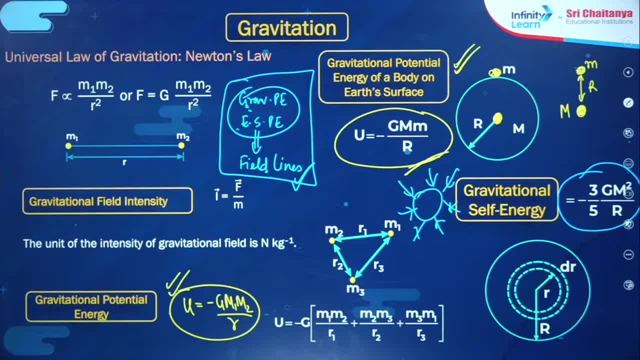 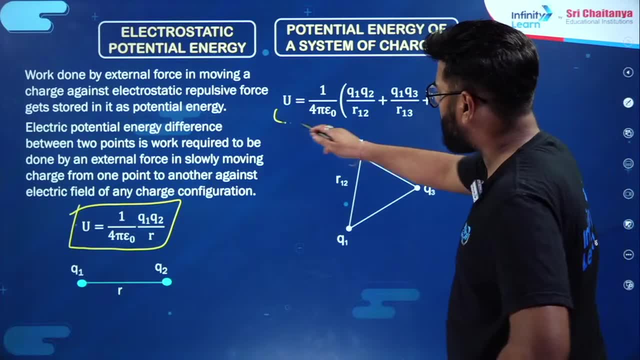 Minus 3 by 5 gm, square upon r. Remember the direct value. Let's move ahead from gravitational potential energy to electrostatic potential energy. So you can see the same concept, Just a negative sign has been removed from here. There are a bunch of charges, So their individual will be this: 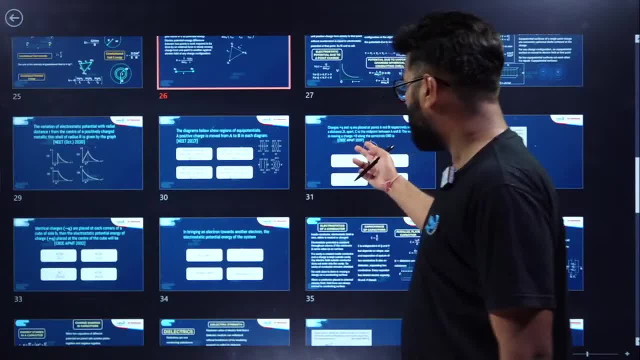 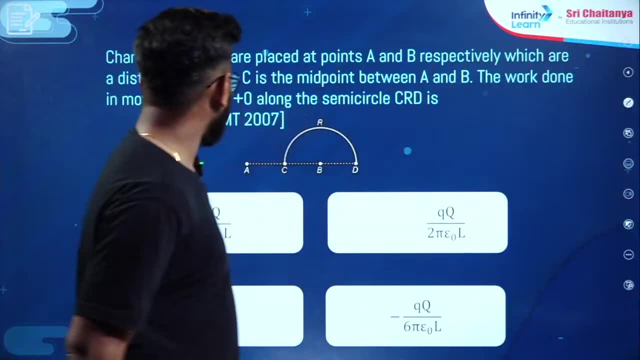 Now look at some questions related to this. Look at this First question: Charges plus Q and minus Q are placed at points A and B respectively, Which are at a distance 2L apart. These are two distances, 2L apart. 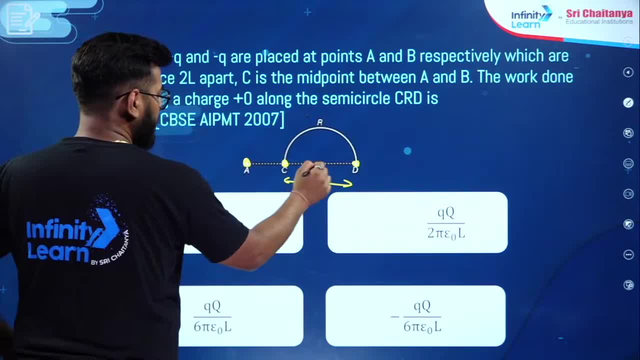 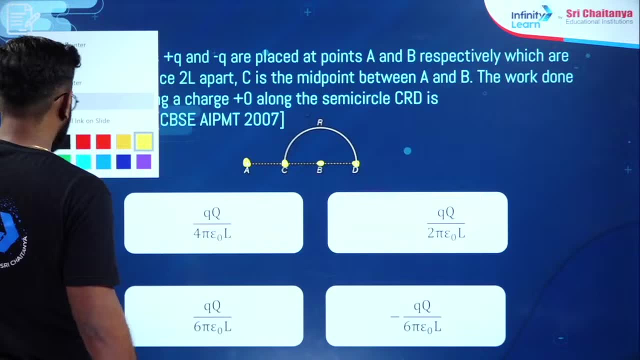 Okay, Okay, one minute. A and B remain here. A and B remain here And this distance is 2L. This distance is 2L. This is not This distance. This distance is 2L. This distance is 2L. 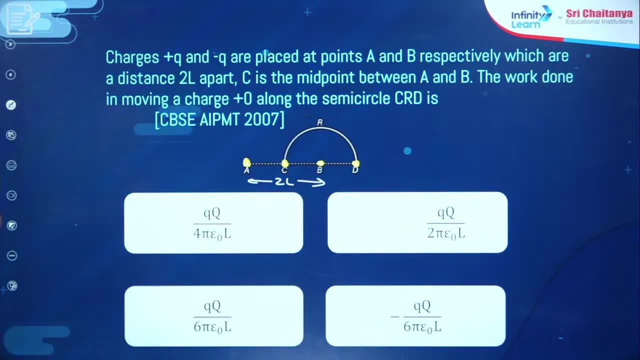 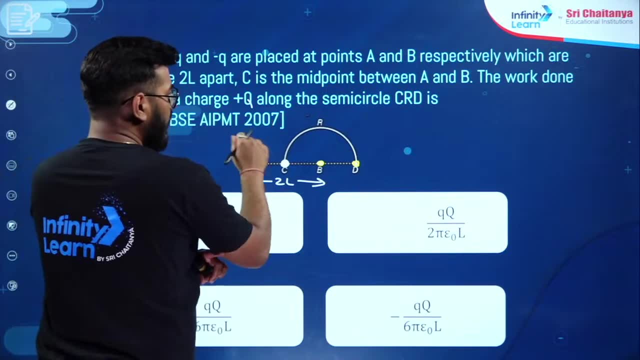 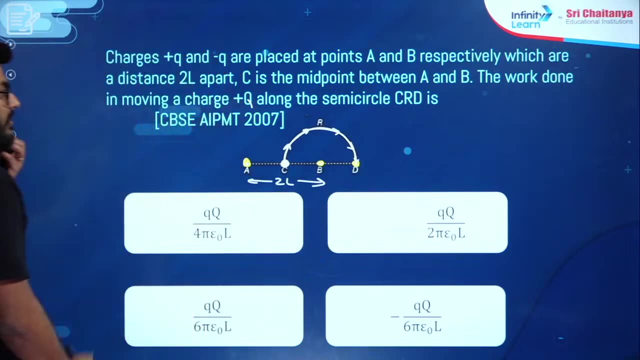 Okay, C is the midpoint between A and B. This is the midpoint of A and B, The work done in moving a charge plus Q along the semicircle CRD. You have to move the charge along this, So how much work will be done? 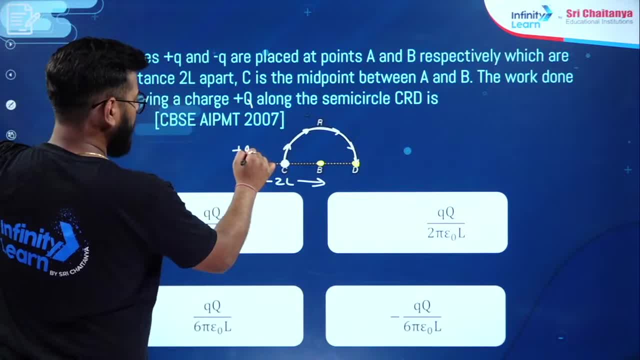 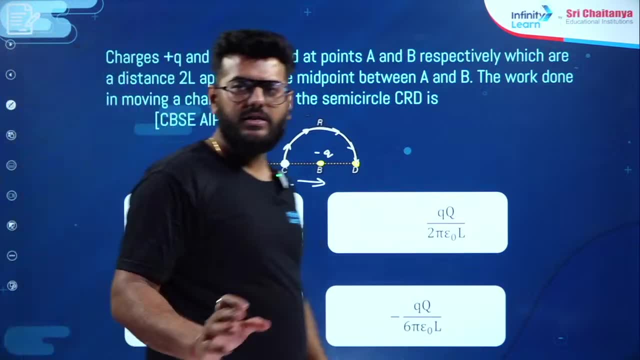 It is a simple point Here: which ones are placed Here? plus Q charge is placed Here, minus Q charge is placed. Okay, So we have to move C point and D point. We have to find The Potential. But first thing is that we can do something. 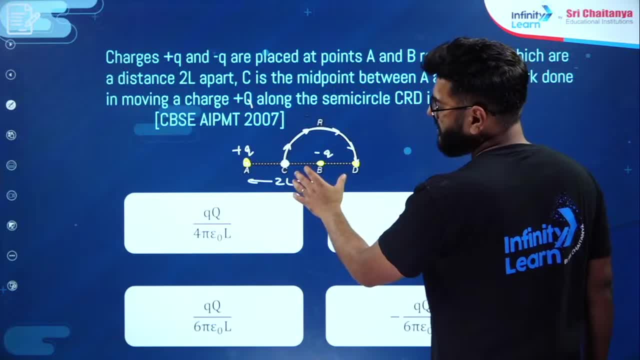 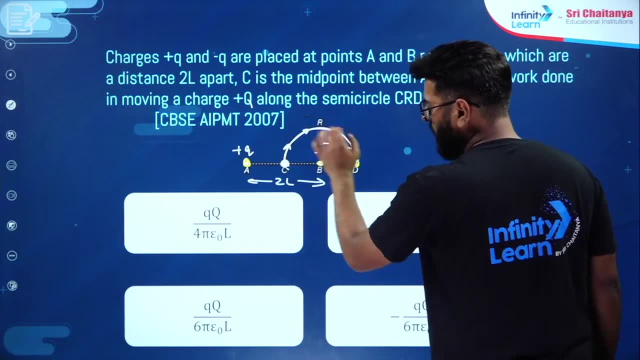 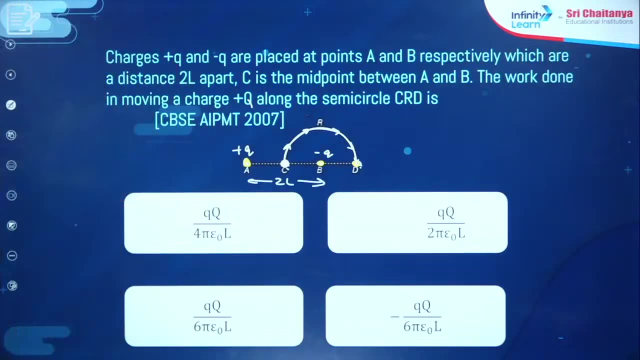 Either we can find potential or second one. we'll see that the potentional energy of the pieces placed in this state during se делают on C and the potential will increase with D, from both aspects. we will know the answer And always remember one thing. 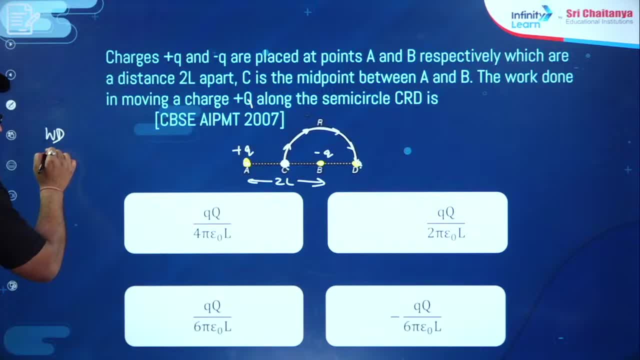 Work done is work done. in any case, it is done is done through external agents. it will always be equal to Delta U Yong, which will be equal to delta u, which means potential energy in final state minus potential energy in initial state, so potential energy in final state. 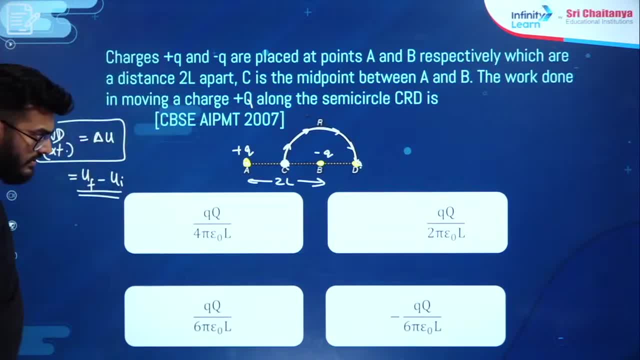 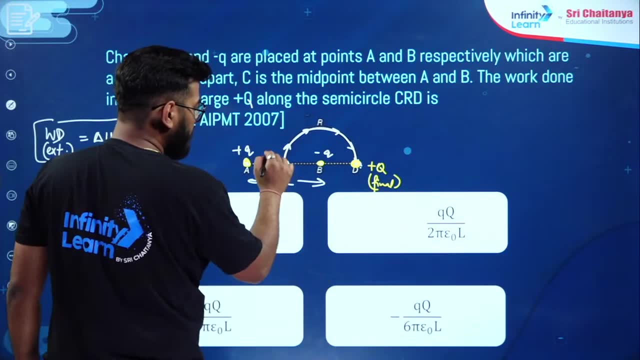 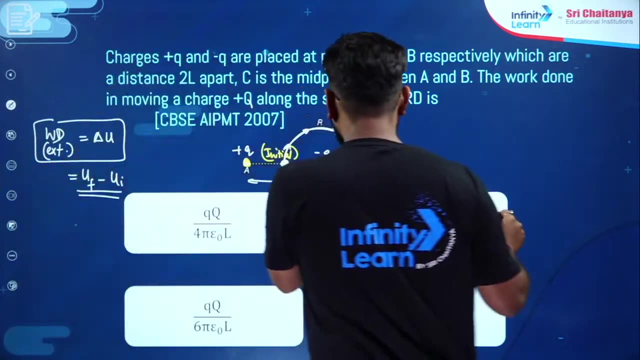 how much is happening. let's find out. in final state, charge plus q is kept here. this is final state and in initial state it was here. this was my initial state. so in final state the potential energy will be k capital q into minus small q, upon the distance between the two. 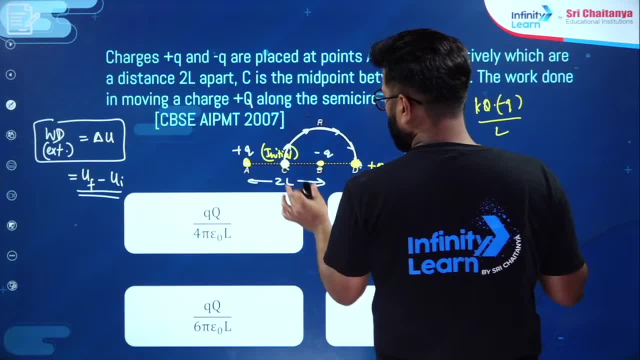 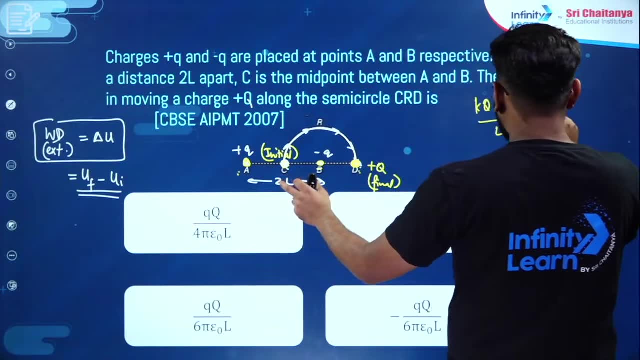 the distance between the two is l, because this is l and this is l. it is kept at midpoint, so it will be l and with this, how much will happen between the two? plus k, capital q, small q upon this distance? 3l. this is u final. 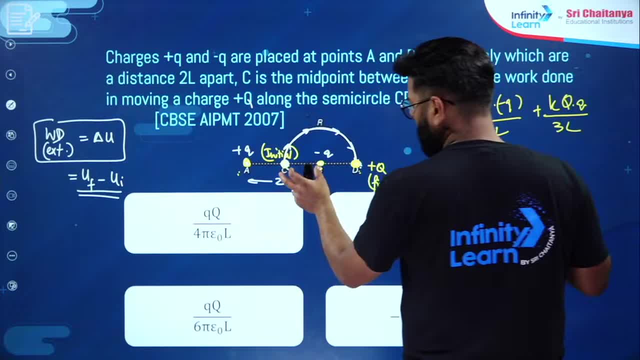 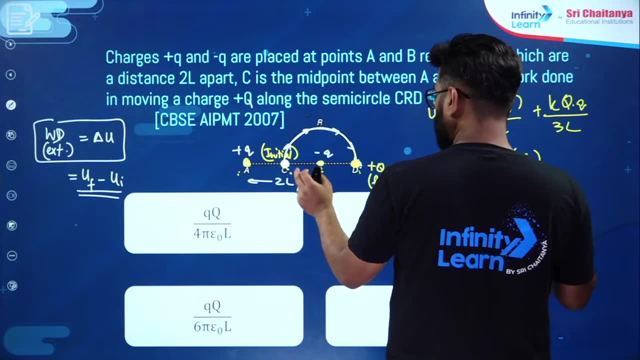 how much will be u initial when it is kept here. so in that case, k capital q minus q upon the distance which is l, kept here in initial state, and between the two it will be l, and between the two k capital q small q upon the distance which is l. 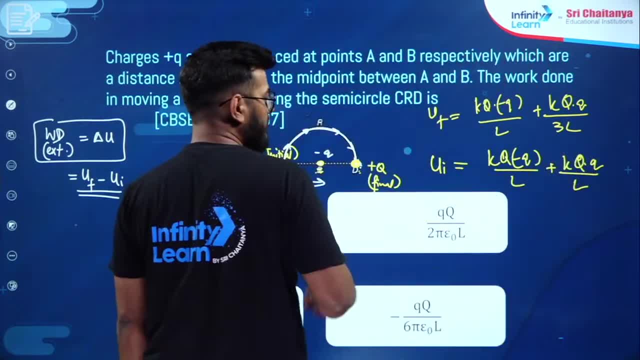 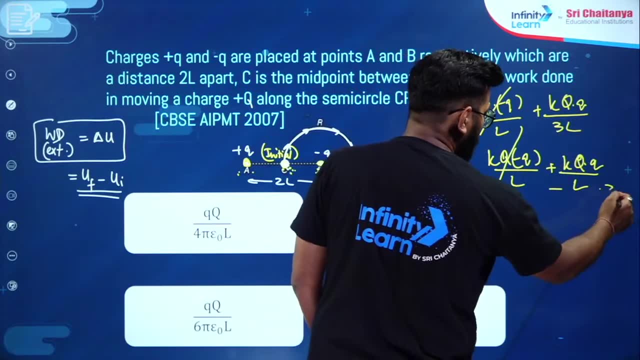 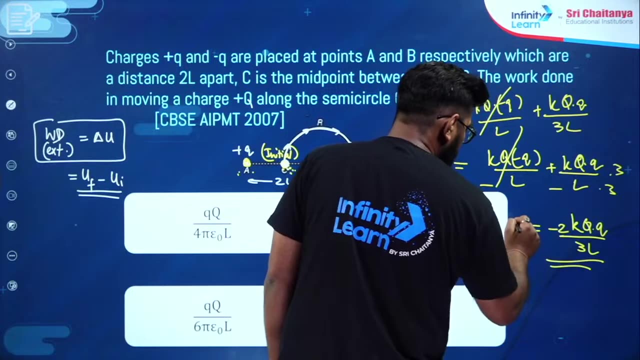 you have to minus both of them: u final minus u initial. you will minus this. this will be cancelled. and k capital q small q upon 3l minus 3 and 3. multiply it minus 2k capital q small q upon 3l. this is my answer. 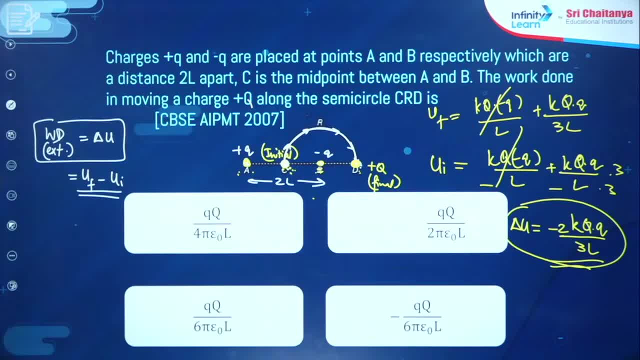 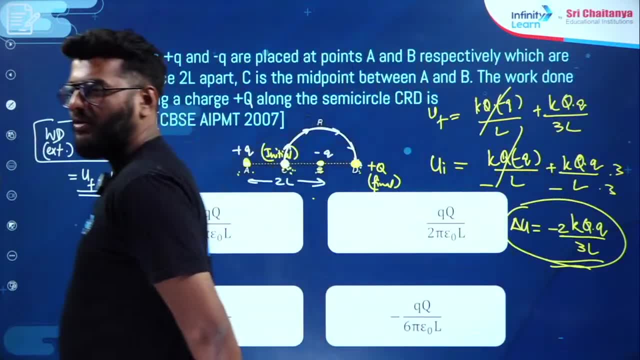 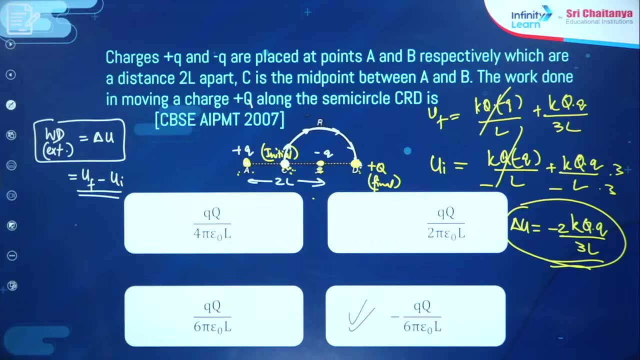 delta u and this will be my work done. so negative work done is coming. there is negative in only one option, so in only one option, absolutely correct, absolutely correct. option number d is correct answer: minus small q capital q upon 6pi epsilon. and if you solve this, 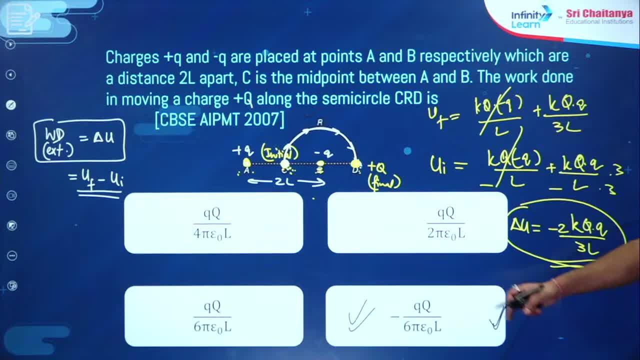 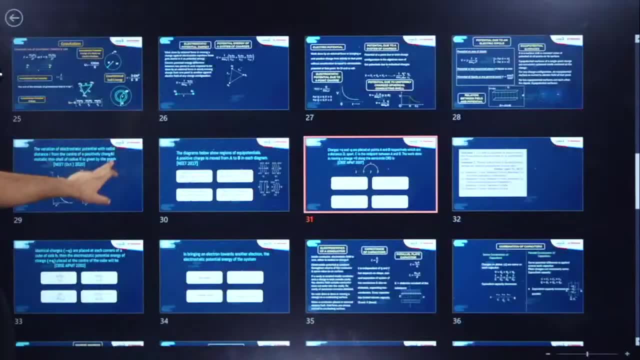 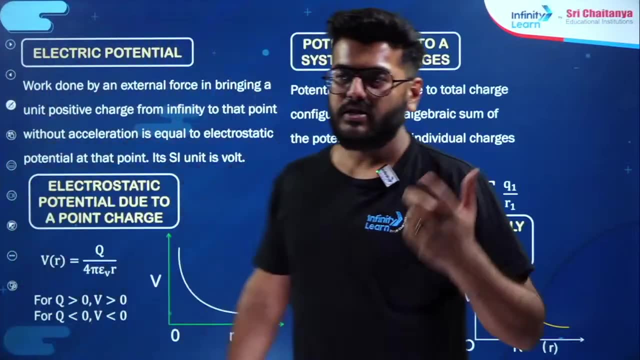 this will be the answer. this will be the answer. in only one option, negative will be same. in only one option, negative will be same. ok, you can solve this with help of potential. how you can solve this with potential. first, gravitational potential is not there. you can solve this with electrostatic potential. 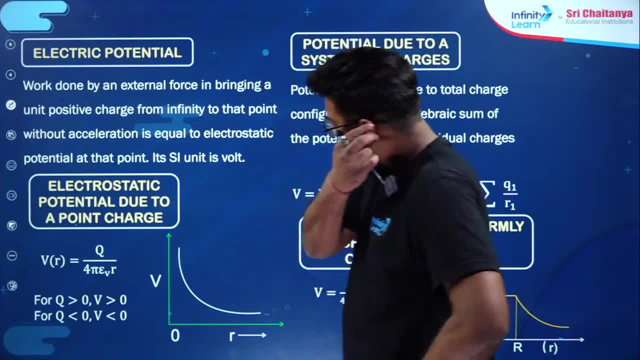 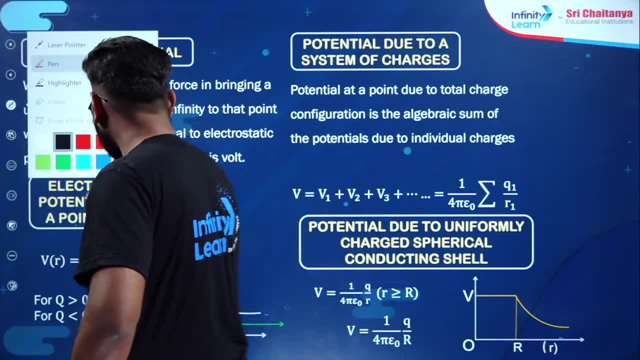 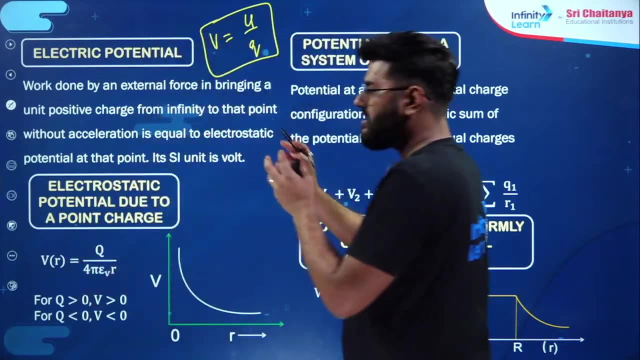 if i talk about electrostatic potential. so because of one charge, what is the potential in its nearby region? because of one charge, what is the potential in its nearby region? it becomes simple: whatever potential energy divided by the charge q. this test charge because of one particular massive charge, capital q. 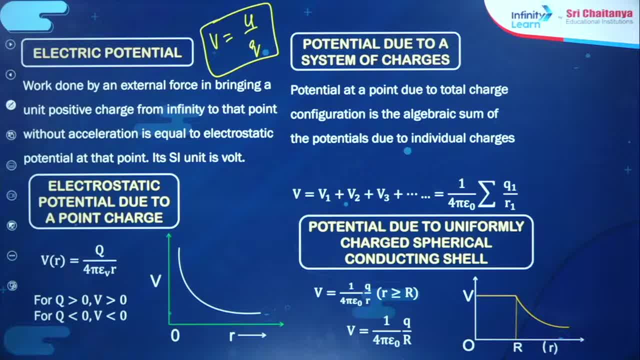 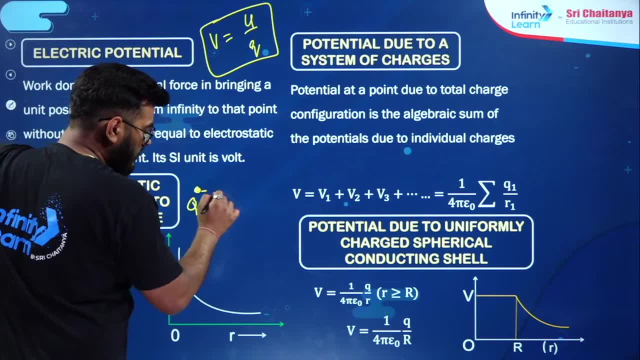 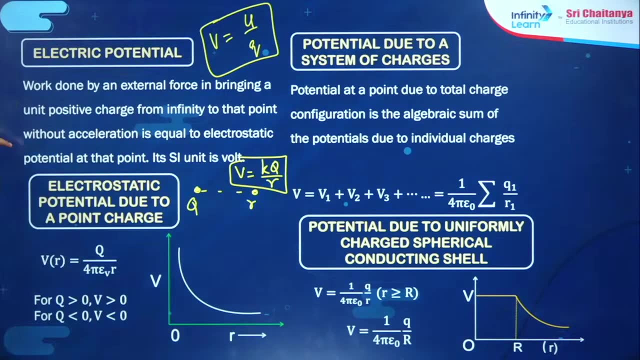 the potential in the nearby region. it becomes u divided by q. so according to this, there is a massive charge capital q about the distance r, the potential that is going to be k capital q upon small r. this is electrostatic potential. if i talk about gravitational potential, 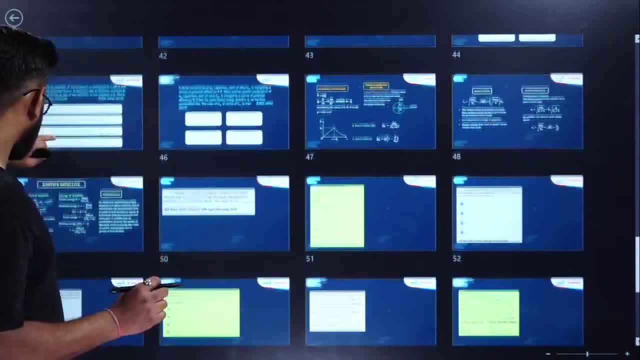 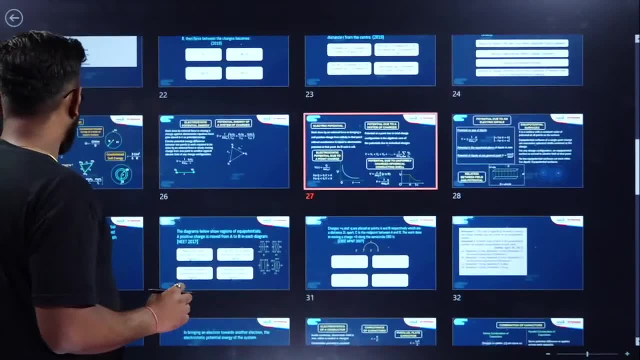 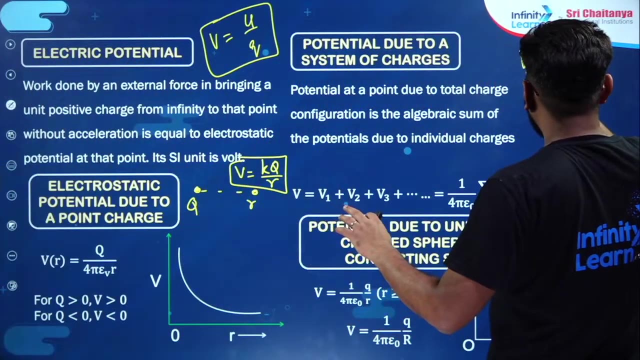 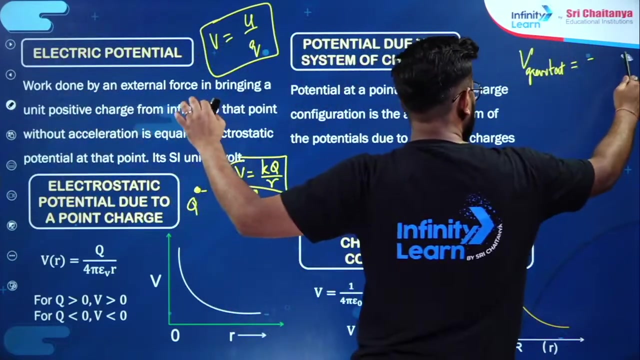 there is only one difference of negative charge. which difference is there, sir? negative charge gravitational potential has the difference of negative charge gravitational potential. if i give gravitational potential instead of this, i will give gravitational potential, then it will be minus of k times capital m, not k minus of g times capital m. 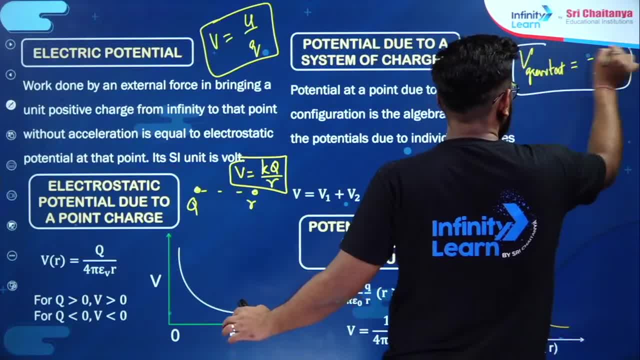 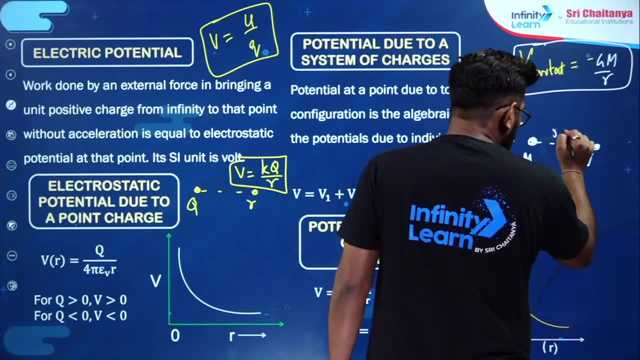 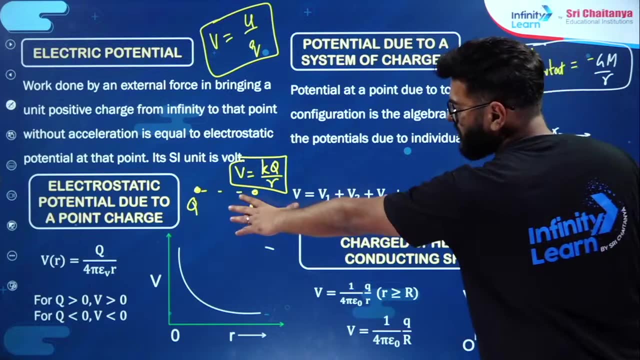 upon small r minus of g times capital m upon small r. please. i am requesting again and again- that is why i have brought this in your mind- to be able to relate this thing. relation is more important. relation is important. these things can happen. you all know it. 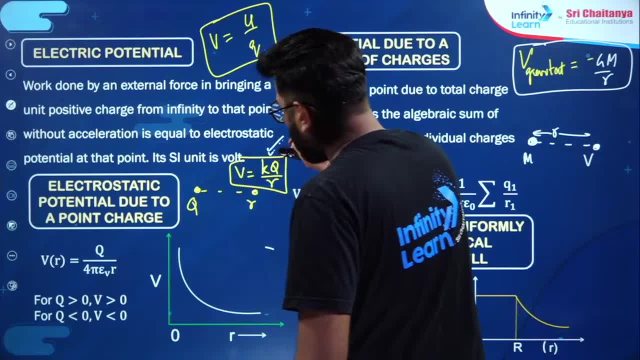 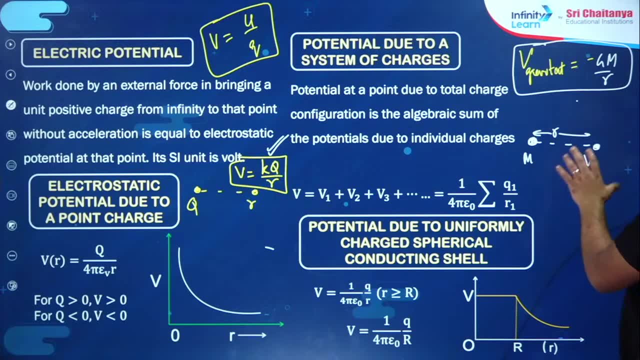 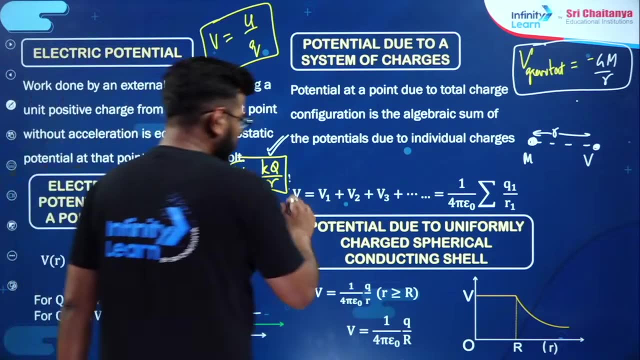 you must be knowing all these formula sets that what is electrostatic potential? because of one charge there is this type of variance. but how can you understand gravitation with this? i am telling you that i only understood that i did not do much effort. the net potential. 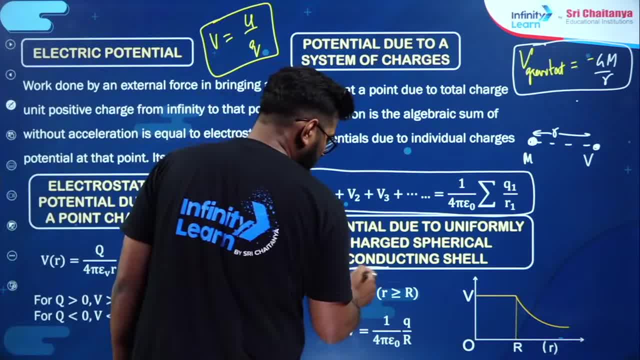 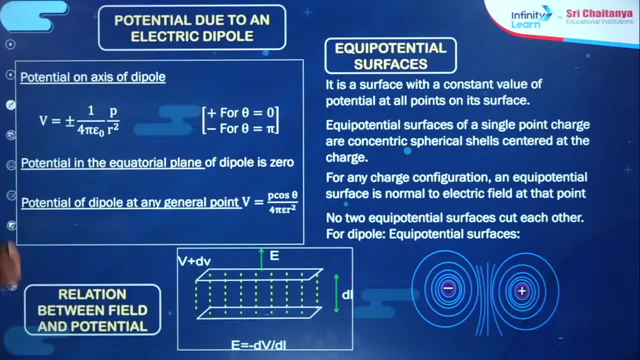 scalar quantity, algebraic sum. because of uniformly charged spherical conducting shell, inside it remains constant and outside it varies with r potential and electric field. as you see, i told about dipole. how is the potential? if you talk about axial point kp upon r square, it will be at axial point. 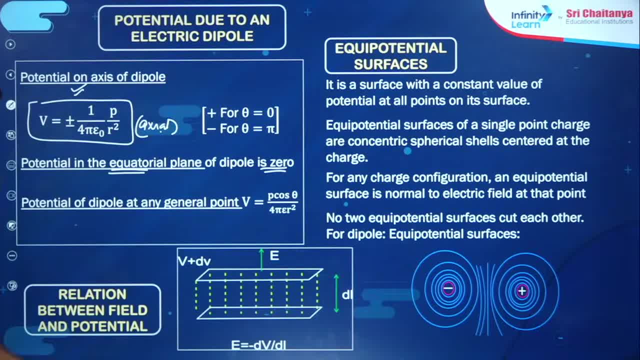 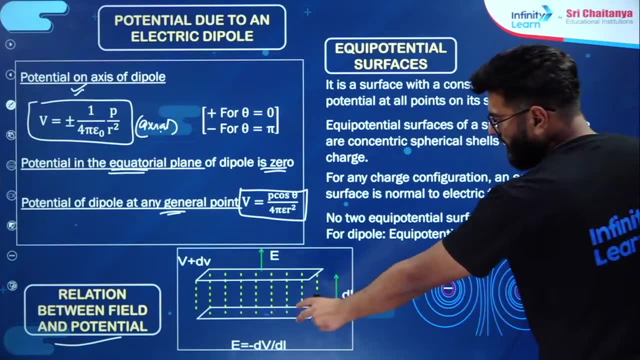 if you talk about equatorial point, it will be at zero. there electric potential is equal to zero potential. dipole any general point, kp, cos, theta upon r square. all these formulas are given relation between field and potential, which is equi-potential surface. relation between field and potential. 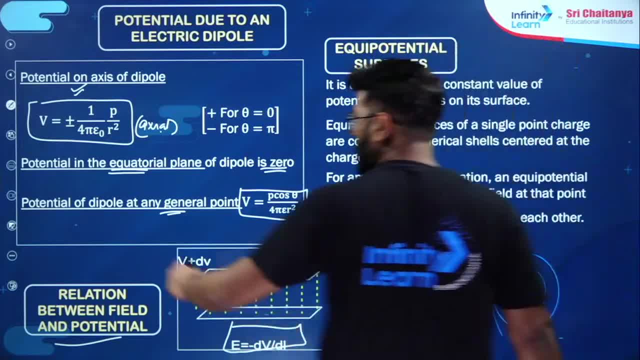 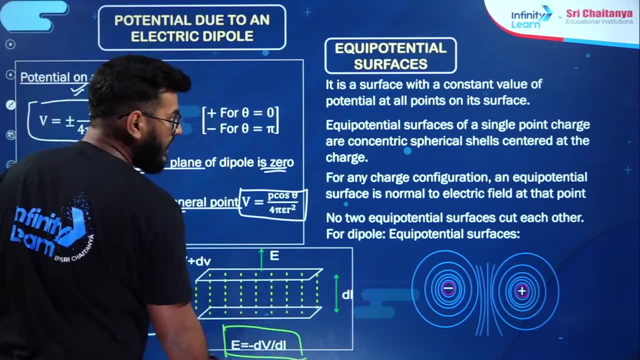 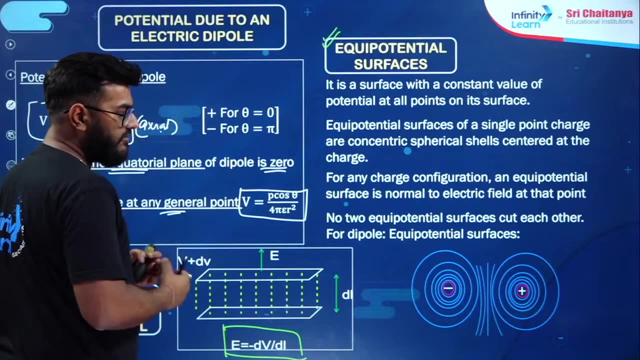 is minus of dv by dr. how much is it minus of dv by dr? minus of dv by dr. this is given dL by dr. this is how you get the concept of equi-potential surface. where there is no potential, the electric field becomes zero. 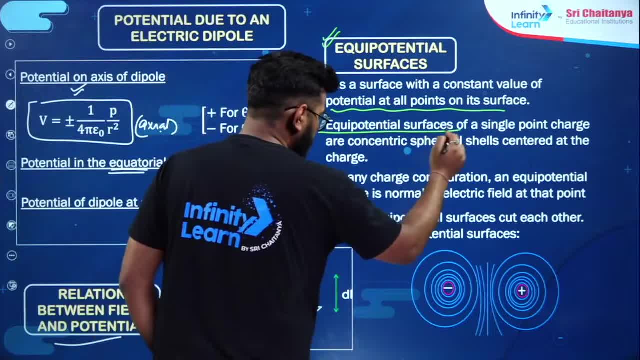 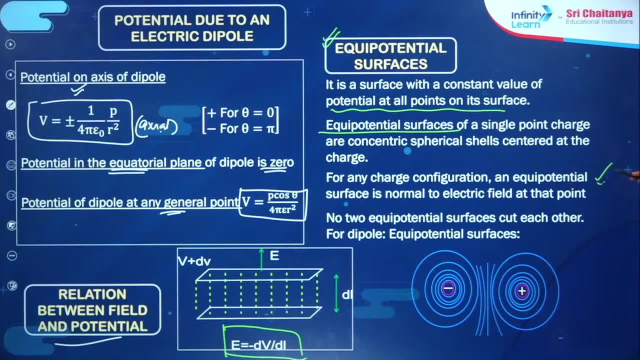 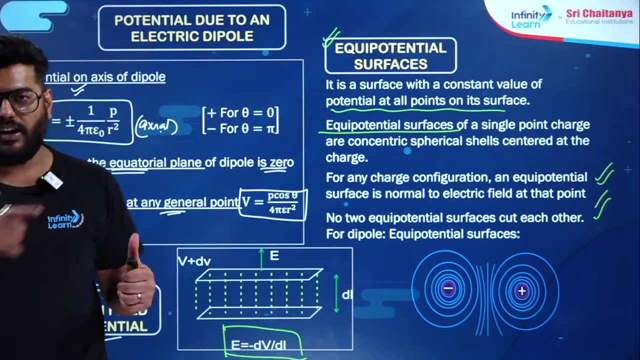 and the surface where the potential remains same at every point is equi-potential surface, always in perpendicular direction and they are all funded. a conductor is always equi-potential. equi-potential can be of three types: planar, which exists in parallel, electric field lines. 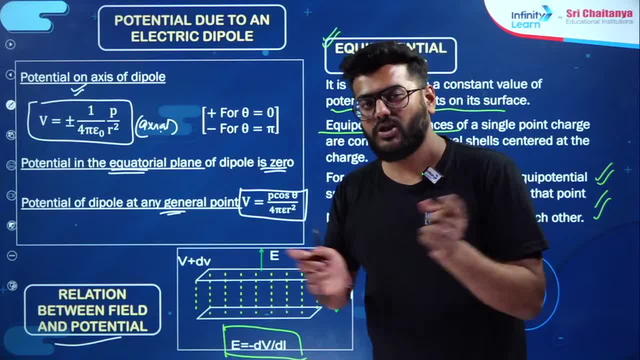 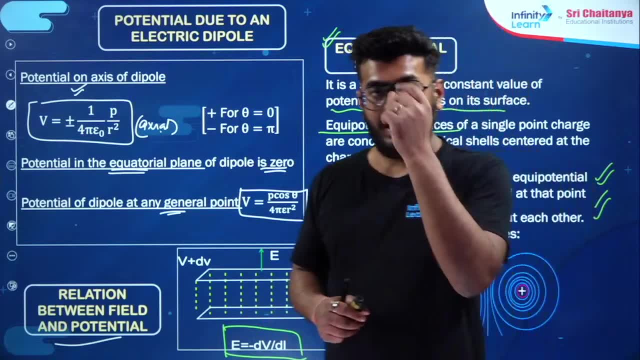 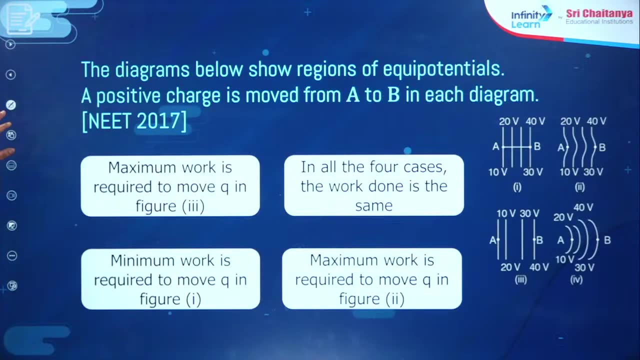 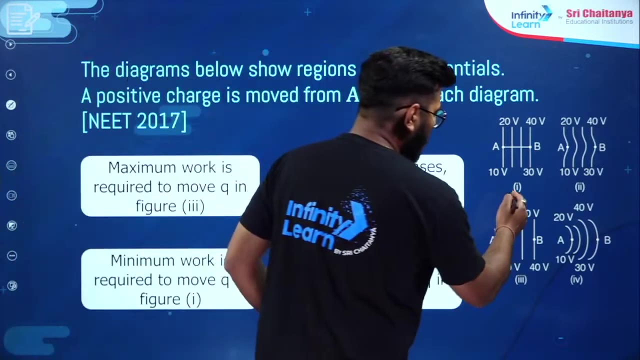 spherical which, because of a charge unit, charge externally. electric field lines are spherical, planar for sheet of charge and cylindrical for line charge. equi-potential surfaces: equi-potential surfaces are same, same potential objects. as you can see here you have four equi-potential surfaces. 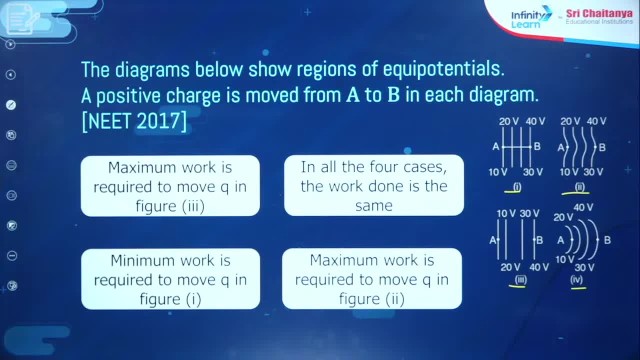 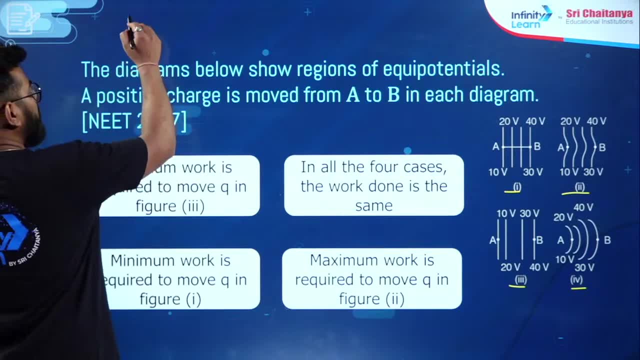 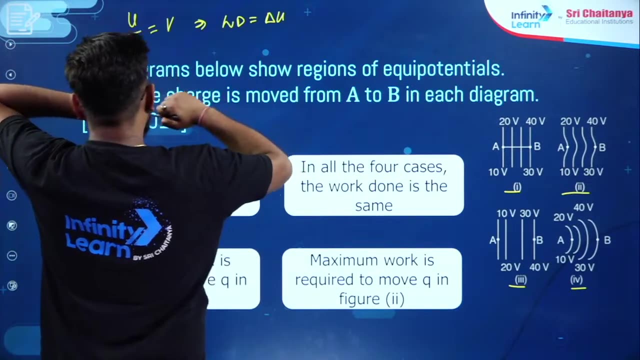 and the question is: the diagram shows below regions of equi-potential surfaces. a positive charge is moved from a to b in each diagram. remember, u by q is equal to v. done now what is my work done? delta u, u is equal to q into v. 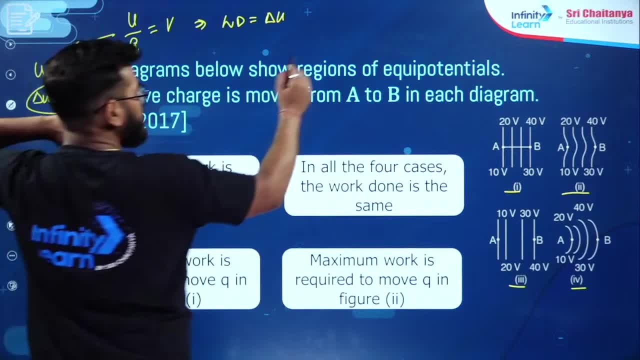 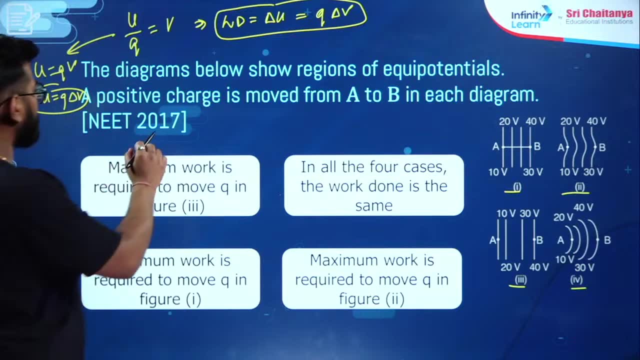 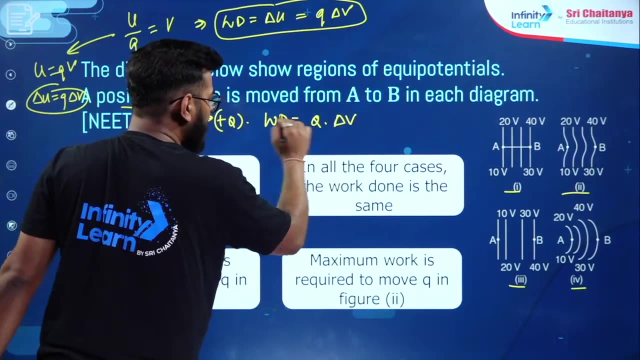 so delta u will be q into delta v. so whatever charge you are moving, whatever charge you are moving into delta v, that is going to be your work done. so here we have positive charge plus q, so work done will be q into delta v, wherever delta v will be maximum. 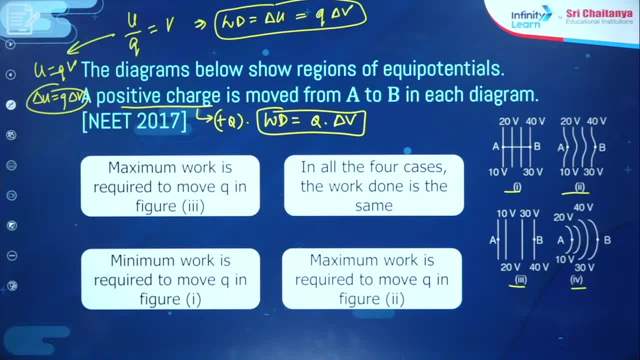 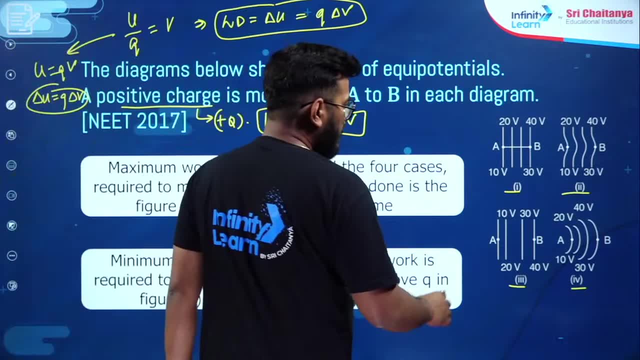 there will be maximum work done come. let's see same in all cases. maximum work is required to move q in figure 3. come on, sir. first 10, 20, 30, 40. second: 10, 20, 30, 40. 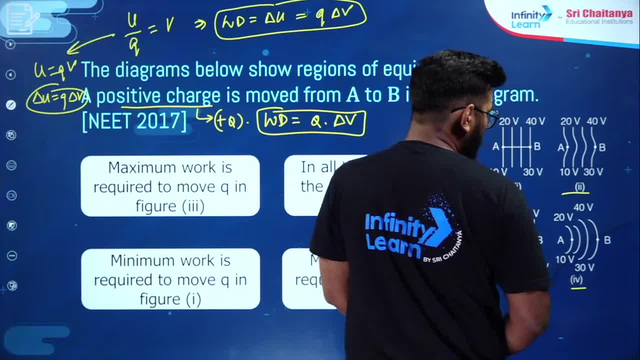 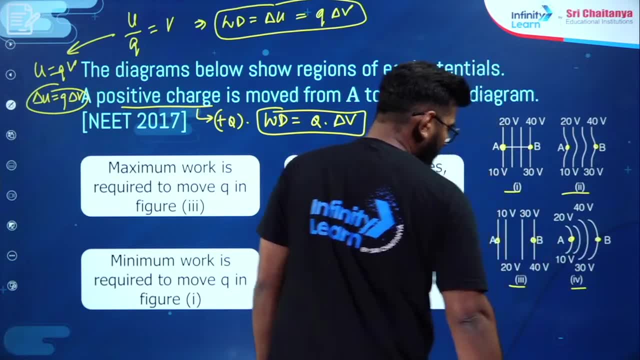 third: 10, 20,, 30, 40. fourth: 10, 20,, 30, 40. what is this? just the structure of equi-potential surfaces. final and initial potential are same, so there is no aspect of maximum work done. 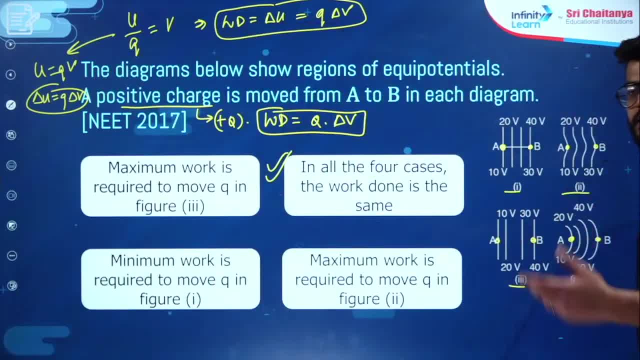 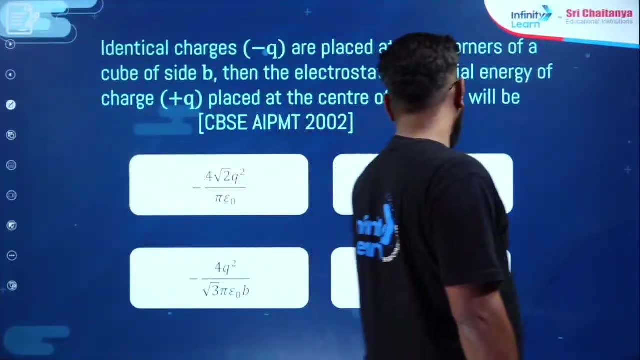 in all the four cases the work done will be same. simple concept: delta v: same, so same work done, absolutely correct. so this is your equi-potential surface p y q. ok, see, this is also a very good question. there is an identical charge minus q. 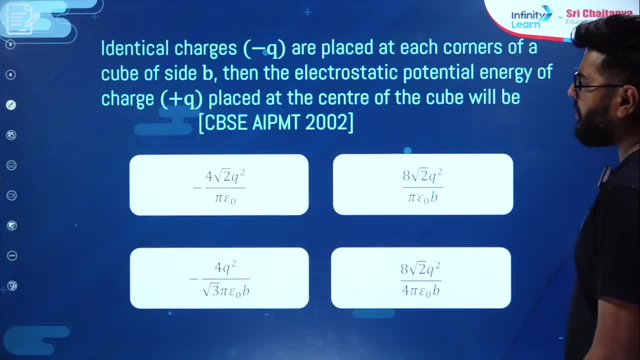 on the corners of the cube, then electrostatic potential energy of charge plus q placed at the center of cube is. I will give you one minute for this and I want you to try all this, everyone try those who are watching later in the session. please try this. 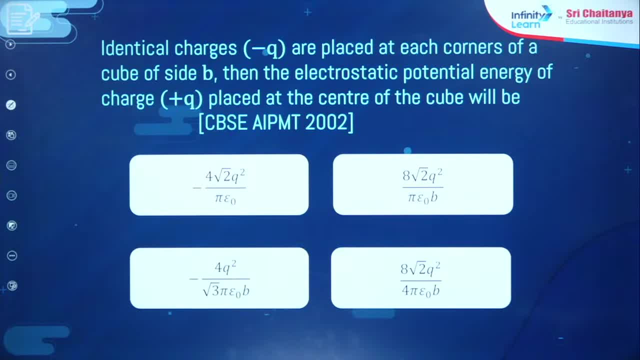 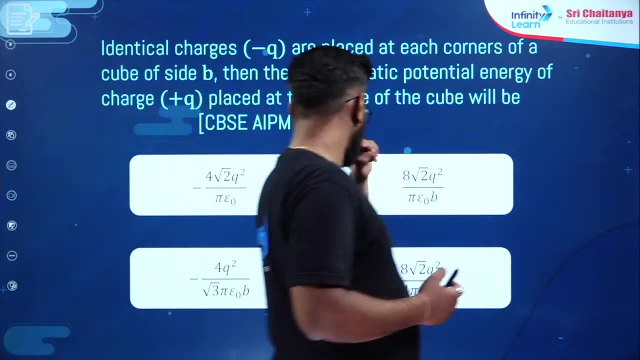 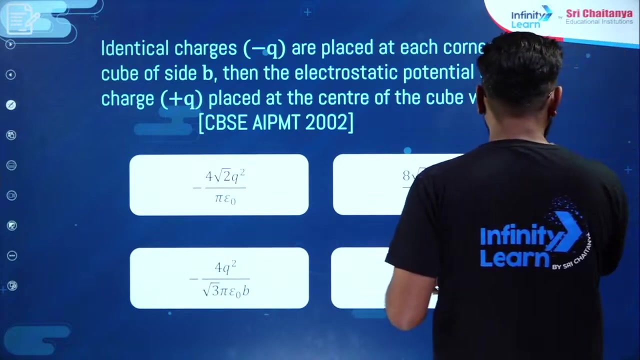 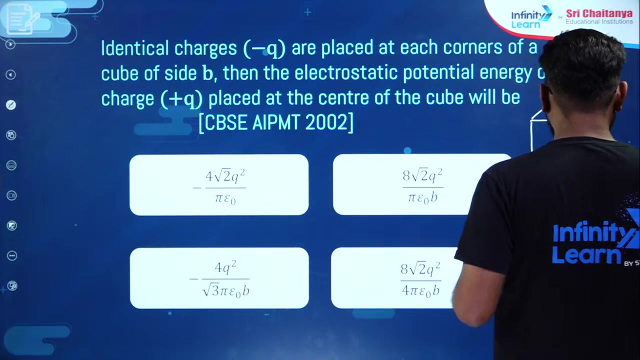 by pausing the video. what is this? option number b: what is this? or is it telling about the previous one? I want everyone to try this. this is a very good question. it is a nice question. we will discuss it later. ok, I will give you the answer. 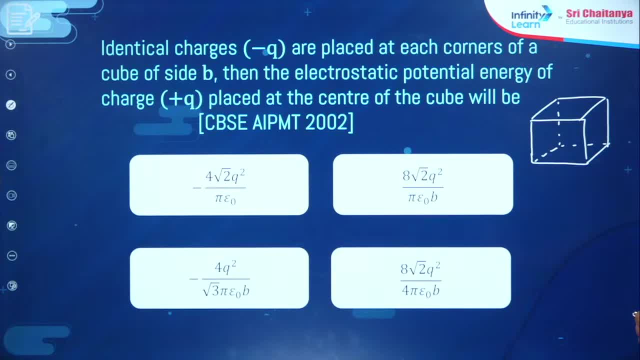 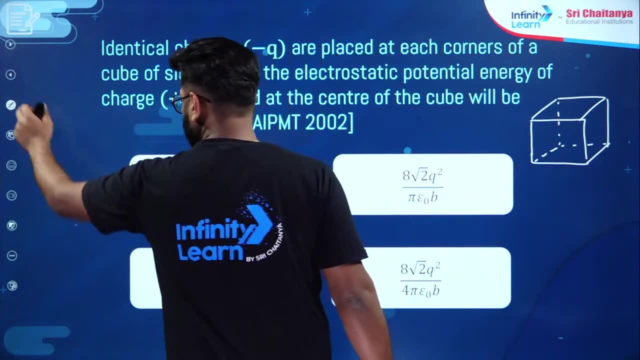 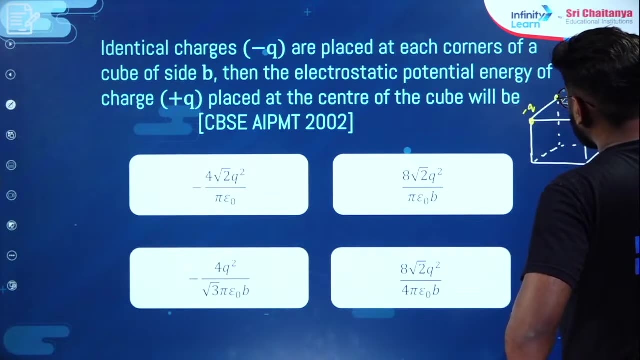 by pausing the video, ok, ok. so the answer is by pausing the video, ok, ok, ok, ok, ok, ok, and you have placed it at the center. what have you placed at the center? you have placed it at the center. plus q charge. 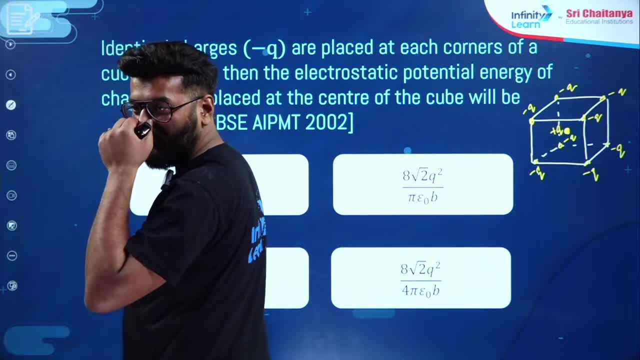 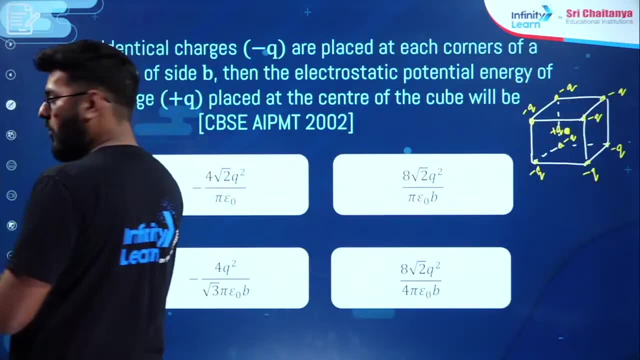 so here you should know only one formula: there is a factor of root 3 in which the answer is the same. you have said it absolutely right. you have said it absolutely right. you have said it absolutely right. very good, you should know one thing here, which is body diagonal, which is called body diagonal. 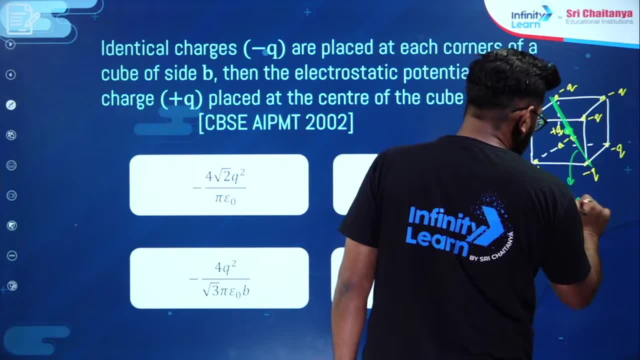 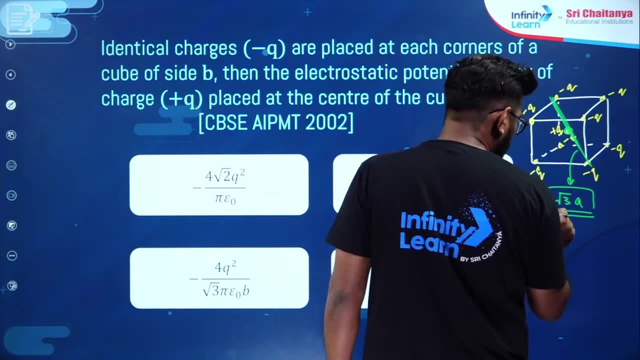 and the value of body diagonal is equal to root 3a. so every charge at the distance is body diagonal by 2, that is, every charge at the distance of root 3a by 2,. the value of r is at root 3a by 2,. 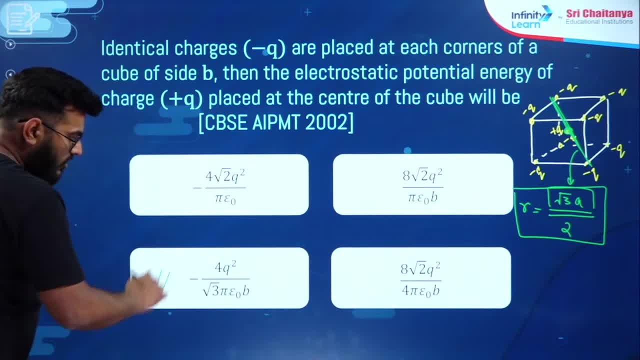 now, root 3 is in one option, which is option number c, and negative should also be there. why? because minus 3a by 2,, minus 3a by 2, you are taking the element of plus q and if you talk about the correct value, then see: 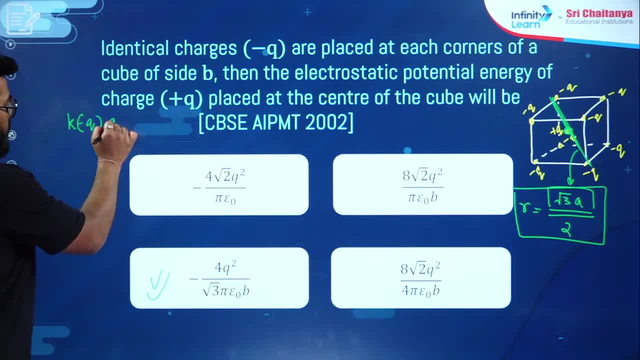 how much will it be by one charge k minus q, small q upon the distance between the two? how much will it be root 3a by 2, now just solve it. the answer will come 1 upon 4 pi epsilon. 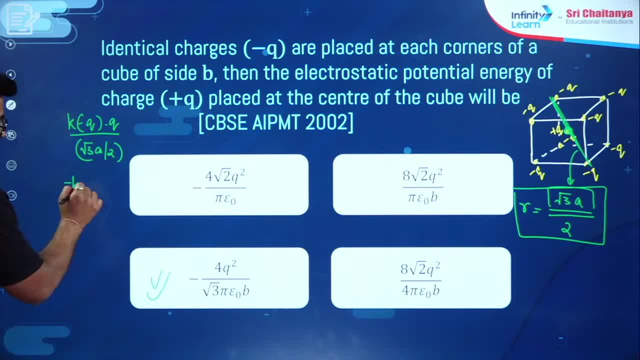 and it will cancel with 2,. so 2 pi root 3 will come k q square upon 2 pi epsilon naught into root 3,. ok, is it clear? and this is because of 1, and total will be 8,. 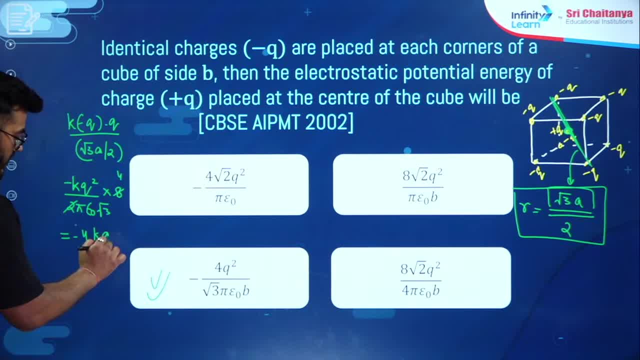 so 2 will go from 4, so minus of 4 k, q square upon root 3, pi. epsilon naught this is the answer. ok, here here this can also be said. here this can also be said. 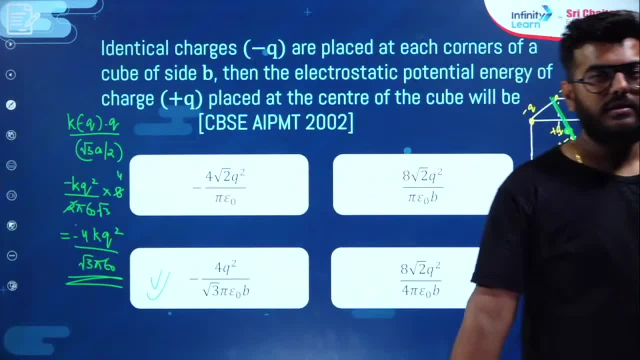 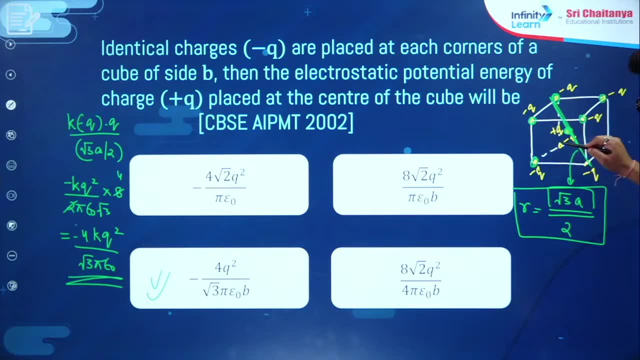 that how much is their individual total potential energy. so, in that you will have to pair both, you will have to pair both. you will have to pair both. I will give you a homework. try this and see that their individual potential energy will be how much of all the negative charges. 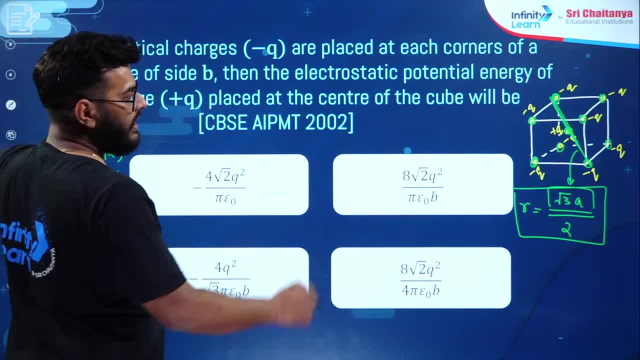 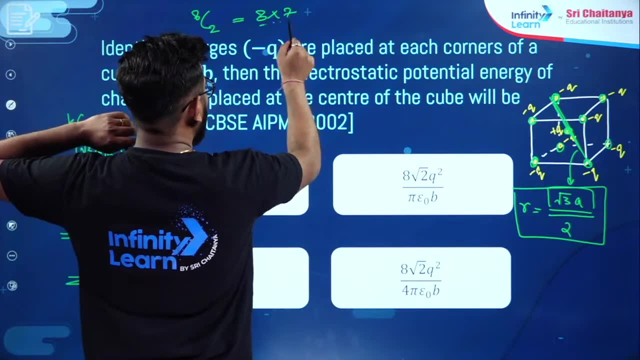 here. if you talk about the total, then the total is 8 right 8 c2, 8 c2, total is 8 charges right: 8 c2, means 8 into 7 by 2, total will be 28 pairs. 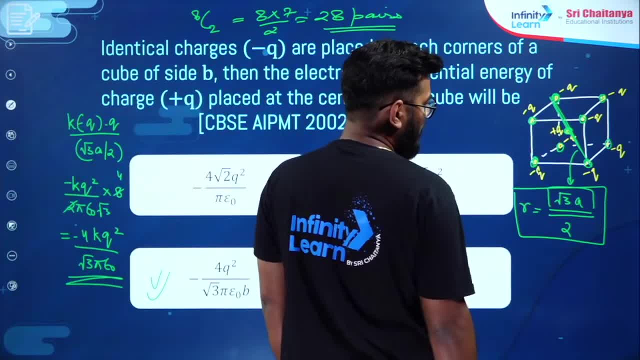 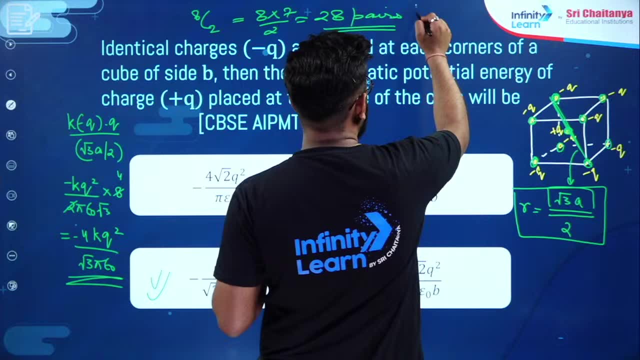 28 pairs will be made and you have to see that on every face, your total will be 12,. on every edge, your total will be 12 and 4 will be your body diagonals. out of 28, your total will be 12 on your face. 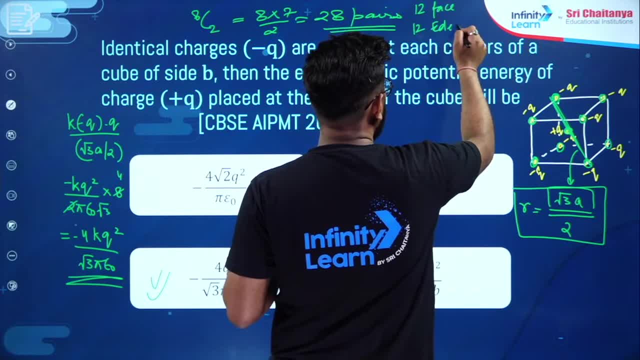 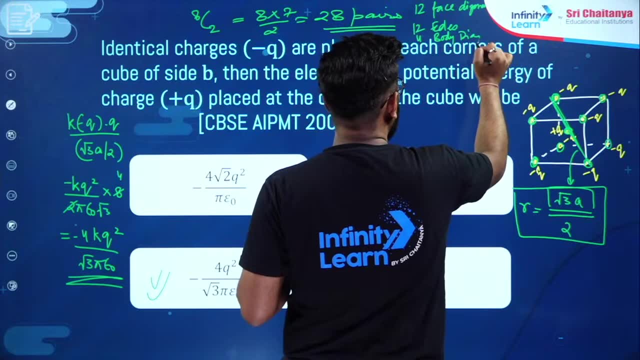 12 will be your edges, your face will be diagonal 12,. 12 will be your edges and 4 will be your body diagonals. this many pairs will be made. try it and see, imagine it and see and ask for the total potential energy and see. 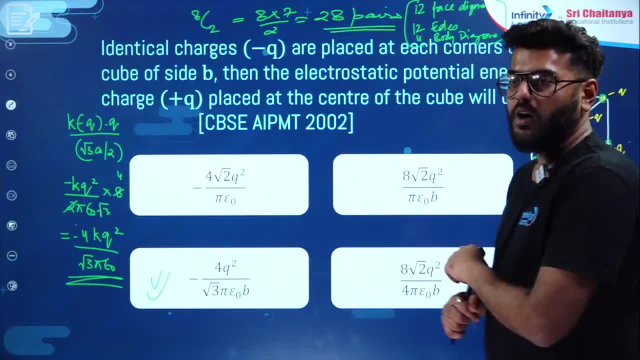 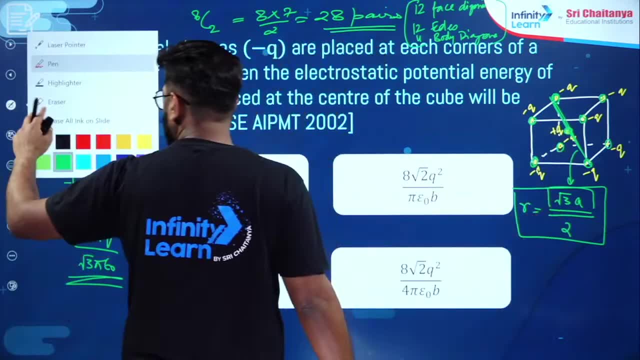 if you take it from infinite and write everything, then it will come 7 times. I am not saying that, I am not saying this. I am saying: forget for a second. this is a question of plus q charge. this is not a question of plus q charge. 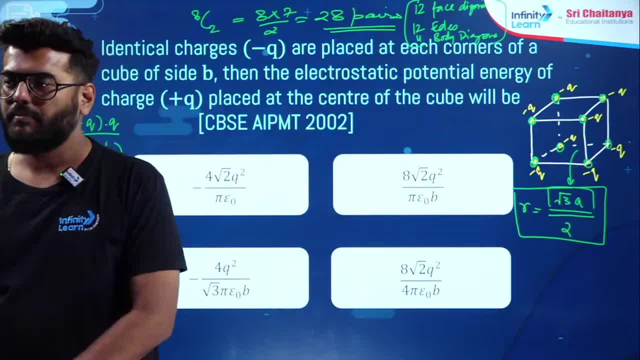 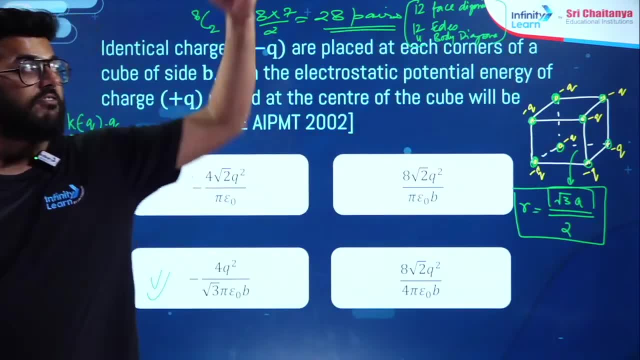 here all the negative charges are sitting on vertices and you have to find out the total potential energy of the system. this is the question. that is a different thing. if you take it from infinity and bring it to its center, then how much work did you do? 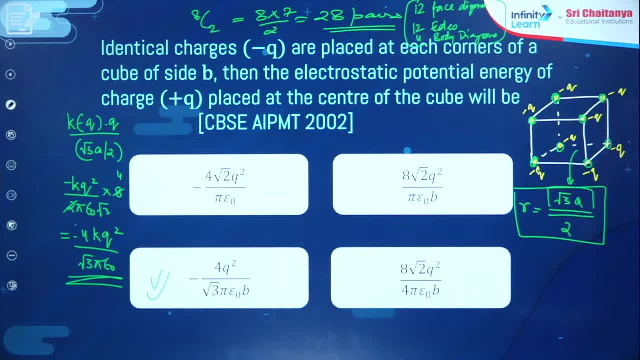 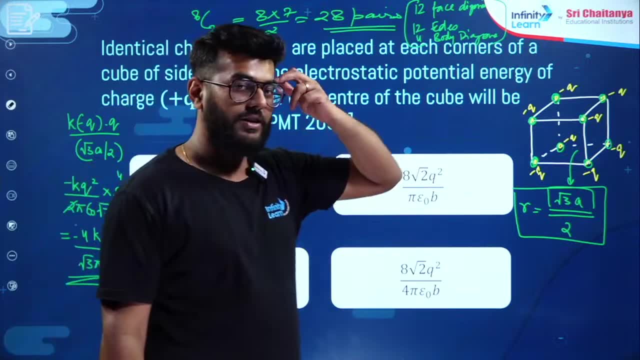 I am not saying that, I am just saying all the corners have negative q and negative q charges. so how much is the total potential energy? so total will be 28 pairs minus q, minus q, like this from this you see. 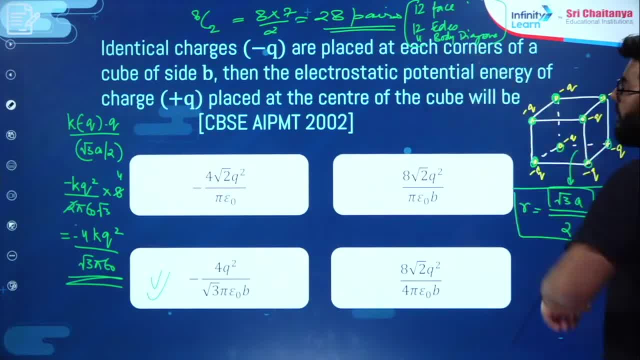 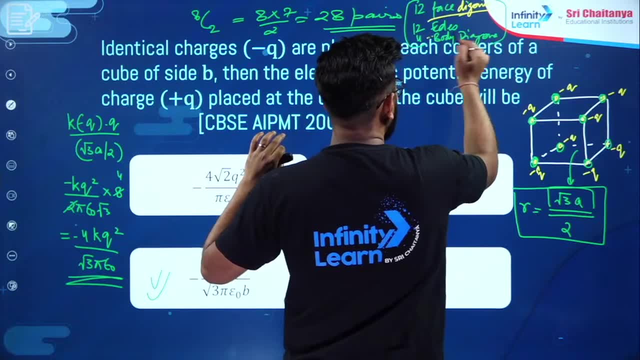 12 will be phase diagonal, 12 will be your edges and the remaining 4 will be your body diagonal. try it, imagine it and think this was asked in JEE main. maybe it is an old question. ok, in bringing an electron towards another electron. 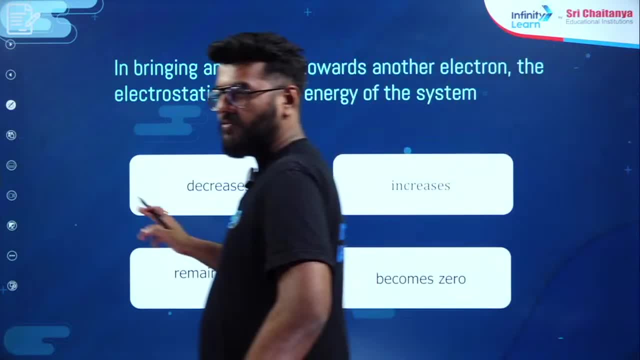 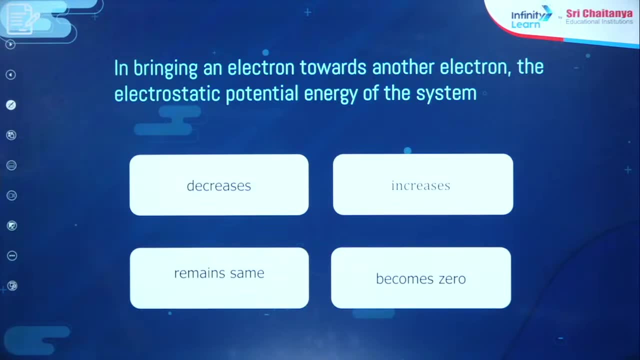 the electrostatic potential of the system. I have already done this in the class. tell me quickly what will be its answer in bringing one electron to another electron, the electrostatic potential energy of the system increases or decreases or remains the same? 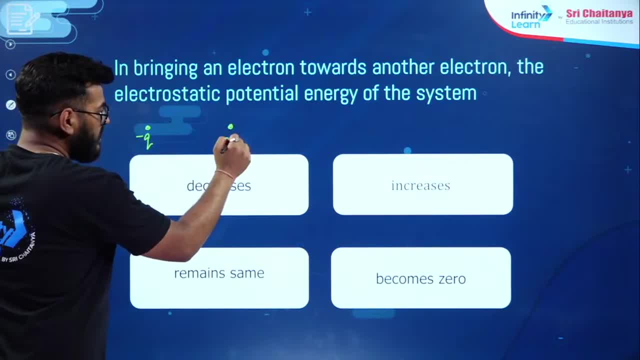 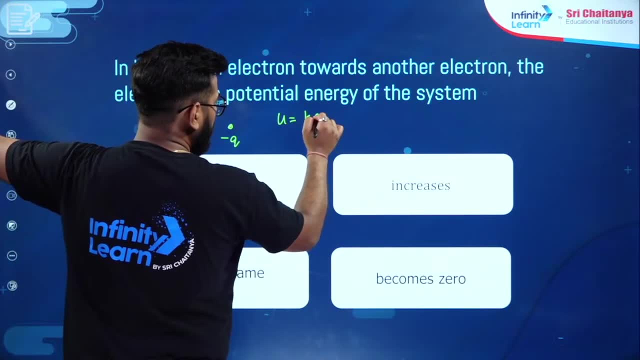 one electron. if I am bringing one electron to another electron, then what will happen? the potential energy will increase or decrease. sir, the potential energy is kq minus q into minus q. divided by r, this will be plus kq square by r. 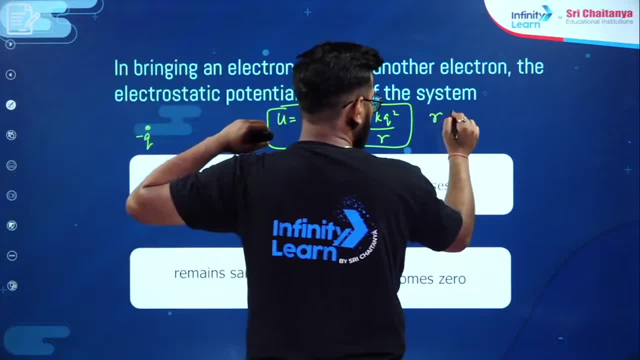 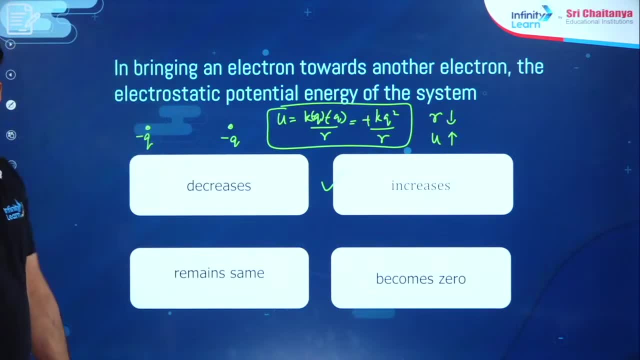 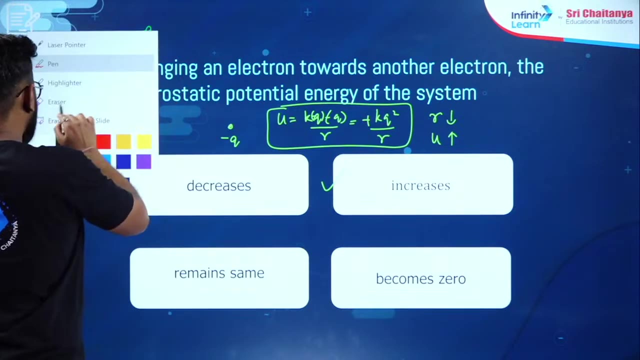 so if I am bringing it closer, if I am reducing r, then the value of u will increase. it will increase. now one more variation in this. if assume here I bring minus q closer to plus q, if I bring minus q closer to plus q, 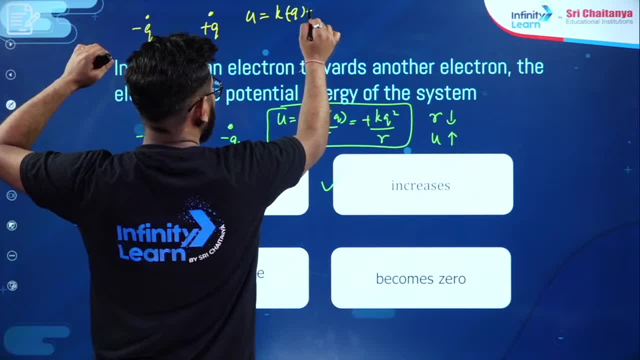 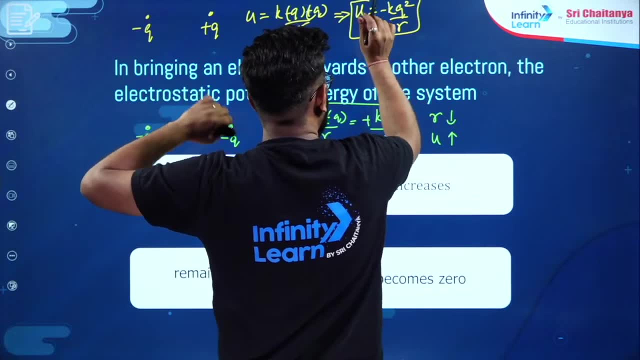 then what would be the potential energy? k minus q plus q divided by r? this would be: u is equal to minus of kq square by r. now, since it is negative, if I increase r, if I increase r, then the overall value will decrease. 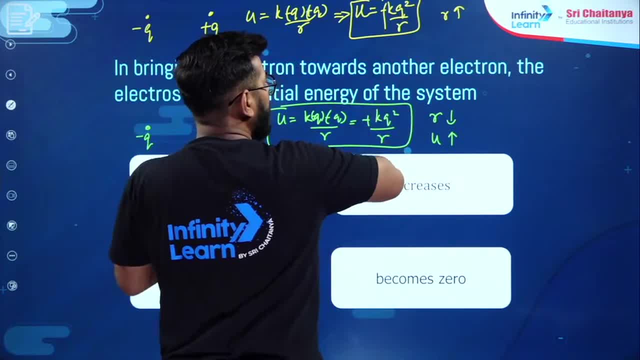 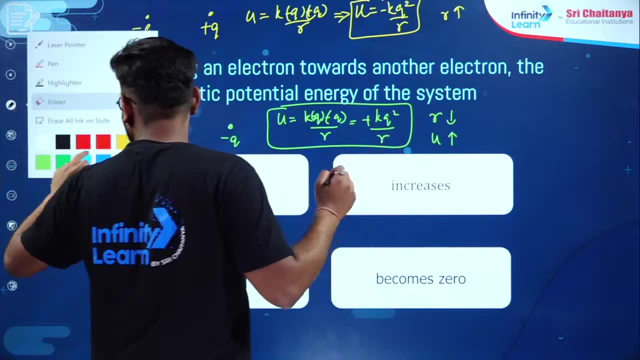 this magnitude will decrease. and this magnitude will decrease in the negative. it will decrease. more means how much will it decrease? see in the negative. in the negative, which is minus 5, it is smaller than minus 2,. 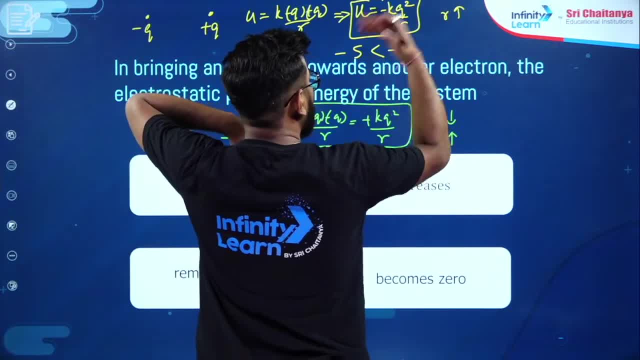 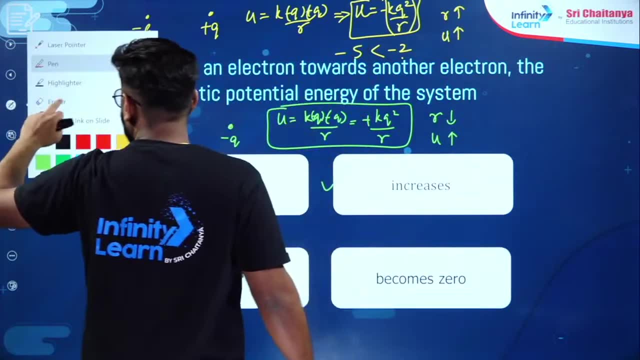 isn't it minus? minus 5 is not going from minus 2, it is increasing. so this magnitude will decrease, but it is in the negative, so the value will increase, that is, it will increase. the potential energy will increase. 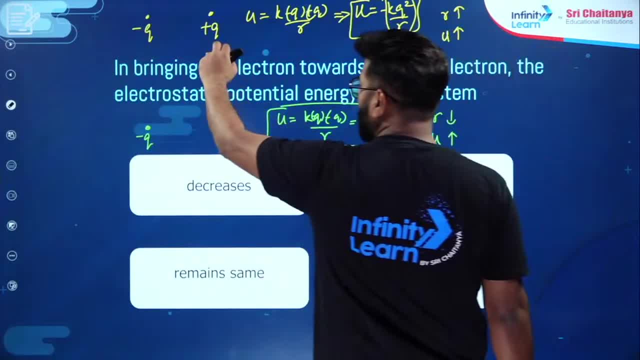 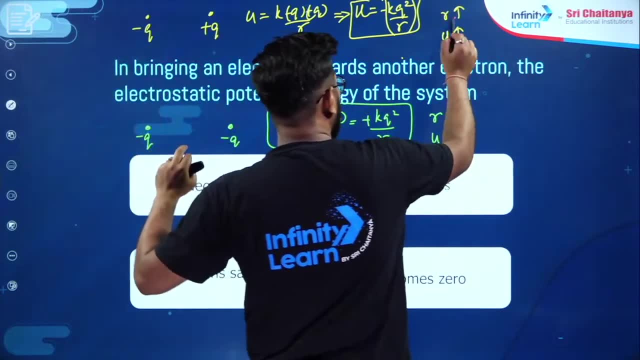 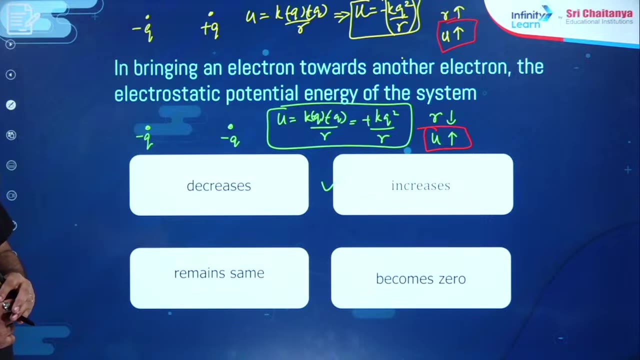 understood if, if in the negative and positive, if you decrease r, then the potential energy is increasing. the potential energy is increasing, it is increasing. but if in one negative and one negative, then the potential energy one minute. 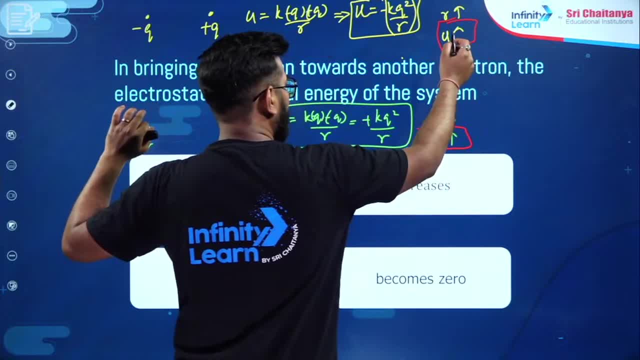 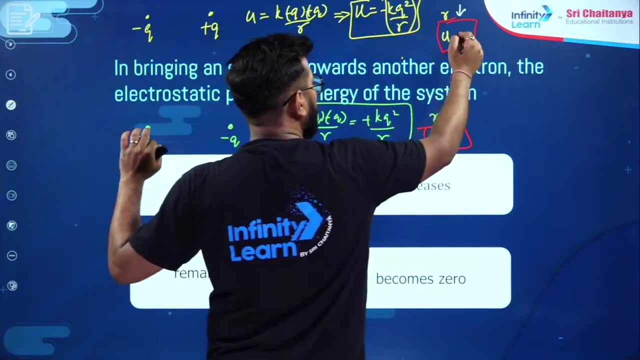 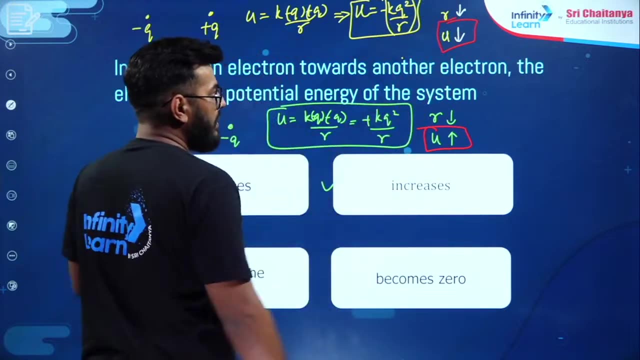 sorry if we decrease r. sorry, if we decrease r, then this value will increase. increase means it will decrease more. yes, this is the case. if you decrease r, if you increase r, then it will increase too. means. here is the same nature. 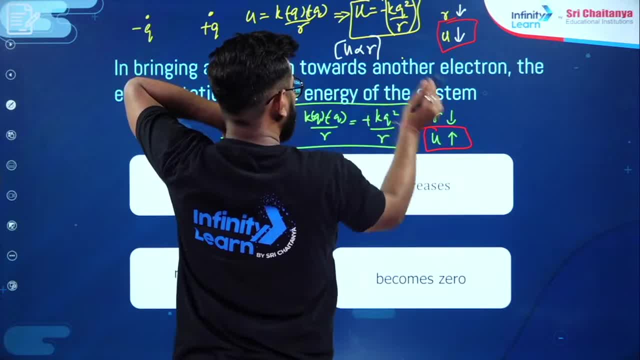 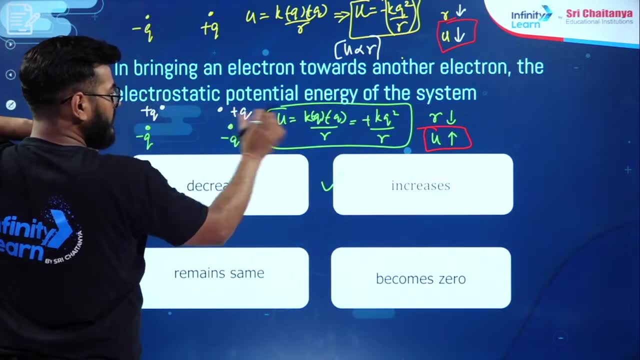 when it is negative, then u is directly related to r, and in this case it will be negative, negative. same charge, even for positive, positive too, even for positive, positive too, same nature will remain means your u is directly related to whose. 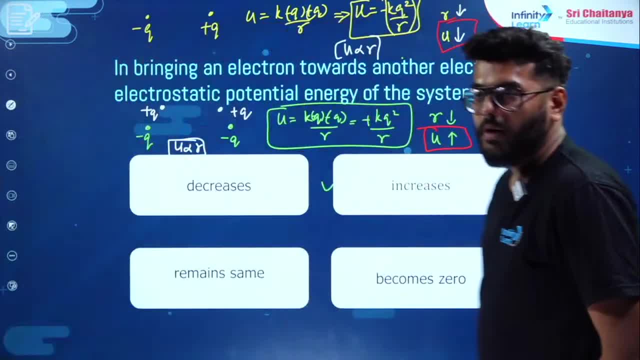 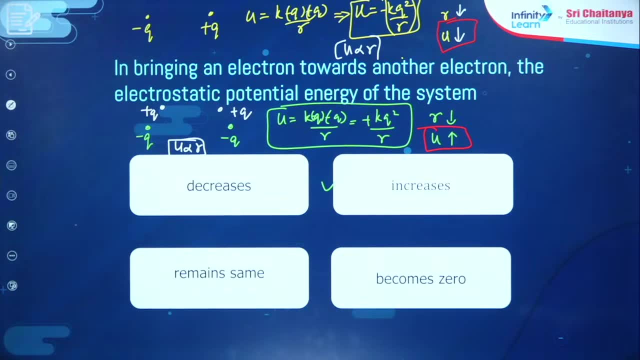 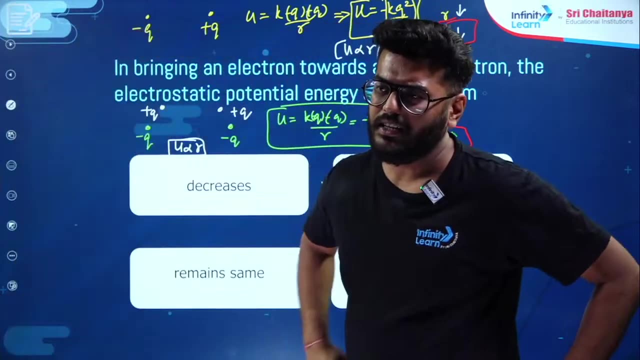 to r. if I talk about two masses, if I talk about two masses, if I talk about two masses, two negative charges repel but we take towards, we take towards. so in universe, the work against, against what is written, I can't see. 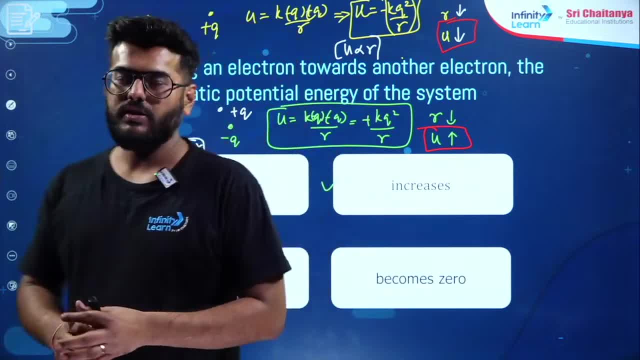 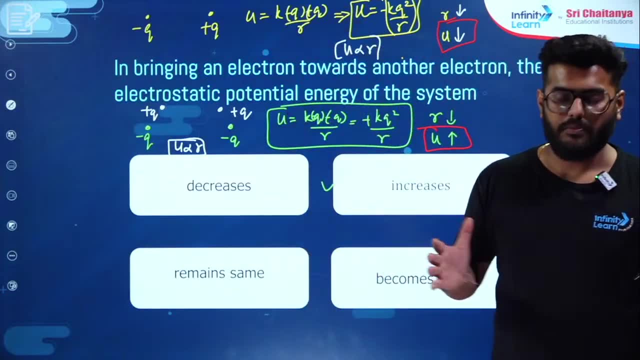 if you want to understand the concept in this way, then you can understand that whenever there are charges of same polarity, then you have to work, you have to work, you need to bring them, you have to bring them. so if you bring them, then your energy is disappearing. 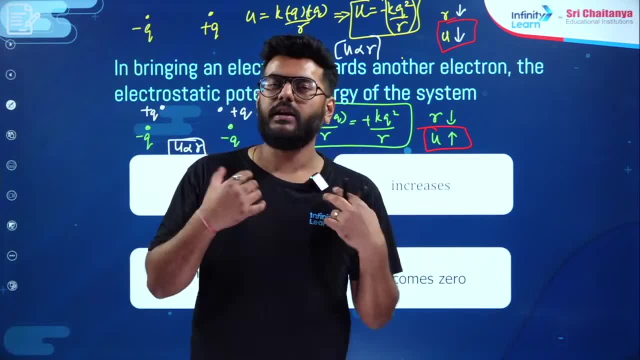 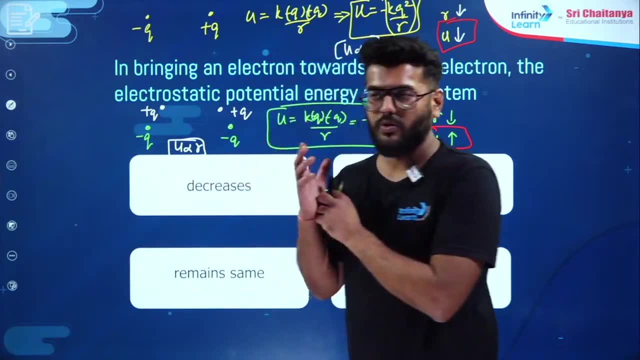 you are repelling each other. you are bringing them closer. you are dissipating your energy. if you are dissipating your energy, then where is your energy going in the form of their energy? the work you are doing is being stored in their energy. 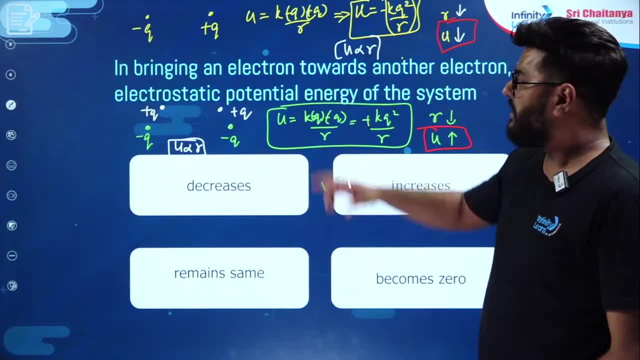 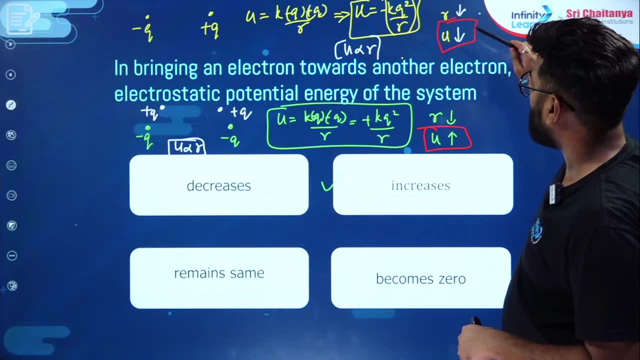 so the work you are doing is being stored in their energy, so their potential energy will increase. here they want to come themselves. so their potential energy is decreasing. so as the value of R decreases, the potential energy will start decreasing. if I talk about two masses- 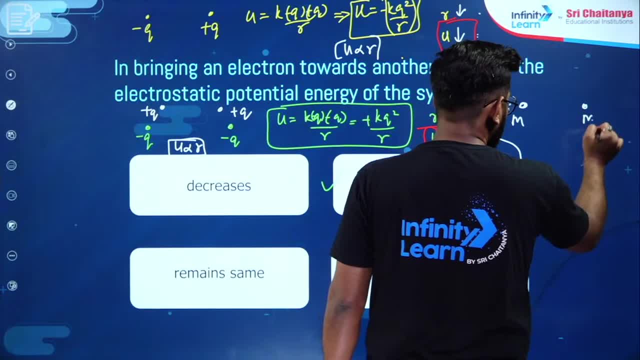 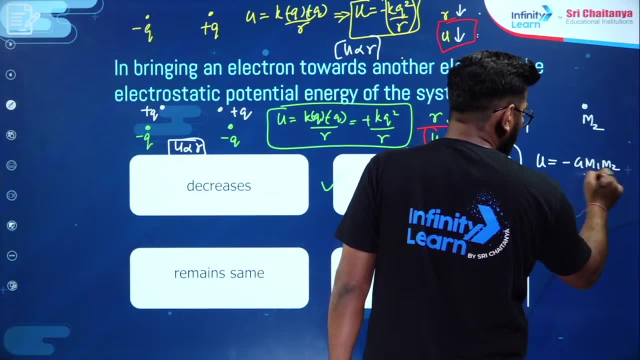 two masses, M and M. so what will happen here if their value decreases? M1, M2. so here you will see minus of G, M1, M2 by R. so here also, as the value of R decreases, the potential energy will also decrease. 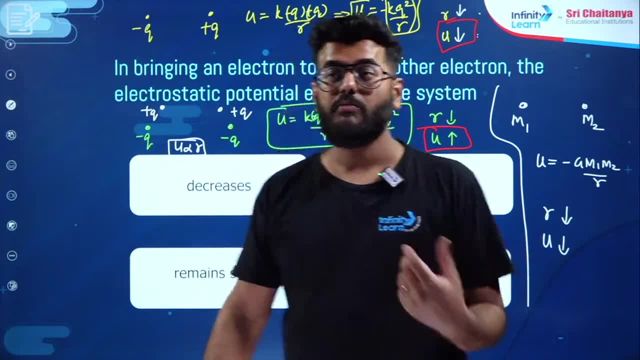 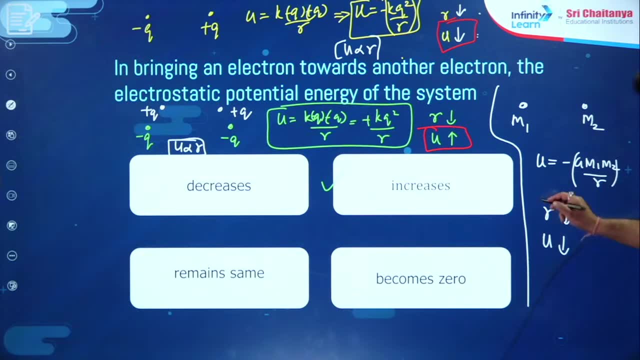 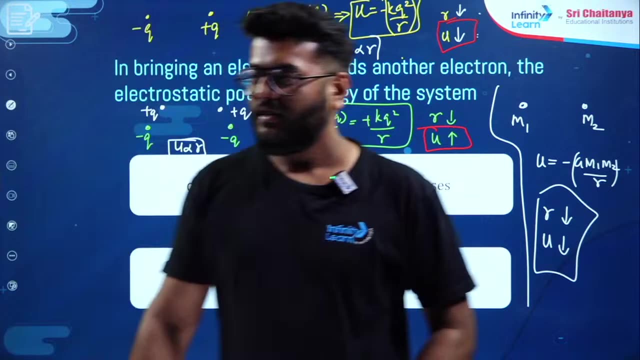 as the value of R decreases, the potential energy will also decrease. you can see, if it decreases, then it will increase overall, but because it is negative, then it will decrease overall. so the calculation for this will go like this: is it clear? did you understand the thing? is it clear? 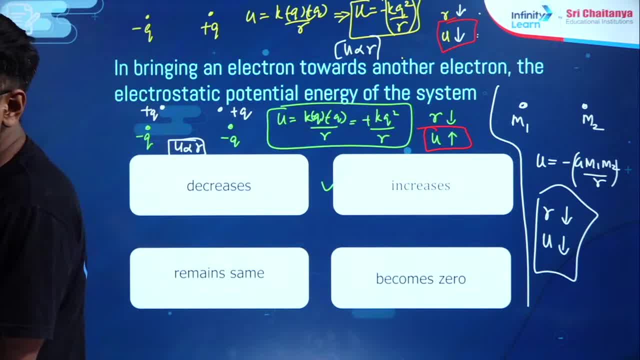 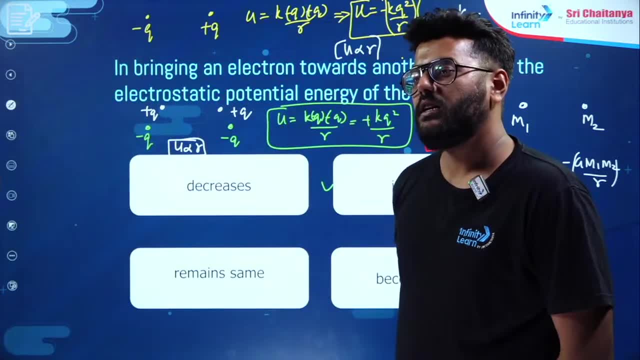 suppose you don't have anything, just free space, then the first charge lie is 100 from infinity, change in potential energy is 0, then if you bring the second then due to the first, then it will keep going like this. so do it like this, do it like this. 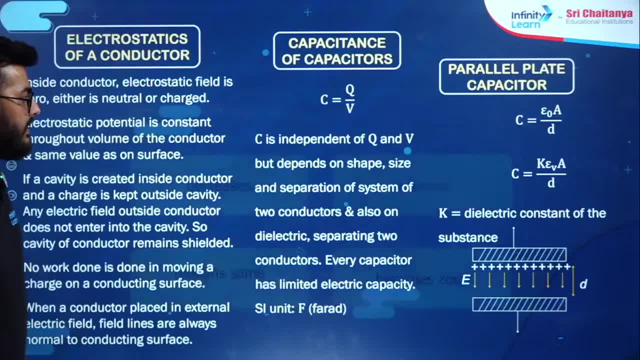 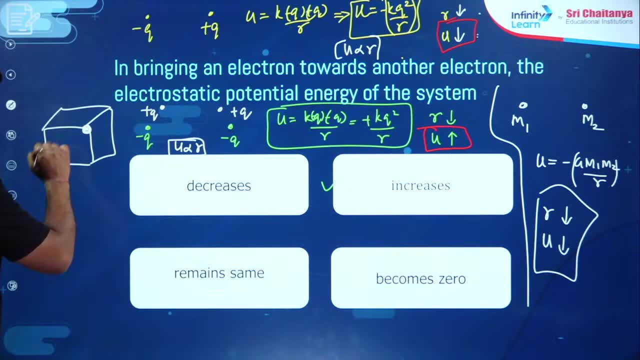 but what will happen if you do it like this? see the problem. for this. what will you have to find out? first lie: you don't have to do any work. second lie: so because of this, you will have to find out that how much is the potential energy between these two? 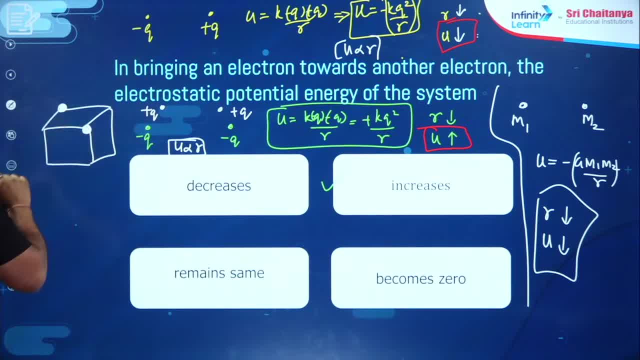 you have done that much work, how much is the potential here, how much is outside? you have done that. then when you bring the third, then because of this you will have to find out here, because of this you will have to find out here. 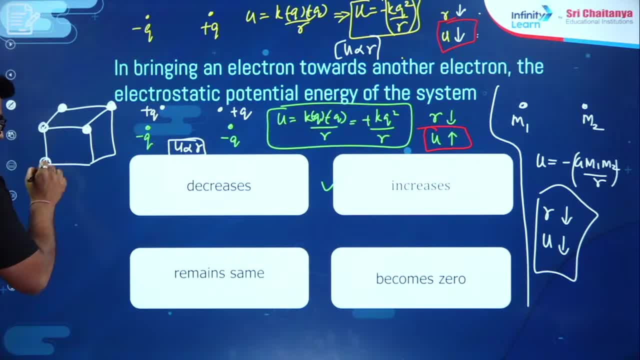 then if you bring the fourth, then you will have to find out. because of this, because of this, because of this. then if you bring the fifth, then because of this, because of this, because of this. if you bring the sixth, then because of everyone. 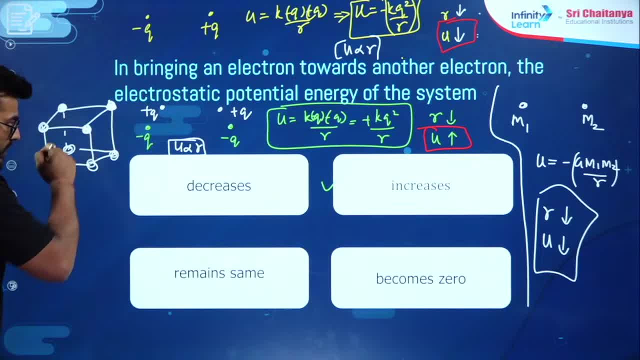 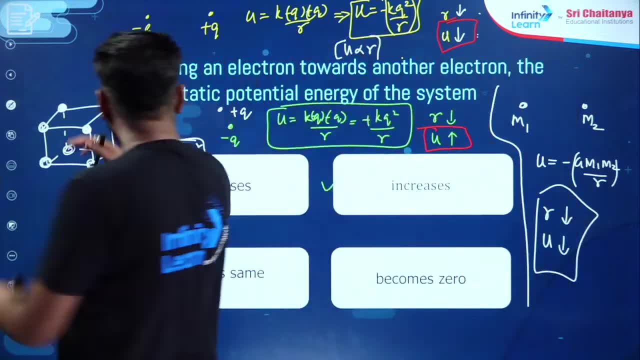 if you bring the seventh, then because of everyone, and if you bring the eighth, then also because of everyone. so if you do it like that, then also the answer will come. but how long is the method? just think about it. ok, so please remember this. 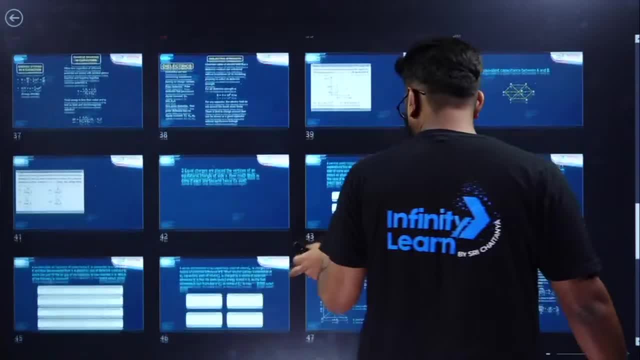 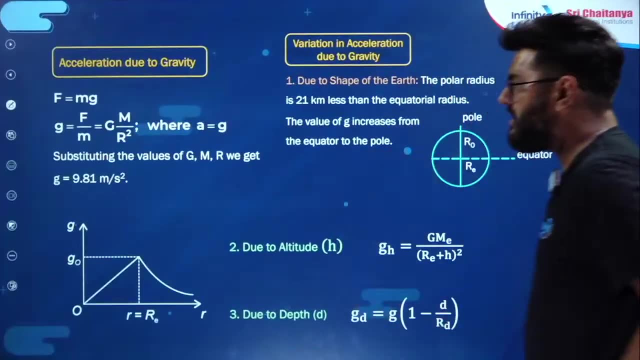 Now, before starting the capacitor, I want to tell you about the acceleration due to gravity. aspect of gravitation. Yes, it will be a long solution. There are still many questions in the file, so please download today's notes and try all the questions. 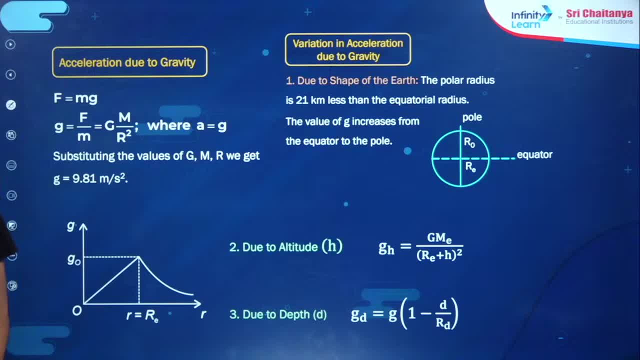 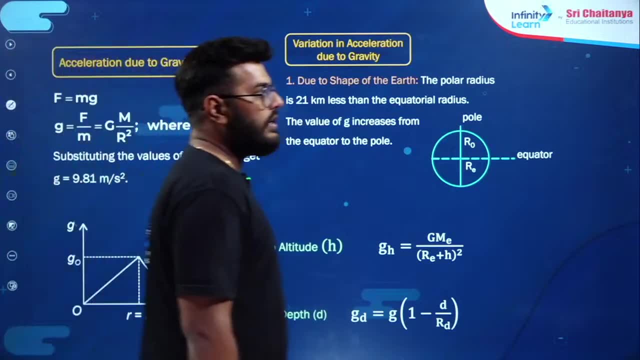 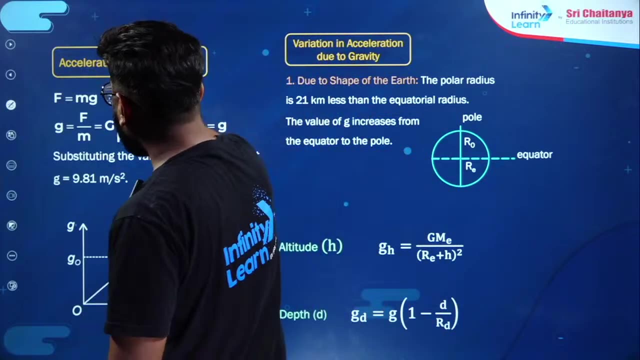 I have already done a lot of them. there are some new ones too, But please solve these questions because they are good ones. Acceleration due to gravity is a magnitude of gravitational field intensity, Because how does acceleration due to gravity come- The force is related to mass- into acceleration. 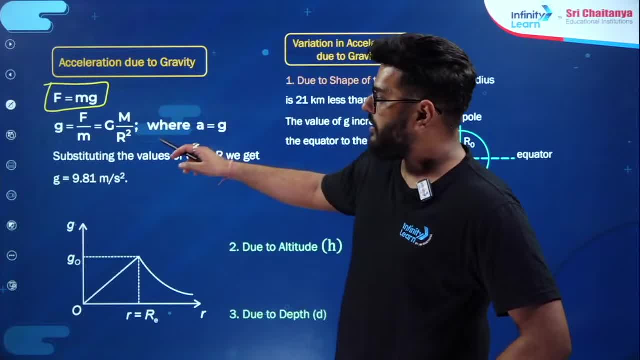 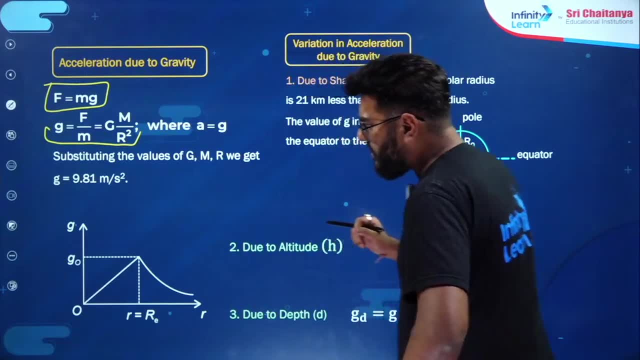 And the value of g is f by m. So the value of g is gm by r square, Where m is the mass of the planet and r is the radius of the planet when it is on its surface. Now how does its variance occur? 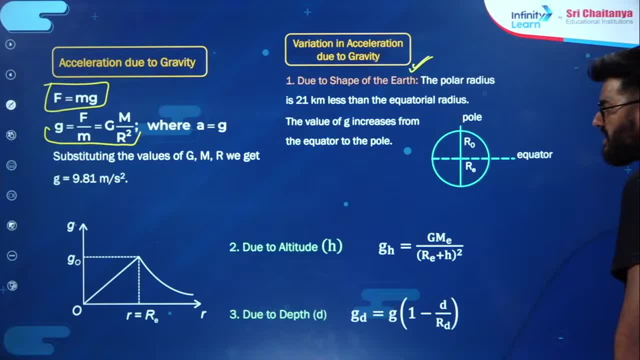 Its variance occurs Because of the shape of earth. There is more gravitation on the poles and less on the equator, because the radius of the poles is small and the radius of the equator is more. Altitude is done by height h. 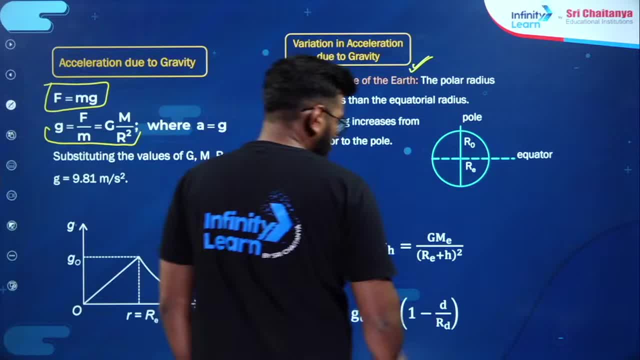 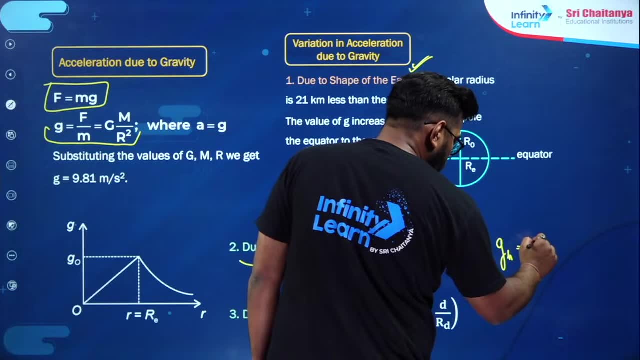 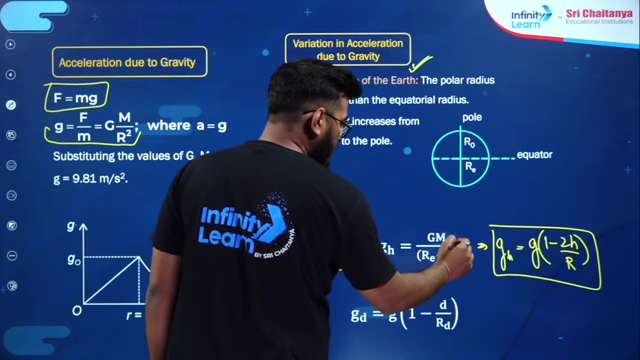 How much is it gm by r plus h square? And you can write this as well: g at h is equal to small g 1 minus 2h by r. When can you say this? You can say this: Multiply r square by r square. 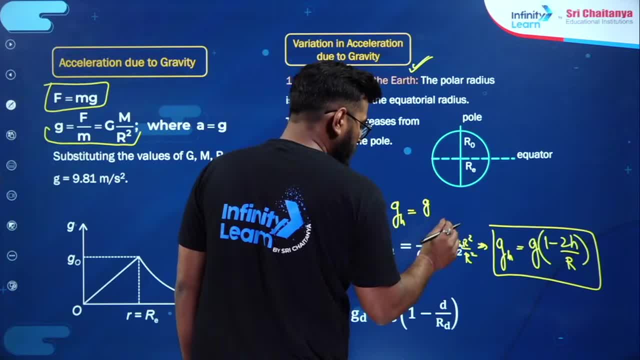 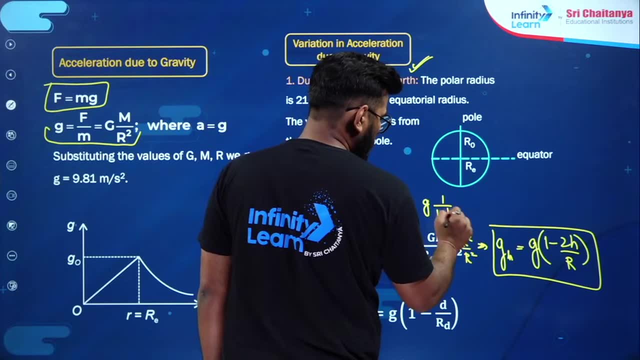 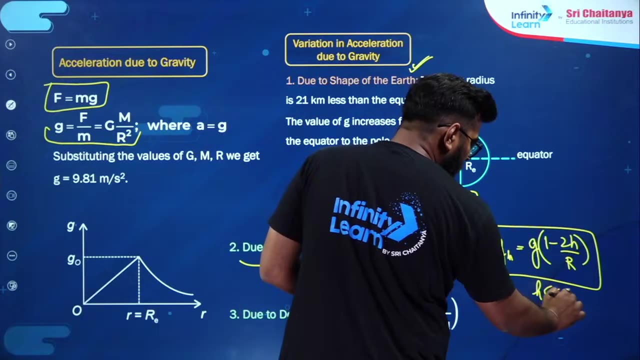 This is the formula. g at height h is equal to g 1 upon 1 plus h by r whole square. This is the formula, And the other formula is this: When is this valid? When the value of h is very small from the radius of earth. 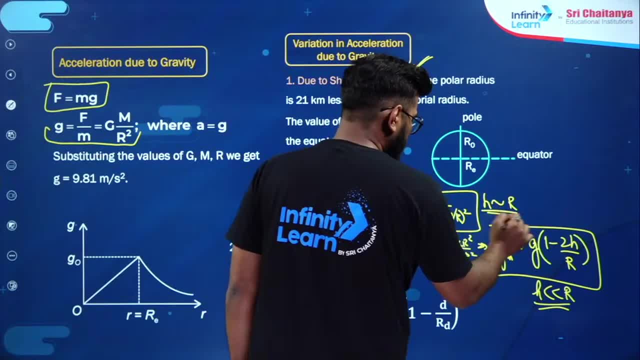 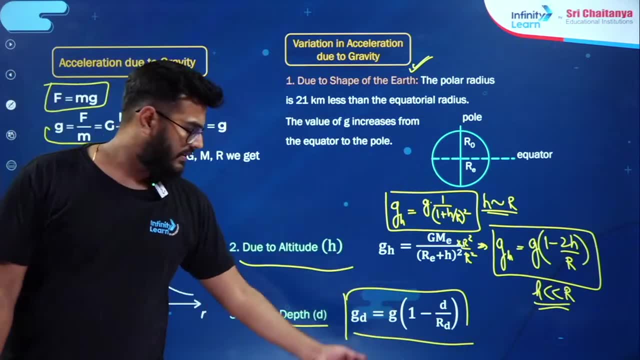 And this is valid everywhere. This means when h is comparable to r, This is the depth. when you go to D, If you go to any depth, the formula is going to be the same: g 1 minus d by small r. Now acceleration due to gravity. 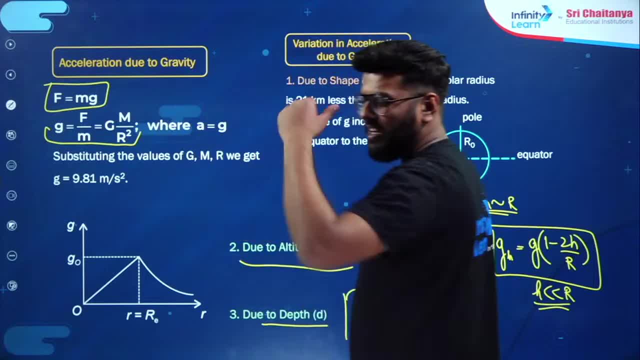 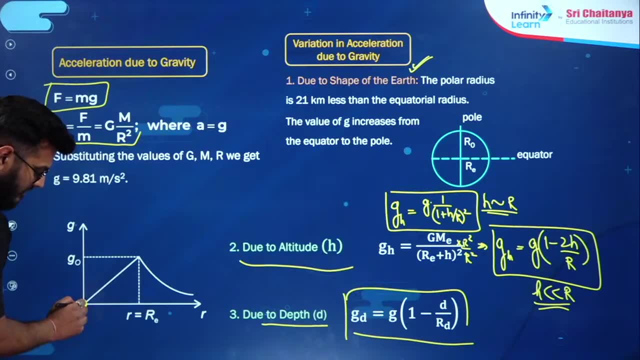 As I told you, acceleration due to gravity is actually the intensity of your gravitational field lines. Now, the intensity of gravitational field lines, You tell yourself how the gravitational field line goes. If I talk about the inside, then the gravitational field line is directly related to r. 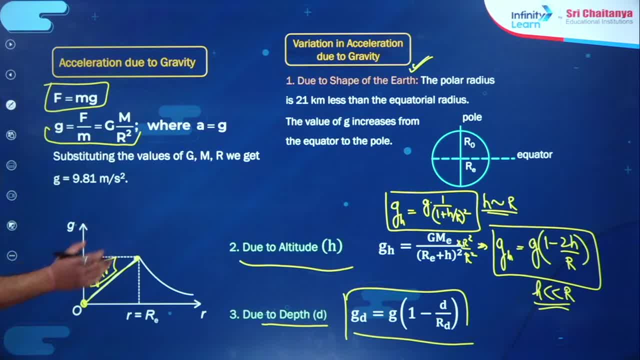 Like there is an electric field line in a non-conducting sphere, And how does it vary after that? How does it vary After that? it varies from 1 upon r square. So according to the variance, the values are also written here. 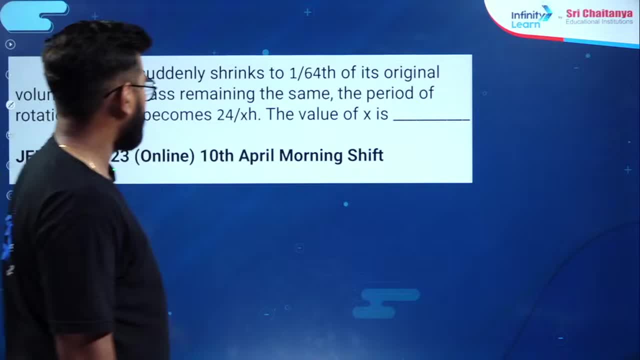 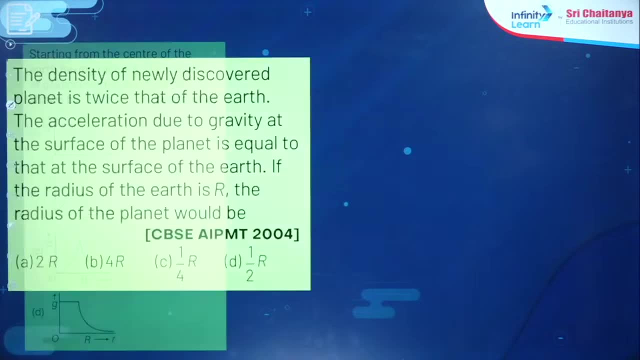 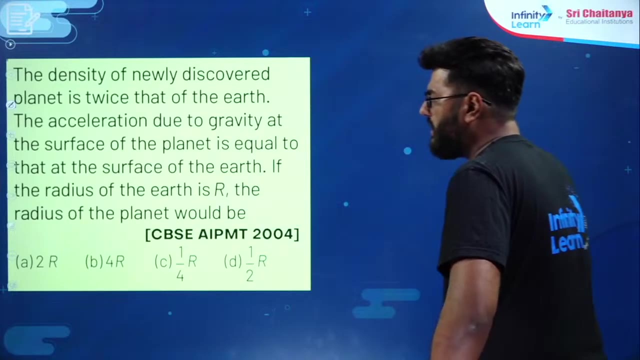 Now there are questions related to this which we want to see. So let's see quickly. The density of a newly discovered planet is twice that of the earth. The acceleration due to gravity at the surface of planet is equal to that at the surface of the earth. 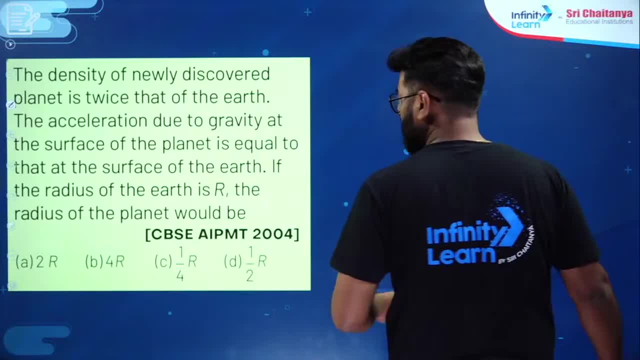 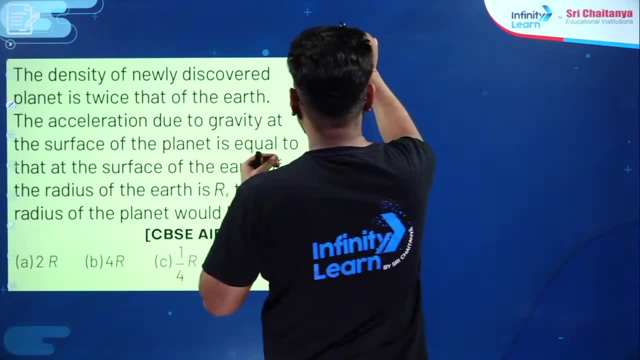 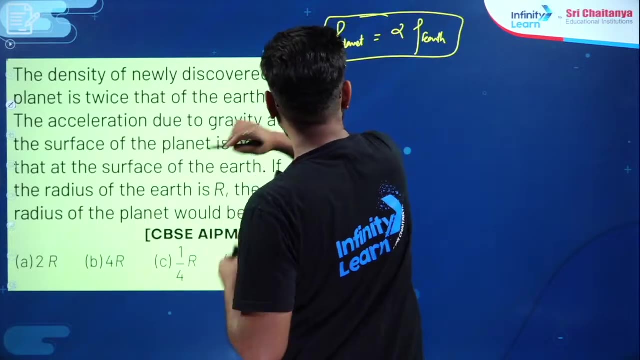 If the radius of earth is r, the radius of planet would be: How much would the radius of planet be? The radius of planet would be: how much? Look, the density of a newly discovered planet is twice that of the earth. The radius of the planet will be 2 times the density of the earth. 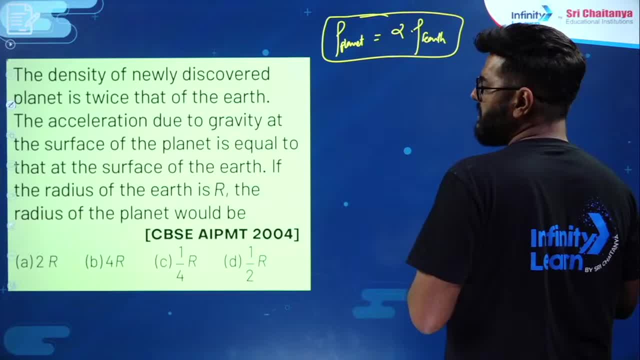 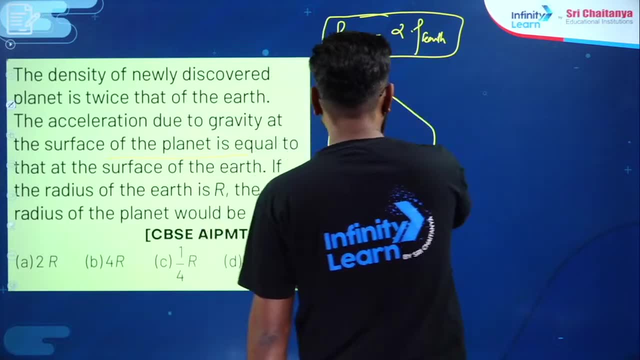 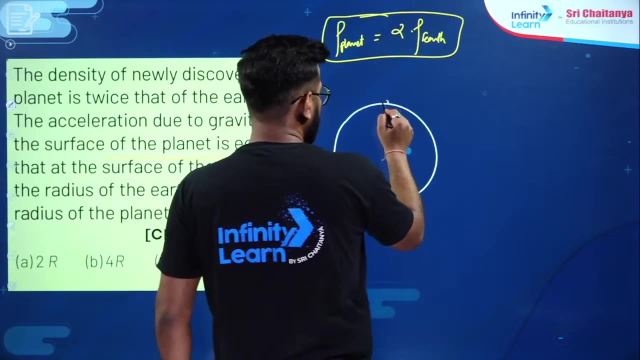 Okay, done. The acceleration due to gravity at the surface of the planet is equal to the acceleration at the surface of the earth. Okay, the acceleration due to gravity at the surface of the planet, On any planet, how much is the acceleration due to gravity? gm upon r square? 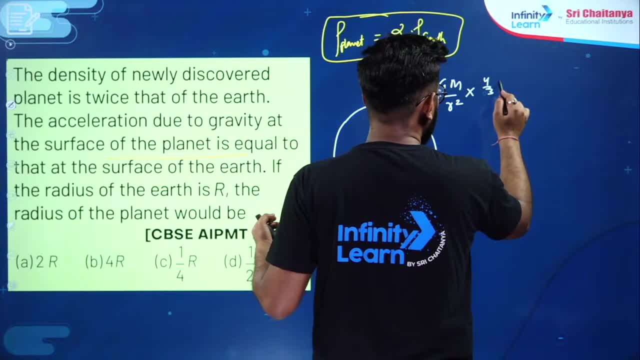 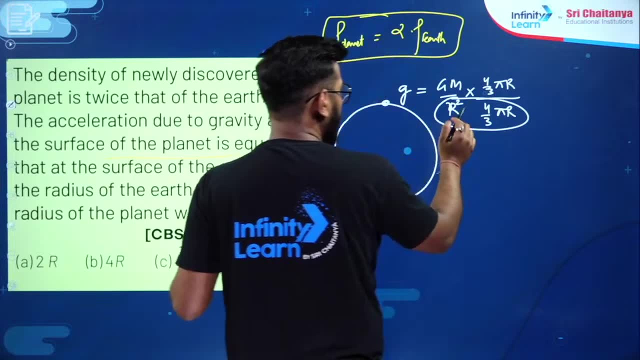 I am not enjoying it. I will bring it in density. How will I bring it? 4 by 3 pi r multiplied by 4 by 3 pi r multiplied by Right? Yes, Now, 4 by 3 pi r is volume. 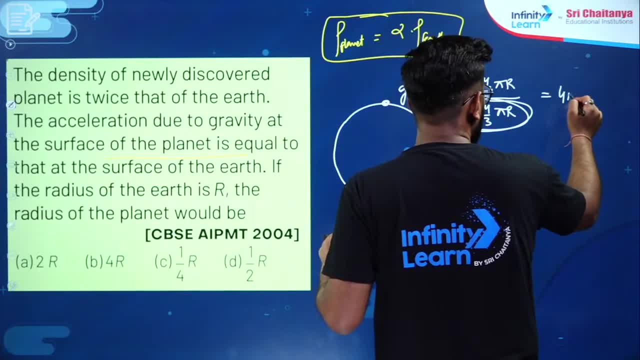 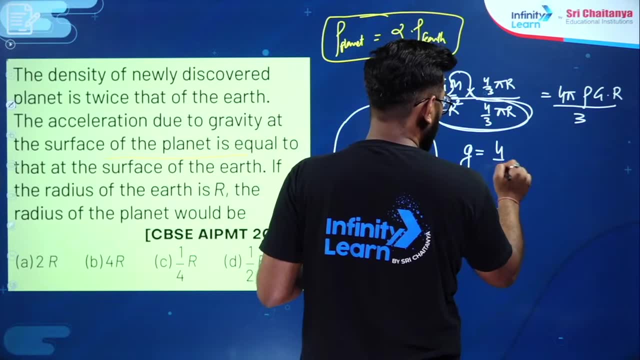 And mass upon volume is density. So see, the formula has come: 4 pi rho gr by 3.. So how much is the value of g? g is 4 by 3, 4 pi by 3 rho gr. Okay, Now, from here you will understand something interesting. 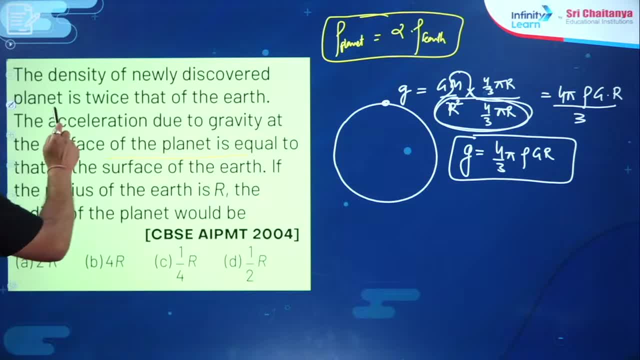 What, Sir see? the value of g. What is changing here? Density is changing And what is changing? Radius of earth is r and the radius of planet will be, And the value of g is equal to both. Okay, So you take g. g is directly proportional to rho into capital R. 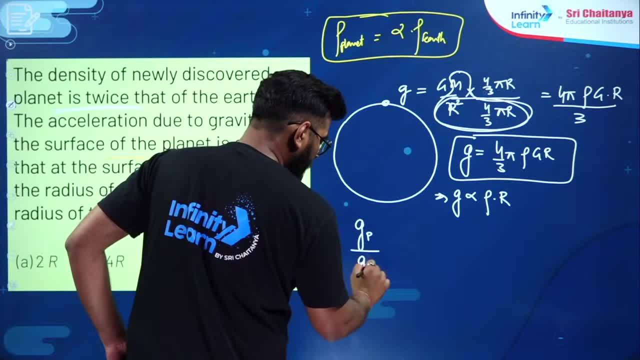 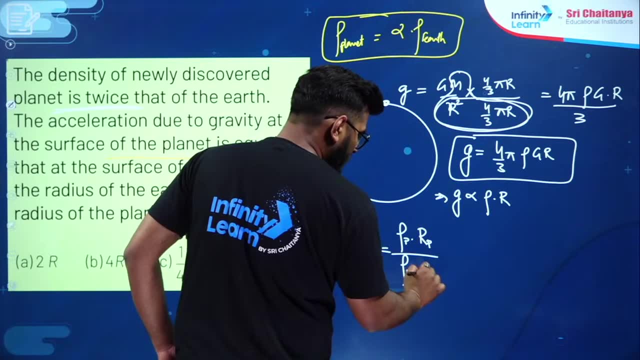 And here relate: g on the planet is to g on earth Is equal to rho on the planet into radius of the planet, is to rho of the earth into radius of earth. That's it, These two are equal. So 1 is done. 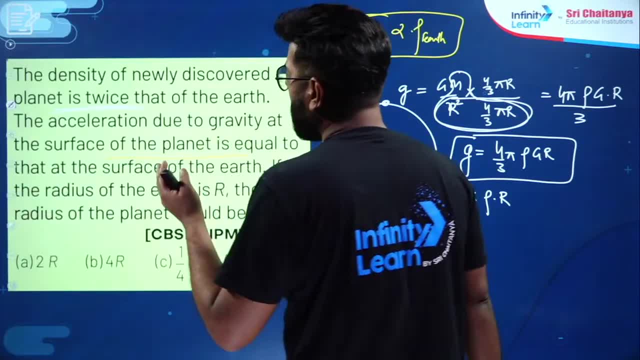 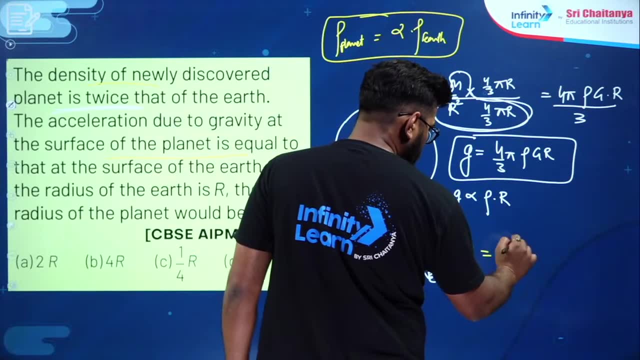 Now, how much is rho of planet? Is rho of planet given, Discovered newly? planet is twice that of earth. Its density is twice that of earth. It has come twice, So 1 will be 2 times. rho of earth is to rho of earth into radius of the planet, into radius of the earth. 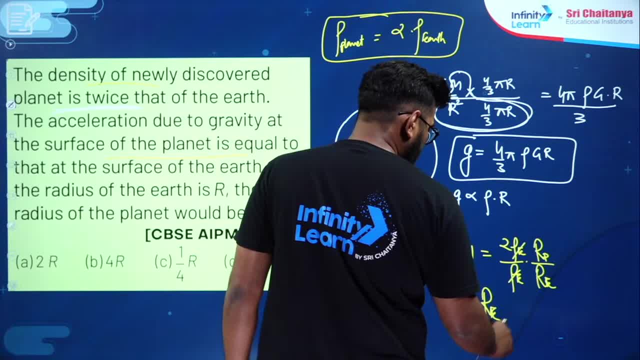 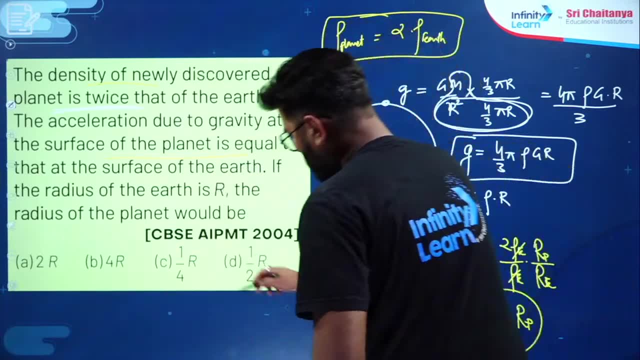 This is cancelled. So how much will be radius of earth? Radius of earth will be half of radius of the planet. You had to tell this only How much is the radius of the planet? Half of earth? Okay, Option no D. 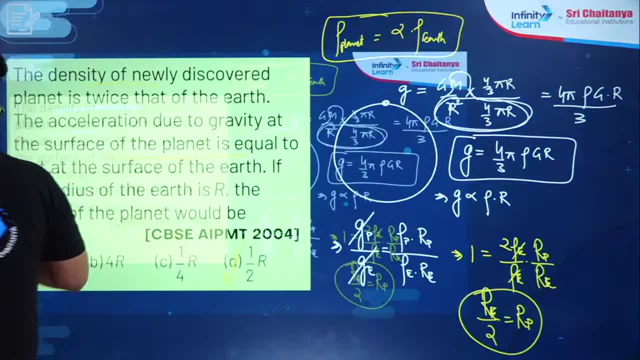 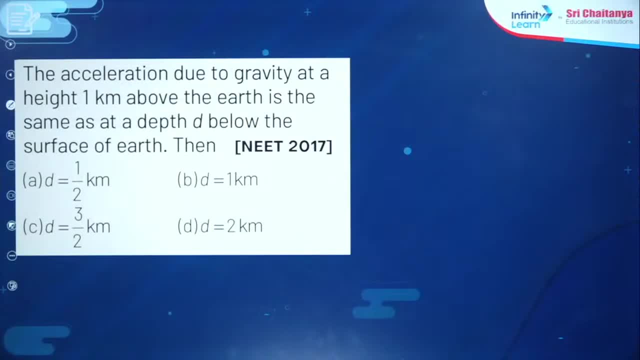 Very good, Very, very good, Very nice, Very nice. Okay, After that, see this: The radius acceleration to gravity at a height 1 km of the surface is same as at a depth d below the surface of earth. Then Simple question: 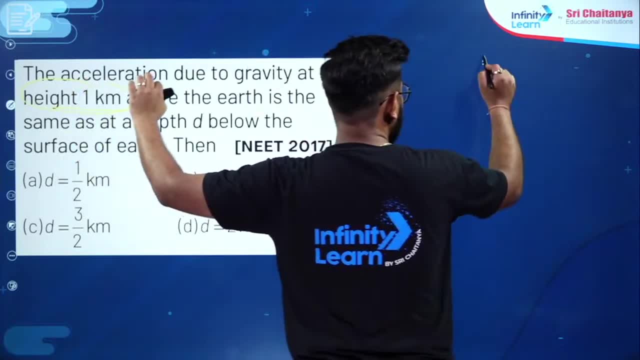 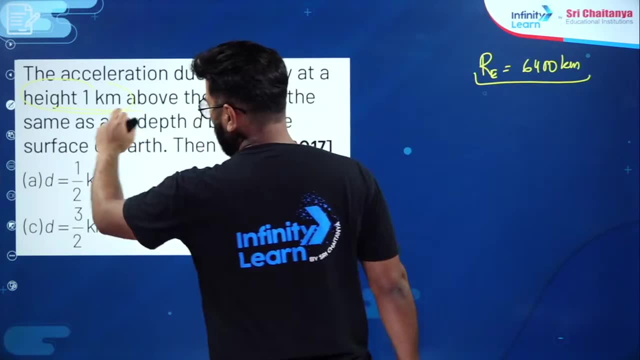 He is asking height above 1 km. Now see how much is the radius of earth. Radius of earth is 6400 km. So if you are going up and down, 1 km Means you are taking height 1 km. 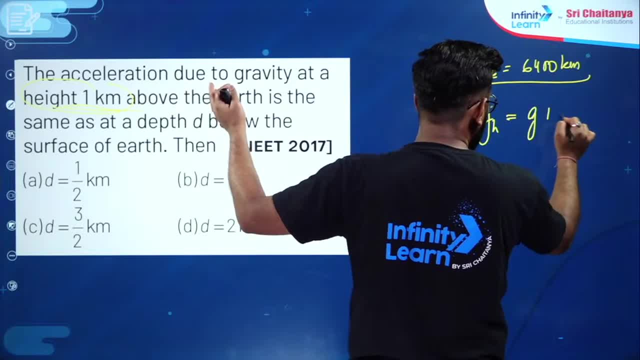 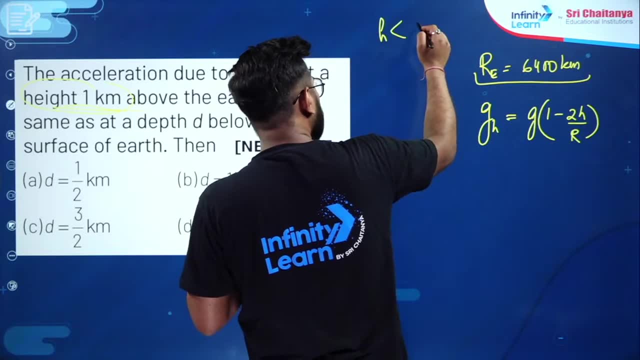 So, obviously, which formula you have to take? You have to take g into 1 minus 2 h by r. There is no doubt in this. As long as the value of height is given less than 50 km, By the way, 50 will also be more. Take 10.. 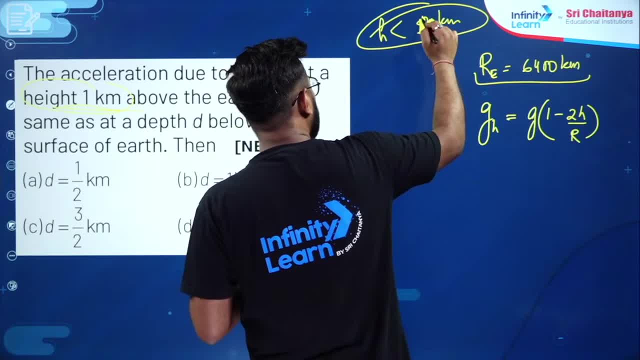 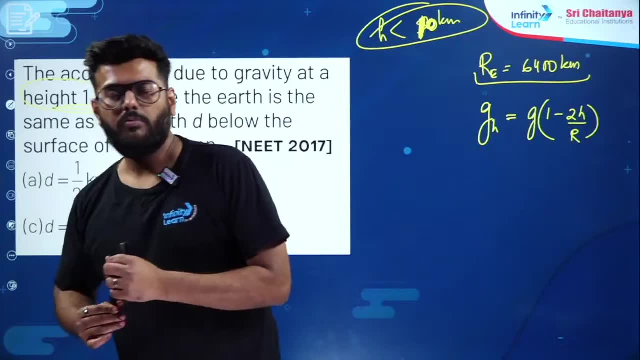 Because in 50, we should not take this into account- But less than 10 km. And do you understand the meaning of less than 10 km? I am talking about Mount Everest. I am talking about Mount Everest. What is the height of Mount Everest? 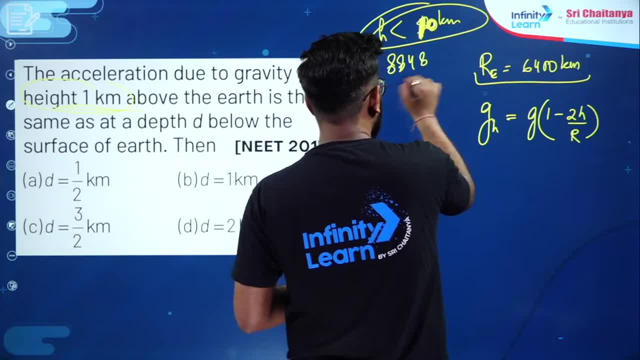 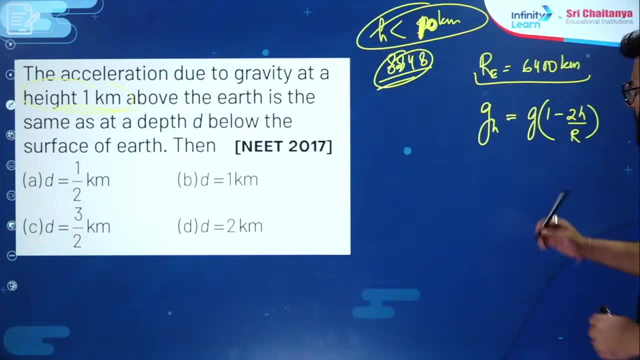 8.8.. 4.8.. Means: 8.8 km. This is the height of Mount Everest. So if your height is less than 10 km, Then you can definitely use the formula. So it is simple. 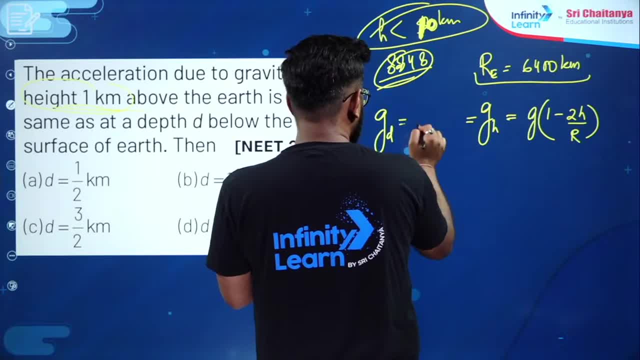 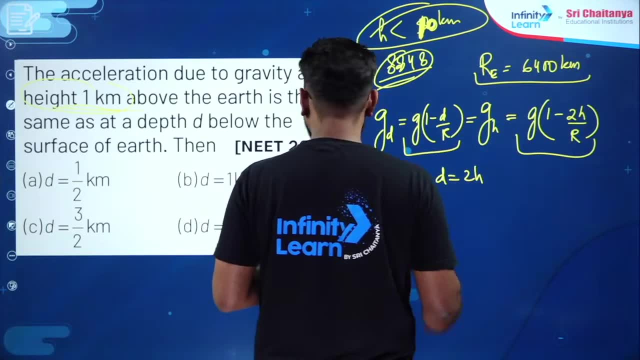 What is this thing? being equal to? Acceleration, to gravity at a depth d Which is g 1 minus d by r. Relate this with this. Clear cut is visible. The value of d is equal to 2 h. H is given as 1 km. 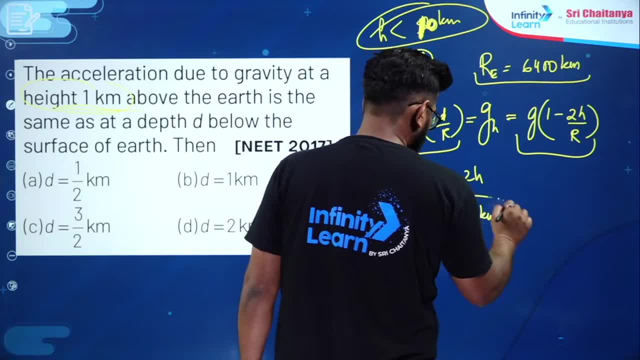 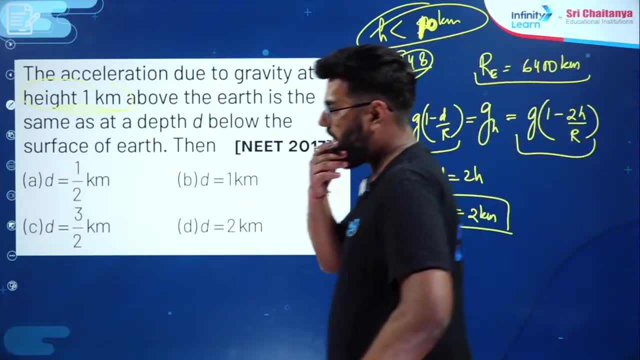 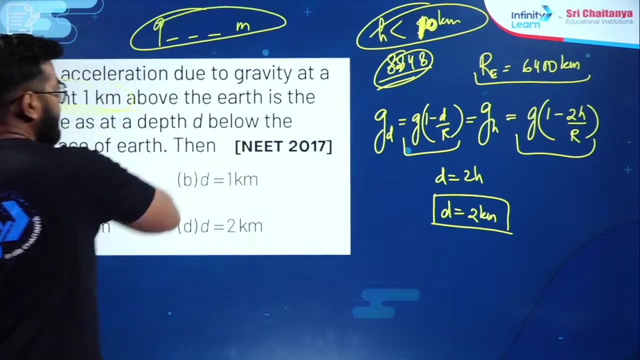 H is given as 1 km, So it is d, 2 km, Although it is very difficult to go 2 km. Mariana Trench is something around 9000.. 9000, some meters, Some 9k meters. 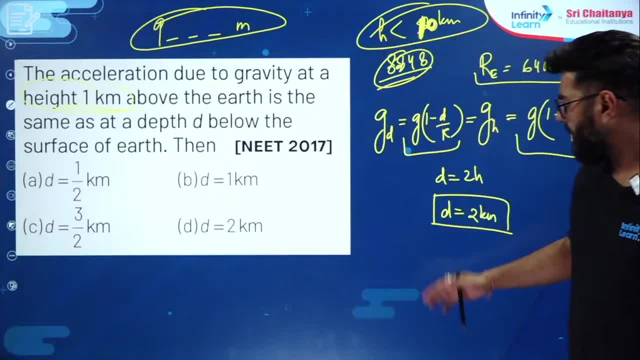 If I am not wrong. If I am not wrong Means the depth of 2 km is not possible. It is not of Mariana Trench, So we are. It is a big thing, Neat. people made good questions. 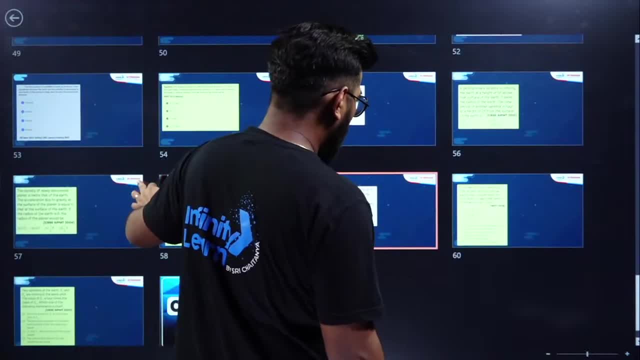 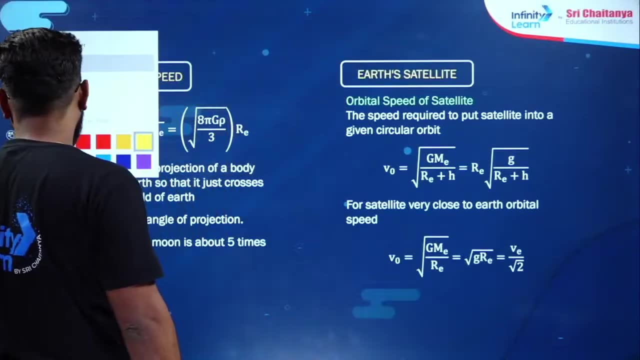 There is no logic. Ok, Come on, Let's move ahead And let's know about satellite Before satellite. one more interesting thing to know, Which is escape speed. Now, what is escape speed? People remember escape velocity. If you remember escape speed, it will look better. 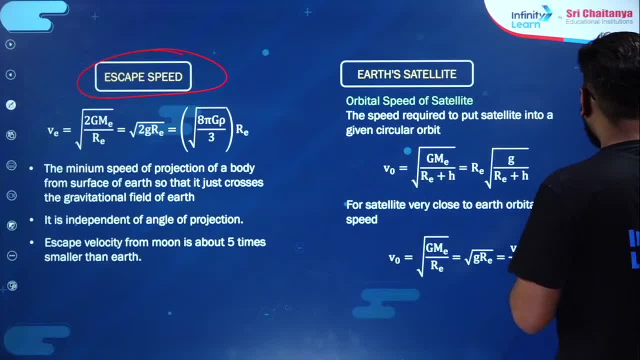 Why? Because there is no sense of direction. Many people think, Sir, if we leave it like this, then it will go. You leave it like this, Leave it like this, Or leave it lying down, Leave it tangentially, There is no problem. 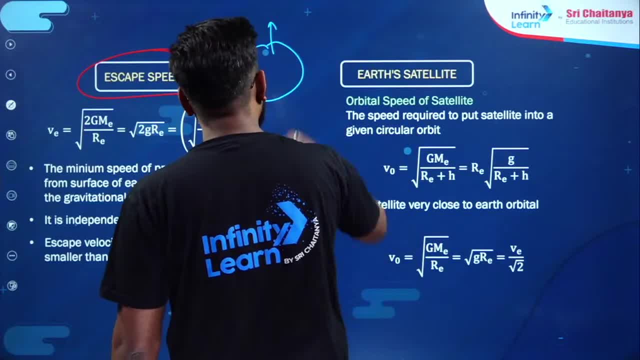 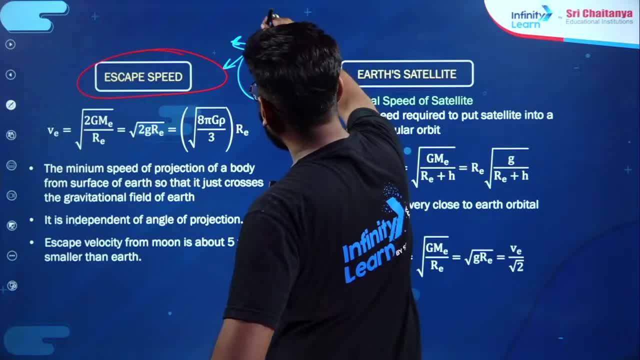 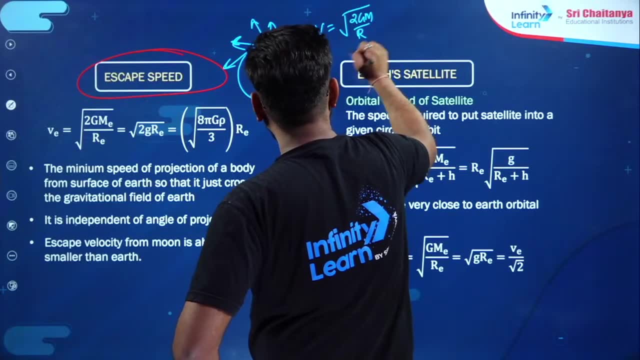 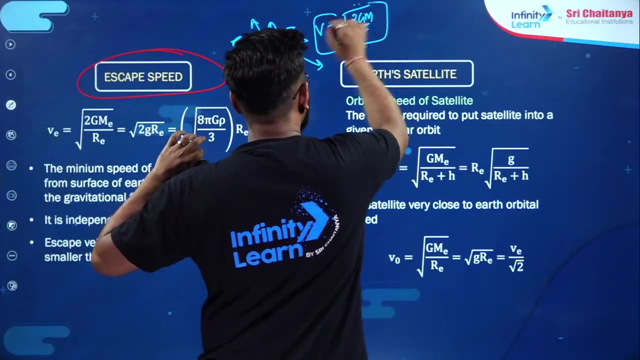 It is clearly fine, But the point is the escape velocity. It will be your under root of 2 times GM upon R, Not even R. Take small R, Small R. Why small R? Because you do not know from which distance you are leaving. 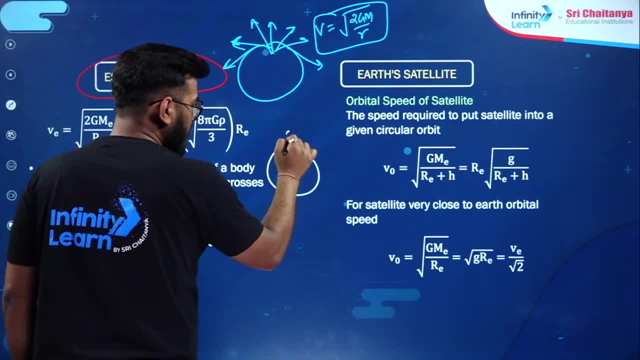 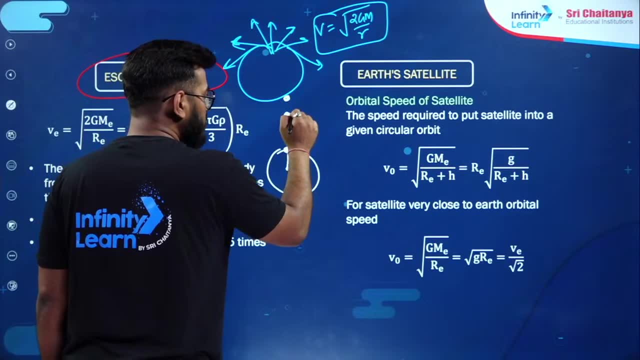 You consider Leave from the surface of the earth, Or leave from here, Or leave from here, Or leave from here. Wherever you are leaving, Remember one thing. So the escape velocity from here will be under root of 2gm upon r. 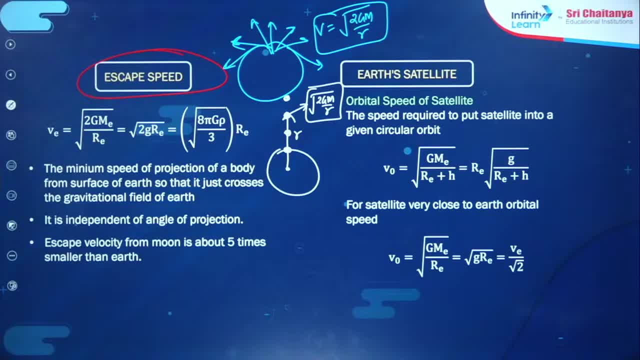 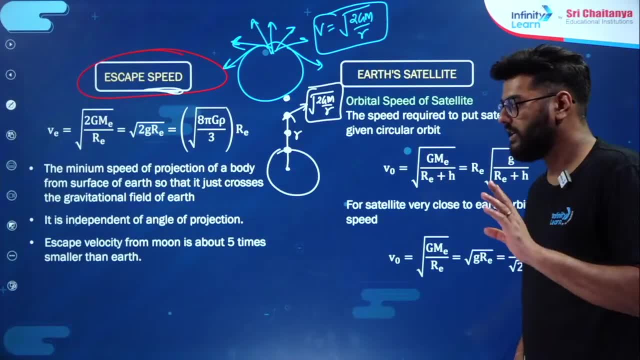 Under root of 2gm upon r, Simple aspect. That's why it is better to understand escape speed. Why? Because there is no involvement of direction. You can project on any direction. Okay, It is independent of the angle of projection. 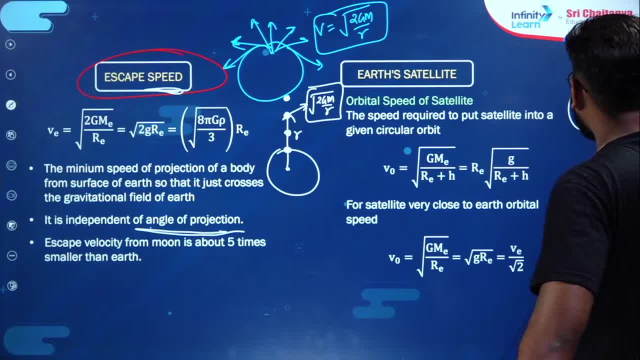 What is orbital speed If we assume that there is a satellite around the earth which is moving in a perfectly circular orbit, Although no one moves in a perfectly circular orbit? Yes, One satellite moves like geostationary satellite, Otherwise normally they don't move. 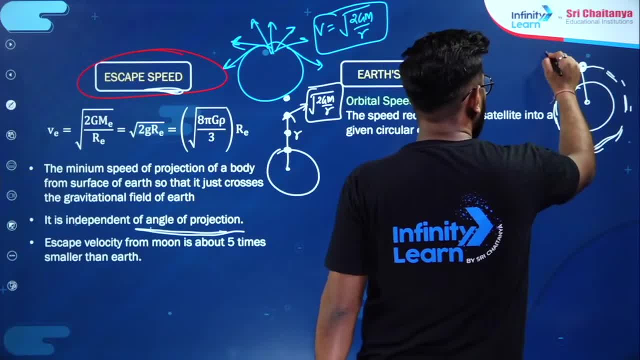 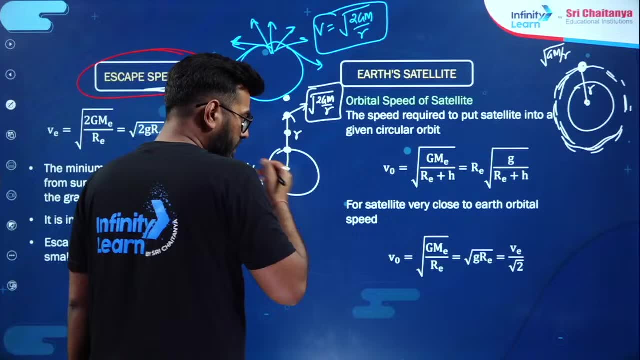 But if it is moving, then its orbital speed will be under root of gm upon r, Where r is the distance from the center of earth to that point. So it will be under root of gm upon r, Okay, Where h will be the radius of earth plus the height h. 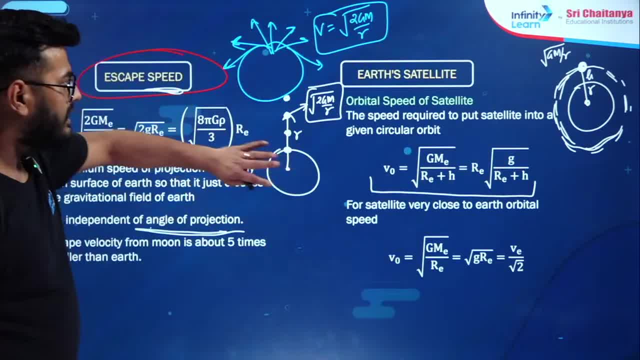 So it will be equal to re plus h. Okay, So you can see at any point, Assume that you are at this point. So at this point escape velocity will be: It will be under root of 2 gm upon r. 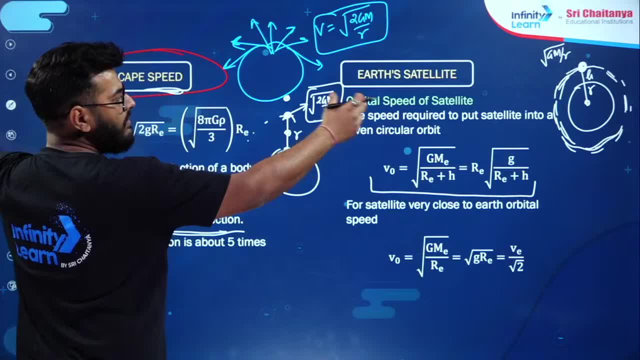 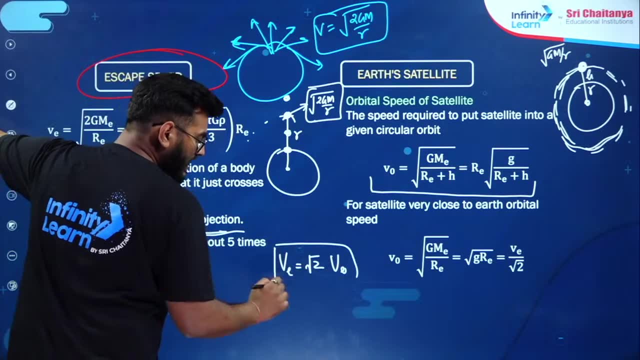 And assume that it is moving in a perfectly circular orbit. So its orbital speed will be under root of gm upon r. So at any point of earth The escape velocity will be always root 2 times orbital velocity. This does not mean that orbital velocity will be there. 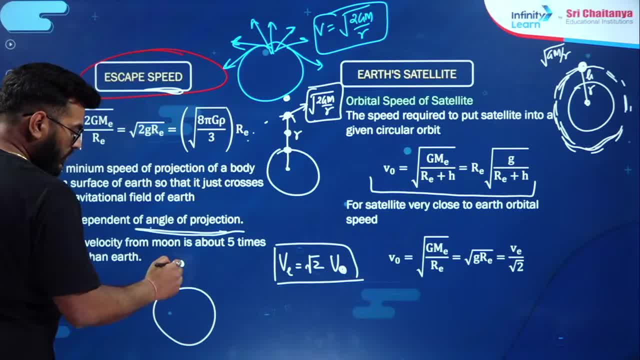 No, it is not necessary. It is possible that you will leave the particle after bringing it here. If you leave it, it will fall down. Orbital will be there when it is stuck to an orbit, That it is moving around, an orbit. 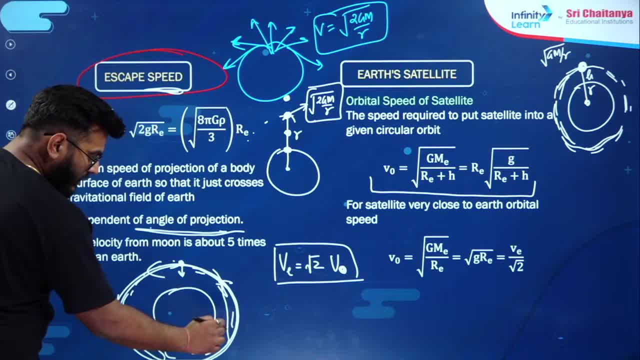 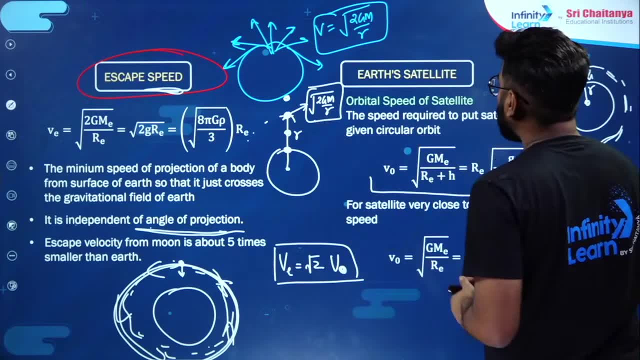 Then the concept will come that orbital speed is there And if it is orbital speed, then at that time escape velocity will be root of 2 times. So if you assume, Let me ask you a question. Let me ask you a question. 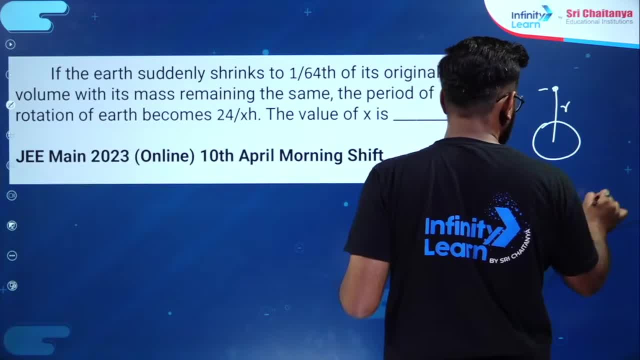 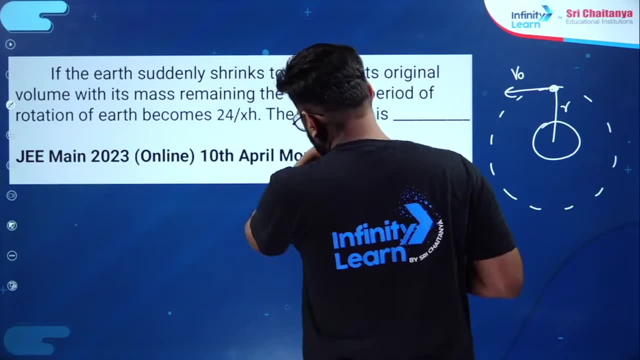 There is a satellite at a distance of r from the earth Which will have an orbital speed: vo. So, from now on, how much extra velocity will you have to give it so that it leaves the earth? Simple thing, sir: How much will it have to give escape velocity which is equal to root of 2 times vo. 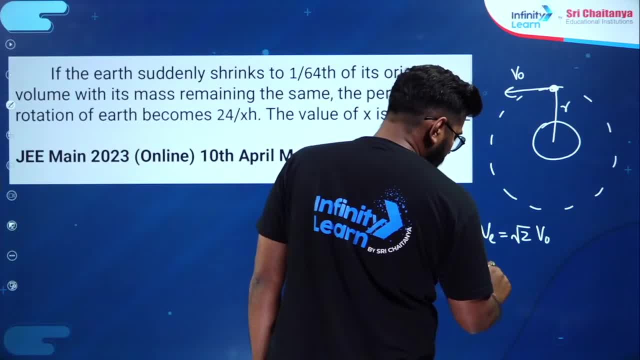 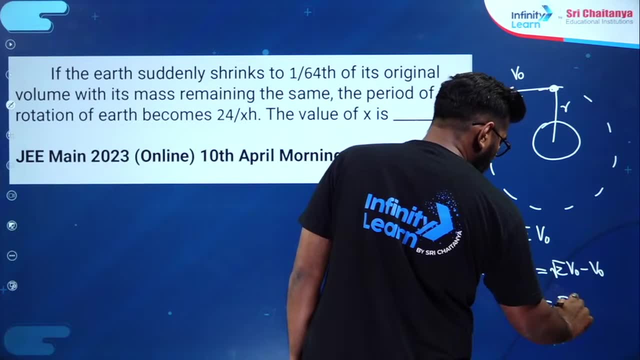 But now it has vo already. So how much extra velocity will you have to give? You will have to give extra velocity: Root 2 vo minus vo. That means root 2 minus 1 into vo. If you give this much extra velocity, then it will work. 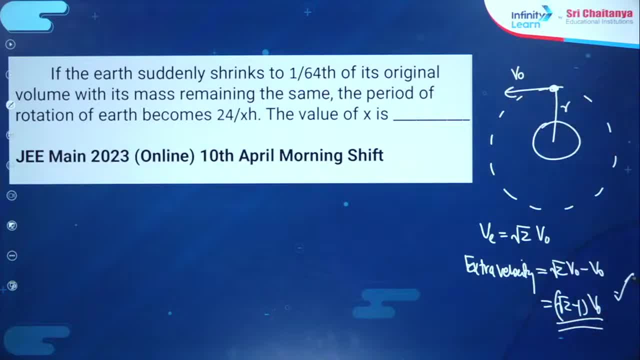 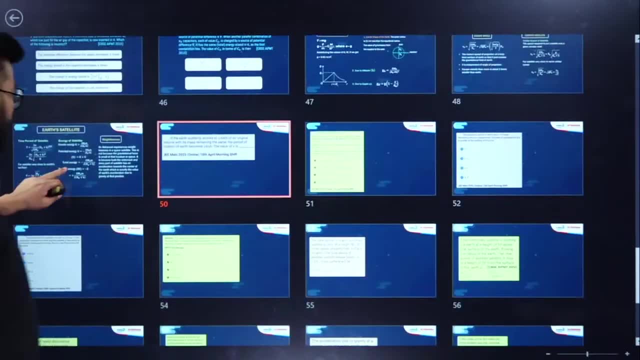 If you give this much extra velocity, then it will work. If you give this much extra velocity, then it will leave you and escape. Where will it go? It will go to infinity. Look at the question. Okay, for this question time period should be known. 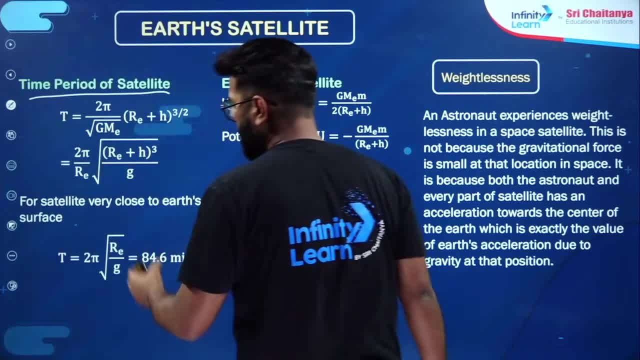 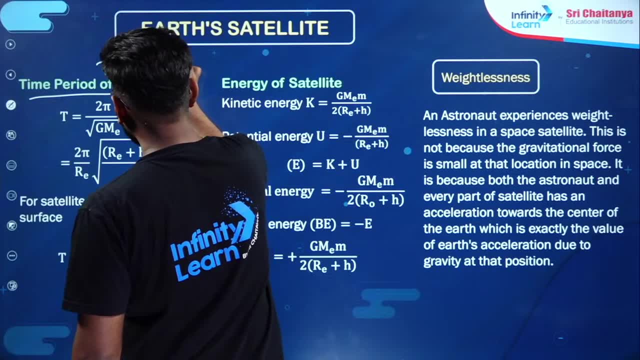 The relation of time period. is this Time period of a satellite, Time period of a satellite? What does it vary on Time period of a satellite? The radius of R is T squared. It is directly proportional to the radius of the hole cube. 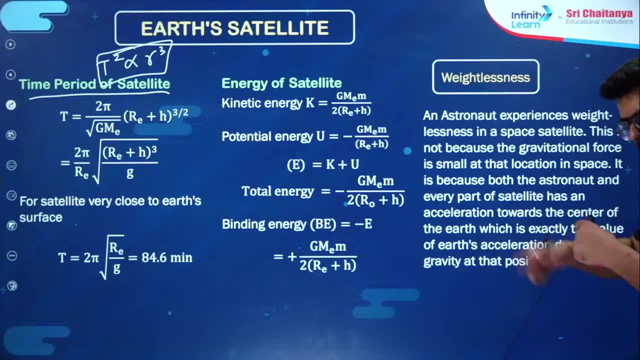 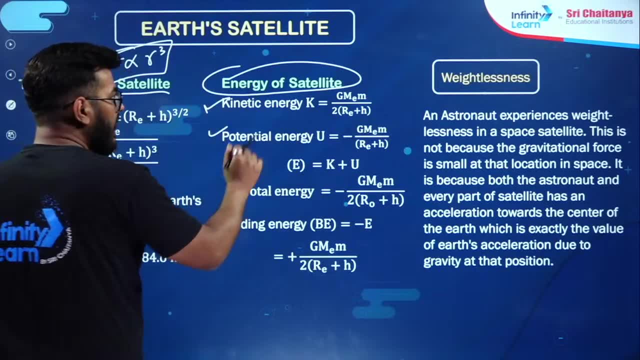 Just like semi-major axis, here it is the radius of the Earth's hole cube If it is moving in circular orbit, And the energy of a satellite is very important. Kinetic energy plus potential energy is made up of the sum. Remember here the value of kinetic energy is half of the value of potential energy. 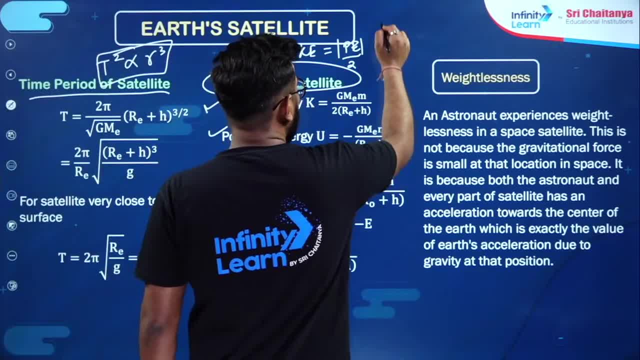 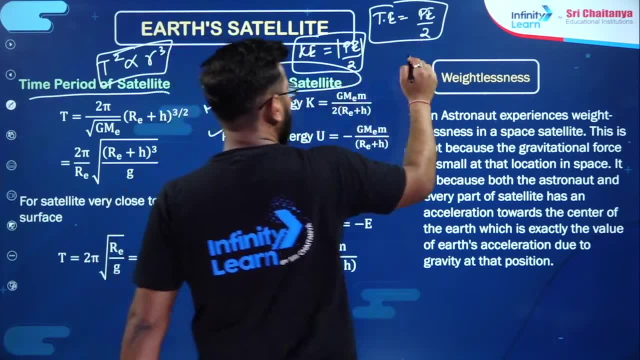 Potential energy is negative, so its value is half Total energy is Potential energy by 2 is equal to the value of the negative sign, Okay, And kinetic energy is equal to the magnitude of the total energy, Not the negative sign. So kinetic energy will be positive. 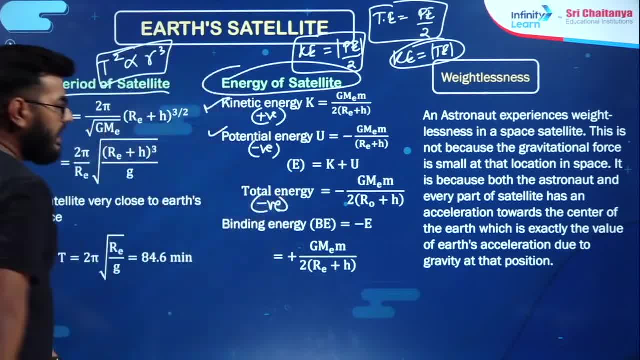 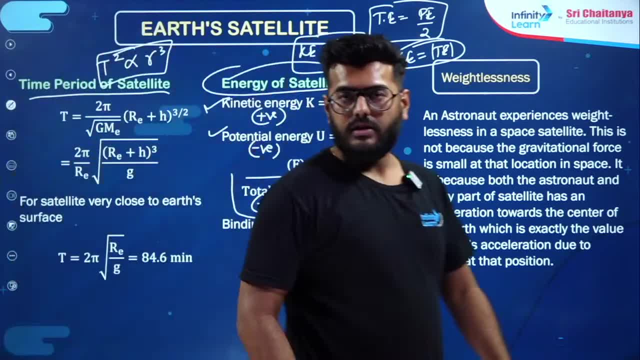 This will be negative And the total energy will also be negative And the relevance of negative total energy is very good If the total energy of any system is negative, Any total. Assume that you are studying with me And the total energy of both of us is negative. 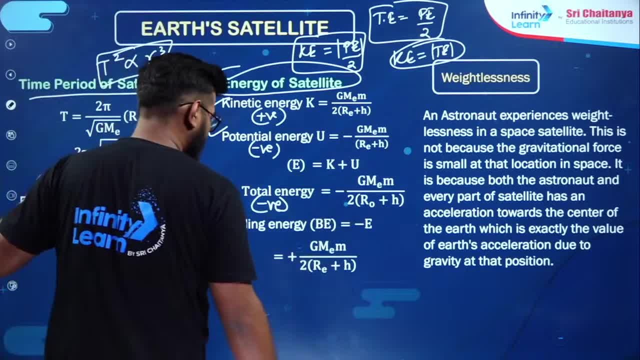 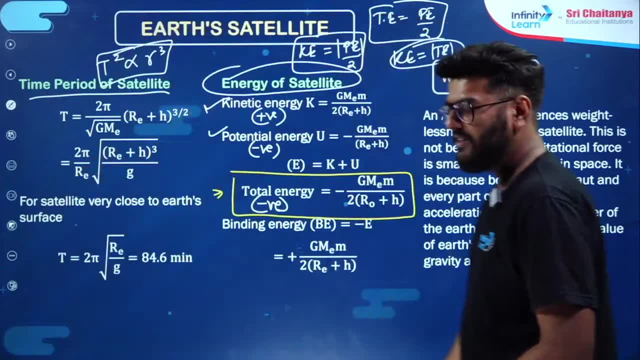 This means that you cannot leave me, But I don't want you to do this. You should take an exam And study with the great masters of mine By going to a good college, But you will need a binding energy for that. 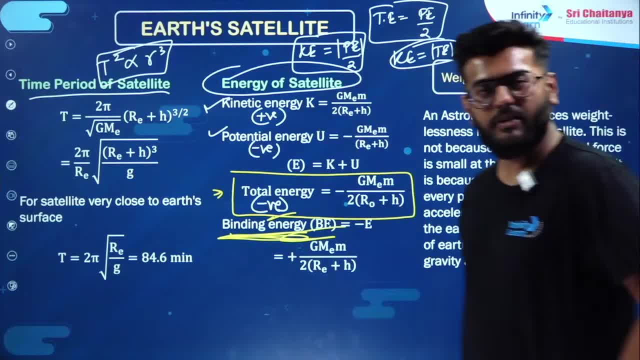 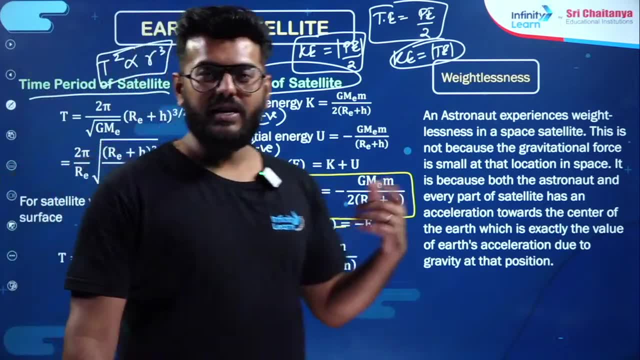 Meaning who will give you the binding energy. You will have to take the exam. It will work as a binding energy And it will make the negative energy between us positive. Only then you can get rid of this Maya trap. Otherwise you will be stuck in this Maya trap. 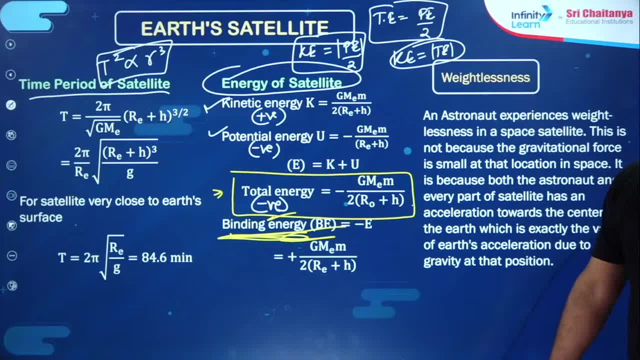 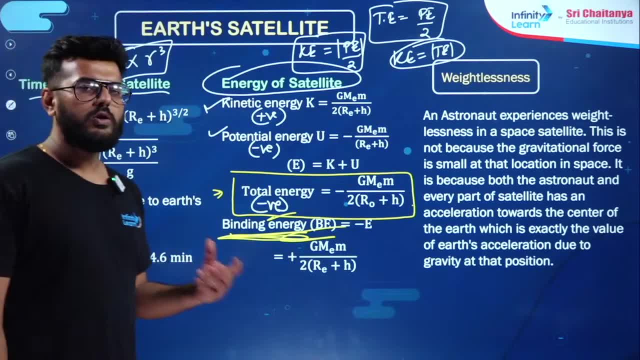 Did you understand anything? So your total energy is negative. Any systems that are bound With any planet or any sun. Even if you talk about the total energy of earth and sun, it is negative. Why is it negative? Because it is a bound system. It cannot leave the earth. Now let's solve it. If earth suddenly shrinks to 164th of its original volume, with its mass remaining the same, the period of rotation of earth becomes 24 by xh. The value of h is: 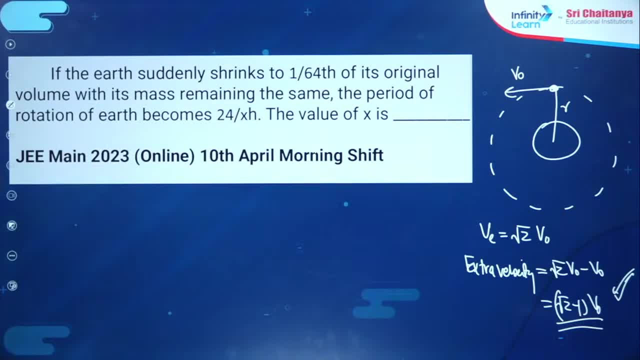 This question is basically of rotational motion. Okay, Let's do it. So what is rotational motion? The earth suddenly shrinks to 1 by 64th of its original volume. So what will happen? What will happen is that 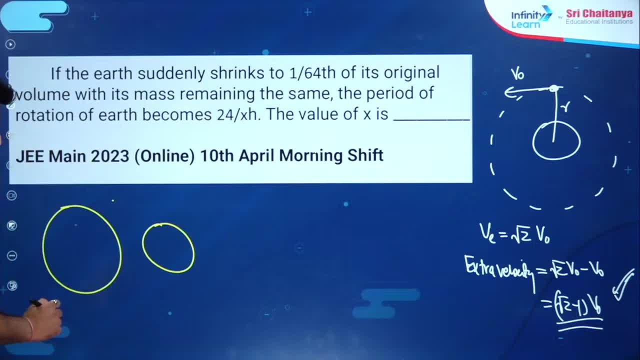 The new volume will be. The earlier volume was 4 by 3 pi capital RQ, Now 4 by 3 pi small rQ, And this is 1 by 64th, Meaning it's 1 by 64th. 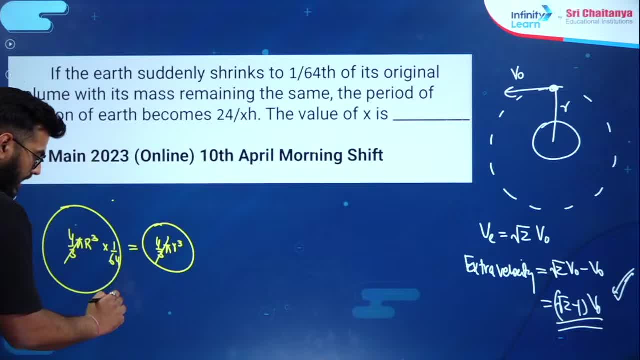 Clear. So we will cancel 4 pi by 4 pi. What will be the value of r? This is 4 cube, right? This is 4 cube, So this will be r by 4.. This is the new radius. 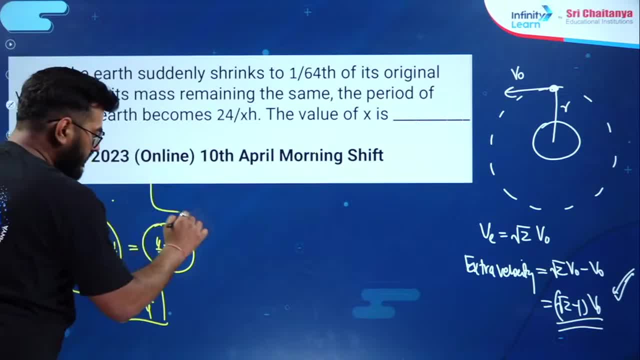 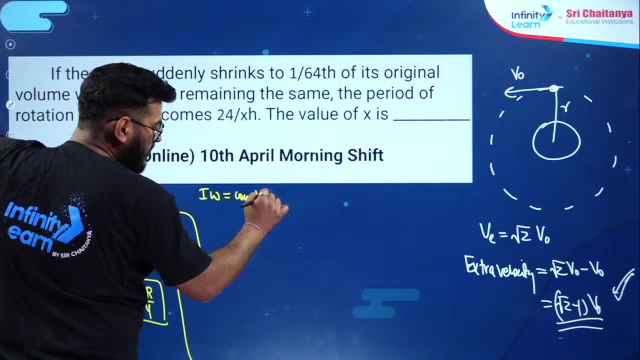 This is the new radius. Okay, Now, this is the new radius. So what is the difference between that? Look, When it shrinks, the angular momentum remains constant. The angular momentum of the rotation of the earth was constant, Okay. 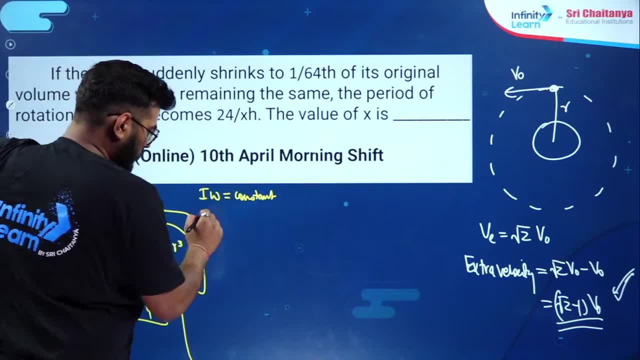 The angular momentum was constant. It used to be like this. Later it will be like this. So how much will be the angular momentum of the earth? Because the earth will behave like a solid sphere, So 2 by 5.. 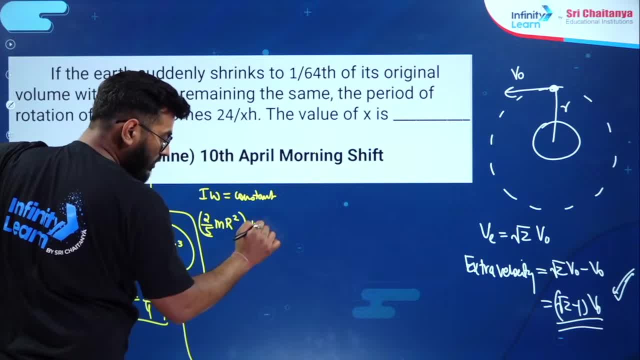 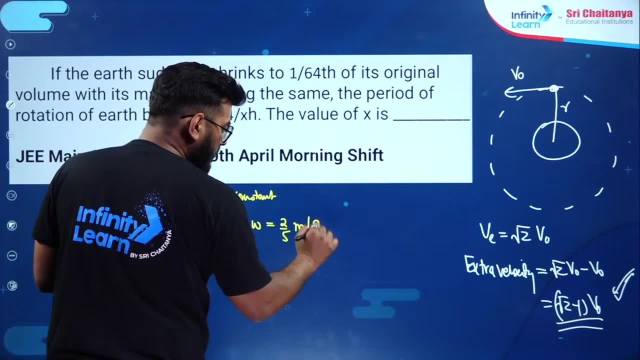 m was earlier r square i into omega, was this? And later? how much will be 2 by 5?? The mass is going to remain the same. The radius is just r by 4.. This is the moment of inertia Into the new omega. 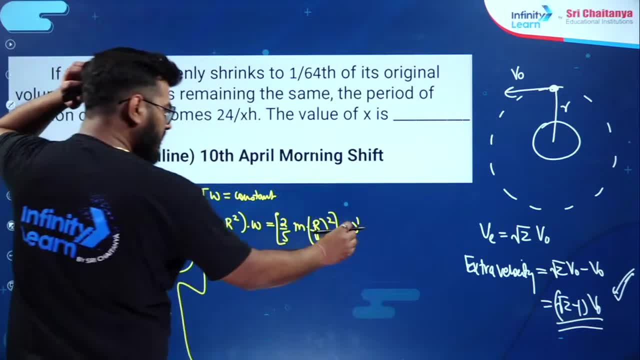 Omega dash. What are you doing, sir? I am doing this because the omega dash is changing. That is why the time period is varying. So 2 by 5m, 2 by 5m. Cancel R square. 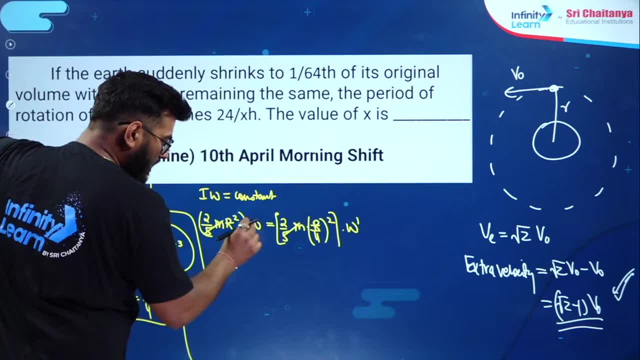 Cancel from r square. Instead of omega, I will write 2 pi upon capital T. Earlier, the time period of the earth was 24. And later how much will be? 1 by 4? whole square, 1 by 16.. 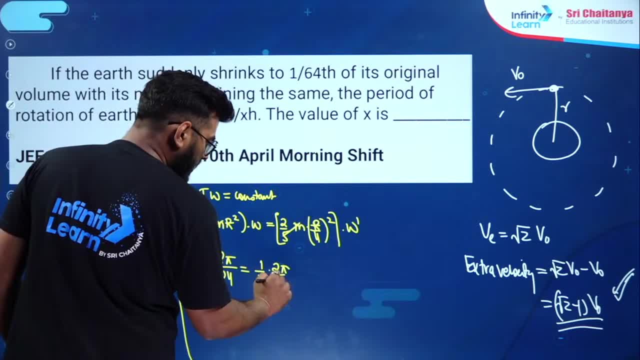 1 by 16.. Into omega dash will be 2 pi upon new time period. T dash: 2 pi, 2 pi. Cancel. How much is the value of T dash 24 by 16.. What did you ask? The value of x, h. 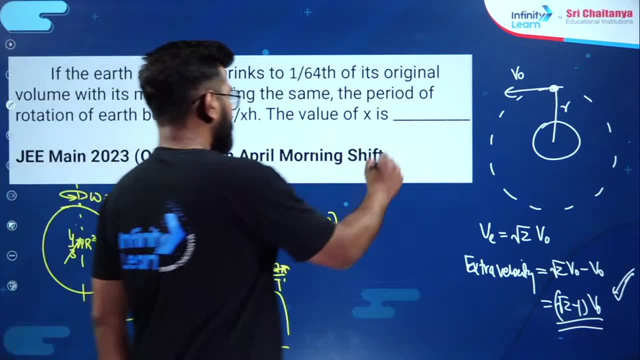 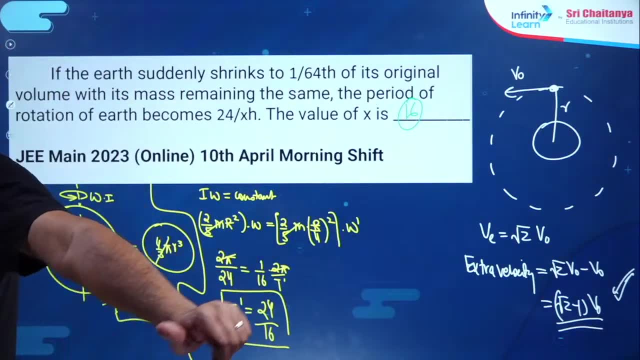 The value of x h. The value of x h. How much 16.. Didn't you understand? Is it clear or not? 8r became r and rho became 64. I don't even mean rho. What is the need of rho, Abhishek? 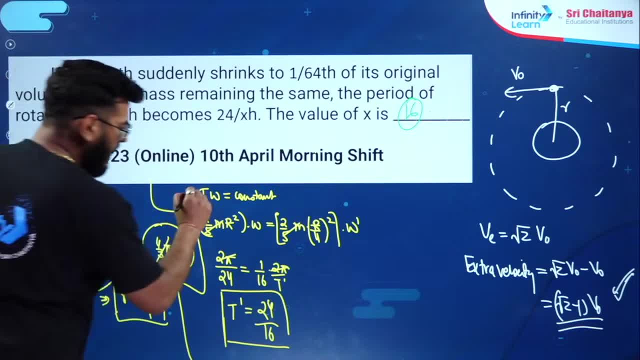 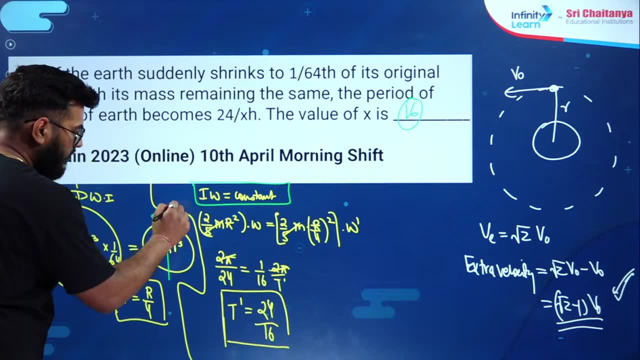 What is the need of rho? There is no need of rho. It is simple logic. Angular momentum will be conserved. Earth is stuck. What will happen if the earth is stuck? It will start moving fast. It will become its new omega dash. 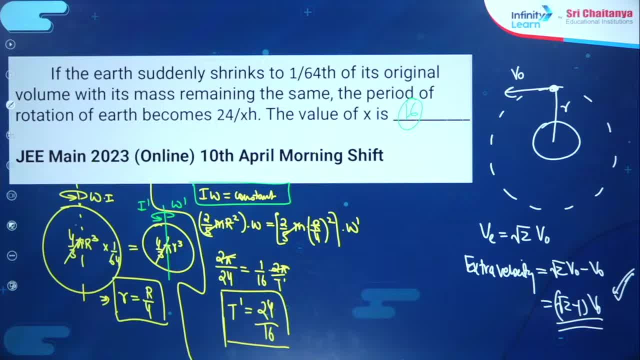 And it will become its new i dash. The concept of conservation of angular momentum is complete. This whole chapter, this question is more motivated than the conservation of angular momentum. It is more motivated. From there you can solve it in a better way. 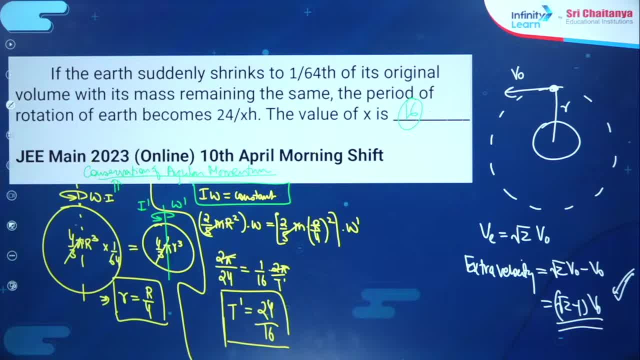 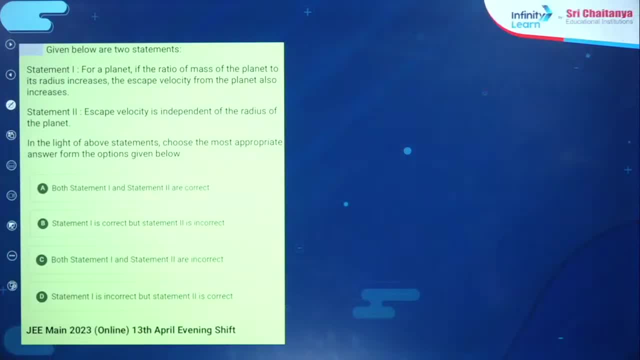 From the conservation of angular momentum. Are you understanding? Is it clear? Okay, Look at the next. For a planet. if the ratio of mass of planet to its radius increases, the escape velocity from the planet also increases. If the ratio of mass of the planet to its radius increases. 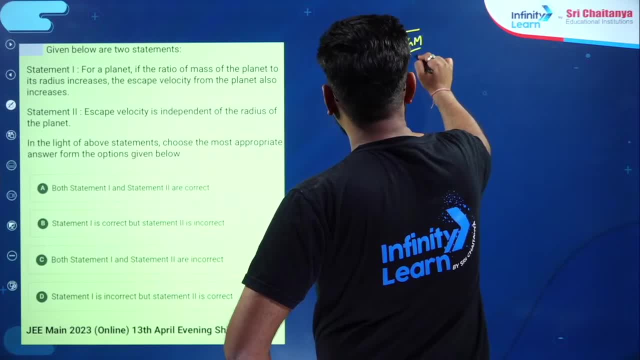 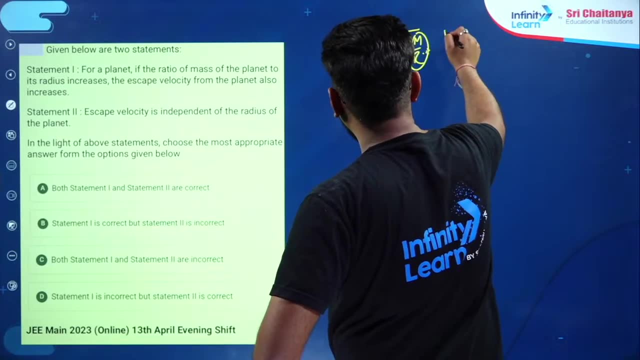 then what is the escape velocity, Sir, under root of 2gm upon r? So if the mass of the planet to its radius increases, if this ratio is increasing, then obviously the escape velocity will also increase. Yes, option number is absolutely correct. 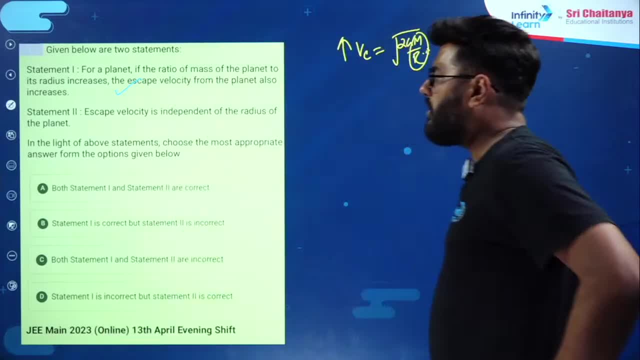 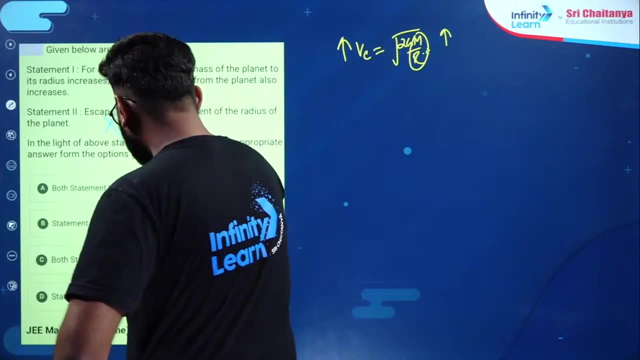 You are absolutely right, sir. Escape velocity is independent of the radius of the planet. No, It depends on the radius. So statement 1 is correct. statement 2 is incorrect. Okay, these questions are very good. The options are not looking good. 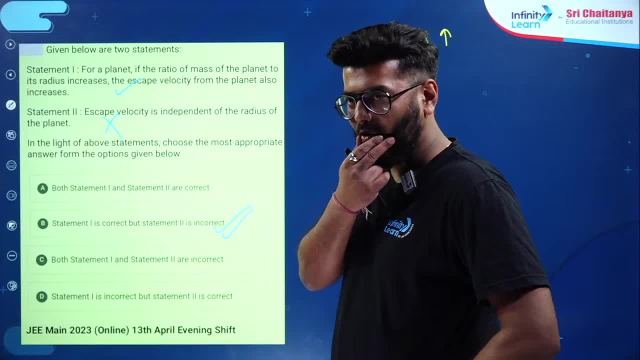 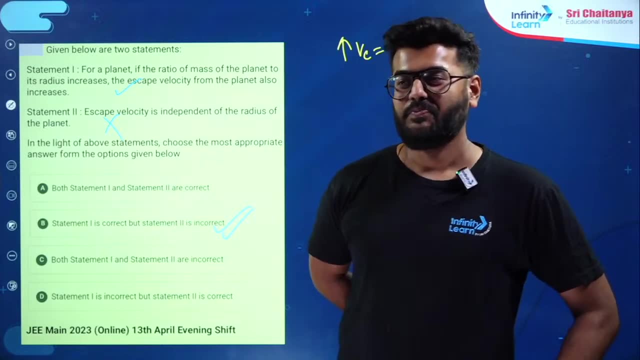 These are very good where one is wrong and the other is right. Either both are right or both are wrong. Those are very scary Where both are right and ask for reasoning. Where they ask for reasoning, Okay. So for them there is a simple trick. 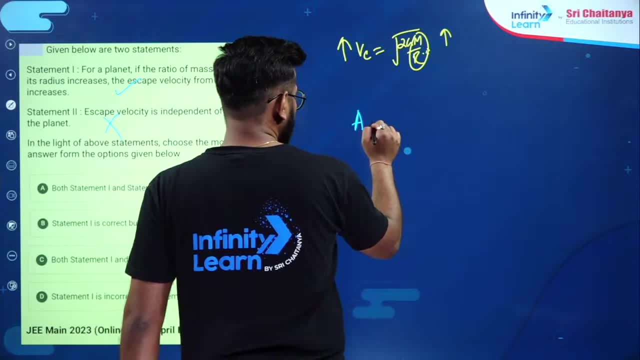 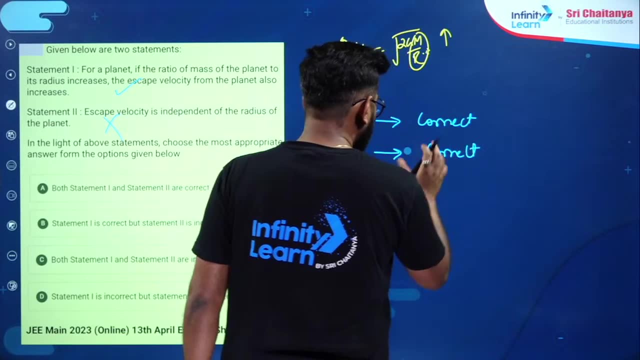 This is not the assertion reason, but the statement one, The assertion reason one where the assertion is also correct And the reason is also correct, And just tell me whether it is the correct explanation or not. Put a connector between them Because or since. 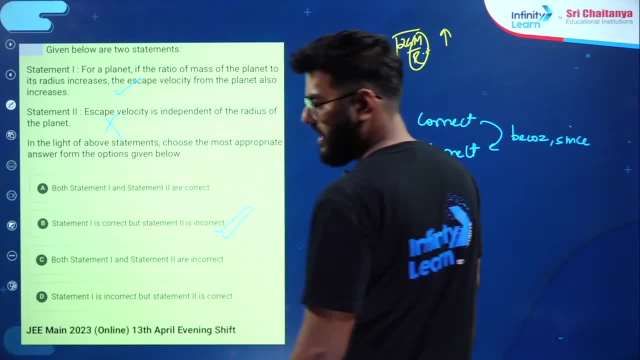 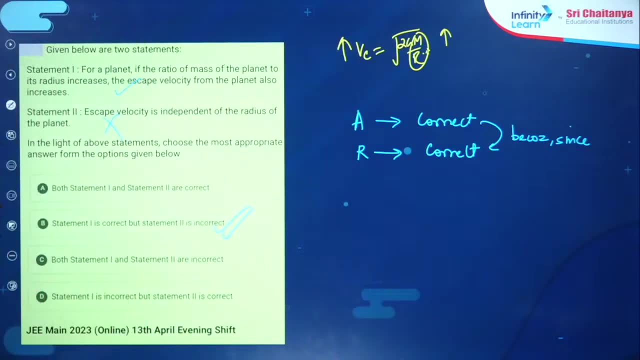 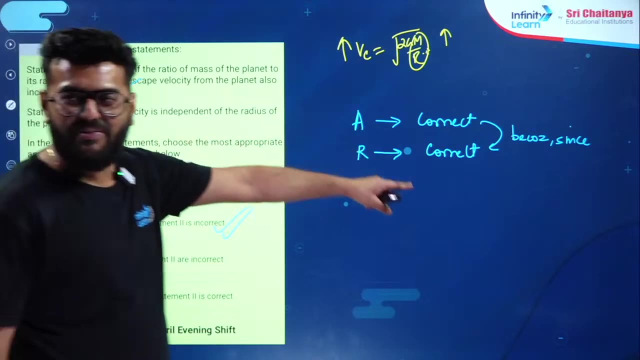 Okay, do you understand? Put a connector between them. Write, because If it is sitting correctly, then it is correct. Okay, Although he also knows he also has such clever things. Do you know where it is correct? It fits in bio-bio very well. 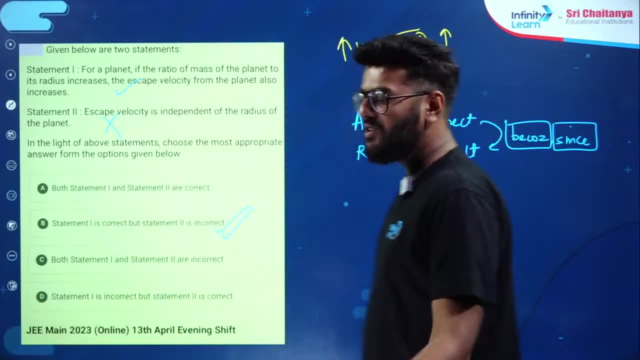 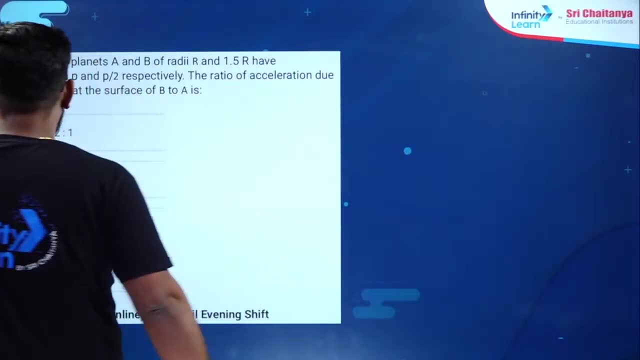 It doesn't fit in physics. The concept should come in physics. If the concept doesn't come, then because, since these are English jokes, they fit in bio-bio, they don't fit in physics. Okay, next thing: Two planets, A and B of radii, R and 5.5R, are densities rho and rho by 2.. 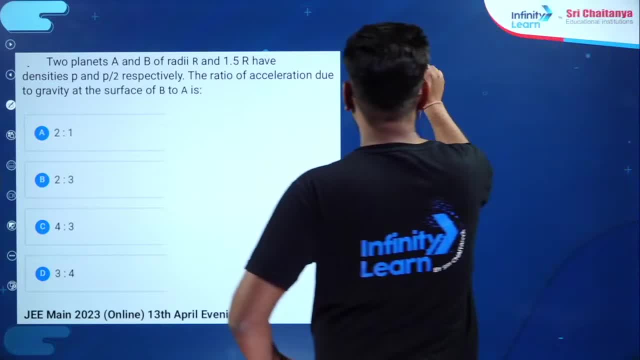 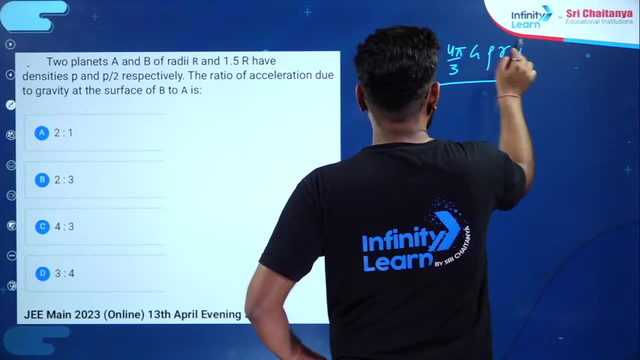 The radius of acceleration due to gravity at the surface of B. Now just tell me: the value of G is 4, pi by 3, G, rho, R, It is depending on this Right. So two planets, A and B, of radii, this much and density, rho and rho by 2.. 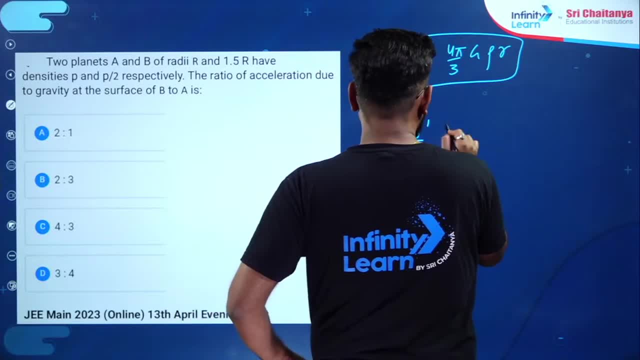 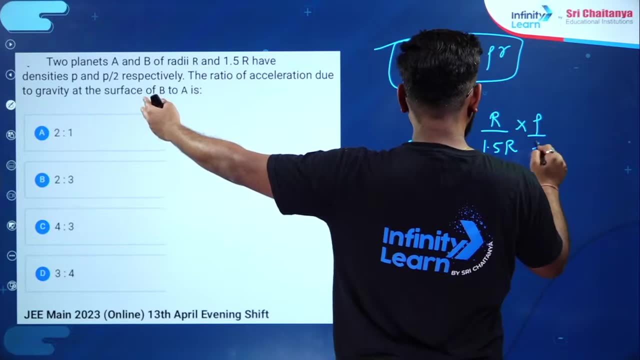 Ratio of acceleration. See how much the value of G1 is to G2 will come. G1 is to G2 will come. R1 is R and the second is 1.5R And the density of the first one is rho and the second is rho by 2.. 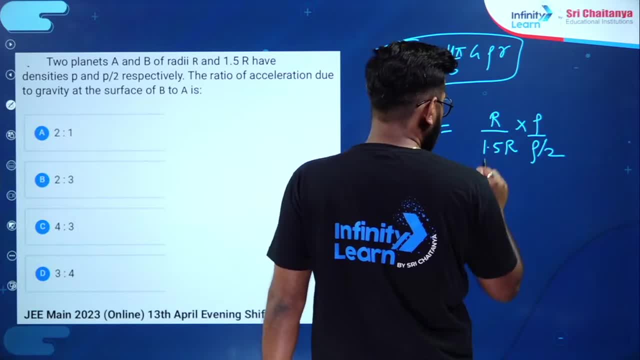 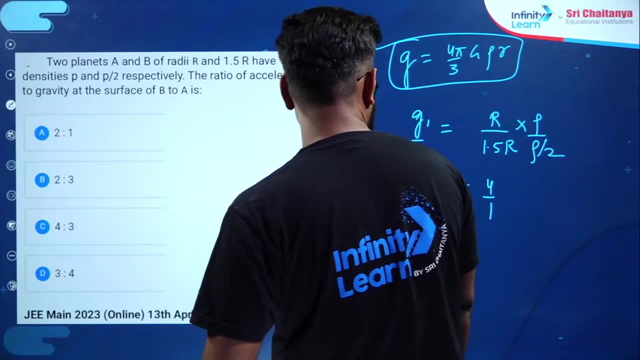 So this rho by 2 will go up. This 3 by 2 rho by 2.. So 4.. The answer is: 4 is to 1.. 4 is to 1.. No, No, Sorry. 4 is to 3.. 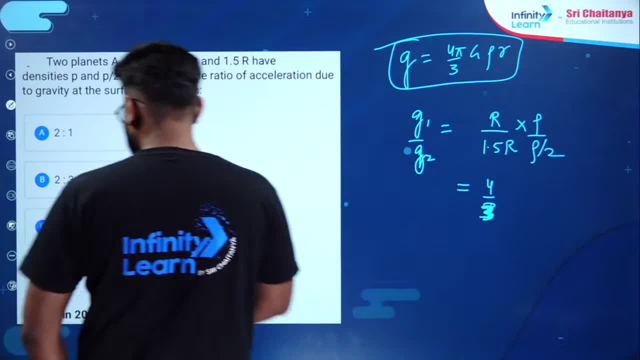 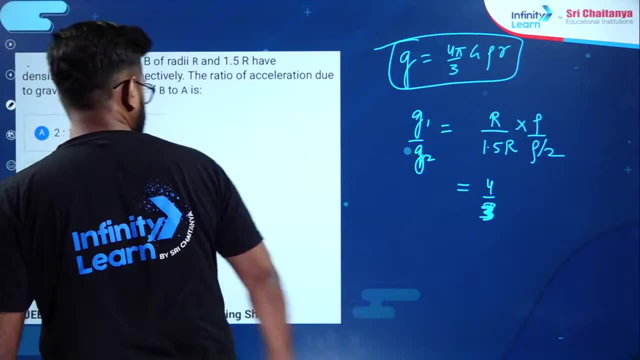 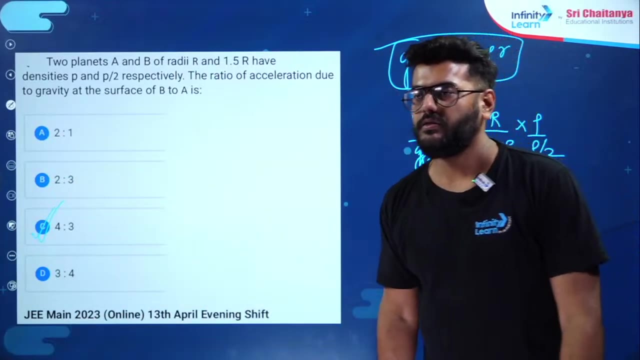 4 is to 3.. Because here 3 will also come. 4 is to 3.. Option number C. Option number C: 4 is to 3.. It is in option number C. Okay, Clear, Let's go. 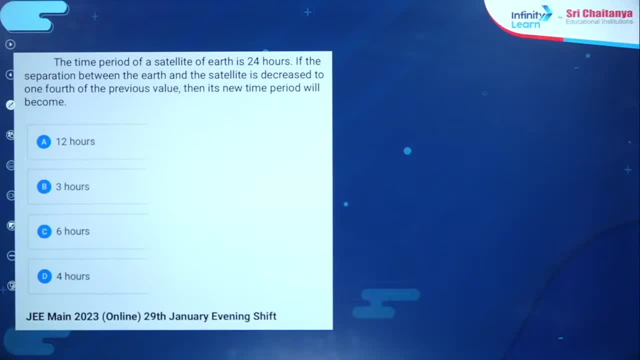 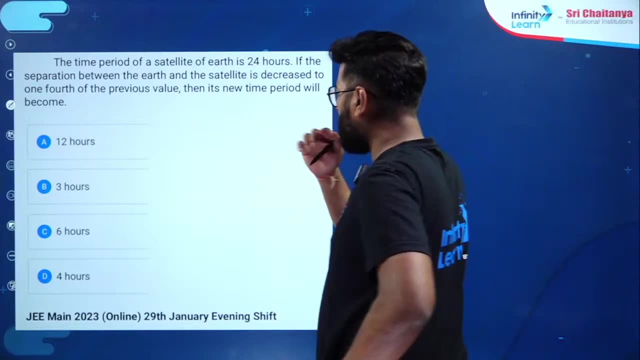 Time period of a satellite is 24 hours. if the separation between Earth and satellite is decreased to one fourth, If, If, If. If the separation between Earth and satellite is decreased to one fourth of the previous value, Then its new time period will be. 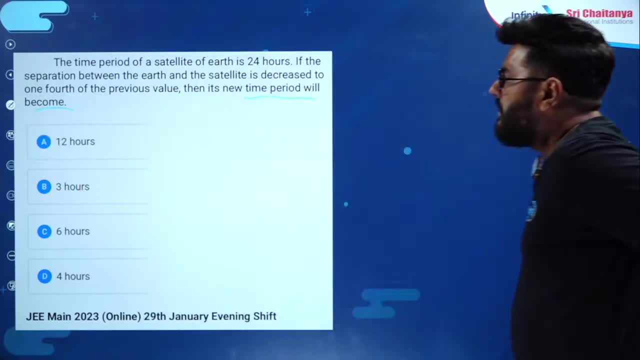 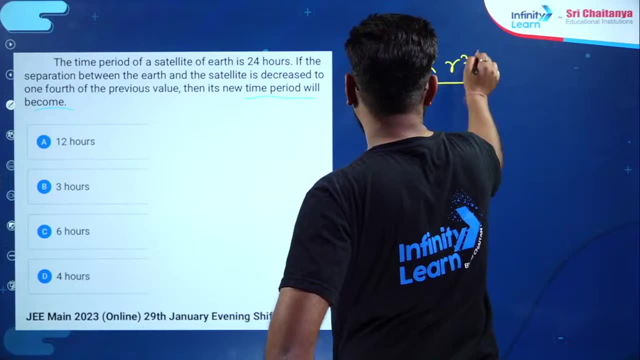 How much will be the time period? How much will be the new time period if the distance is reduced to one fourth? It is a simple clause. T square is directly proportional to R cube. I hope you can do it easily with this. Direct formula is also a question. 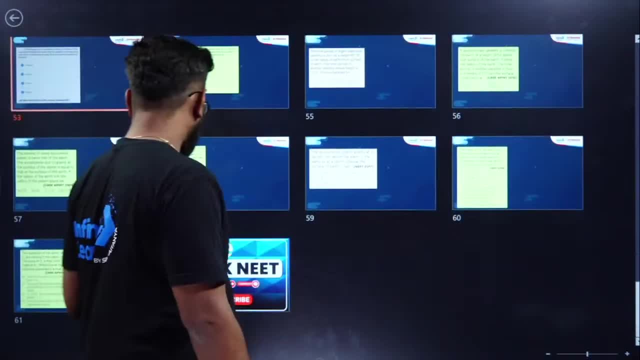 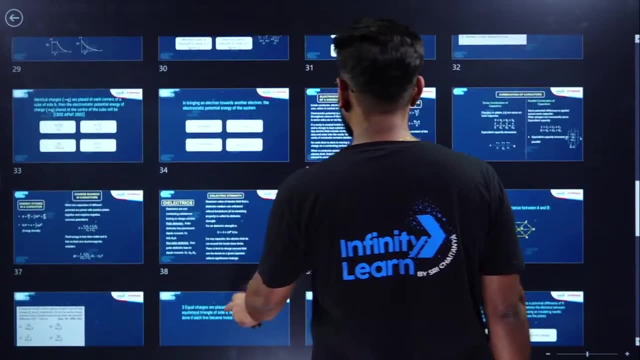 So there is not much issue to be solved in this. Okay, So I hope you got some clarity from all this. Now let's move on to our final individual element, which is our capacitor. So let's look at the properties of the conductor and the capacitor. 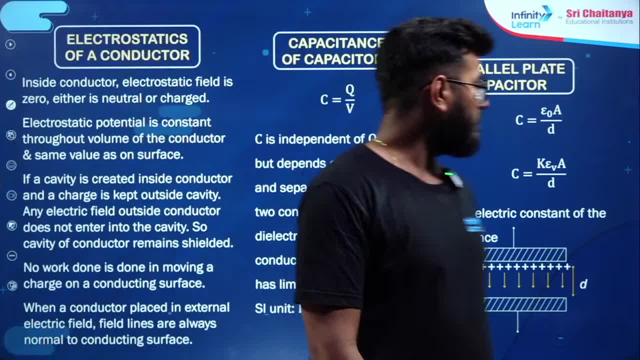 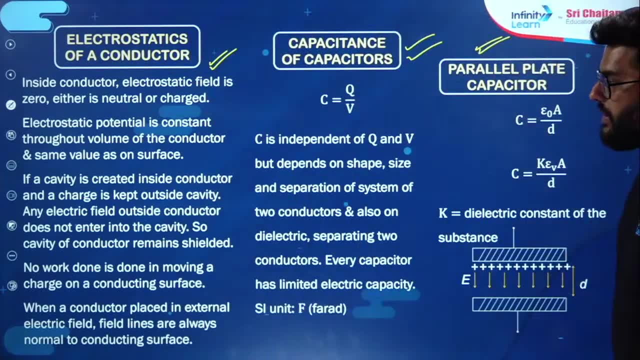 Six hours. Very good, Rakesh, Very good. Now let's talk about the capacitor, which is an individual topic. Capacitor, which is also very important. Okay, So here in front of you, the properties of the conductor are kept, that there is equal potential. 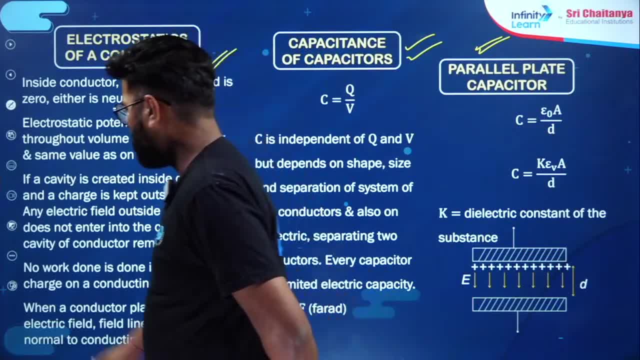 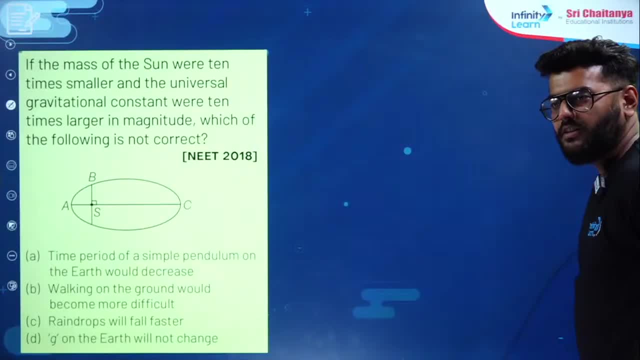 That question was Kepler. Which Kepler was it? Will you be saying this one, This one, Neat 2018?? This is not a question of Kepler. Do it, Solve it. Solve it and tell me what the answer is. If mass of Sun were ten times smaller and the universal gravitational constant were ten times larger in magnitude, which of the following is not correct? 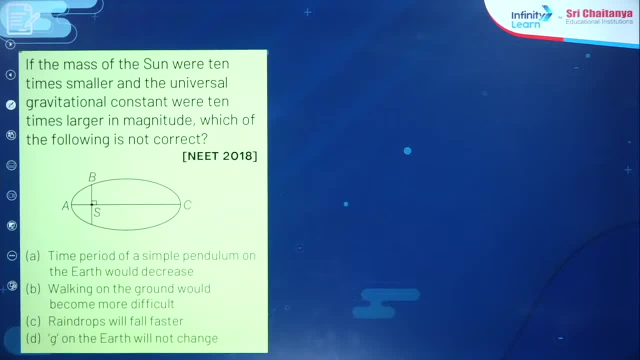 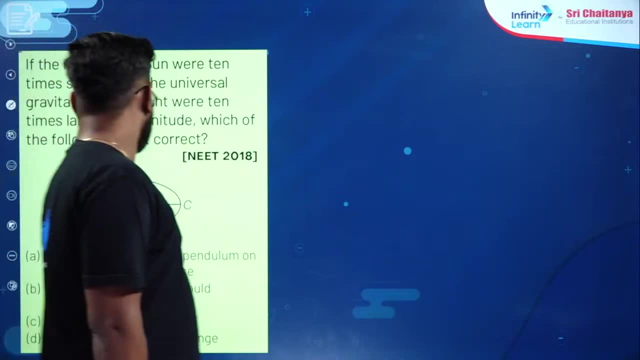 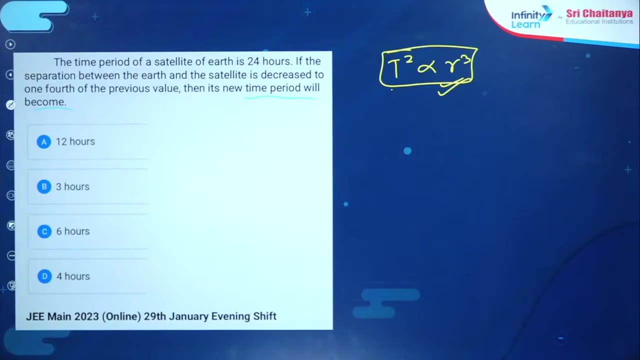 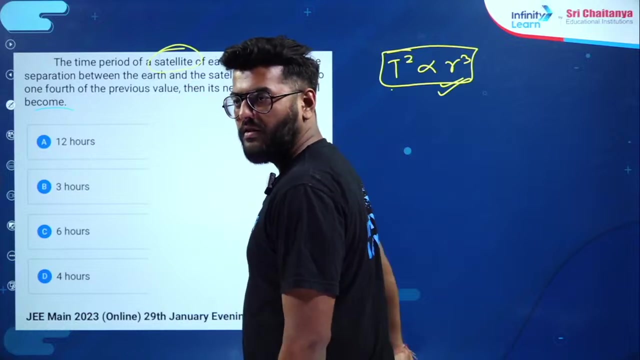 Which of these is not correct? This one, This one? No, it is not of Kepler. You are talking about the satellite, You are talking about the satellite. Satellite is 24 hours. This is the case of geostationary satellite. 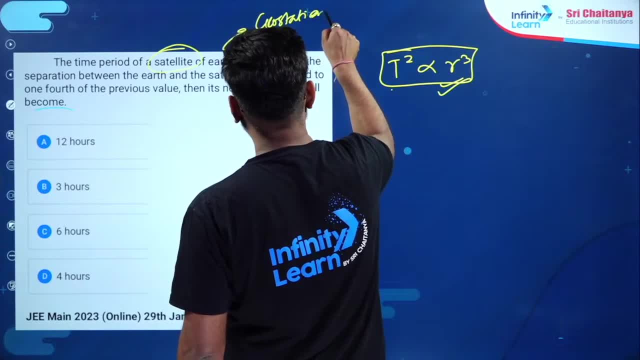 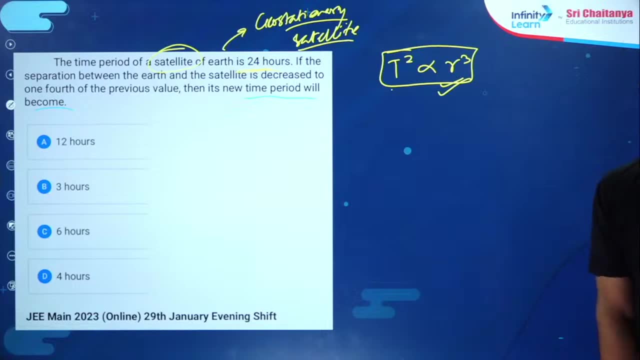 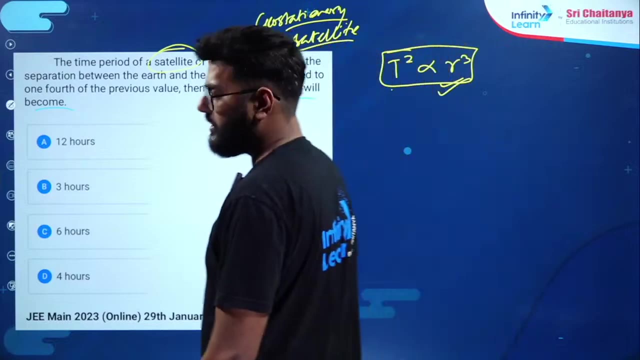 Kepler will come to the planet. Oh brother, Kepler comes to the planet. The law of time period is fine, It will remain the same. It will remain the same, But it comes in satellite motion. Is it clear? You will do it. 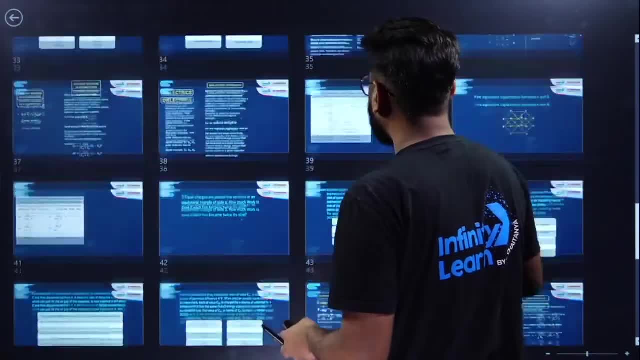 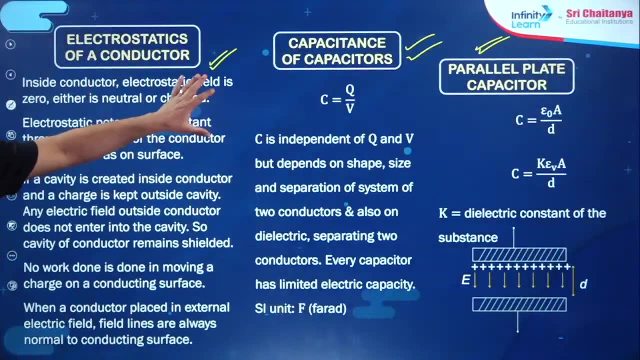 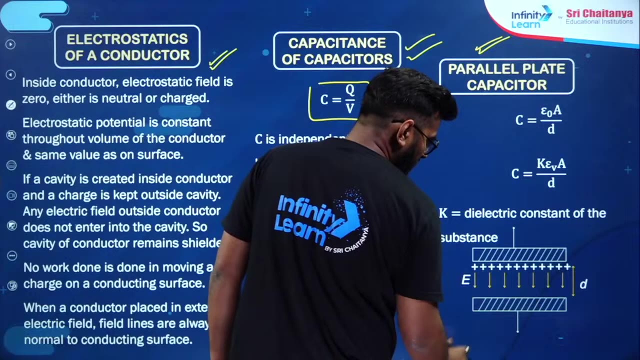 That question does not have so much difficulty. I have already done that. I am going on the capacitor. Capacitor is a good question. So capacitor is a charge conducting plate in which an electric field line will remain in between Established. here is positive and here is negative. 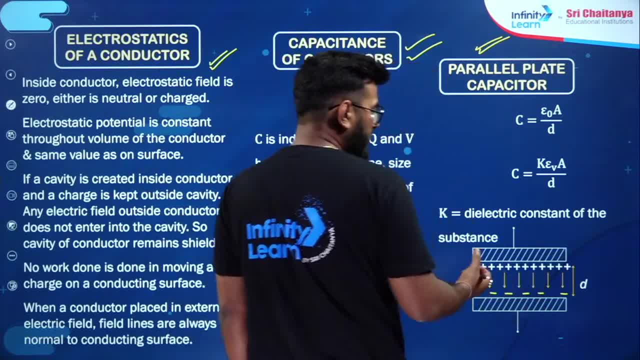 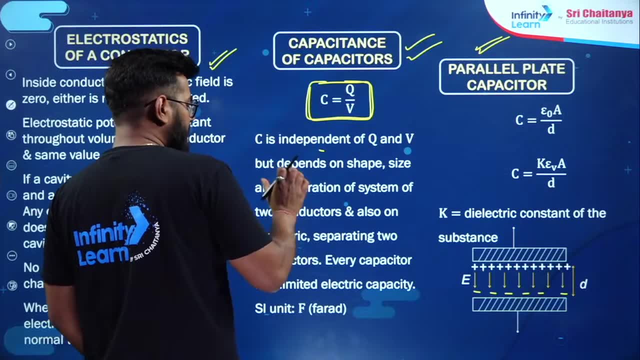 So the electric field, So the electric field lines will not go. Energy is stored in them And the main work of the capacitor is energy storage. Q is equal to Cv, Where C is called capacitance of the circuit And the value of C is A epsilon naught by D. 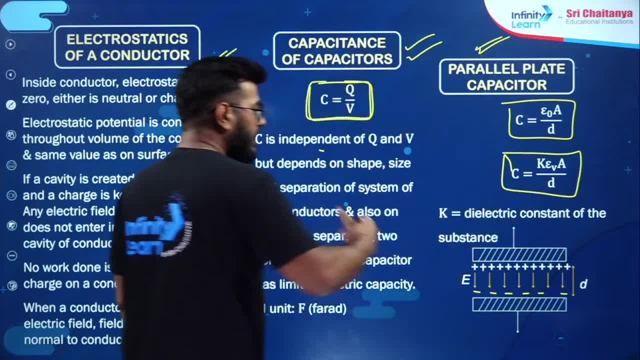 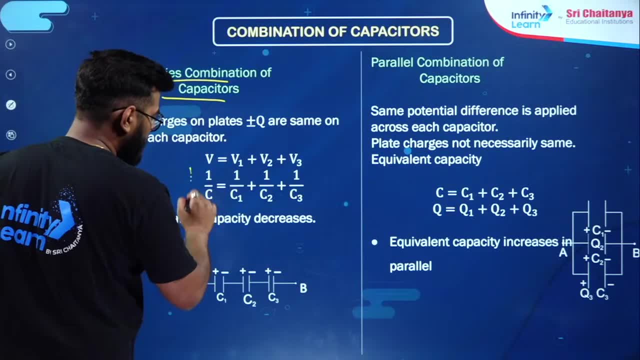 If any dielectric is put in the middle, then Ka epsilon naught by D. We will see the case of dielectric further now, Series parallel combination of capacitors. So series combination is attached in the same way as parallel resistors are attached. 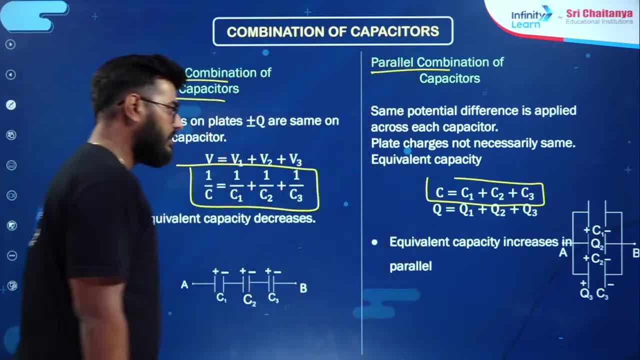 And parallel combination is attached in such a way that in series there is a combination of resistors. In parallel, the charges remain the same, Potentials are different. In parallel, the charges will remain different and the potential will remain the same. 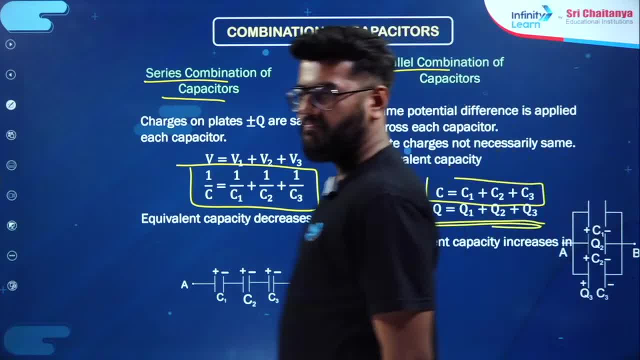 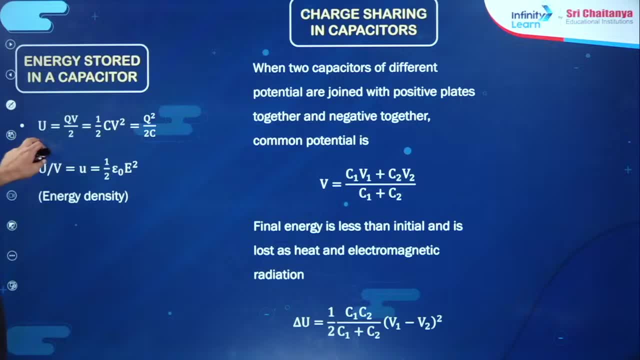 And in series. the charges will remain the same on each capacitor. And what will be different? Potential will be different. Then the energy stored in a capacitor is half Q square by C And the energy density is half epsilon naught V square. 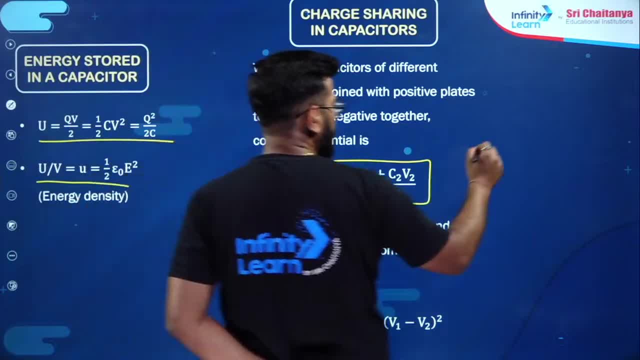 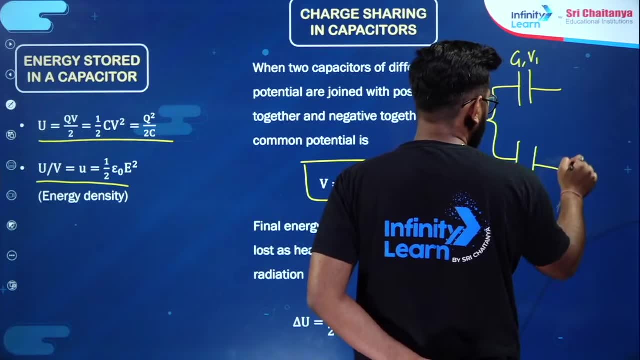 This is a very important question: The charge sharing that happens. Suppose I have taken two capacitors: One capacitor is C and its across potential difference is V, And I have taken the other four capacitors, whose capacitor is C2 and its potential difference is V2.. 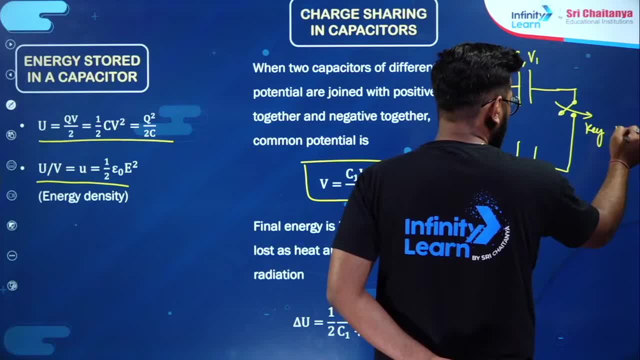 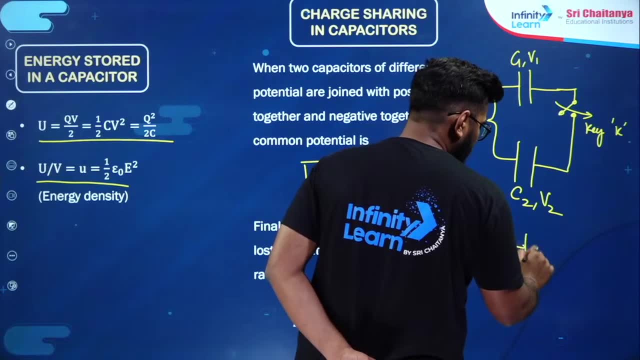 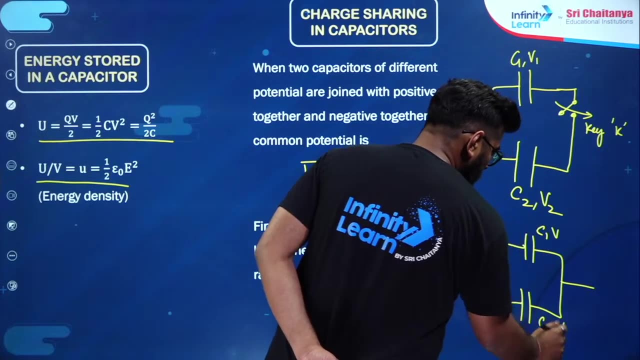 As soon as I close this key K, then the simple thing will happen: The charge sharing will happen, And until the final potential is not the same across the two, until then the charge sharing will continue. The final potential that will remain is important. 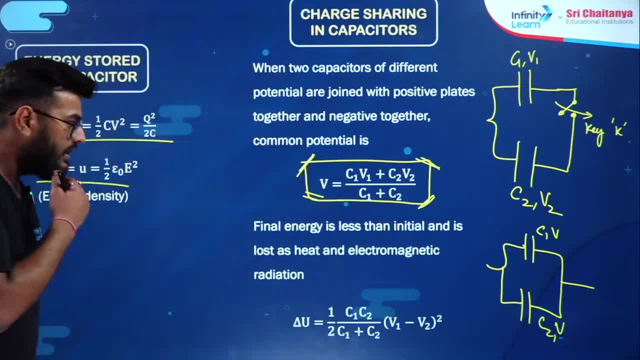 C1, V1 plus C2, V2 upon C1 plus C2.. One is this and the other is the energy loss. What is the value of that Half of C1, C2 upon C1 plus C2, V1 minus V2, whole square. 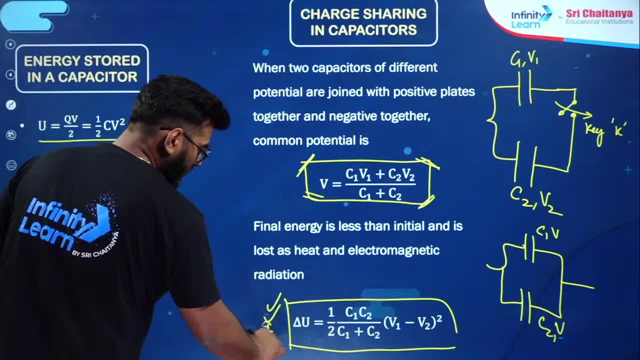 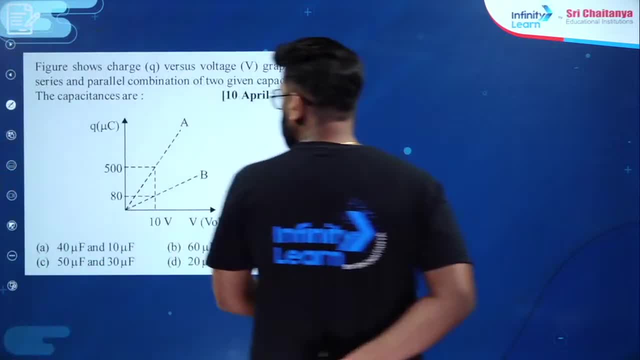 So you have to remember this. You have to remember this. This is important. You have to remember this. This is important. You will remember directly. There are many questions. Let's see the question first. Figure shows charge Q versus voltage V4 series and parallel combination of two given capacitors. 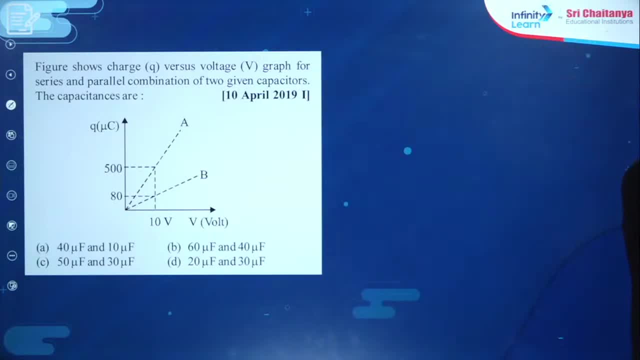 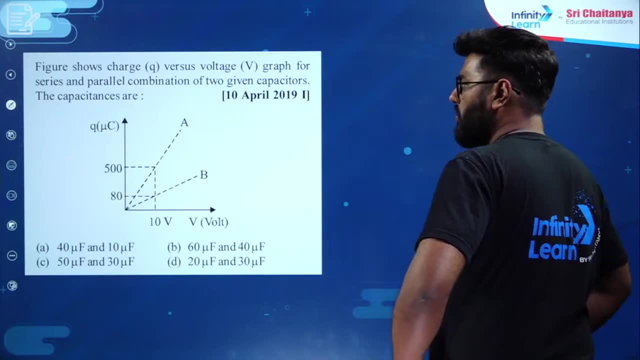 The capacitance are. This is the question of JEE April 2019.. Look, here in front of you, the Q versus V graph is given for the series of parallel combination of two capacitors. Now look at it carefully. First, look at it carefully. 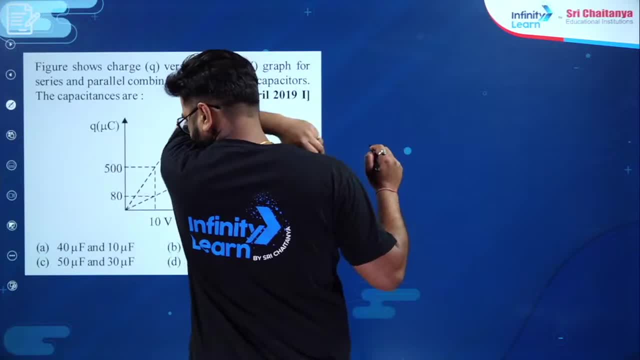 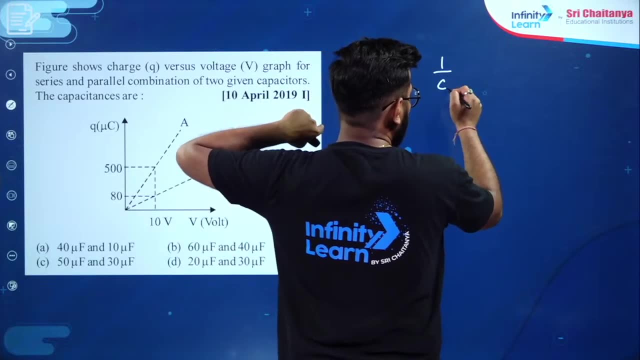 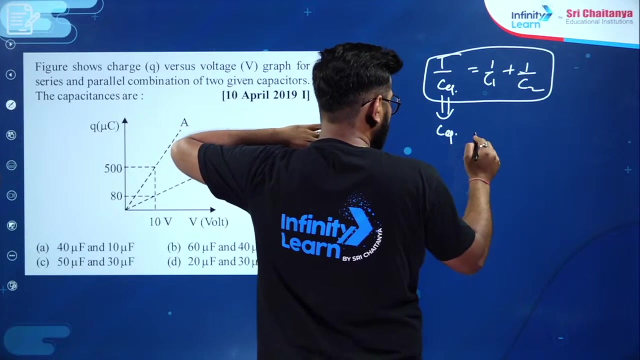 Whenever the capacitors- not only the capacitors, even the resistors, whenever your resistors are connected in this way, 1 upon C equivalent equals to 1 upon C1 plus 1 upon C2.. The C equivalent in this is always lesser than the least. 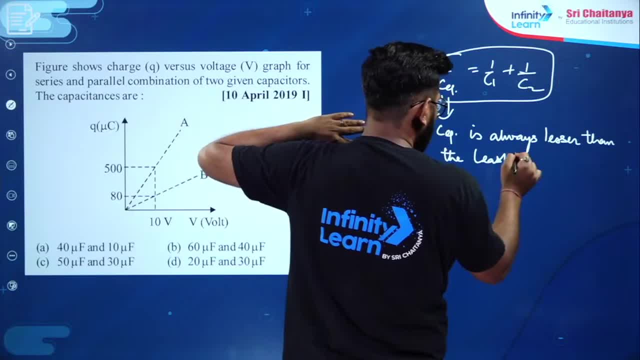 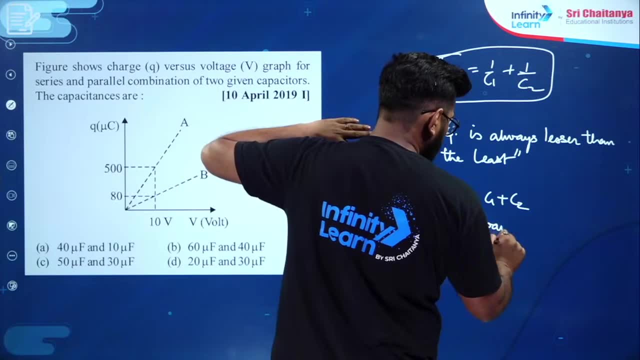 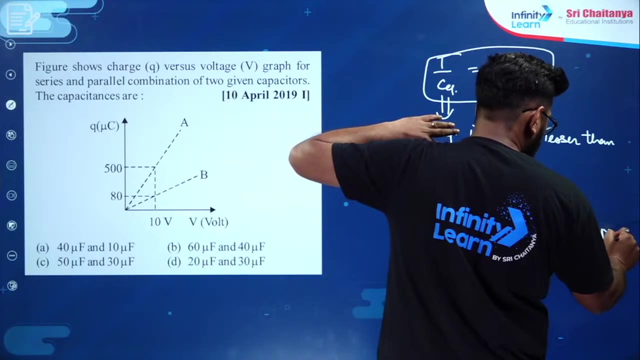 It is always lesser than the least. Always remember this thing. And whenever they are connected like this, C equivalent equals to C1 plus C2. So it will be always greater than the max value. The C equivalent will be greater than the max value. 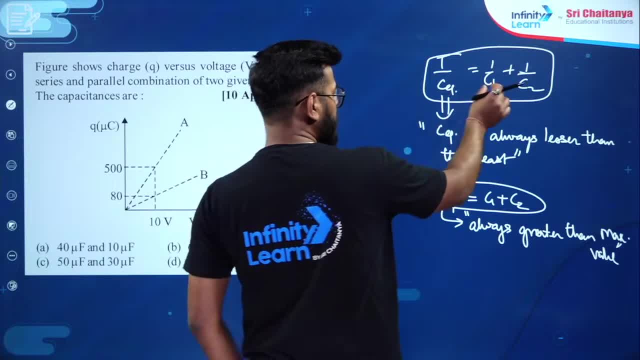 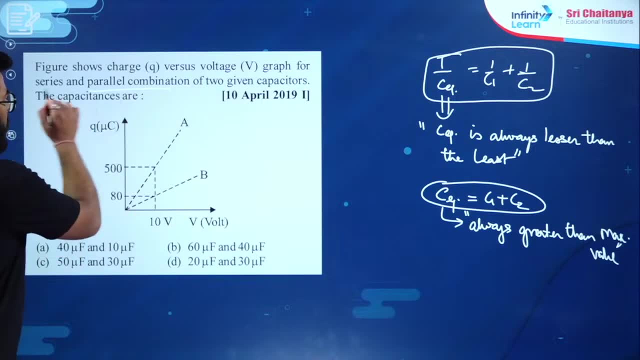 If C2 is greater, then C equivalent will be greater than C2. And in this C1 is the smallest, So this C equivalent will be smaller than C1.. Okay, So now tell me, will it be more in parallel or in series? 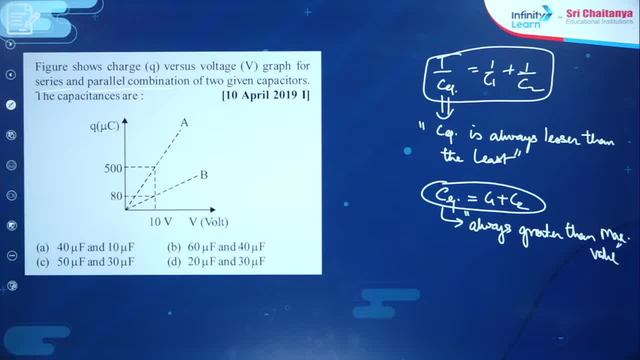 Will it be more in parallel or in series? It is obvious, sir. Parallel addition happens in this way, so parallel will be more. So here parallel is more. Hmm, Okay, So the value of parallel is more. So now see how much C equivalent value is coming in parallel. 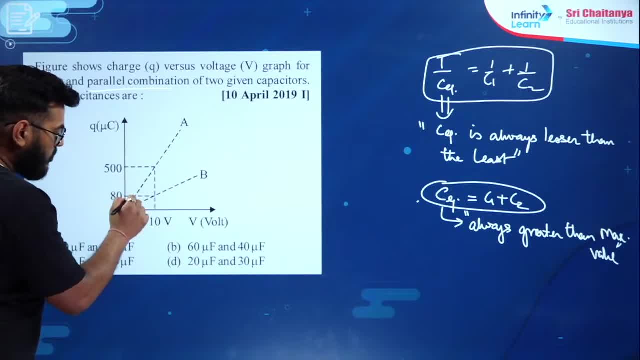 How much C equivalent value is coming in parallel. See, where the slope is more, the answer will be parallel. right, Where the slope is more, the answer will be parallel. So the value of parallel is coming For parallel. get the slope of this. 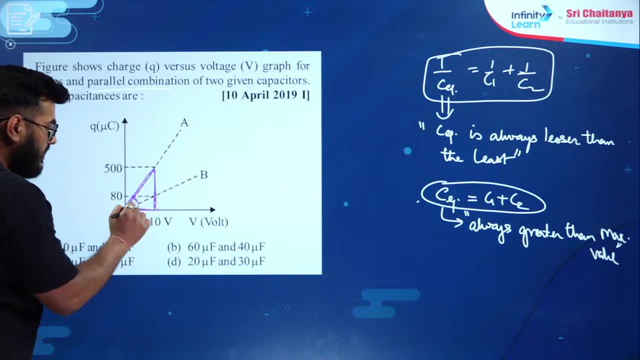 Okay. how do you know, sir, that the answer will come from the slope? only Because Q is equal to Q by V will be C, which is tan theta, right? So now, how much is the value of tan theta? in parallel, 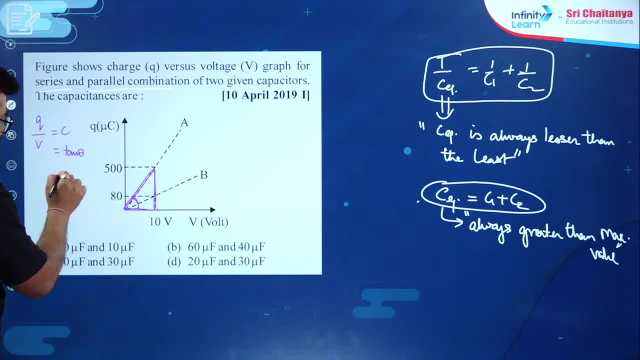 Sir, this is the total value of 500, 500 by 10.. This is 500 by 10., In which This is your series in parallel. In parallel, That is basically the value of C1 plus C2 is equal to 50.. 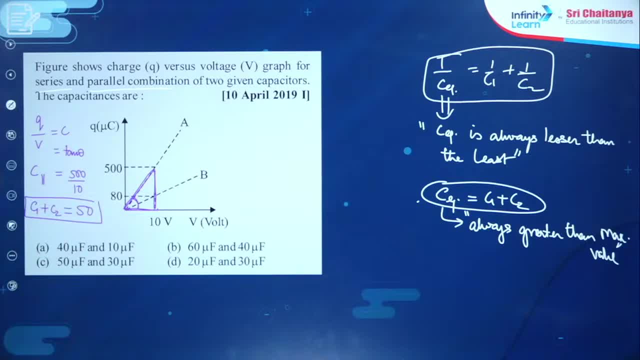 The value of C1 plus C2 is equal to 50.. Clear, Done So by this, option number C and option number B have already been rejected out. Option number C and option number B have already been rejected out. Clear, The calculation can be done in option number A and option number D. 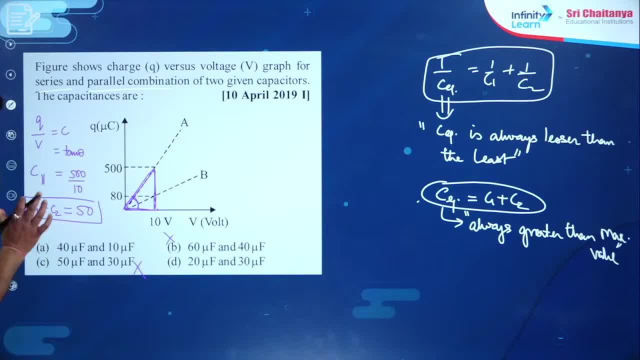 Okay, Okay, sir, Done Now. C1 plus C2 is 50.. Let's subtract C1 and C2.. Let's subtract this series one. The series one will be smaller. How much is coming in this, sir? 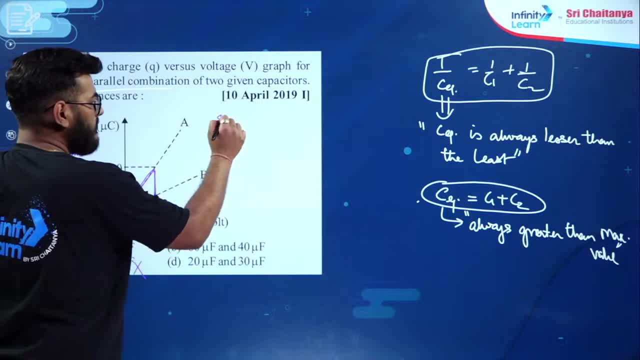 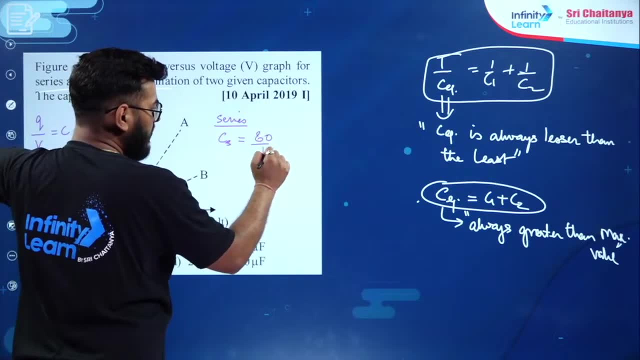 80 by 10.. C equivalent in series. How much Cs is coming in series, Sir? this is 80 by 10.. 80 by 10.. And how much is coming in series C1, C2 upon C1 plus C2.. 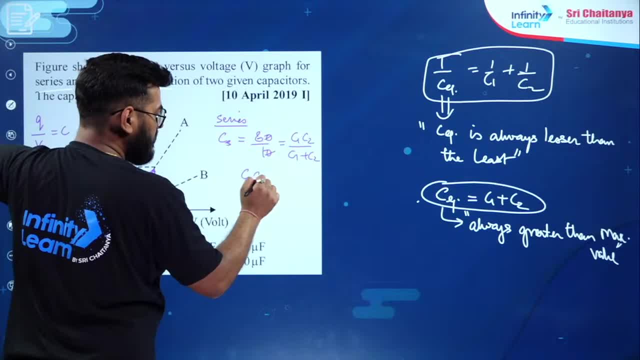 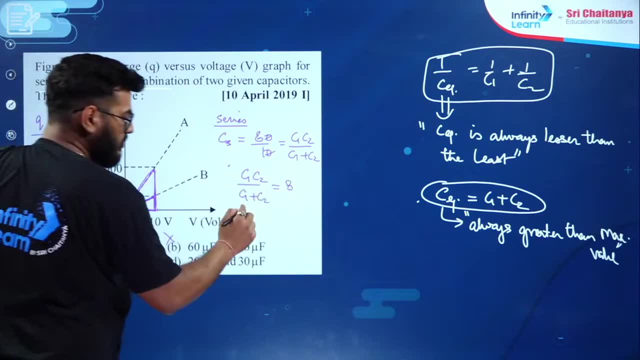 Clear. So how much will this be, Sir? this is equal to 8. C1, C2 upon C1 plus C2 is equal to 8. Clear. How much is the value of C1- C2? 50. So give this 50 there. 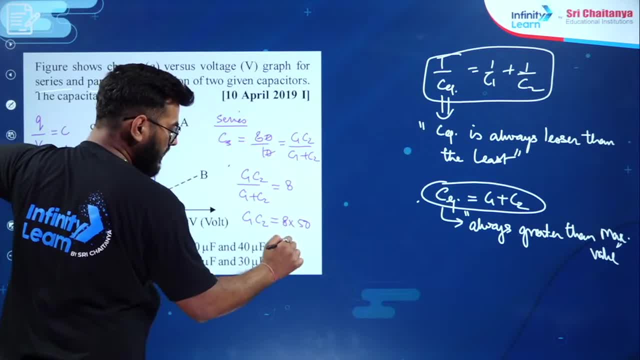 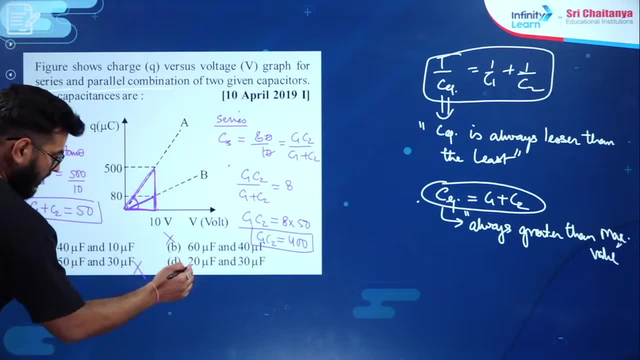 How much is C1 into C2?? 8 into 50. That is 400.. Now, if you want, you can solve these two and remove them, But you can also look at the options. If it is 20 and 30, then the answer is 600. 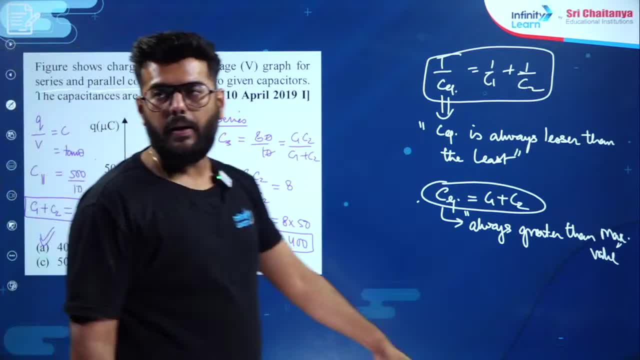 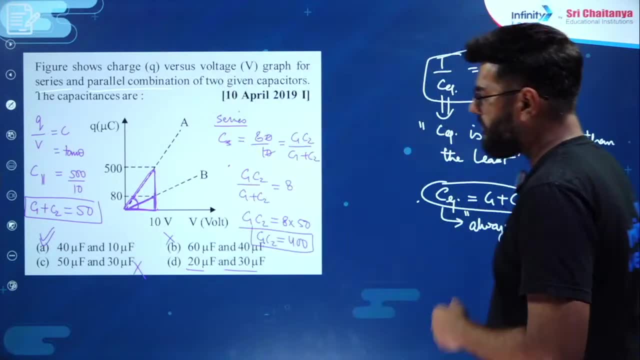 And if it is 40 and 10, then the answer is 400.. Option number A is absolutely correct. It will be A Absolutely correct. Absolutely correct, Did you understand? No, Is it clear or not? So the parallel one should be known. 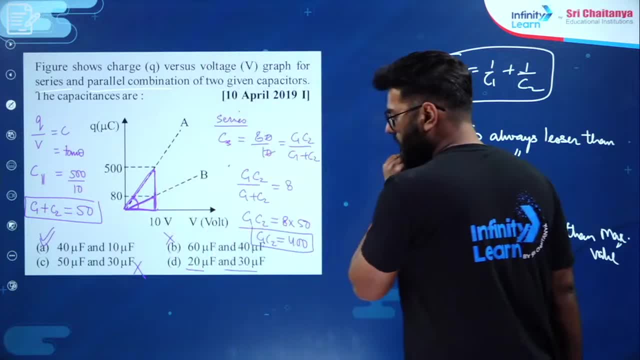 The parallel one will be more sloped And the series one will be smaller sloped, Right, So the small one is here. There are 8 values in the series, And how much is C1, C2 upon C1 plus C2?? 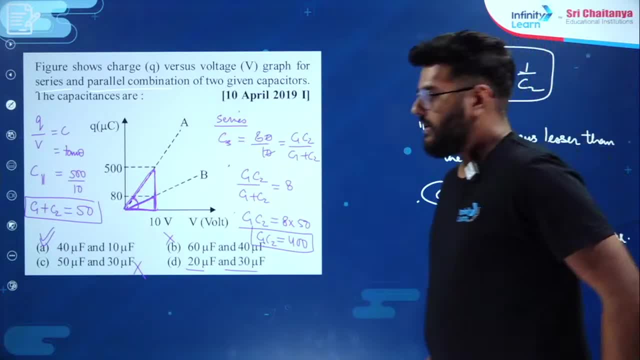 If you put the value of C1 plus C2 here, then the answer is 400.. OK, Let's go. Next question: Find the equivalent capacitance between A and B. We have to find the equivalent capacitance between A and B. 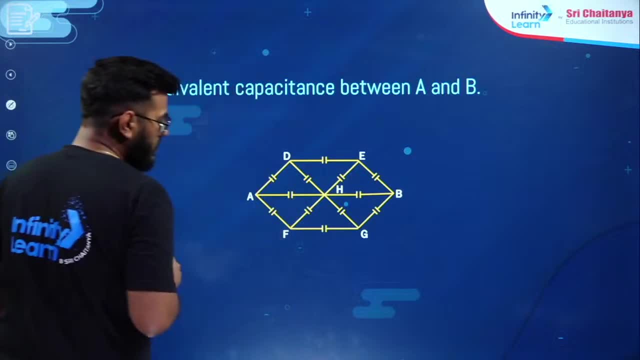 Now look, It is a very standard method. There is an approach of symmetry in it. The approach of symmetry is that when the charge will come from here, then the charge will be disturbed by seeing where I will go. So it will see three ways. 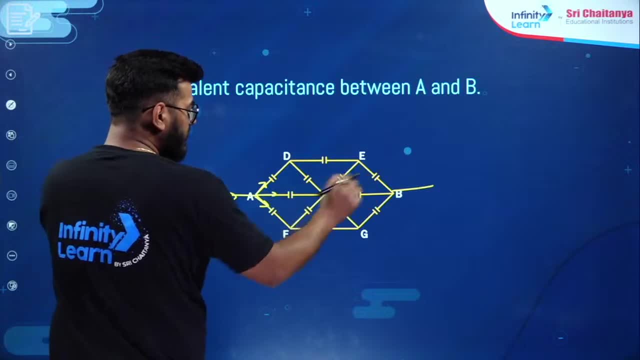 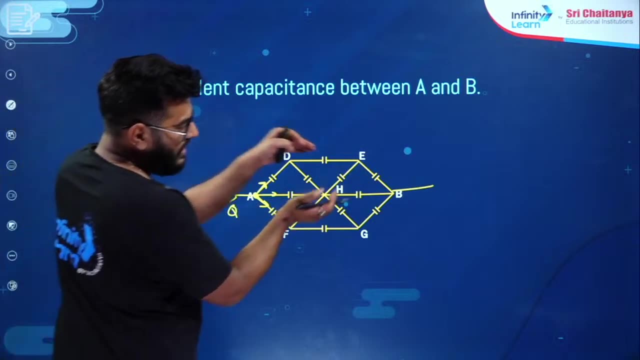 One is this, one is this and one is this, And it will also see how the exit is. So look the side in which I am taking entry and the way in which I am taking exit. then you are maintaining symmetry. You have made a perfect triangle. 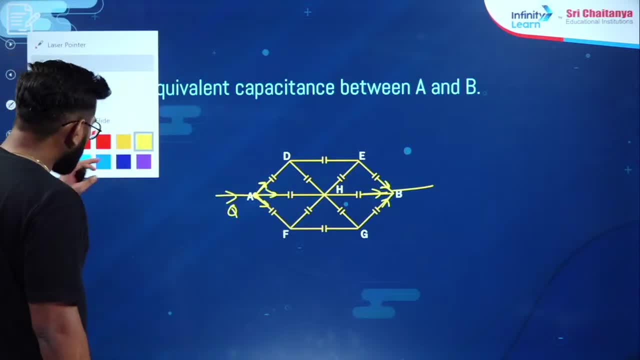 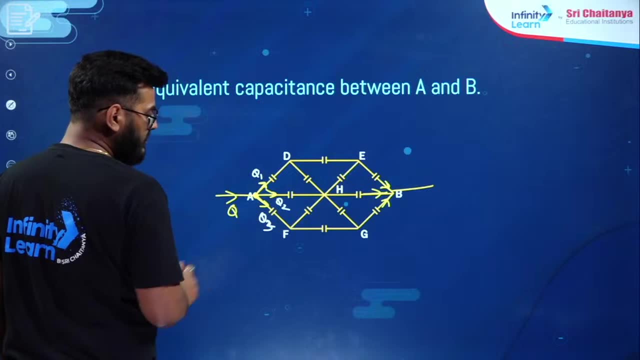 According to which you have got the entry, according to which you are also getting the exit, And because you have done this, then the charge is always equally distributed as it is distributed at the entry, Suppose, at the entry Q1, Q2, Q3 is there. 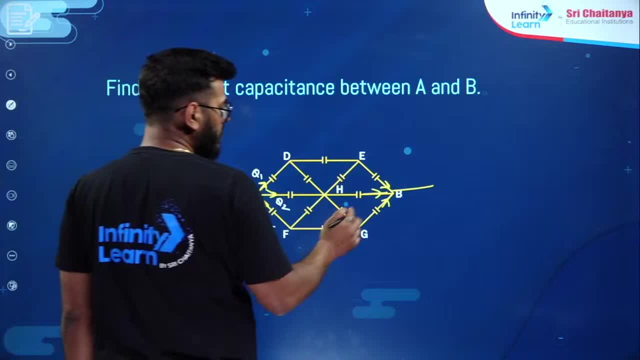 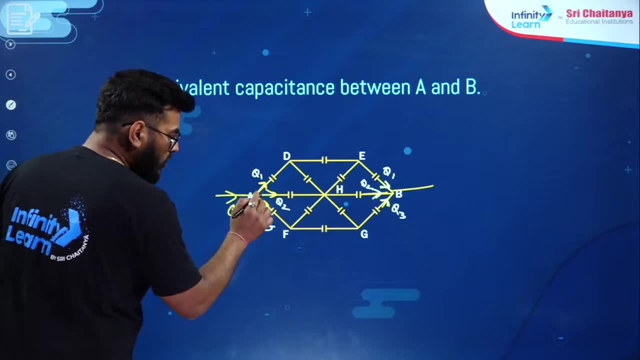 Although I also know that Q1 and Q3 will increase the value. but suppose Q1, Q2, Q3 is there, So to exit here too, Q1 will go from here to Q2 and from here to Q3. And then, if Q2 charge is going on this: 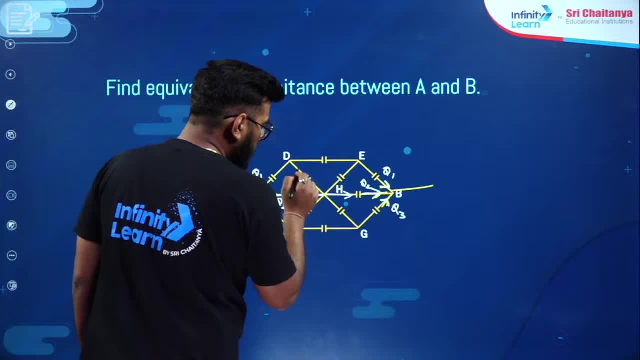 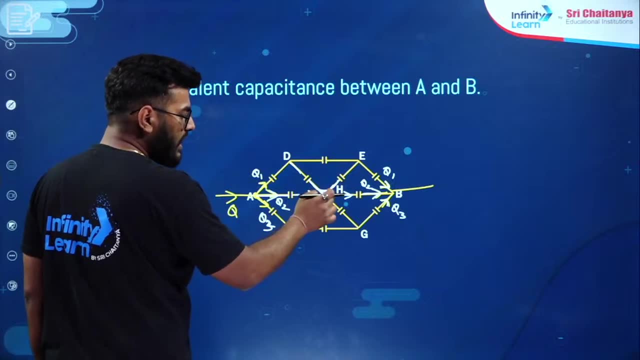 it is going on this and the same Q2 charge is going on this, So there is no point in connecting it here and here. Remove it Why? Because neither the charge is going from here to here and neither the charge is coming up from here. 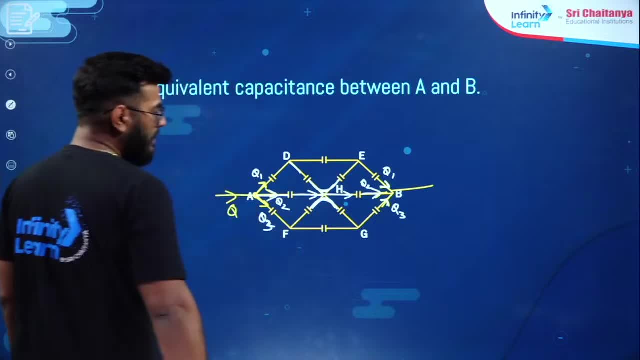 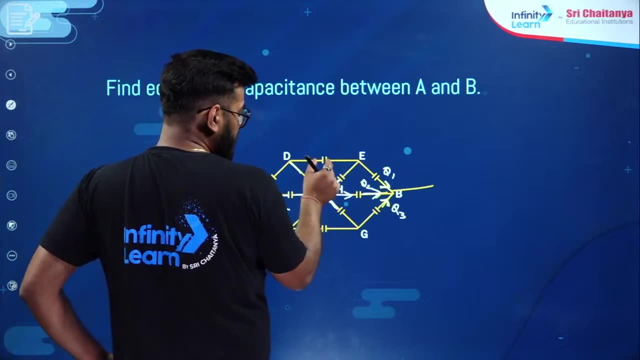 And the same case is with this too. You can remove this too, And if you remove it, then see, this can be solved. This C, this C in the series, then the answer will be C by 2.. C by 2 and C will be 3C by 2.. 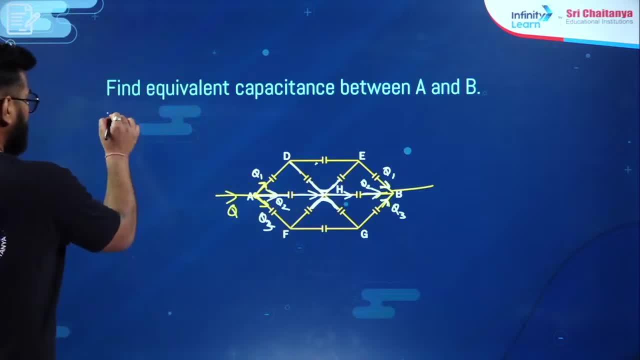 3C by 2 plus 2C, 3C by 2. Plus 2C in the series. So 3C by 2 plus 2C, Here 2, here 2.. How much will it come? 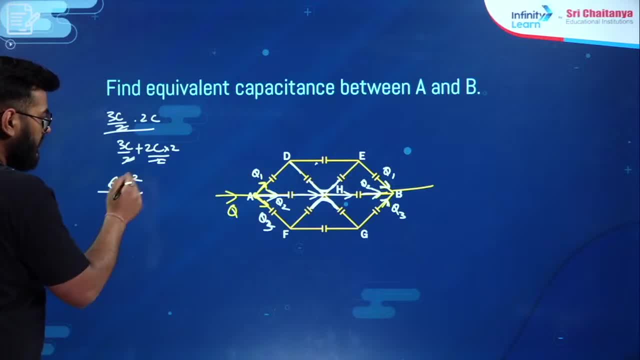 These two. these two will be cancelled by this. This will be 6C square divided by 4 plus 3, 7C, So this will be 6C by 7.. This will come from the upper one. This will also come from the lower one. 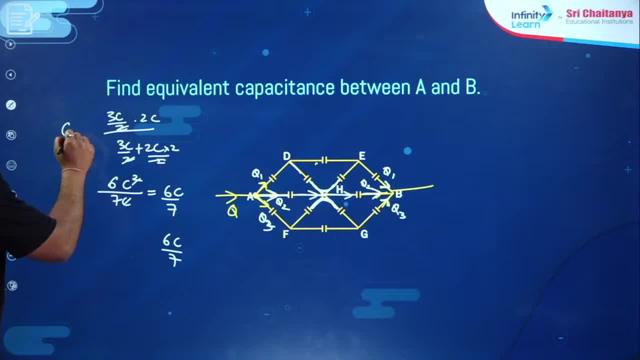 6C by 7.. Okay, This is my C1.. This is my C2.. The lower one, And how much will these two? come C by 2.. So C3 will come C by 2.. So, ultimately, instead of this, one will come from the upper one. 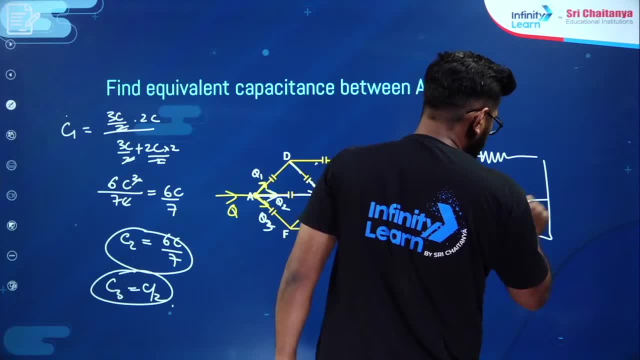 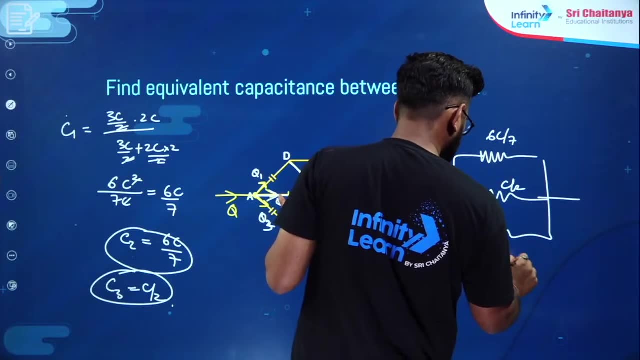 One will come from the lower one And one will come from this one. Okay, How much will this one come? C by 2.. Its value will be 6C by 7.. And its value will be 6C by 7.. 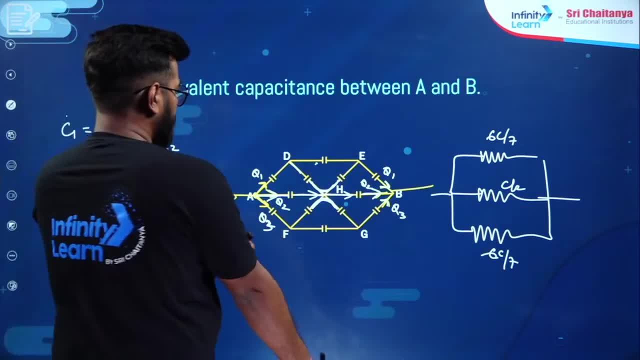 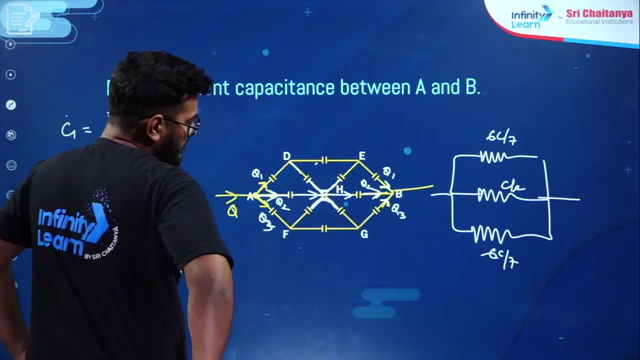 The total is 12C by 7 plus C by 2.. Let me check the upper one once. Let me check the upper one once too: C by 2.. C by 2.. 3C by 2.. 3C by 2 plus 2C. 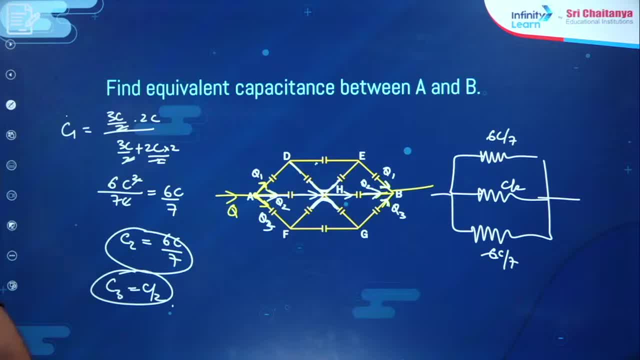 3C by 2 plus 2C, 2C, 2C, 4,, 4 plus 3, 7.. 7, 6C by 7.. Correct, Finally, how much is coming? Let me add everything. 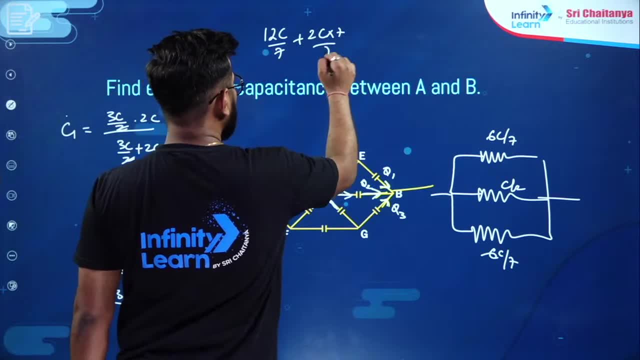 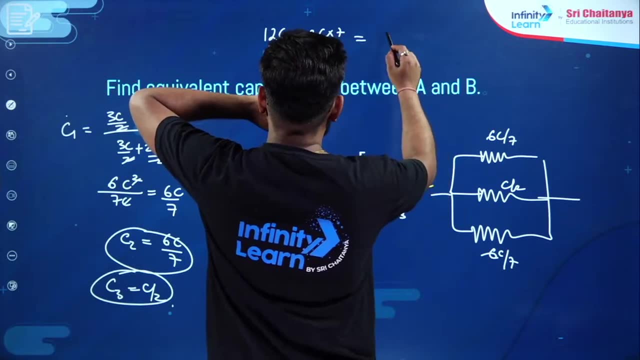 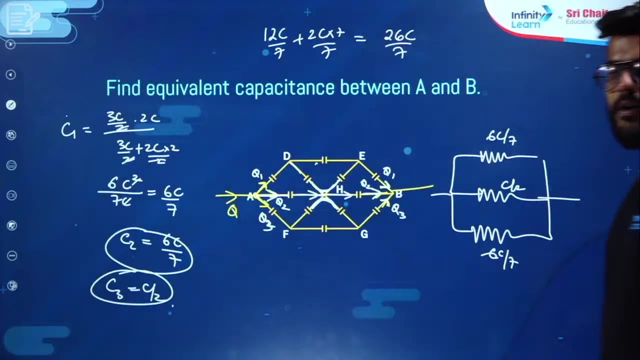 12C by 7 plus 2C Into 7, into 7.. 12 plus 14, 14.. 26C by 7 is coming. 26C by 7 is coming. 1.25 is coming final. 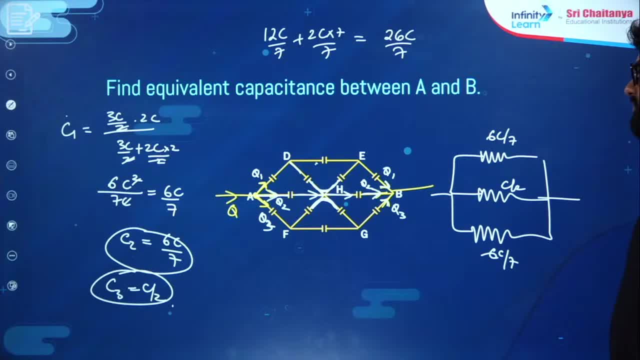 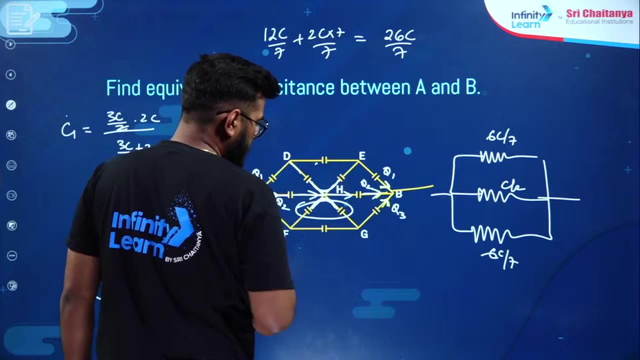 Are you sure? How is 1.25 coming final? Are you sure 1.25 is final? These two are in series, So it will be C by 2.. Then, parallel to this, C by 2 plus C, 3C by 2.. 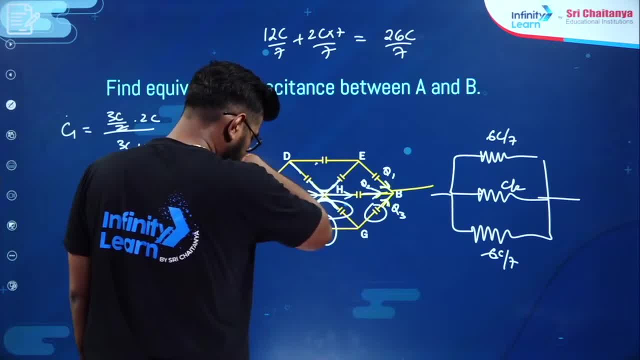 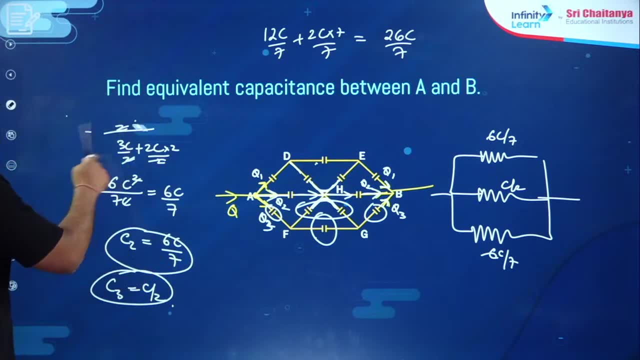 3C by 2, C and C. Oh ho, ho, ho, ho ho. I made a mistake. I am so sorry. I am so sorry I made a mistake of upper one. This C by 2 is correct. 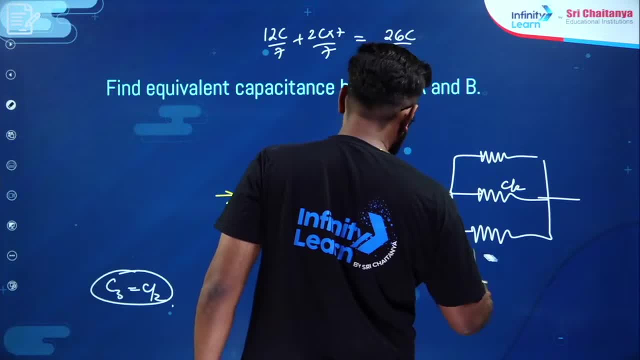 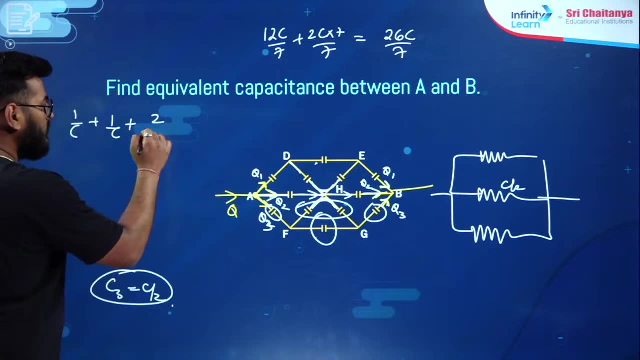 This is not 6C by 7.. This is not 6C by 7.. 3C by 2, 1 upon C plus 1 upon C plus 2 by 3C, This is going to be 1 upon C equivalent. 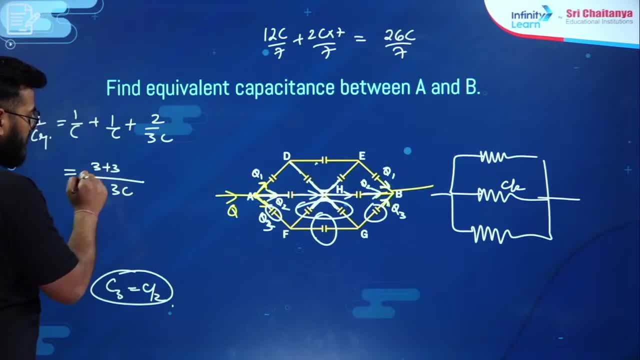 Okay, If 3C is common, then here 3 plus 3 plus 2.. Okay, So this is 6 plus 2,, 8 by 3C. The value of C equivalent is 3C by 8.. 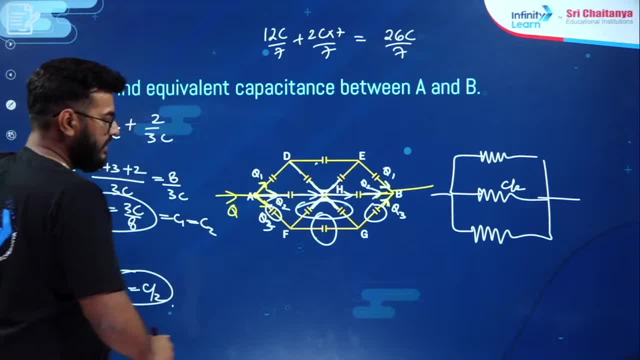 This is done, This will be my C1 and this will be my C2.. So this will basically be 3C by 8 and this will be 3C by 8.. So final is 6C by 8.. 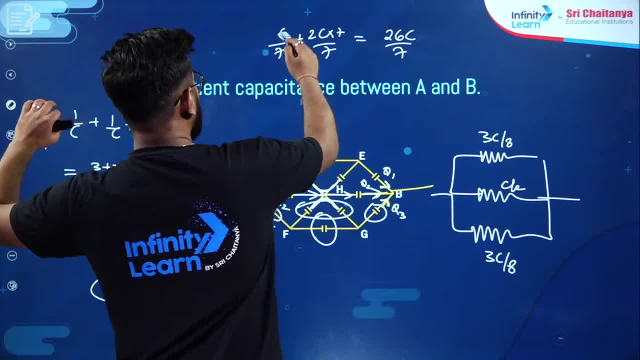 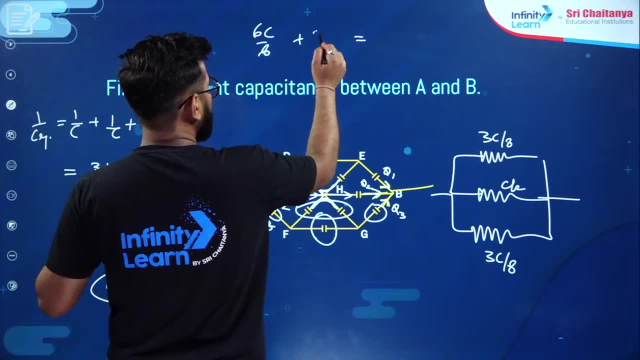 6C by 8.. How much is it? 6C by 8 plus 2C, 6C by 8 plus 2C, 6C by 8 plus 2C, This 3, this 4, here 4, here 4.. 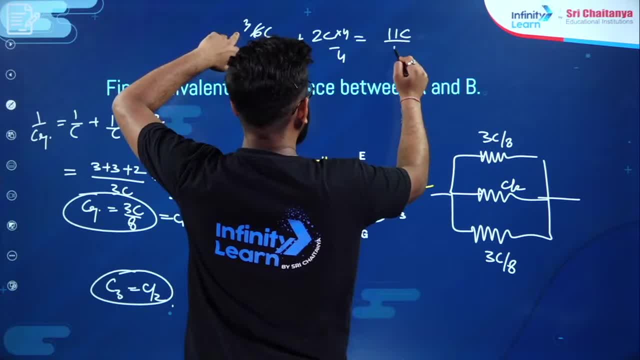 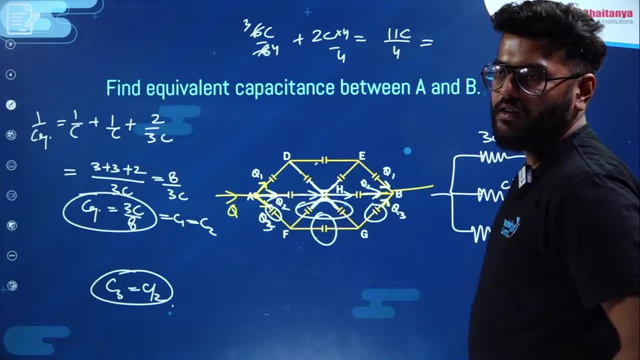 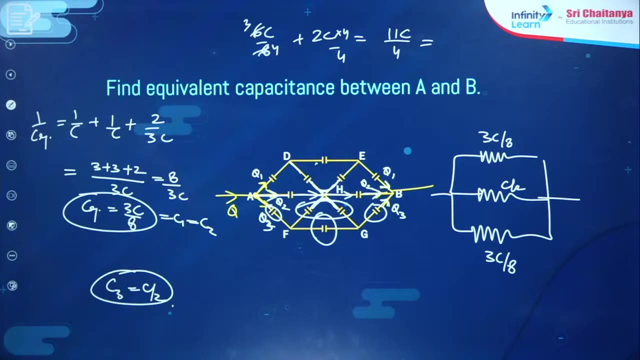 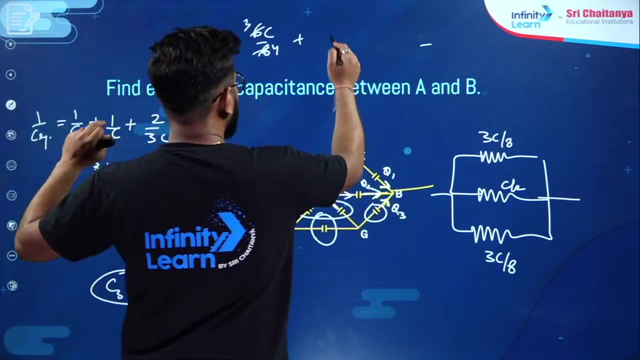 So 8, 8 plus 3, 11.. 11C by 4.. That means, Bro, 11C by 4 is coming. Did I do it wrong? still, Hmm, Hmm, C by 2.. 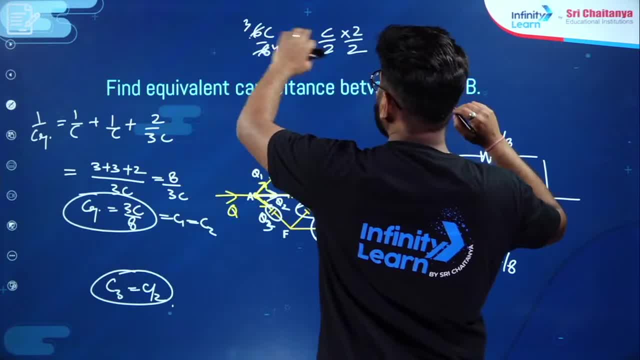 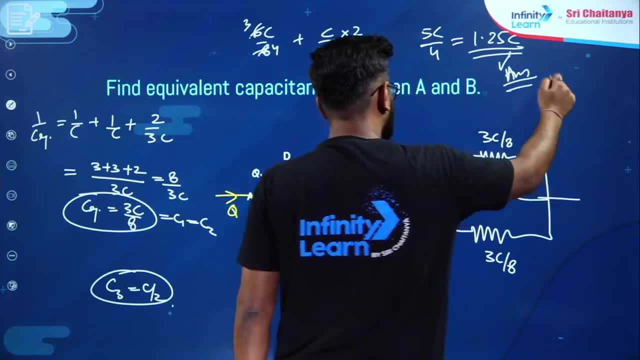 2 or 2.. You have become old, sir. 3 plus 4, 5C by 4.. 1.25C, Correct? The answer is sour plan. I am so sorry. 1.25C, you all said it morning. 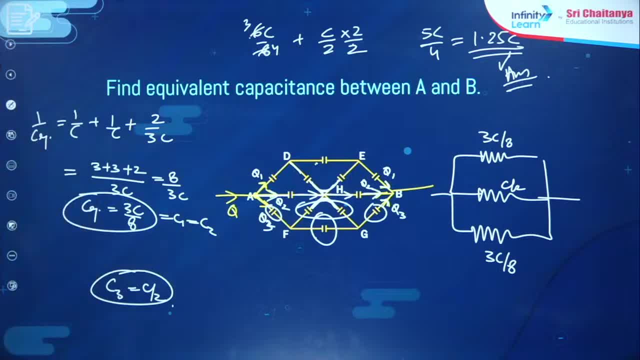 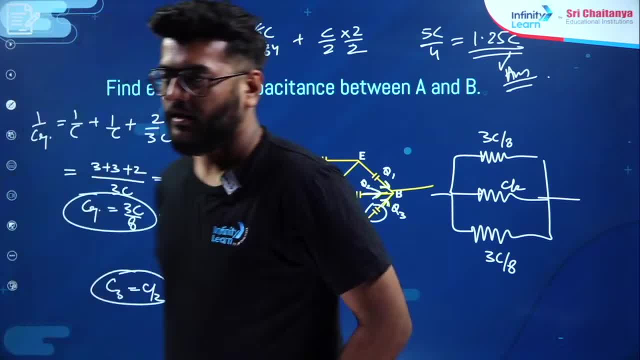 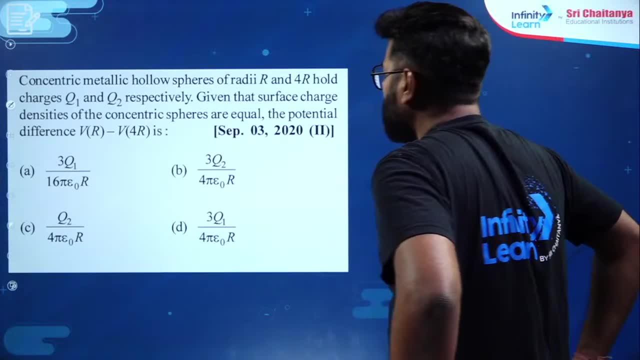 plus C by 2, 1.25C, 5C by 4. answer is coming absolutely right. okay, concentric metal hollow sphere of radar RN4I hold charges Q1, Q2 when there are. don't do this, this is for spherical charges, let it be. 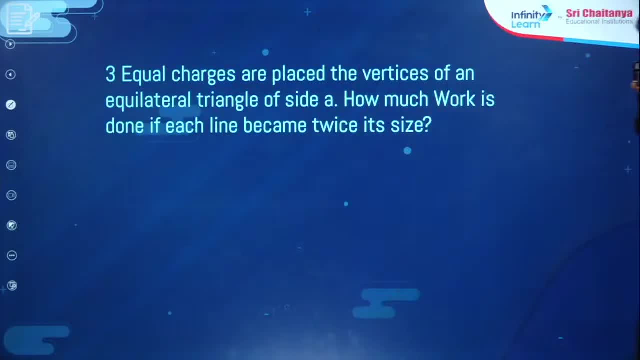 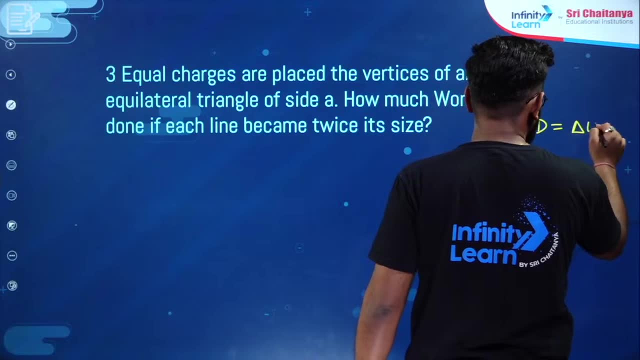 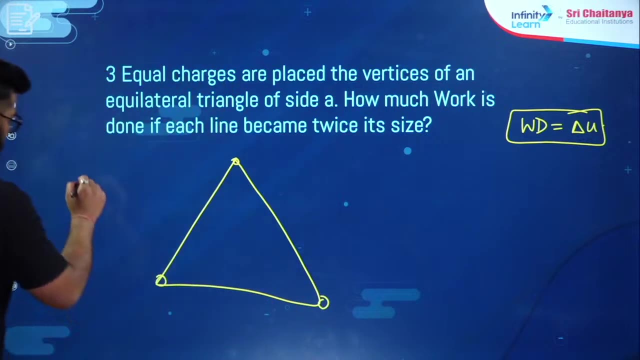 look here: three equal charges are placed, vertices of an equilateral triangle. how much work is done if each line becomes twice in size? simple A work done is equal to change in potential energy. in final state you have to tell. and initial state was this: okay, charge equal. 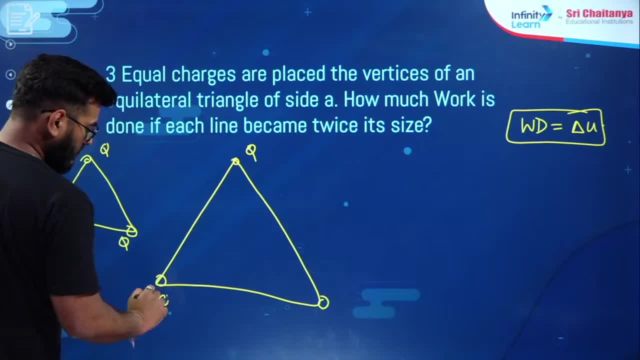 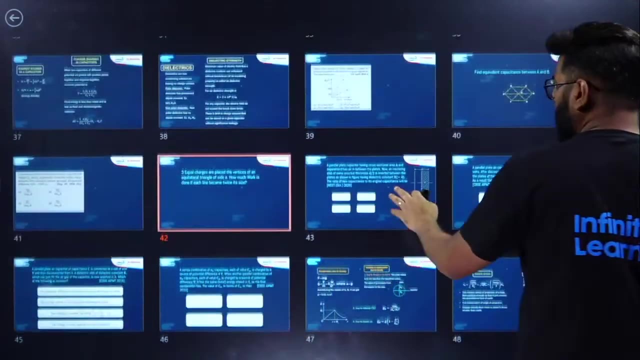 Q, Q, Q and after that Q Q, Q. so after that size will be double, A will be two way, and U final minus U initial, in final state minus initial state, you will get the answer. okay, now look, I am talking about dielectric, right, right. so what are dielectrics? 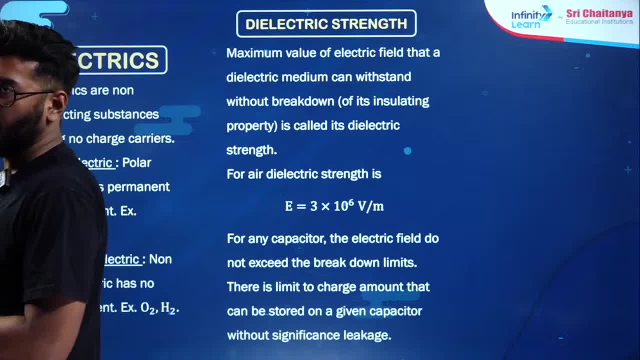 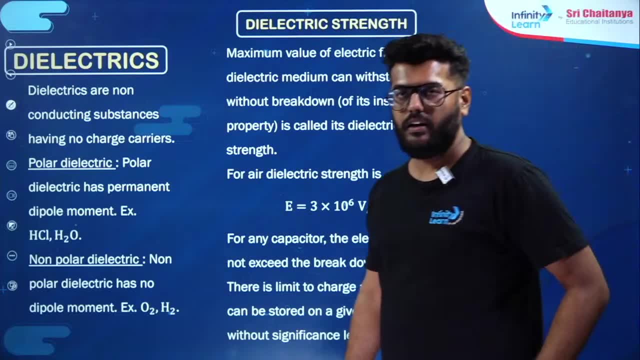 dielectrics. they are the media which you will put in the middle of the capacitor plates, by which you ultimately what you want to do. you want to alter the value of the capacitance and also alter so that more amount of energy can be stored. okay, mostly those. 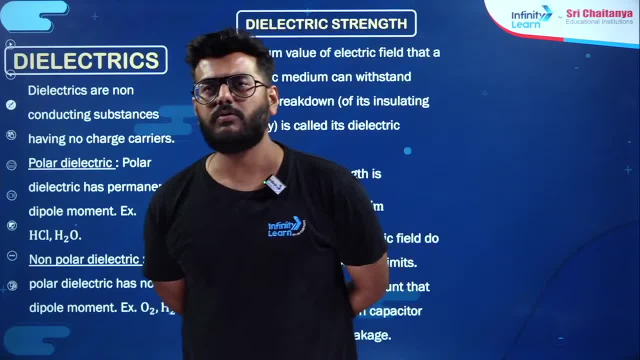 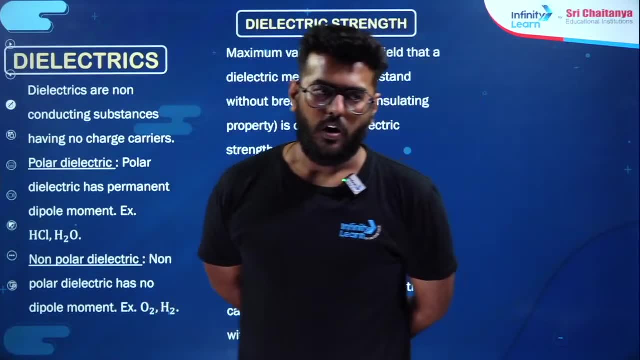 who live in our houses. you must have seen in your house that the capacitor gets damaged, due to which the fan starts to move slowly. so the capacitor is changed because the dielectric is damaged and the capacitance is damaged. the metal sheet does not have any problem. 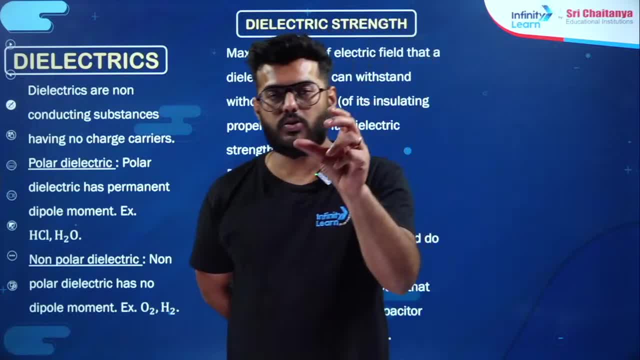 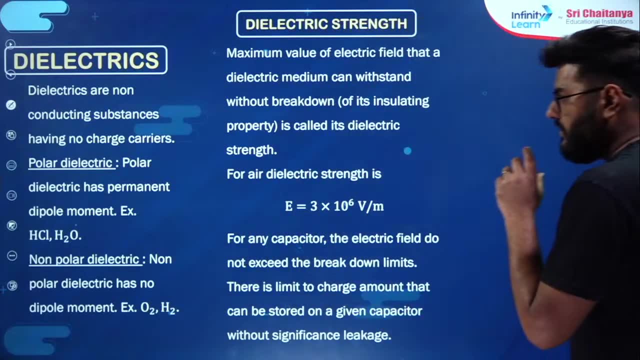 the dielectric in the capacitance is damaged and, due to this, the amount of energy that can be stored is reduced, due to which the fan starts to move slowly. okay, because the energy source is needed, and this is the same problem with dielectrics. okay, so in dielectrics, 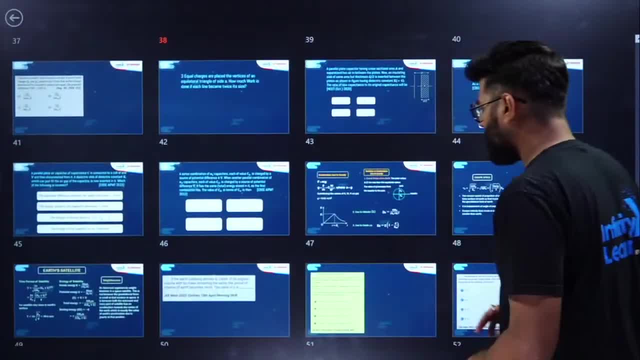 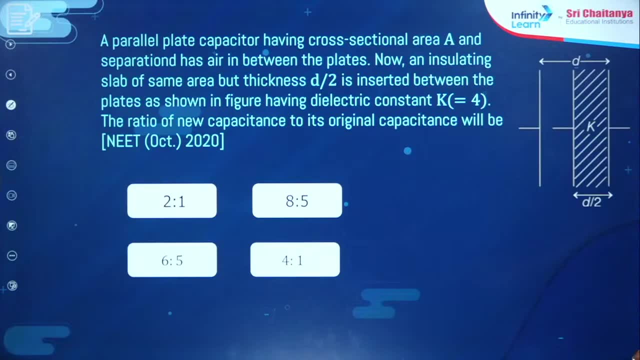 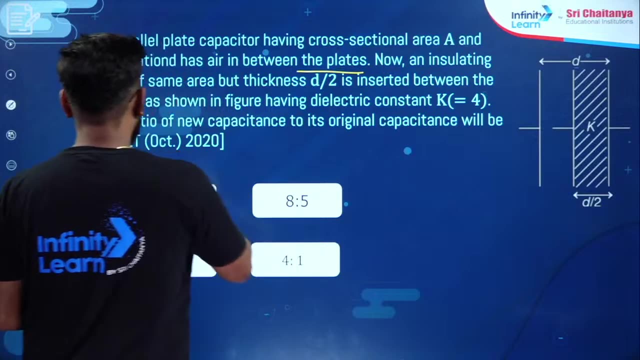 the questions that come come. one is: how is your combination and variation happening? as an example, see this first question, not the first here. it is a parallel plate capacitor of having cross sectional area A and separation. has air in between the plates, now an insulating slab of same area. 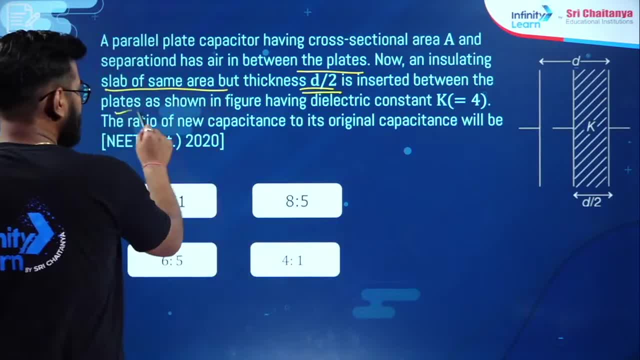 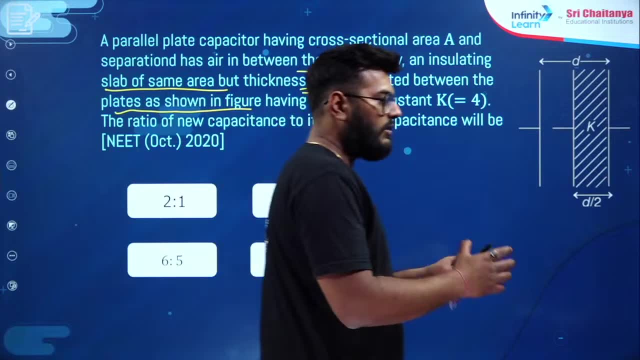 but thickness d by 2 is inserted between the plates as shown in figure. having dielectric constant k equals to 4, the ratio of new capacitance to its original capacitance will be. so the first question comes in this of combination, that if the combination is given, 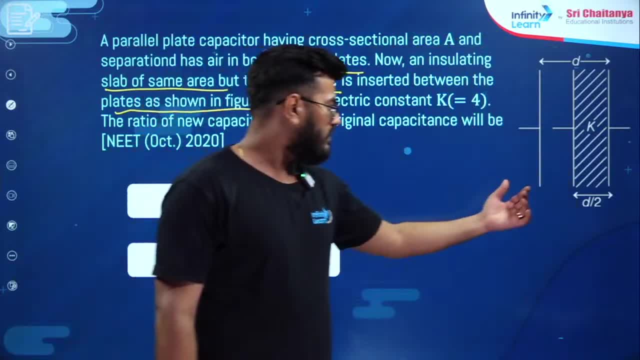 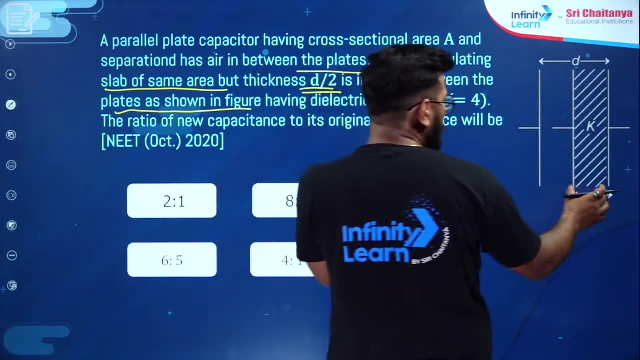 capacitors are installed and dielectric is inserted in the capacitor, then in that the equivalent capacitance will be how much? so in all these cases where series is used here, you assume as much as d by 2 is remaining. d by 2 region, I will assume. 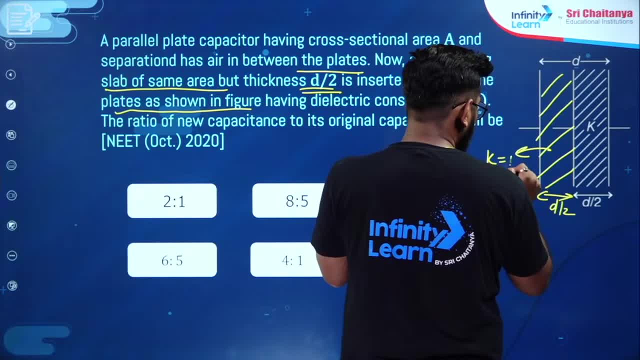 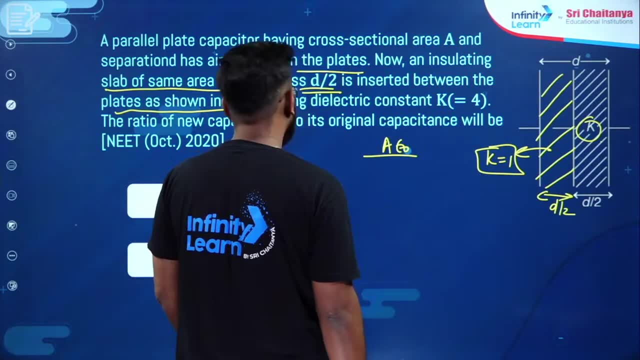 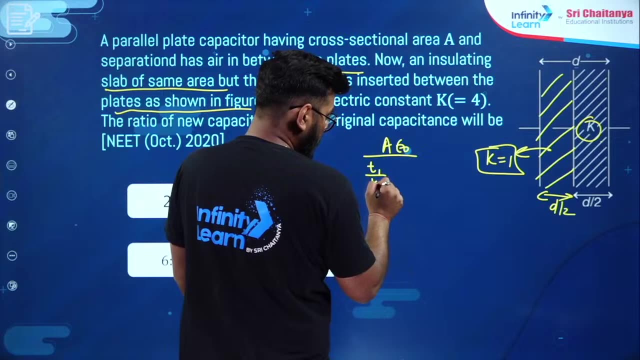 that the value of capacitance will be equal to 1, because there is nothing. and in this k is so simple, A epsilon naught divided by T1 upon k1, plus T2 upon k2, plus T3 upon k2, plus Tn upon k3. 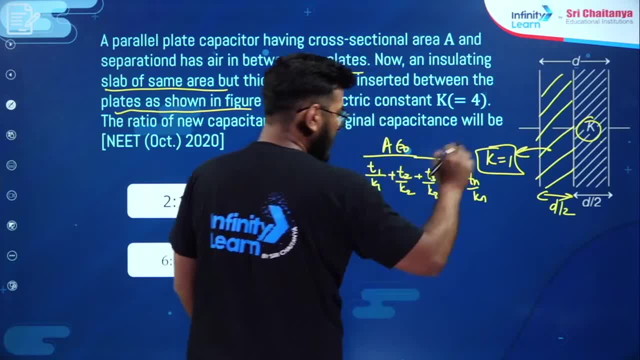 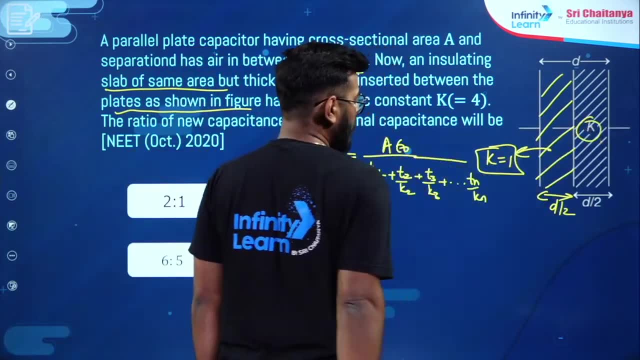 dot, dot, dot plus Tn upon kl. all these are small, small, small. this gives you c equivalent in which, in series combination, in which, in this way, your is installed. so here, if I will get the answer, A epsilon naught. its width is d by 2. 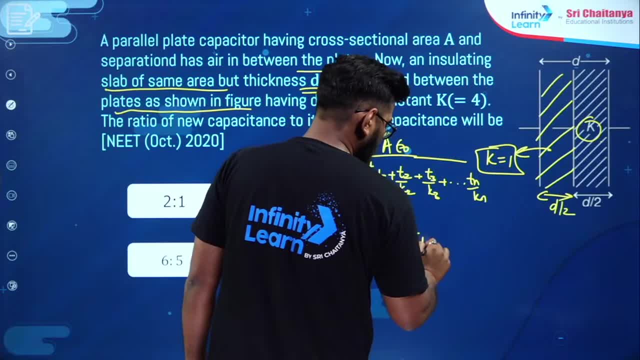 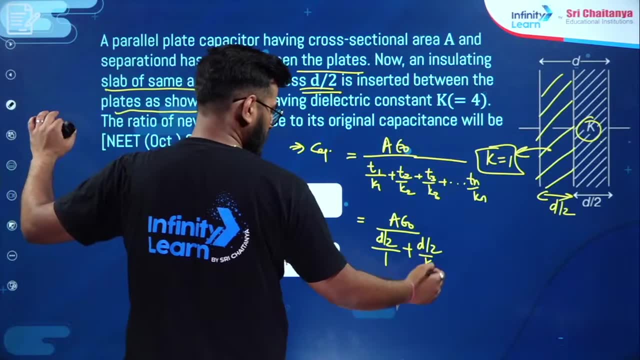 divided by its capacitance- 1, its width is d- by 2- its capacitance is k and k value is given, k value is 4. so keep 4. here, here 4 will be. keep 4, see how much is coming. this 4 here also 4. 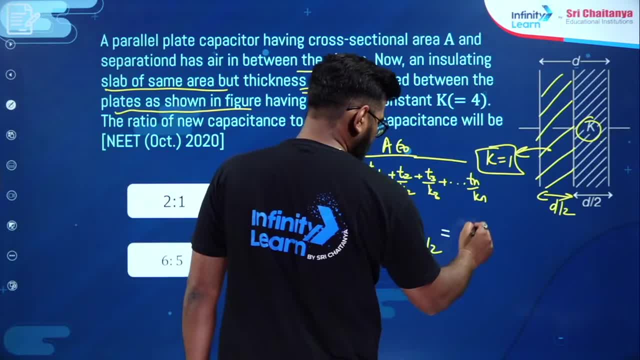 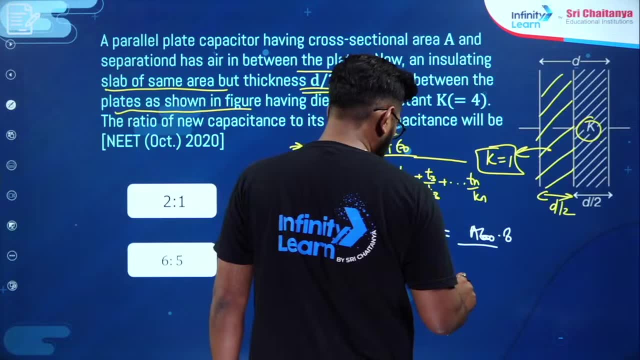 multiply it here also 4. multiply it. how much will come? A epsilon naught. divided by this 4, 2 is 8. 8 will go up, and here 4d plus d means 5d will come, so ultimately 8. A epsilon naught. 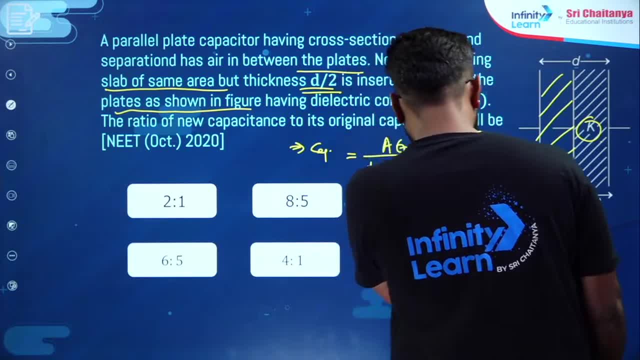 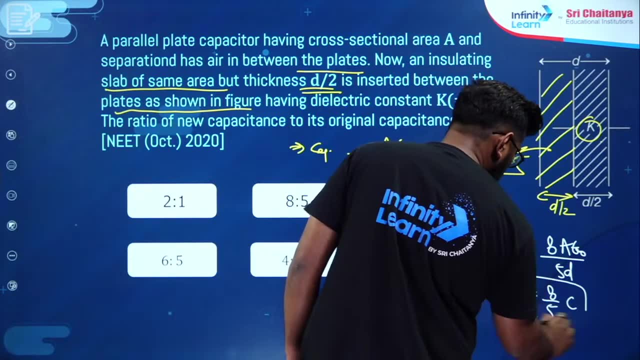 divided by 5d is the answer ok. and earlier how much was earlier it was A epsilon naught by d means 8dash is coming. how much is coming? 8 by 5 times c, because earlier how much was earlier it was A epsilon naught by d. 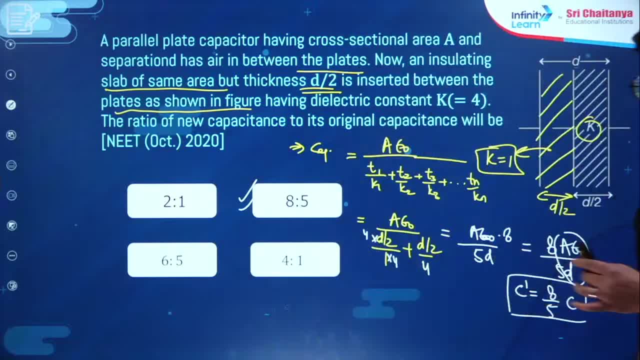 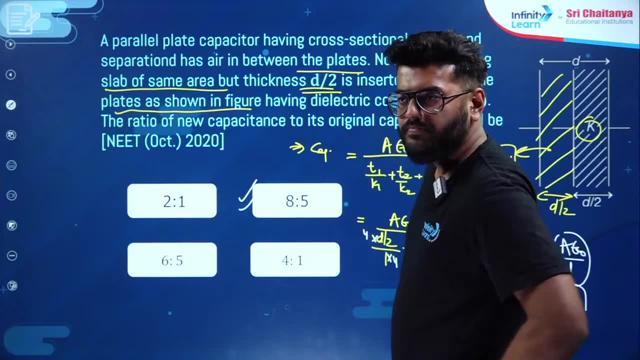 so 8 is to 5. correct answer will come here- which is the ratio of both. it will not be double and it will not be same. so what we are getting from this 8 is to 5. ok, clear. one more question here related to capacitor. 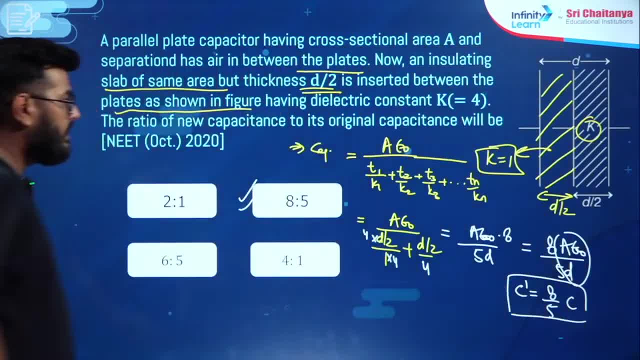 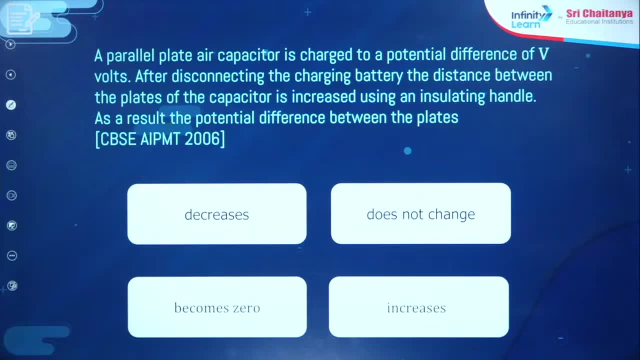 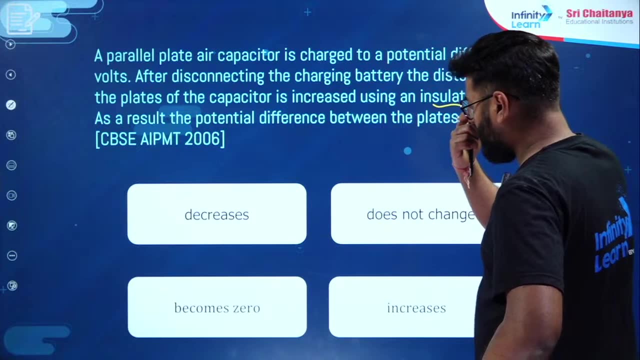 parallel plate capacitor. is there? ok, clear? one more question here. parallel plate capacitor is charged to a potential difference of VV. after disconnecting the charging battery, the distance between the plates of capacitor is increased using an insulating handle. as a result, the potential difference between the plates. 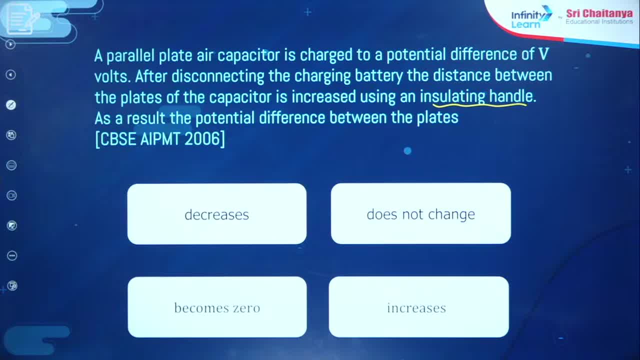 what happens to the potential difference between the plates- ok, battery is disconnected and distance between the plate whenever battery disconnects. battery is disconnected, battery disconnected. so in this you should understand one thing: charge, constant charge will not change at all means. what will we alter? q is equal to cv. 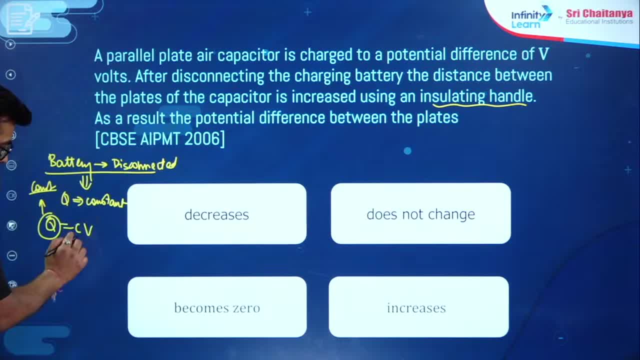 this thing is constant, so c and v will be inversely related and will make changes. if c will be big, then v will be small. if v will be big, then c will be small. if v will be small, then c will be big. now he is saying distance between the plates of the capacitor. 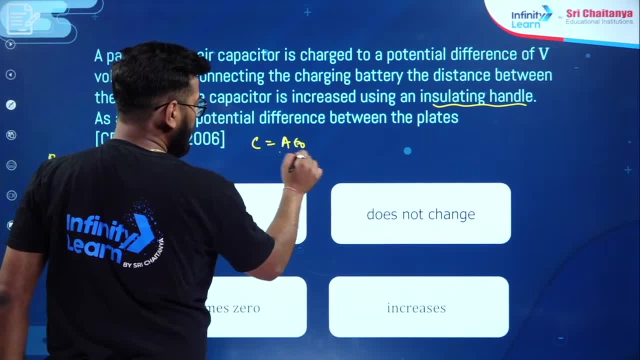 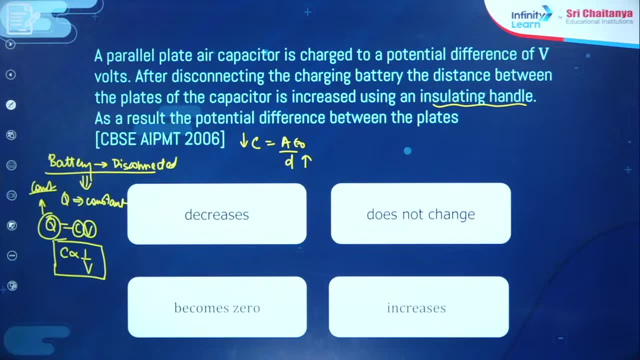 is increased. so c is a epsilon, not by d. so if you are increasing d, then c will be less using an insulating handle. as a result, the potential difference will be: c is decreasing, c is decreasing, so v will be increased. so v will be increased if we talk about charge. 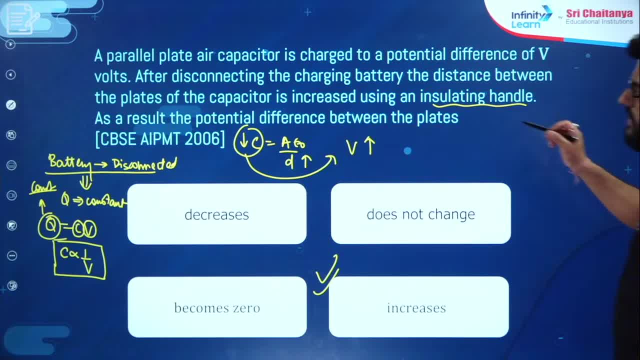 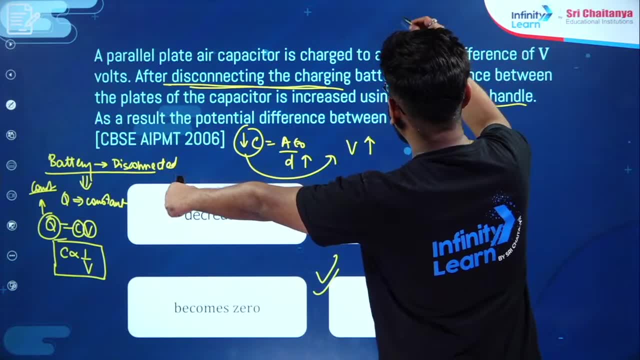 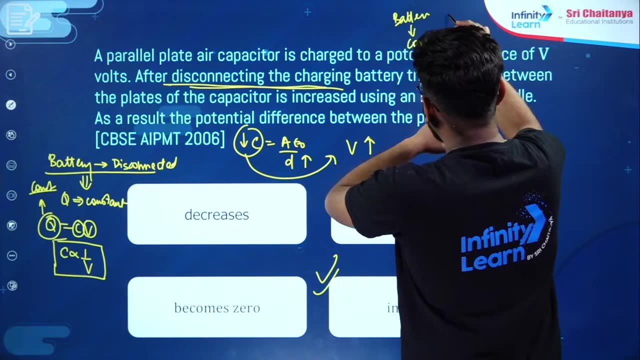 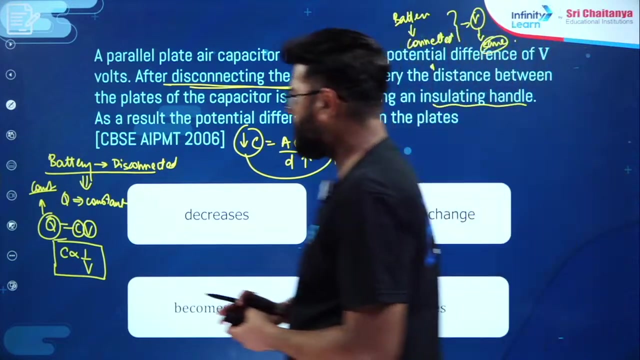 then charge will be constant. always remember, because, disconnecting from the battery, if it will be connected to the battery, then v will be constant. if battery is connected, then if battery is connected, then in this scenario v will be same. v will be same. ok, I hope this is clear. 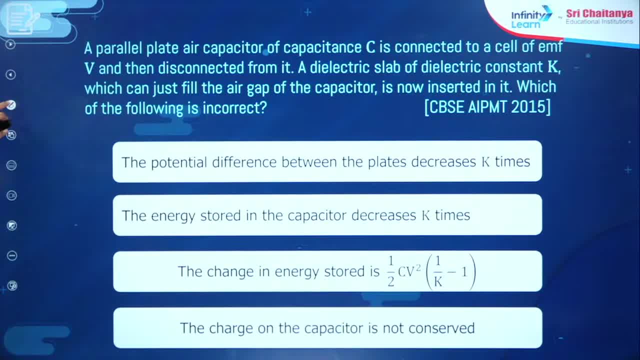 now parallel plate air capacitor is connected to a cell of emf v and then disconnected from it. a dielectric slab of dielectric constant k can just fill the air gap of the capacitor. now is inserted: which of the following is incorrect? see, you have disconnected the. 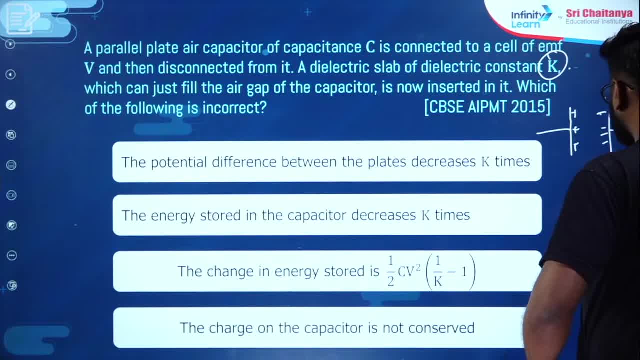 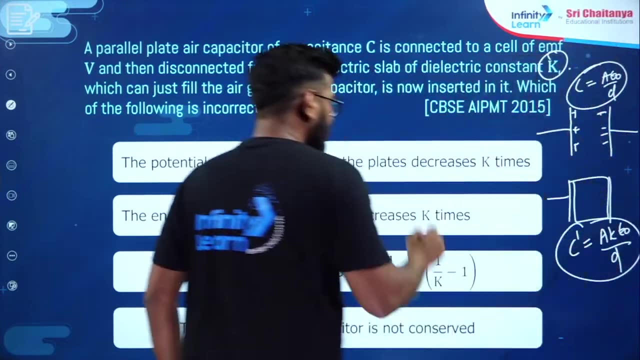 dielectric. and then you have introduced dielectric. what will happen with this? the new capacitance will be a k epsilon, not by d, and earlier c was a epsilon, not by d, so the point here is the same case. the battery is disconnected, so q will be constant. 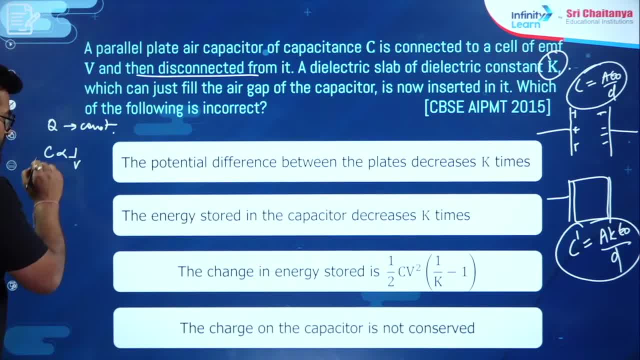 right, so c will be inversely related to v. ok, c is increasing, so v will increase. ok, and what will happen with energy? what will happen with energy? energy will be energy is. don't take half cv square, take half q square by c, because q is constant. 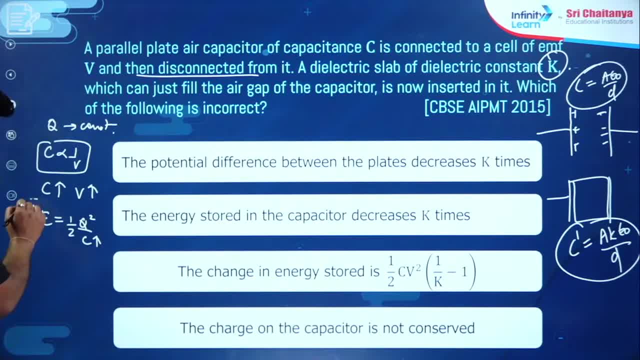 and c is increasing, so energy will be less. energy will be less, c will increase, v will increase. now see potential difference between the plate decreases k times. wrong answer. the energy stored in the capacitor decreases k times. may be, but is it k times or not? the change in energy stored is: 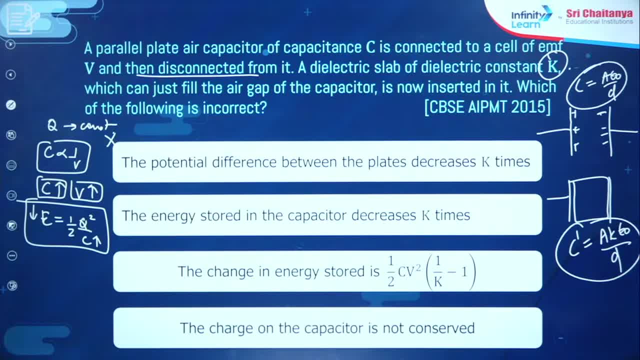 this much, the charge on the capacitor is not conserved. this is wrong. let's see the aspect of energy. let's see the aspect of energy. let's see the aspect of energy. ok, so see the energy. what was the energy earlier? earlier, the energy was half q square by c. 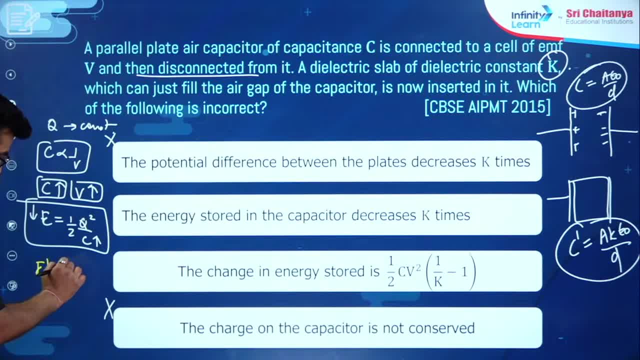 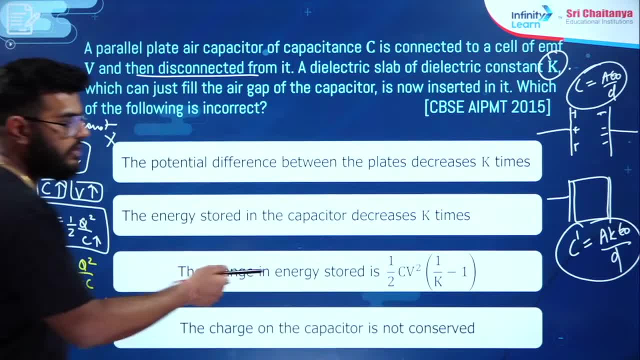 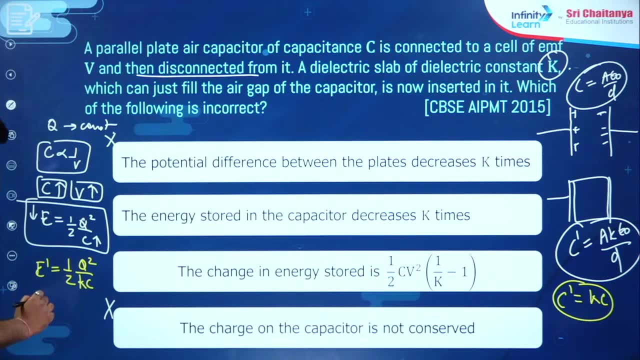 now what will be the energy e dash? e dash will be half of q square by k times c, because a, k epsilon naught means the value of c dash. c dash is equal to k times c k. so here it will be. so the new energy is basically: 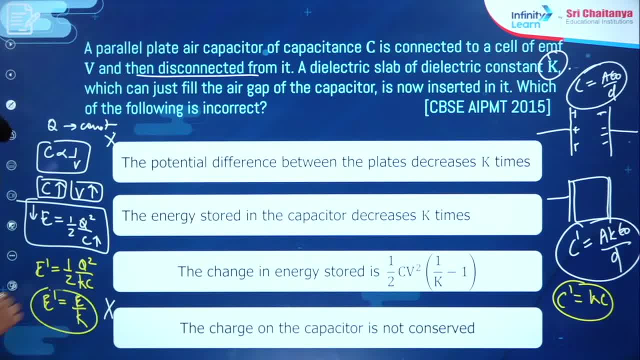 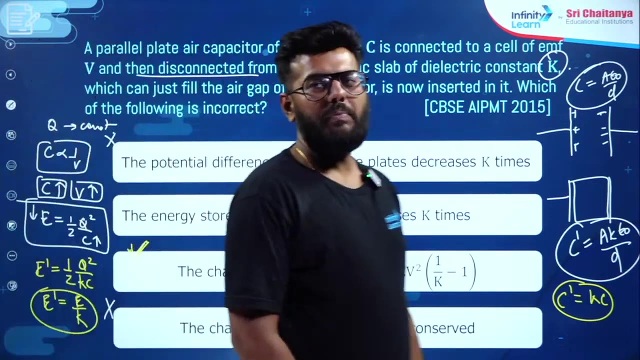 e by k, e by k. so energy stored in the capacitor decreases k times. decreases k times means the change in energy is e by k. this is absolutely correct. the change in energy is happening. it decreases, not k times. it should be 1 by k times. becomes 1 by k times. 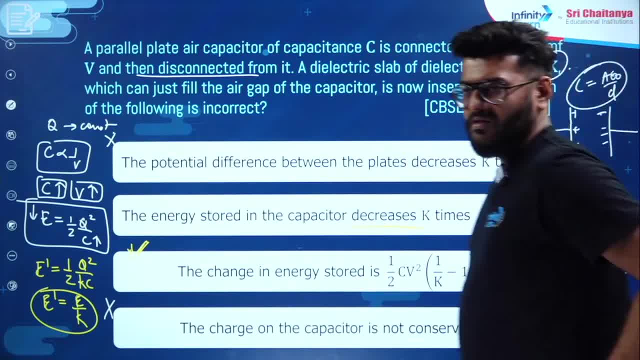 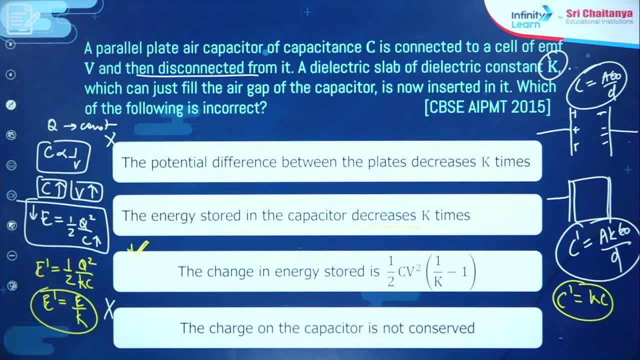 what is the meaning of decreases k times? which of the following is incorrect? ok, it is said. ok, it is said: oh ok, ok, ok, oh yes, oh yes, wait, wait, it is correct. c is increasing, so v will decrease Angle halt. decreases k times is absolutely correct. it is also correct. 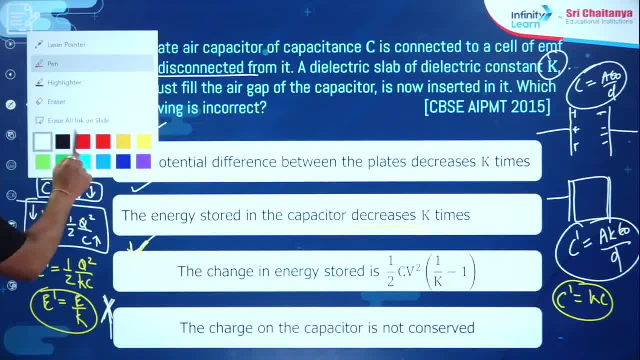 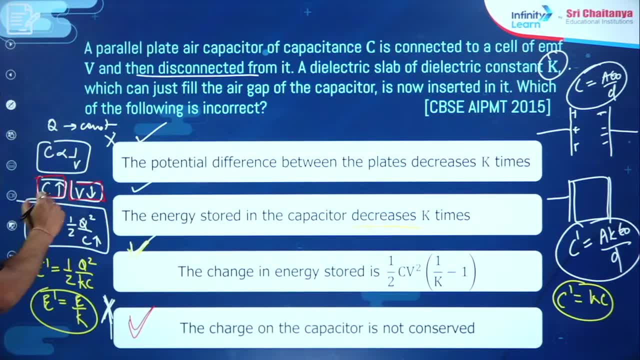 yes, it is wrong. all of these were not required. I had written wrong. c is increasing, so v will decrease, because the relationship is inverse. you see how c is increasing and the energy will also decrease. this is absolutely correct. it is also cooked. if it is also been correct. 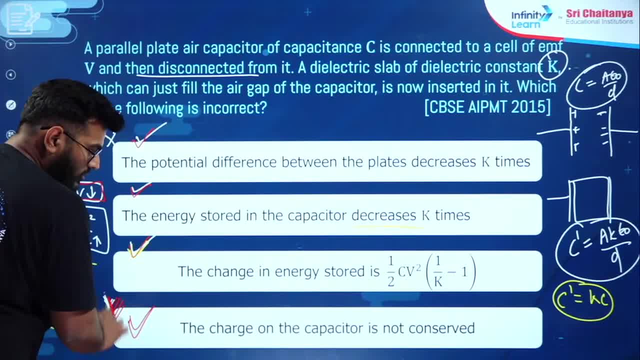 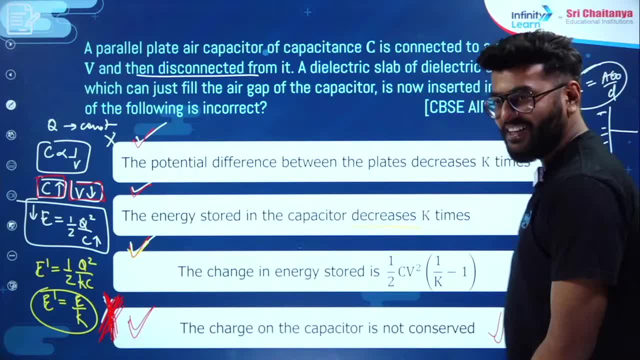 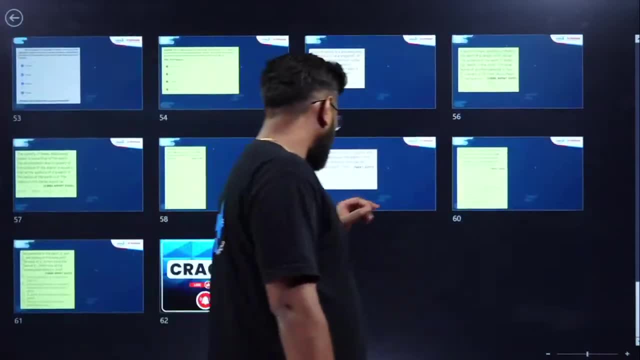 I knew it was wrong. the charge on the capacitor is not conserved. option number D is right. sociality of引 origination in attitude of the capacitor is incorrect. Are you lost? No problem, Let's move on to the next question. There are a lot of questions. 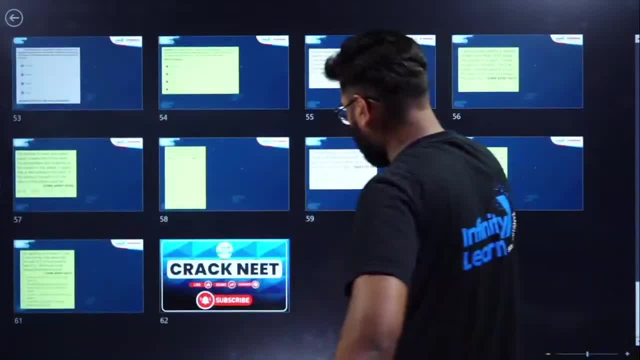 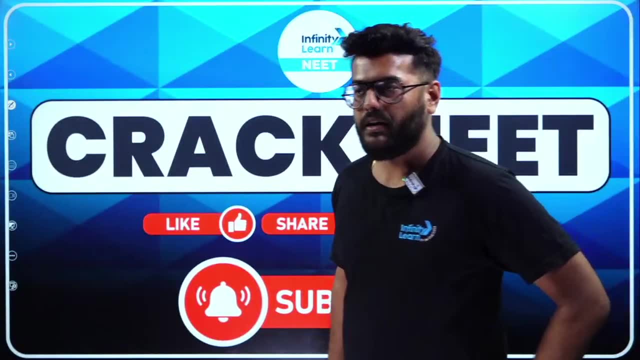 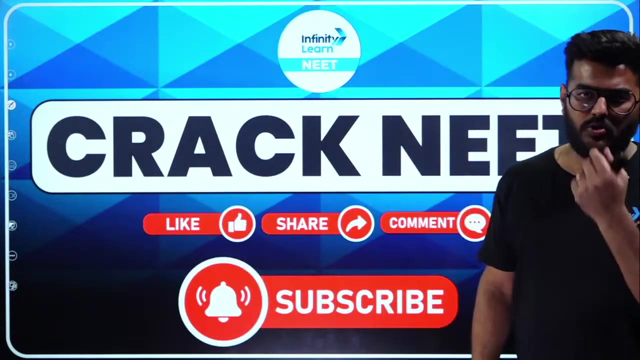 You can see that this is a very big file. It is of 62 pages. So I have time constraint, But you don't have it. You are reading, So all the questions that I have left. I have tried to solve all the questions. 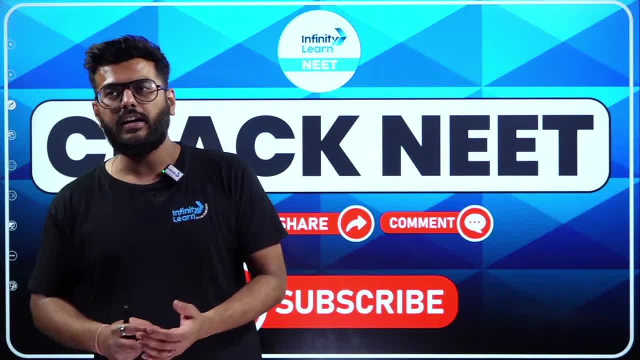 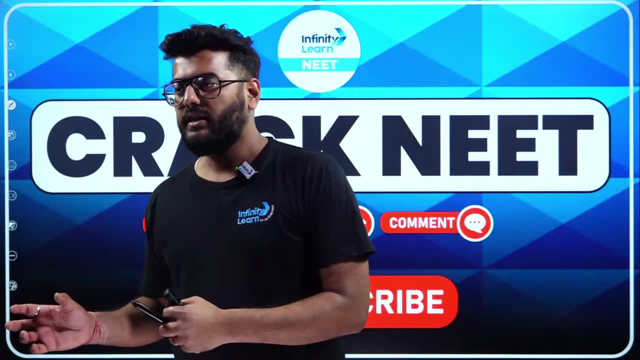 And give you a holistic idea. My agenda for today's session was only one of gravitation and electrostats. You can relate it Like I related it. I have electrostats. I have to give my exam When I studied electrostats. 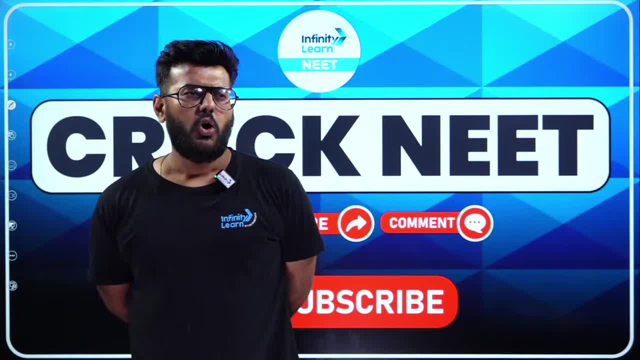 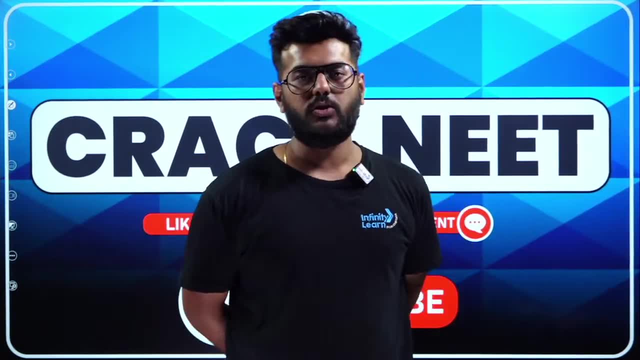 then I started to understand gravitation very clearly And I started to relate it. Same thing with rotational. I relate it a lot. Comparison helps. This is the positive side of comparison. So by doing comparison instead of reading things repeatedly. 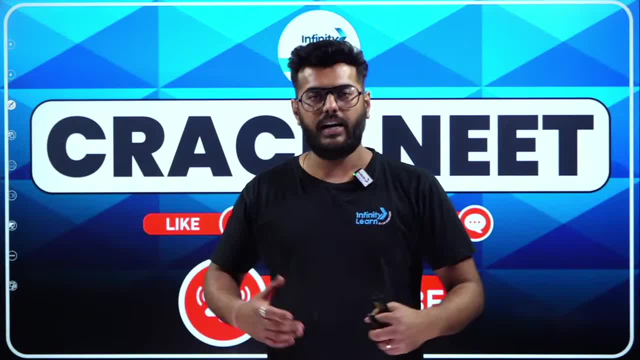 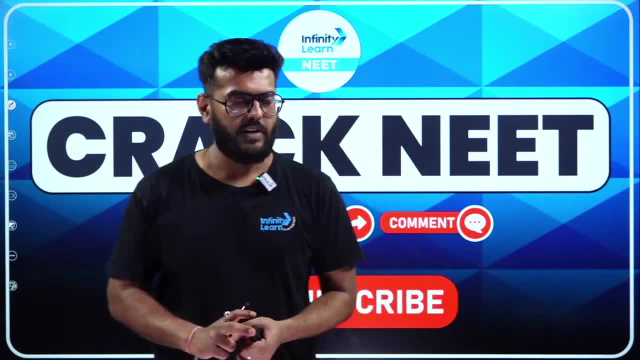 I used to understand it. So that's the same thing for you people as well. You relate gravitation to electrostats, Understand electrostats, but also apply the concept of gravitation, And that's it. I think you must have got some takeaways. 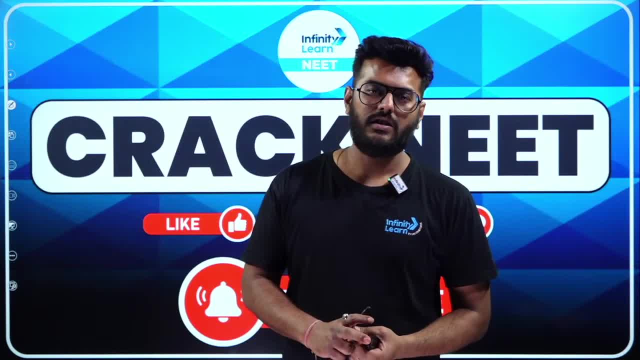 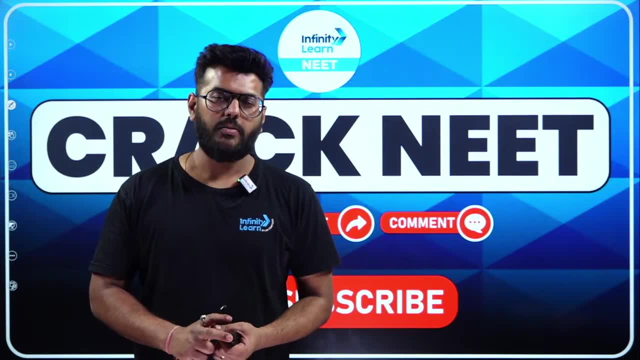 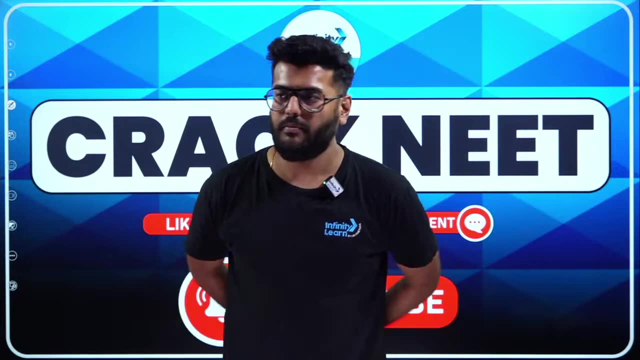 in today's session, Definitely, if you liked it. please like the session And whatever your replies are, any question or any problem, comment box is always open. Please comment. I will try my best to reply personally. See you in the next session. 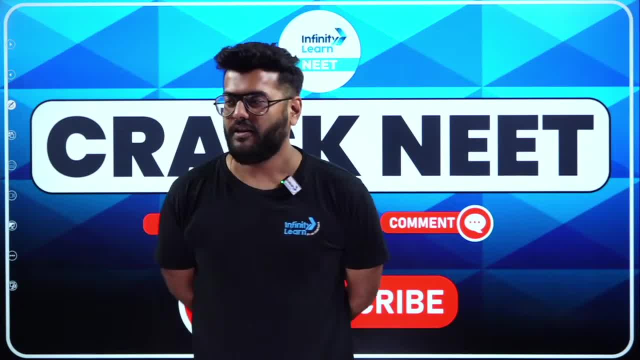 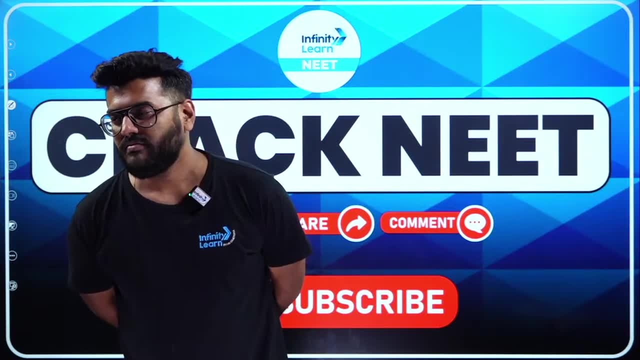 Till then, keep reading, And this time 170 marks. Don't bring it in Physics. That's very, very nice. Abhishek, my heartiest wishes to you. Keep reading. I have to make it for the next 20 days. 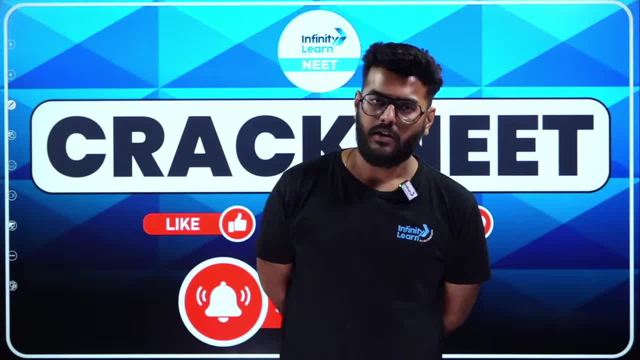 If there is any problem, let me know. I am on Telegram, Telegram, LinkedIn, Insta. wherever I am, I will try my best. 170 marks in Physics- Rest I have to do Bio, Botany, Zoology.